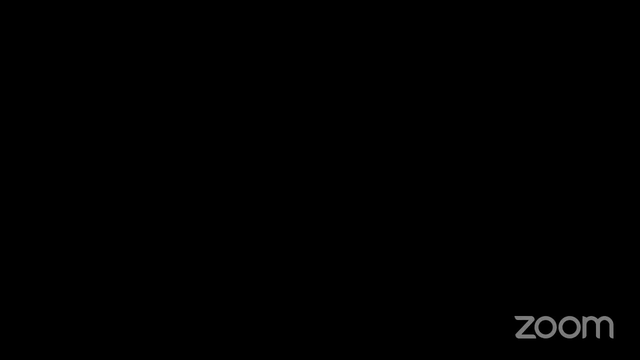 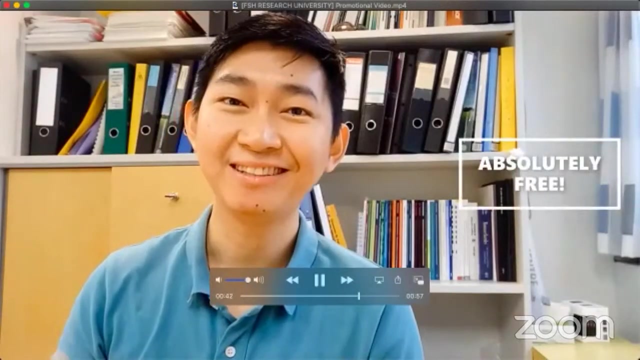 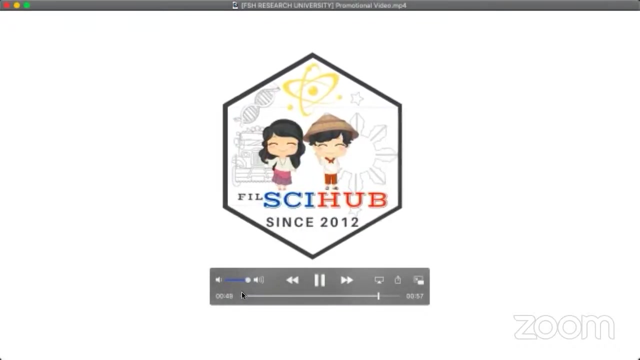 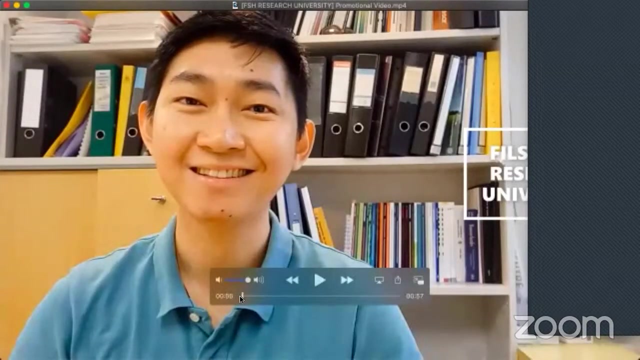 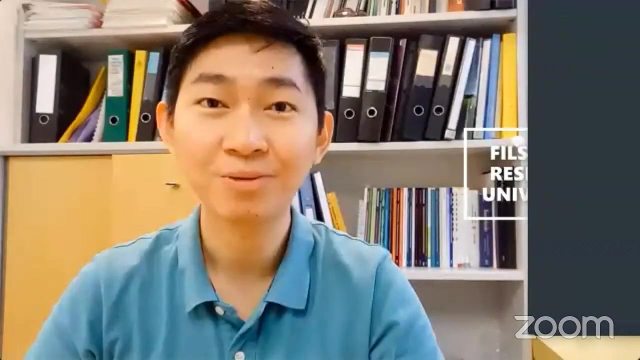 Thank you, And the best part, it's absolutely free. Visit us at philpsihubcom and be part of this learning journey. Let's learn and succeed together here at Philps iHub Research University. Welcome to Philps iHub Research University, your ultimate guide on your next research project. 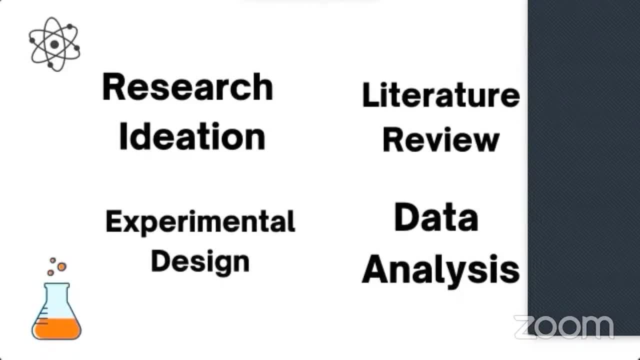 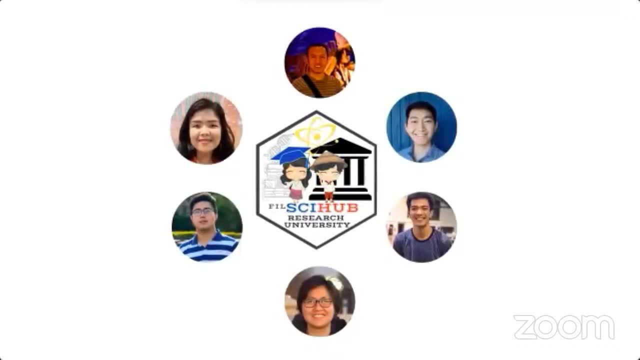 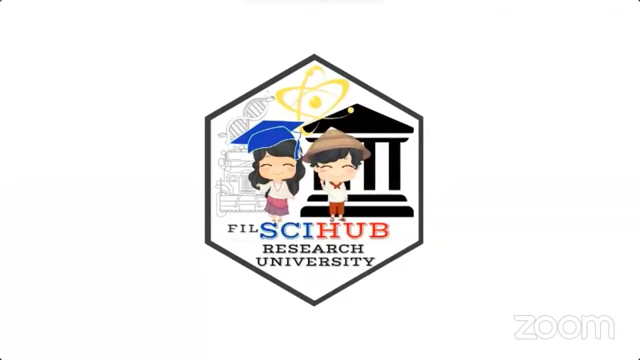 We will lay down the best practices in research ideation, literature review, experimental design and data analysis. to guide you as you carry out your research project. Learn from the Philps iHub team of research scientists and some invited subject matter experts. Philps iHub Research University will be your personal coach. 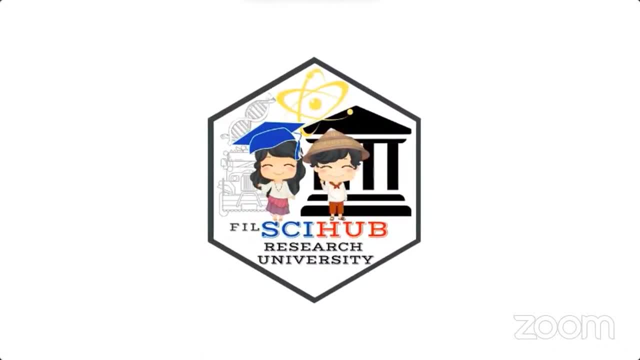 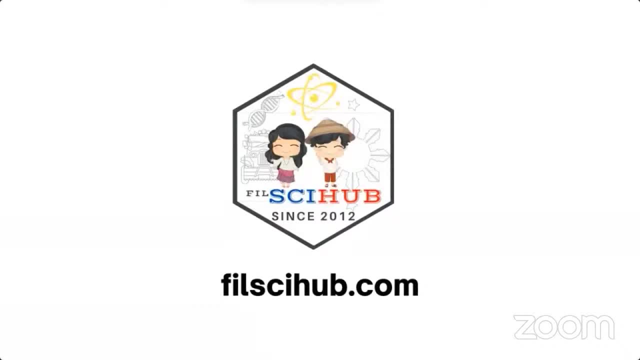 through every stage of your research project, from ideation to final assessment. And the best part, it's absolutely free. Visit us at philpsihubcom and be part of this learning journey. Let's learn and succeed together Here at Philps iHub Research University. 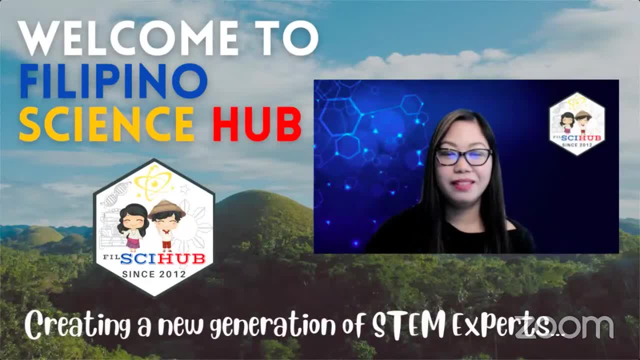 Mabuhay. Welcome to the Filipino Science Hub. Thank you for your continued support to this online platform. To our new participants, thank you for checking us out today and we would like to officially welcome you to Philps iHub. welcome you to the filter hub family. before we start the webinar, i would like to share some 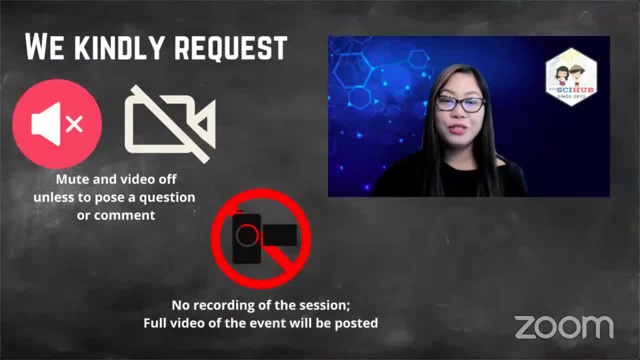 house rules. in order to facilitate a smooth session for our zoom participants, we would appreciate it if you could turn your audio and video cameras off during the webinar. if you have questions or comments, feel free to type them on our zoom chat box or youtube live comments and we will try to accommodate as much questions as possible. 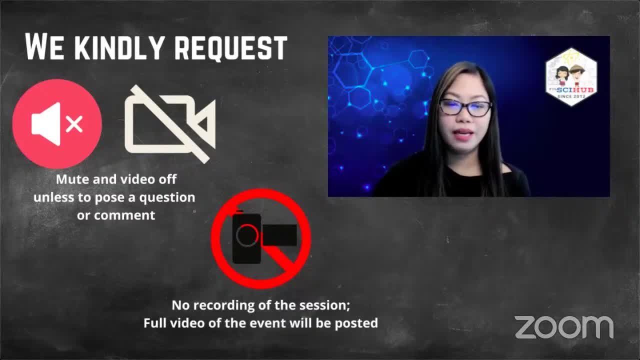 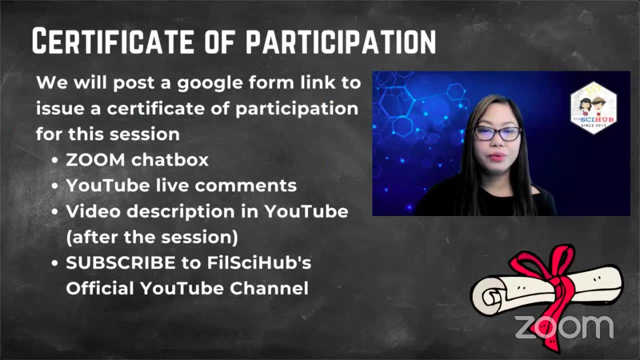 after the talk we will have a 30-minute q? a where the zone participants will have the opportunity to ask their questions live. for those who would like to receive a certificate of participation, a google form link will be posted on our zone chat box, youtube live comments and youtube. 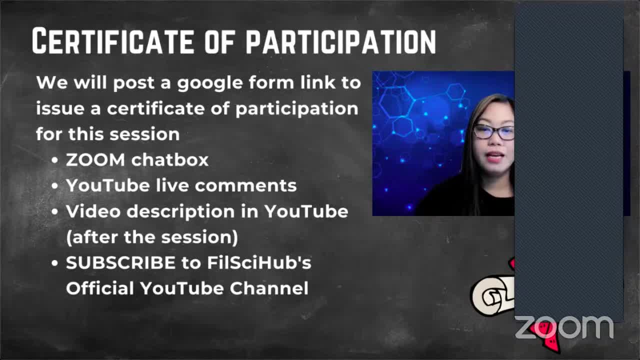 video description towards the end of the webinar. again, welcome to all our zone participants and youtube live viewers. for those who are new and may not be familiar with who we are and what we do are welcome to join our zoom chat box, or the zoom chat box, as well as the zoom chat box. 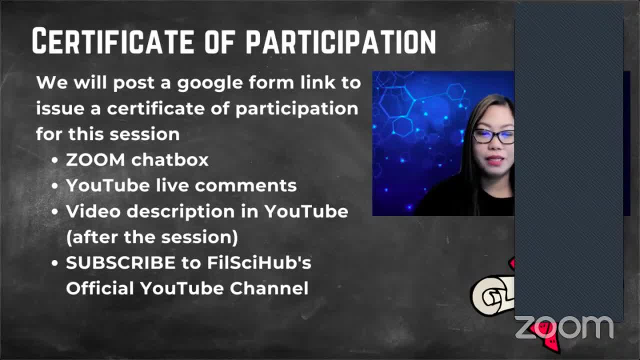 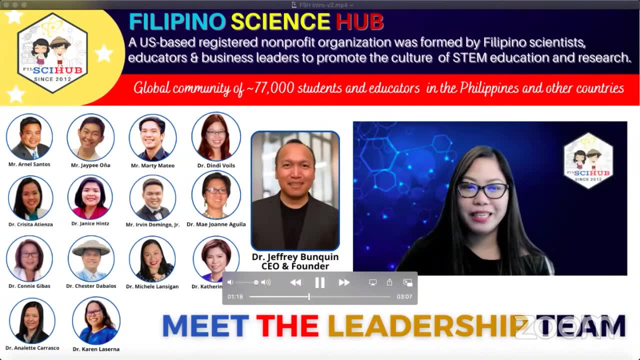 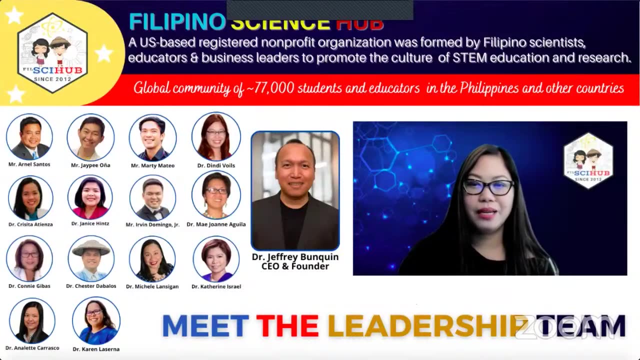 do allow me to share our mission and vision in the next few minutes. Filipino Science Hub is an online platform founded by our CEO, Filipino scientist, Dr Jeffrey Camacho-Monquin, back in 2012.. Currently, we are a registered non-profit organization based in Houston, Texas, United. 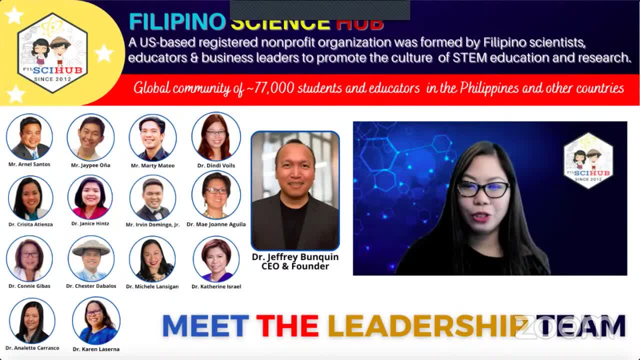 States. Our vision is to promote STEM education and the culture of research among students and teachers in the Philippines and abroad. Our current global leadership team is comprised of volunteer Filipino scientists, seasoned STEM educators and business executives across the globe. Our vision is to see a technology and innovation-driven Philippines, and we believe 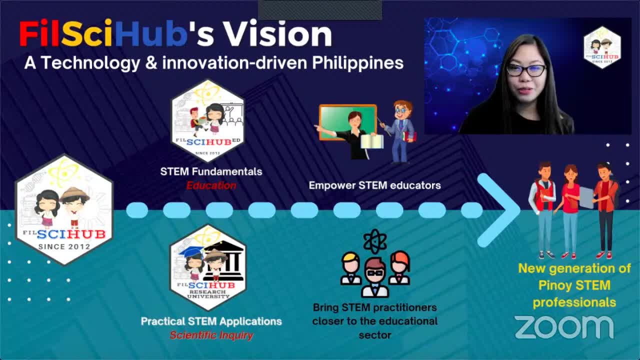 that this can be achieved by creating a new generation of well-rounded Filipino STEM enthusiasts. The vision is being carried out by our two major programs: the Filsa Hub Ed program and the Filipino Science Hub. Our vision is being carried out by our two major programs, the Filsa Hub Ed program and the Filipino Science Hub program. 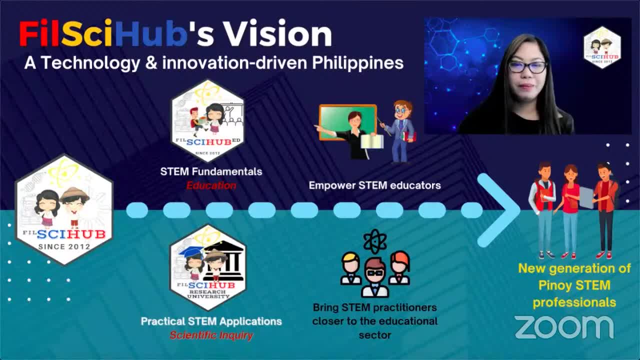 Through Filsa Hub Ed, we are able to empower and support our teachers by strengthening STEM fundamentals education. We believe that this is important because the more equipped our STEM educators are, the more they can inspire students to pursue a career in science, technology, engineering and mathematics. The other major program that drives our vision forward is 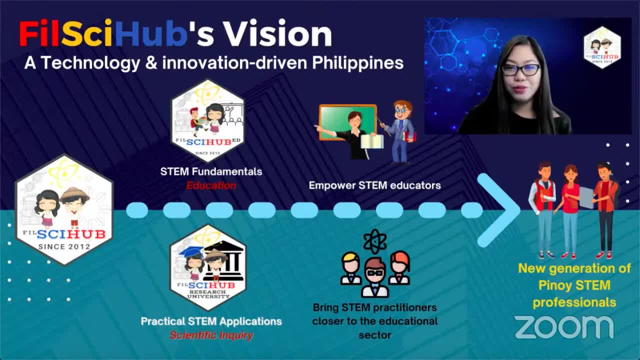 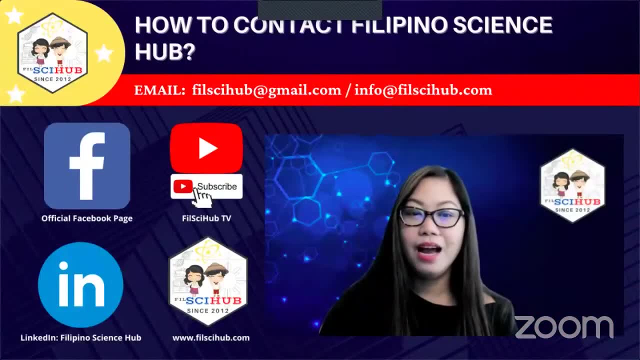 Filsa Hub Research University. This is where we provide tools for fundamentals of research and bring practicing scientists closer to the educational center. Our official website is wwwfilsahubcom. This is where you can access all our materials, such as webinars, tutorials. 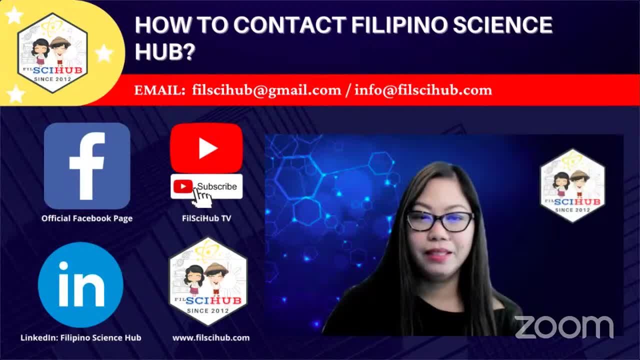 modules, virtual lab and features, all of which are free. We are also present in several social media platforms, so follow us wherever you are most active on to get updated with our work events. Again, thank you for being with us this morning To officially start our 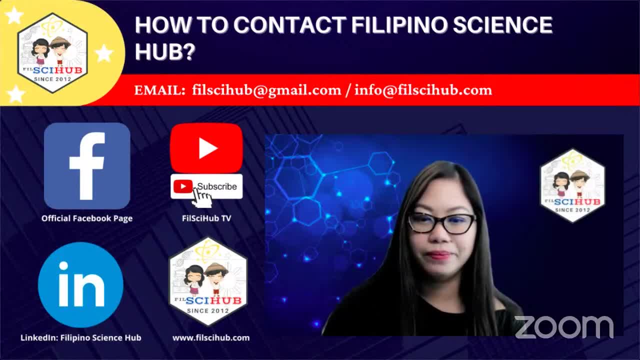 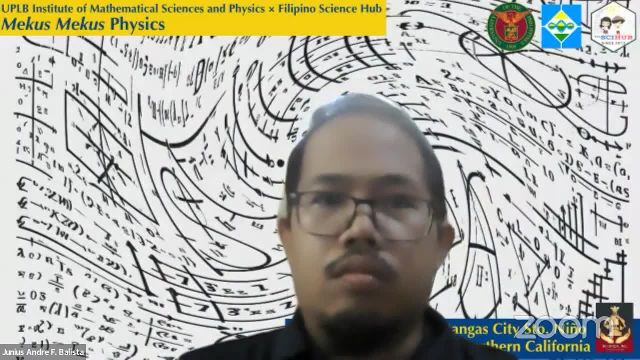 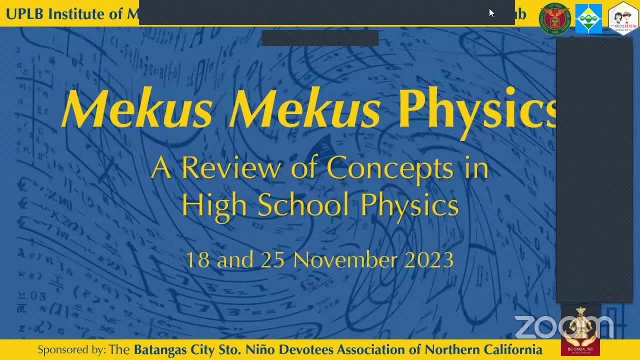 webinar. I would like to turn the virtual floor over to our host today. Good morning, Good morning Morning. Is my audio clear? Yes, Good morning clear, All right, Good morning everyone. God morning participants. This is my presentation. 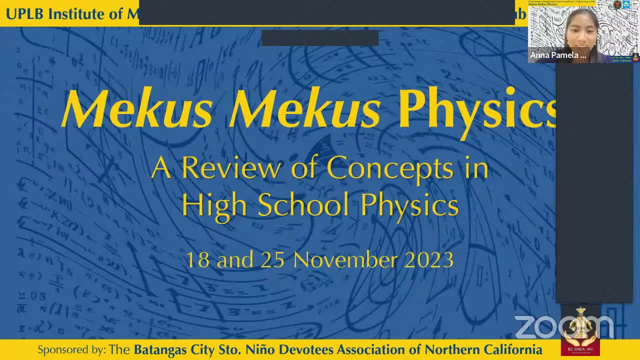 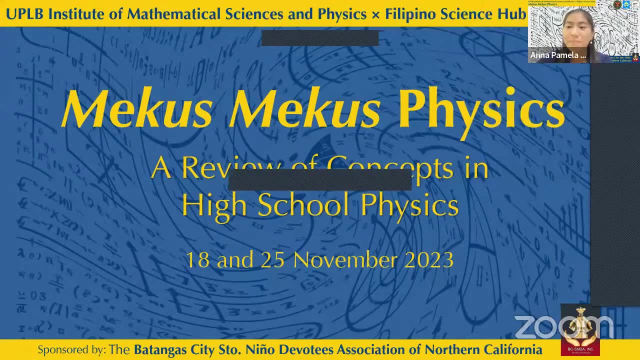 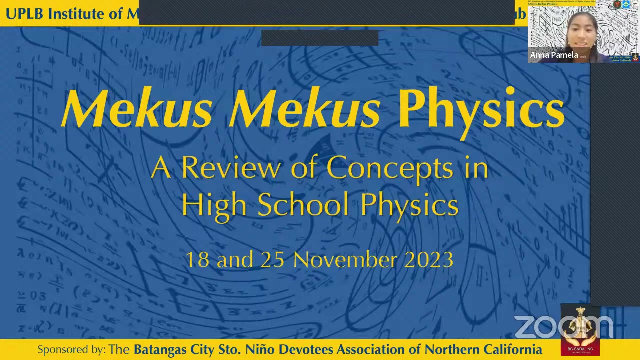 Greetings, Welcome to MECOS-MECOS Physics: a review of concepts in high school physics. I am Ana Pamela Odezus, a faculty member of the UPLB Institute of Mathematical Sciences and Physics. This event is hosted by UPLB IMSP and Filipino Science Hub and sponsored by the Batangas City Santo Nino Devotees Association of Northern California. 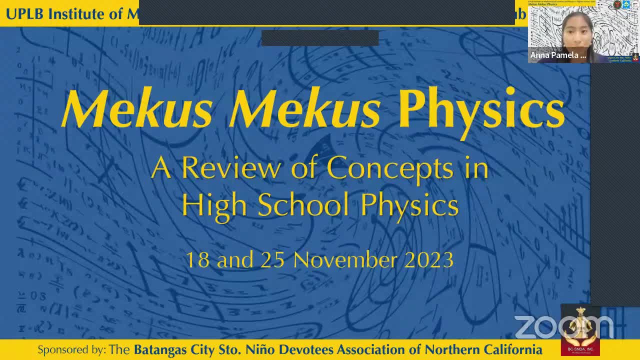 This is a two-part series, so it's happening today and also next week, November 25,, in which participants will be hearing from resource speakers who will share their knowledge on some high school concepts in physics. And so, to start off our event, I would like to call on the IMSP Director, Dr Editha C Jose. 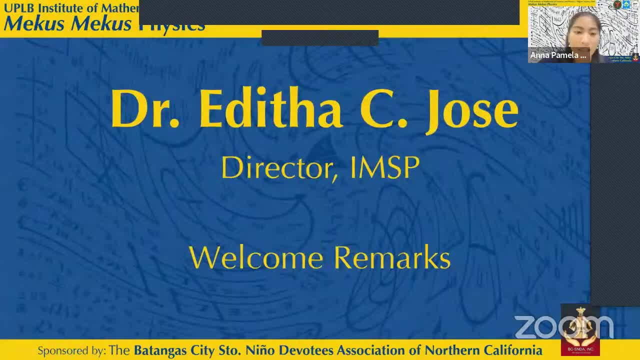 followed by the founder of Filipino Science Hub, Dr Jeffrey Camacho-Bunkins, for their opening remarks. Thank you, Ella. Thank you, Ma'am Ella. Magandang umaga sa ating lahat at Kaiser Jeff na nasa US. Magandang gabi sa iyo, dyan. 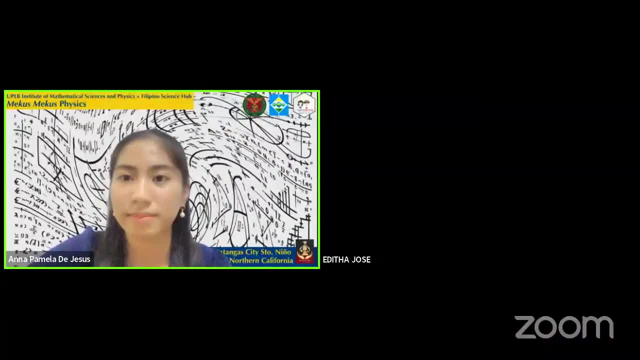 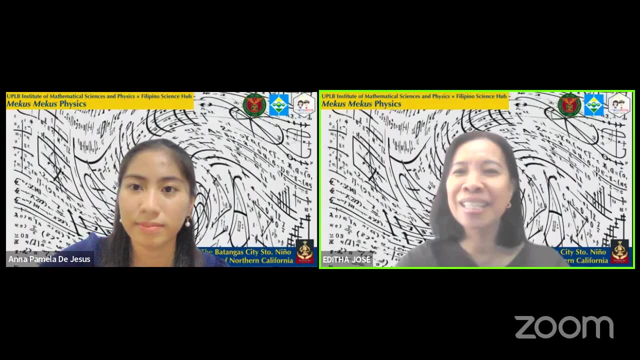 So again, magandang araw sa ating lahat. On behalf of the Institute of Mathematical Sciences and Physics University of the Philippines, Las Banas, I would like to welcome everyone to this two-part webinar about some identified physics concepts which are deemed to be the least mastered by students. 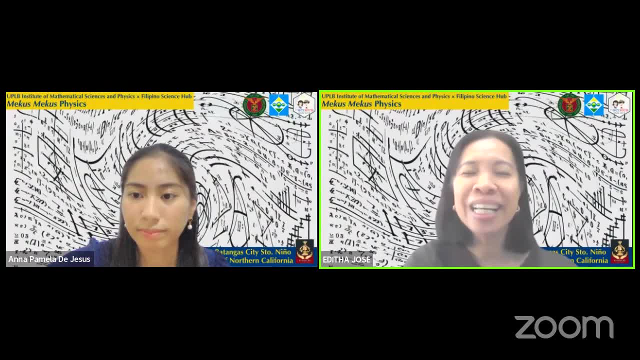 So, for the end time, the IMSP, in partnership with Filipino Science Hub, or PhilSci Hub, which is headed by my student, former student, Dr Jeffrey Bunkuin, are joining forces in our common pursuit to uplift the quality of STEM education and research in the country. 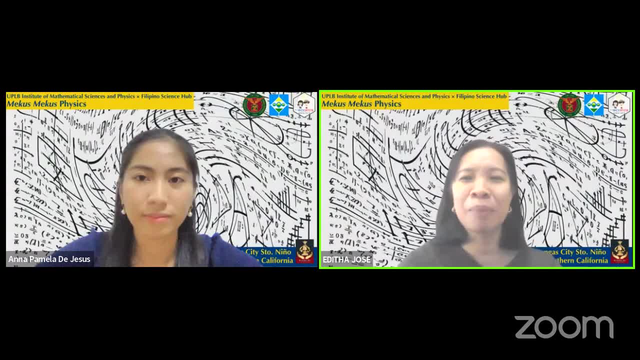 And, at the same time, promote the wonders and power of mathematics and physics. Our institute, the IMSP, is enthusiastic again with regard to co-staging this highly anticipated activity. So, Sir Jeff na yung mag-share mamaya, So last October 2022,. 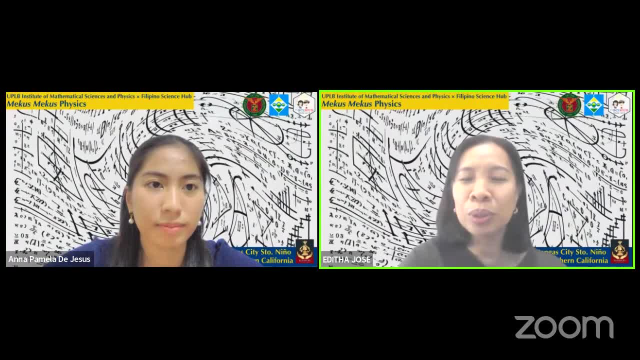 So last October 2022, we featured some DIY or do-it-yourself physics experiments prepared by our physics faculty members, So they presented innovative and creative set-ups in teaching physics. It was a blockbuster event and we promised PhilSci Hub that we will offer it again. 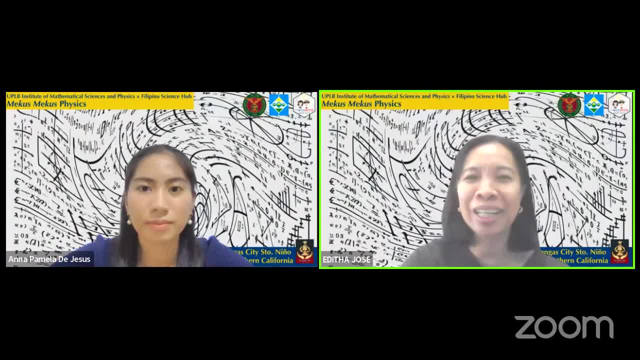 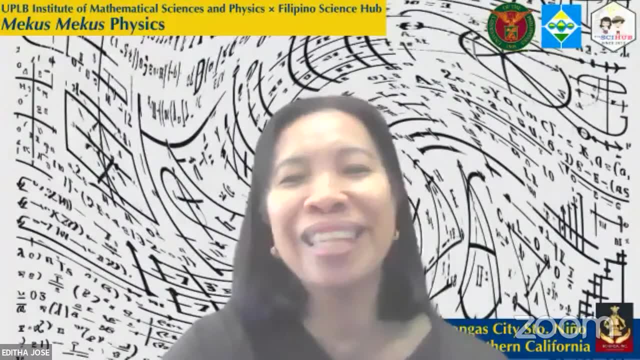 But this time we are offering a different format. But this time we are offering a different format. But this time we are offering a different format. Though physics pa rin So coincidentally So on Monday, November 20, 2023,. 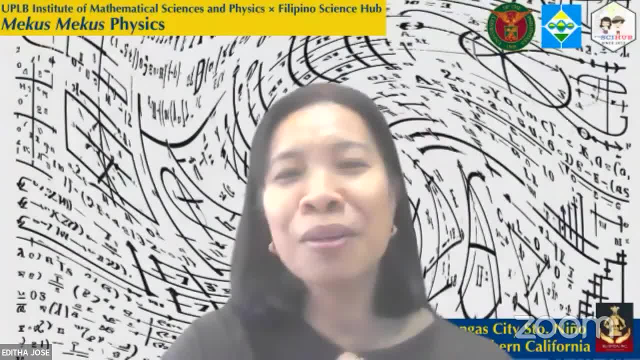 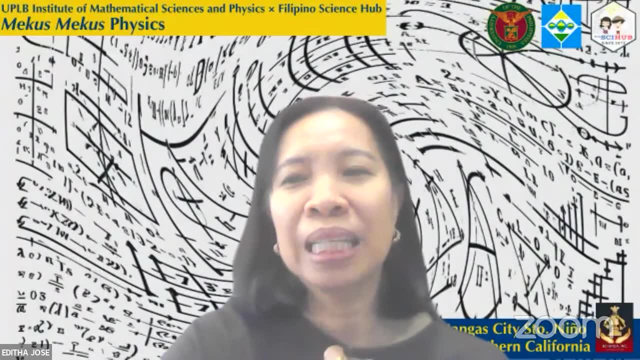 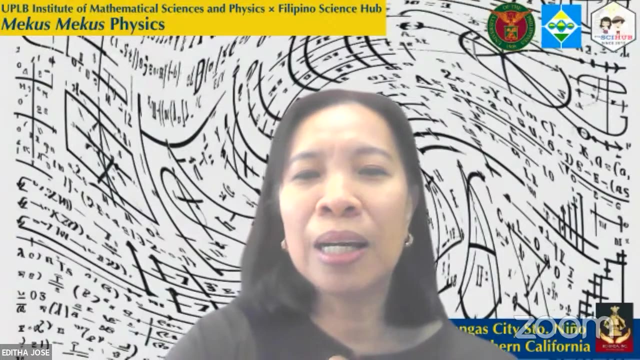 we will be conducting a symposium on astrophysics, particle physics and nuclear physics, And I would like to take this opportunity to invite you all. Maybe later we will send you the Zoom link to this hybrid event. I truly appreciate and thank our speakers for this webinar, Dr Junius Andre Balista and Dr Eduardo Concing, the Extension Committee of the Physics Division for the Logistics and Organization and, of course, to PhilSciHub. 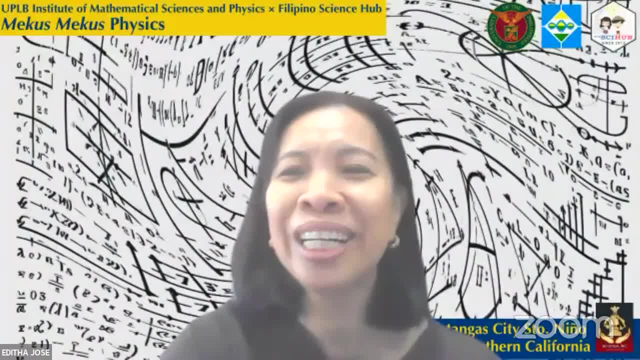 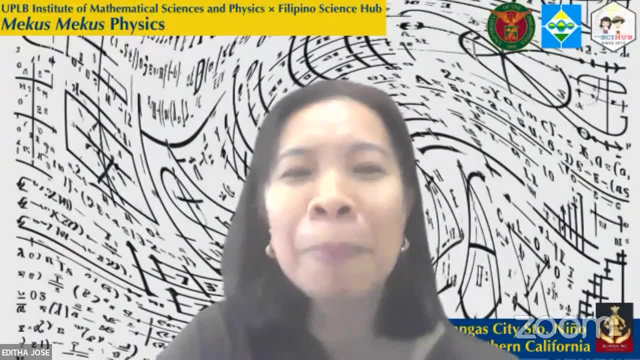 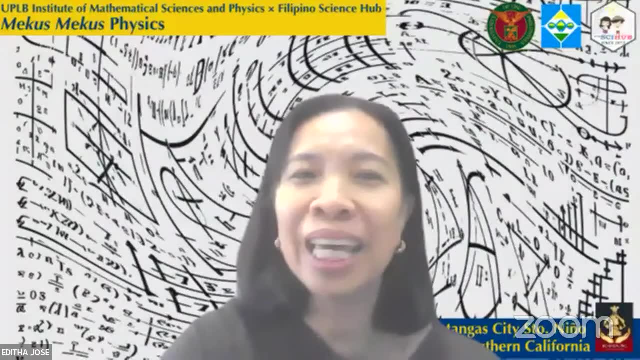 Thank you very much, And to our sponsor, the Batangas City Santo Nino Devotees Association of Northern California. To all our participants, thank you for your participation and we hope that this activity will be helpful and useful to all of you. 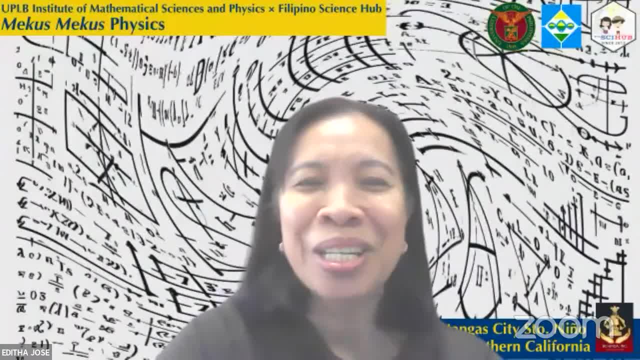 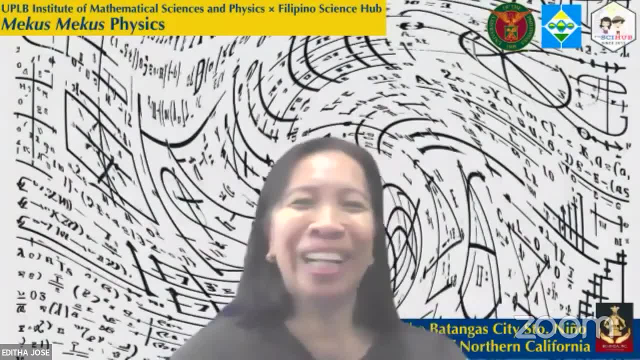 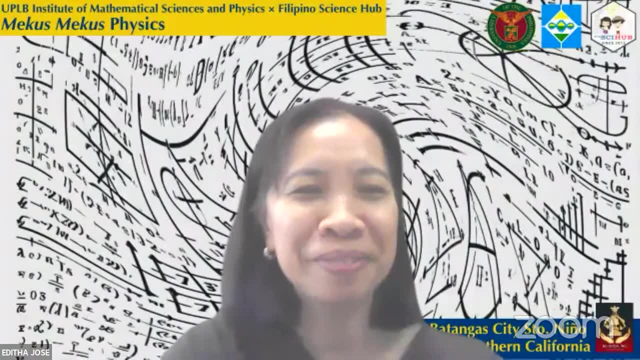 So, without further ado, mga insan imekos-mekos, na natin ito Ayun. Magandang umaga sa ating lahat. Alright, magandang umaga po sa ating lahat. Ako po si Jeffrey Bunkin. I'm a Filipino scientist, a former student of Dr. 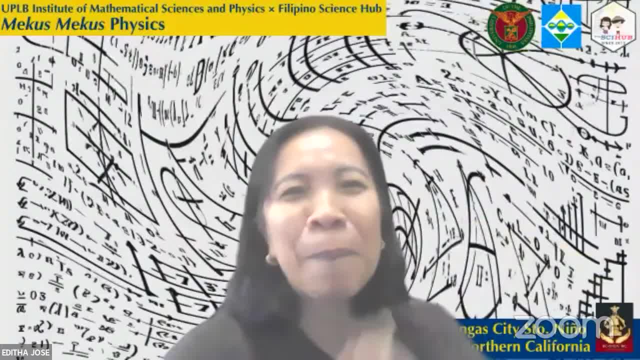 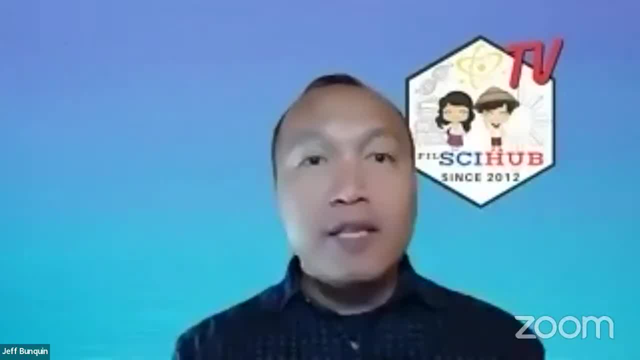 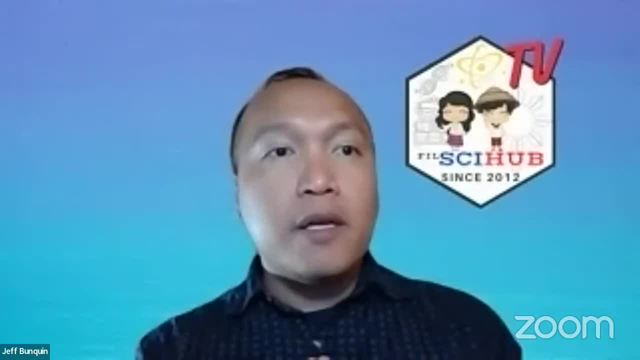 Edica Jose in mathematics, and my undergraduate physics background was actually honed at the Institute of Mathematical Sciences and Physics of the University of the Philippines at Los Baños. So I'm the founder and the current chief executive officer of Filipino Science Hub. So we are very happy to again collaborate with the Institute of Mathematical Sciences and Physics at UPLB for this event. 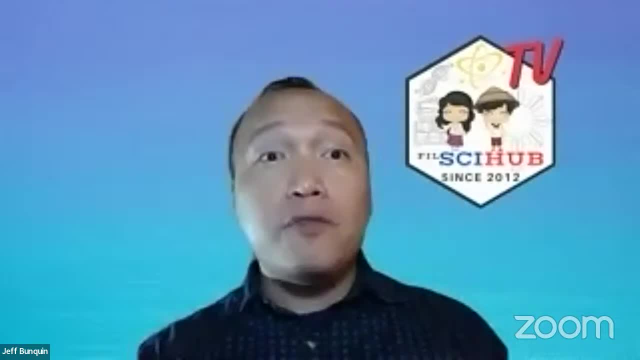 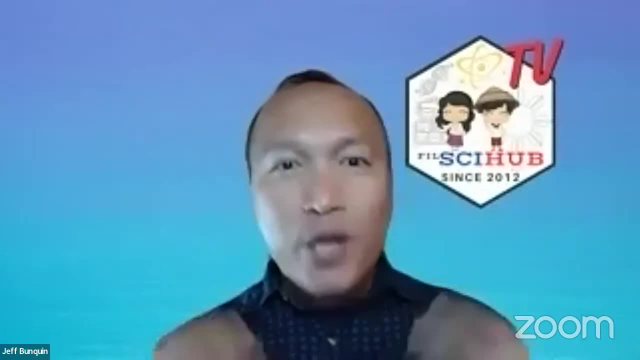 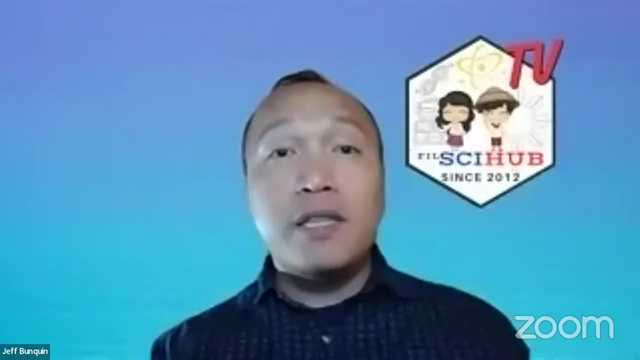 So, as mentioned po in our introductory video, Filipino Science Hub has been partnering actively with established institutions from different parts of the world And we try to bring you some of the leading Filipino scientists and leaders in STEM education para po maihatid namin sa inyong mga guro at mga mag-aaral ang mataas sa kalidad ng pagkatuto at pagtuturo ng STEM. 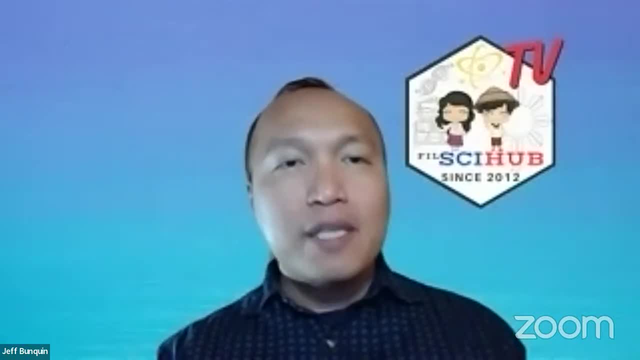 At sa ngayong araw po ito. We're actually happy that IMSP graced us once again, But then this time around they chose to focus on topics in physics that are not always learned in the best possible way. So yung pong gap na yan, yung ipibridge ng ating mga kasamahan sa IMSP. 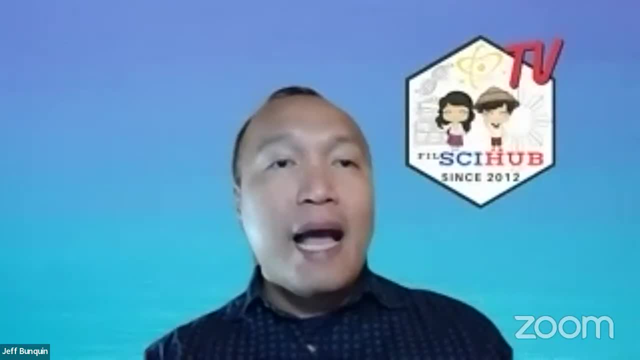 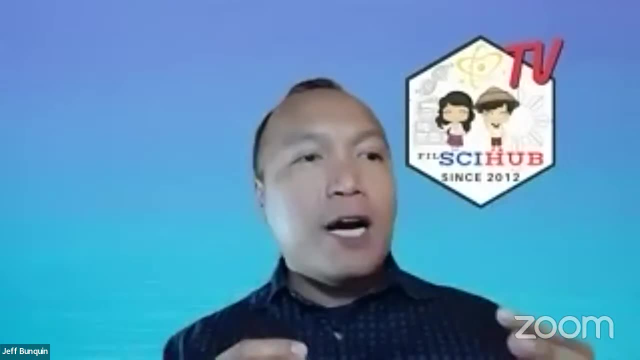 And we're also very thankful to the Batangas City Association of Santo Nino Devotees based in California. So this is an organization of Filipino-Americans po who have migrated to the Bay Area in San Francisco And since the 1970s po they've been very charitable sa ating mga kababayan. 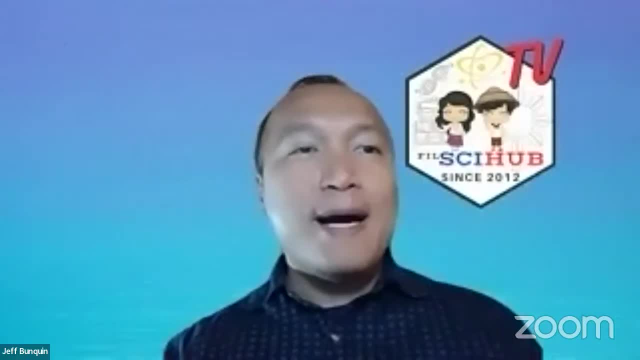 So they raised money. po, which also, in part, is sponsoring this event, And so, without further ado, po, I would just like to welcome you all to this event. I would like to thank everyone who joined, Who joined us today in Zoom and those who dialed in by YouTube. 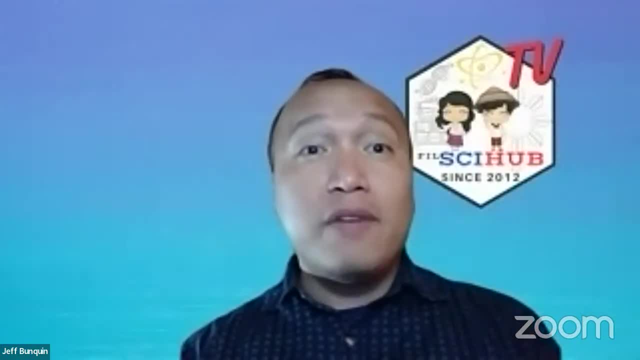 So we hope that you enjoy this event- And, by the way, this is a two-day event, nga pala po- So we hope that you don't only join us today, but we also hope to see you again next week. All right, 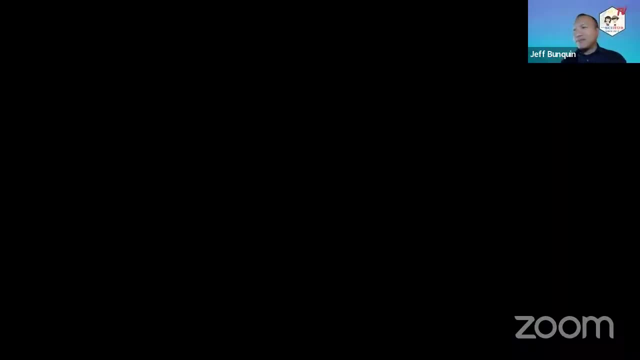 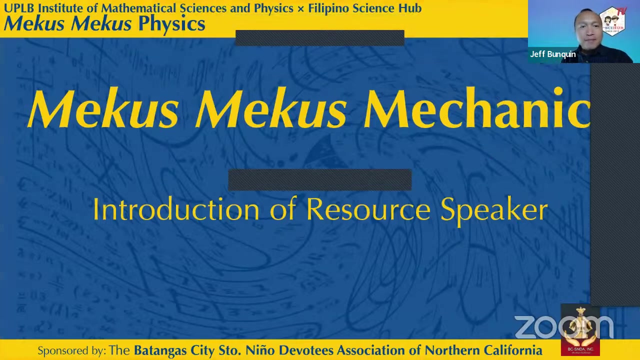 Ma'am Ella back to you. Thank you, po, Ma'am Edith and Sir Jeff for the warm welcome And thank you again, Sir Jeffrey, for allowing our institute to partner with you To go with Filipino Science Hub For this event. 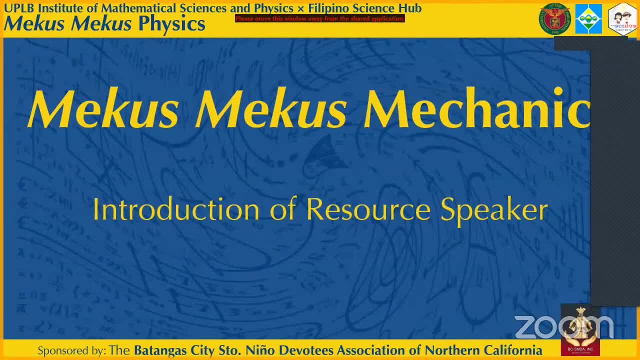 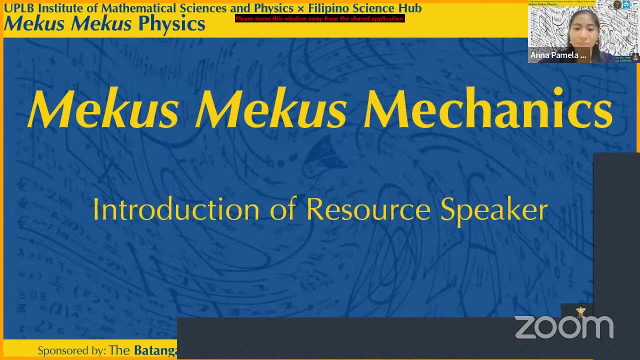 Okay, I hope everyone is ready and expectant to learn from our resource speaker. Okay, So our resource speaker for this morning is an associate professor in physics at the Institute of Mathematical Sciences and Physics, UPLB. He obtained his bachelor's degree in applied physics in UP Diliman Cumlaude. 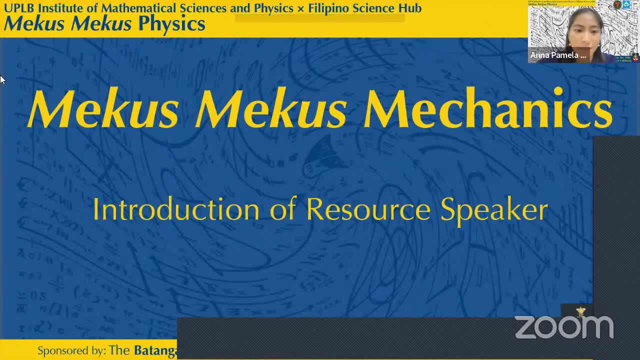 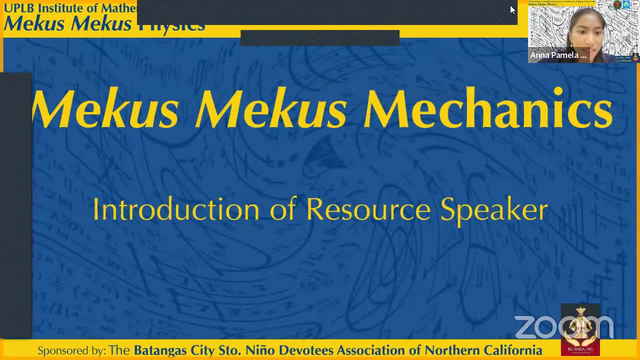 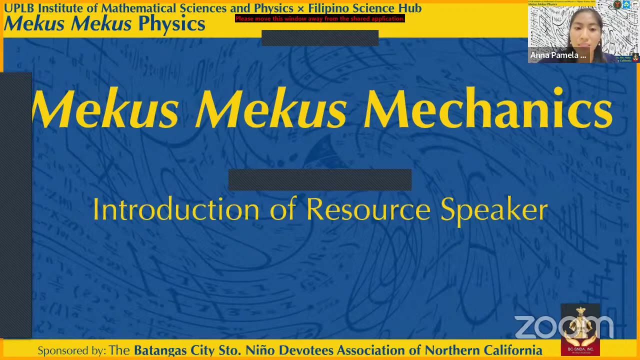 And proceeded with his master's and doctorate degree in physics. He has taught courses in classical mechanics, statistical physics, electromagnetic theory and research methods in physics. He also made minor contributions in the early phases of the curricular development of physics courses in K-12.. 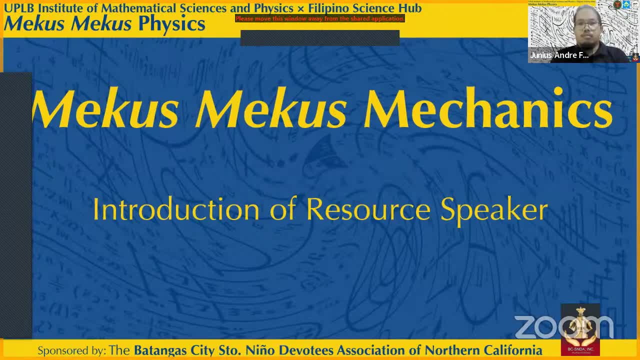 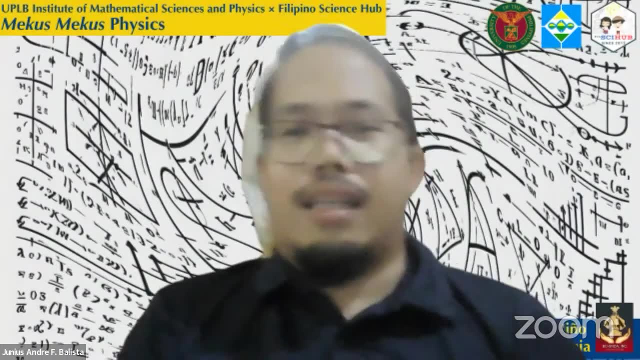 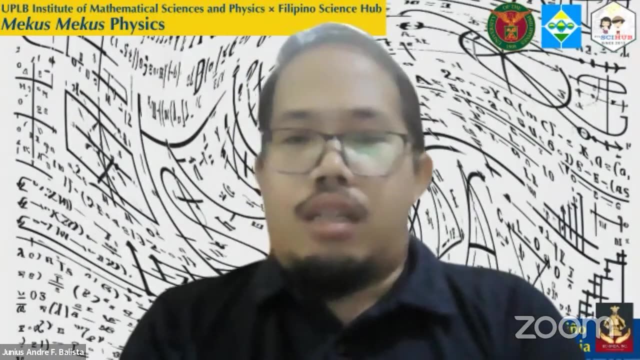 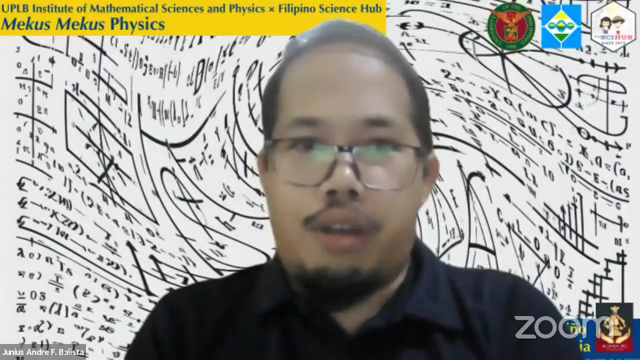 Ladies and gentlemen, please welcome Dr Junius Andre F Balista. Good morning, Good morning. Good morning. So I'm Junius and I will be your resource person for today's topic. Okay, I'll share my screen Shall I. 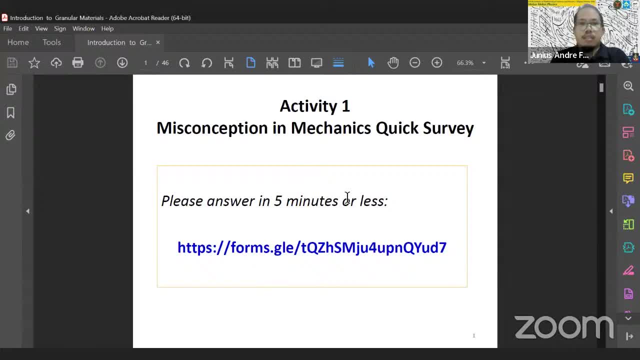 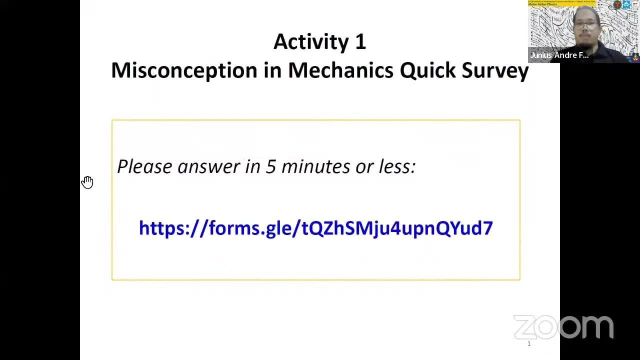 Yes, sir, Okay, Full screen, Okay, Okay, Full screen. Yes, sir, Okay. So, by the way, I requested you to answer a very short quiz, So basically it's an excerpt of a mechanic survey. This will be our conversation piece for this topic. 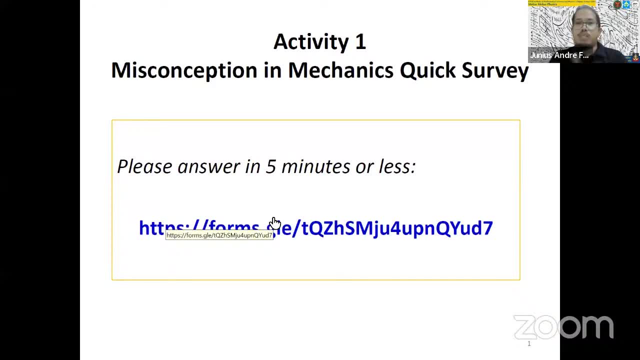 So it's just a short quiz and so that you can better appreciate the topic, And we will share the result in aggregate. so no need- no really need- to worry about this topic. So it's just a short quiz so that you can better appreciate the topic. 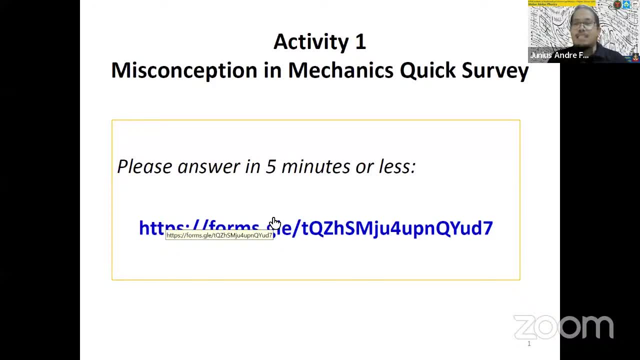 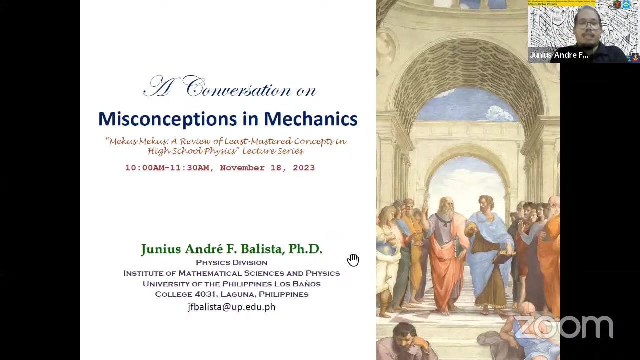 just answer it as honestly and as quickly as you can, okay, so. this is so. yes, sir, um, so, please, uh, spend a few minutes uh answering this, okay, so, just to start now, our, so i am, but again i'm genius- andre f palista, and uh, today we're going to have a conversation. 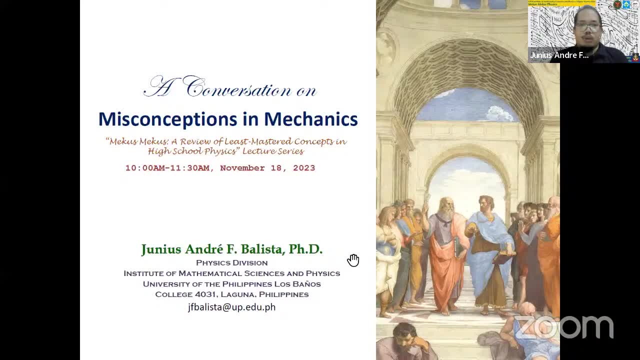 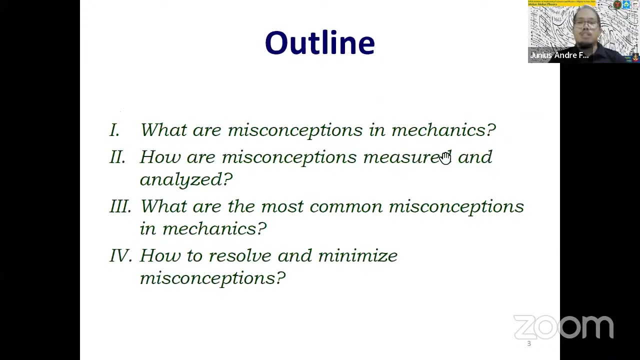 on misconceptions in mechanics. so, uh, this is the first part of the lecture series review of at least of least mastered concepts in high school physics. okay, so, so today, uh, we're going to answer the questions: uh, what are misconceptions in mechanics to mean by that? and uh, how are misconceptions measured and analyzed? and then, uh, we are, what's uh answer? 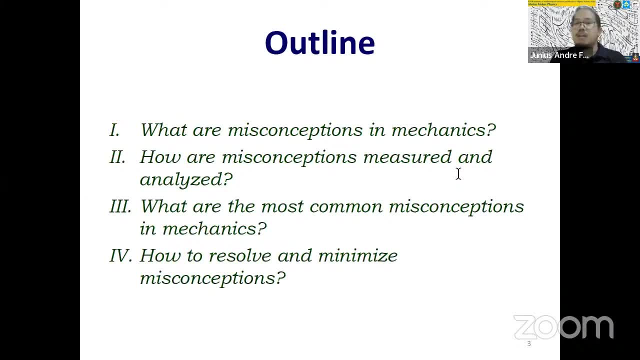 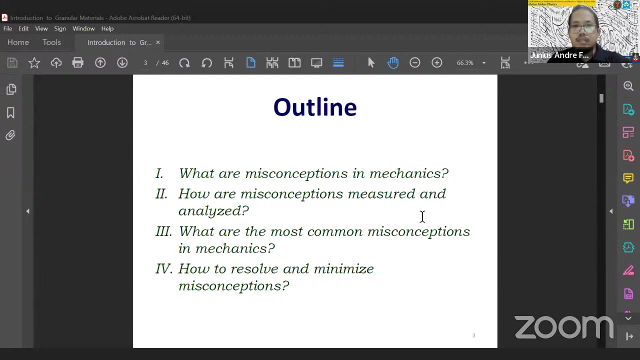 the question: what are the most common misconceptions in mechanics, at least according to one recent research study, and i'm going to uh offer uh ways to resolve and minimize uh misconceptions. okay, so maybe i'm going to pause, uh give a breather. first, uh, please, for you to answer the survey. 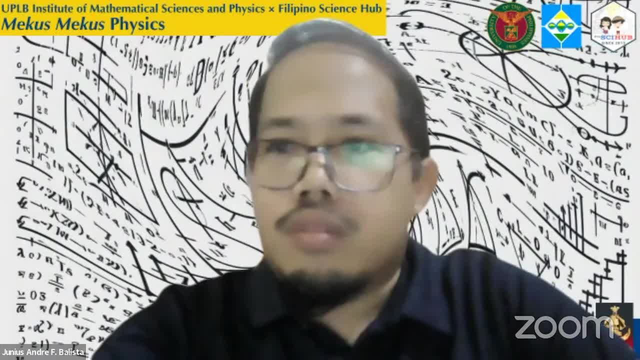 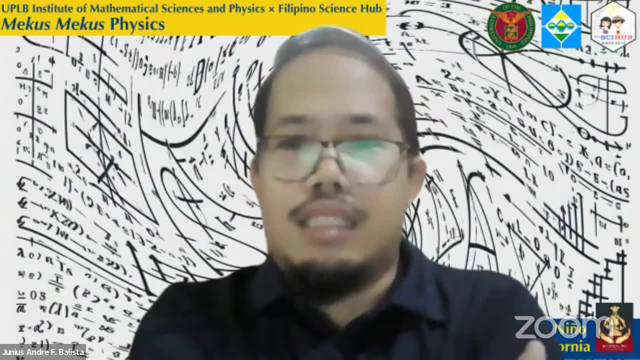 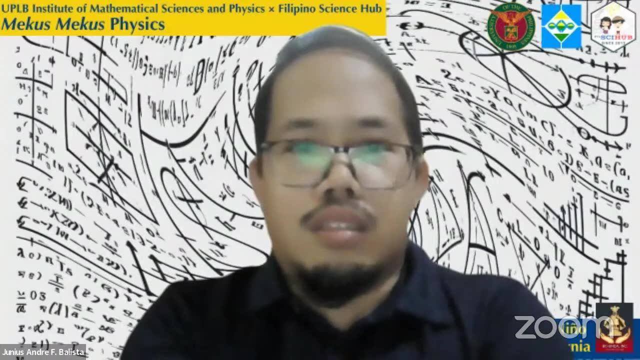 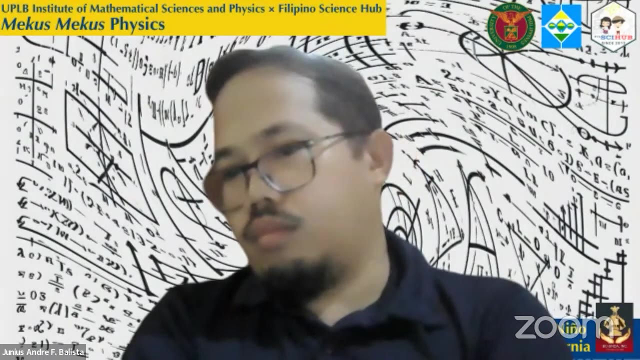 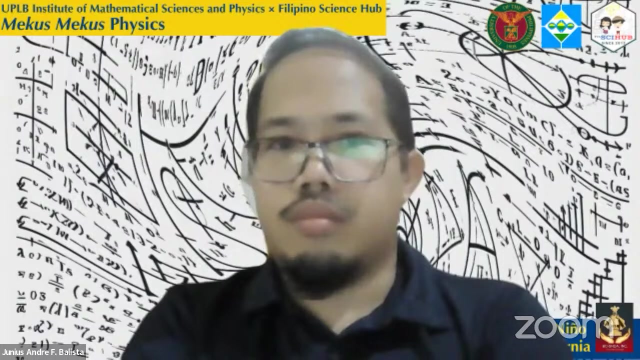 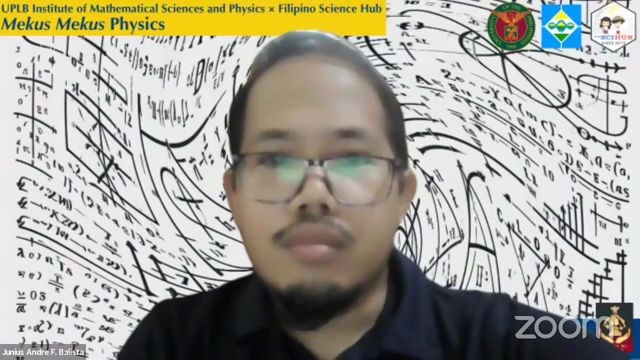 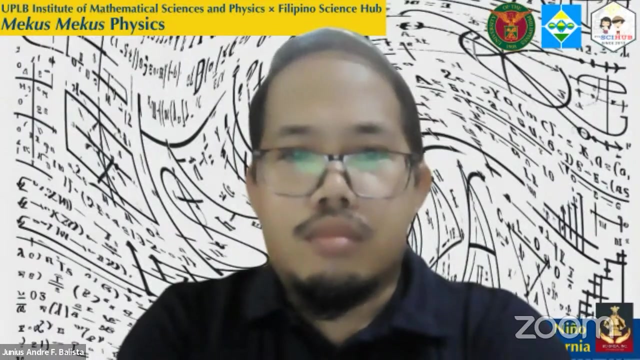 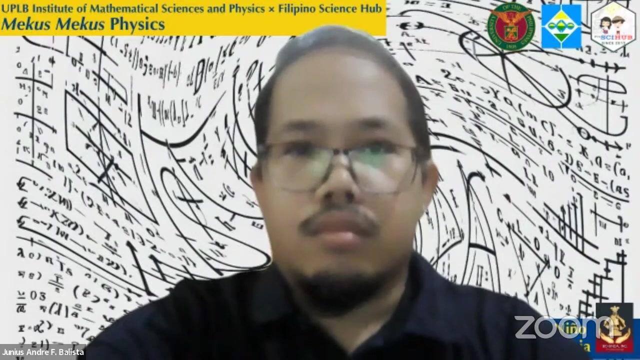 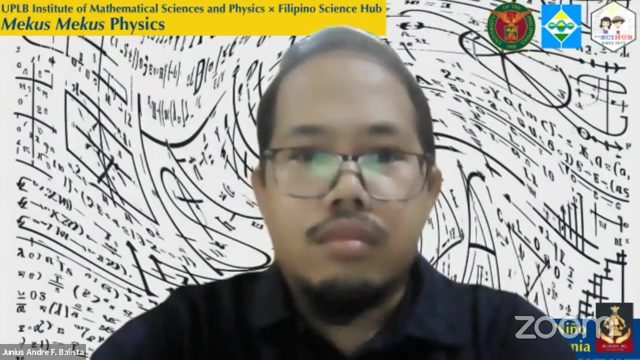 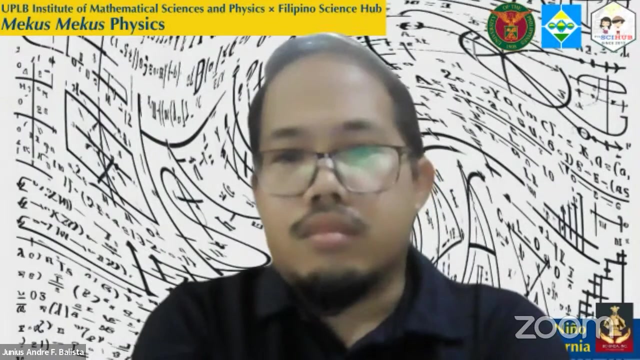 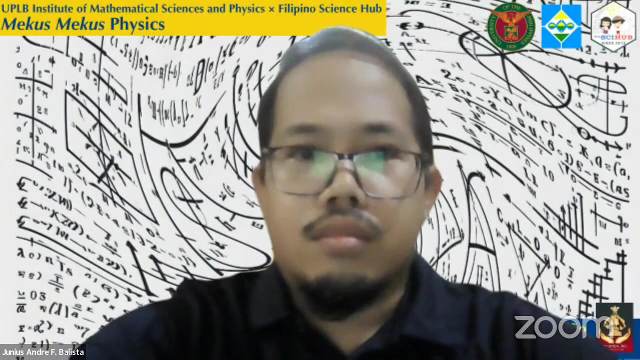 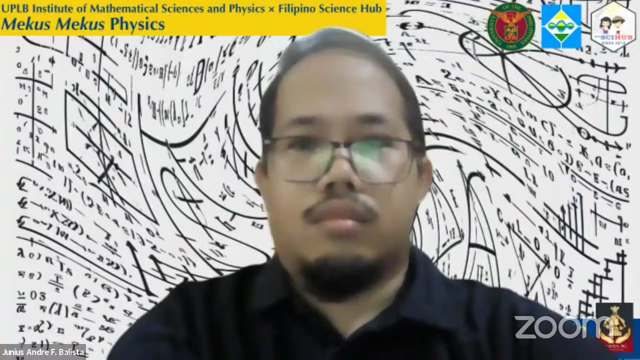 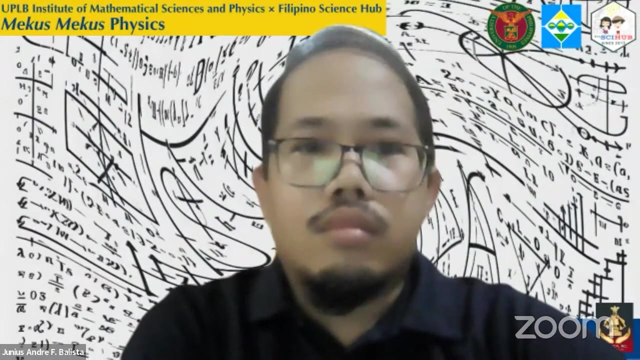 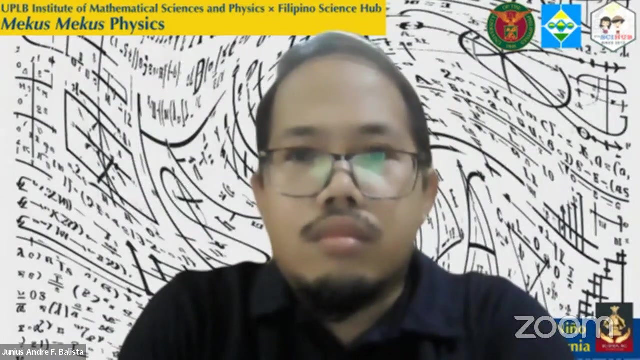 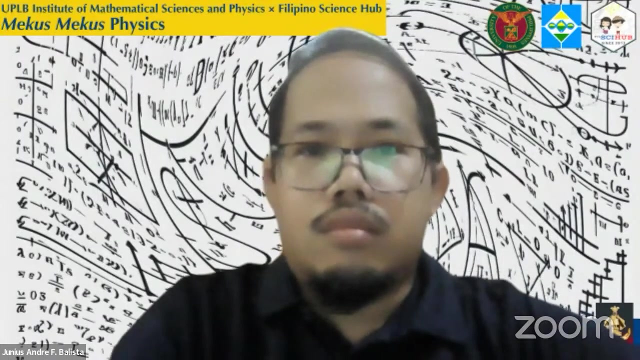 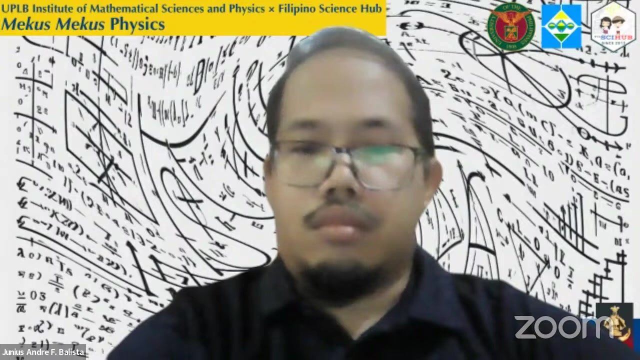 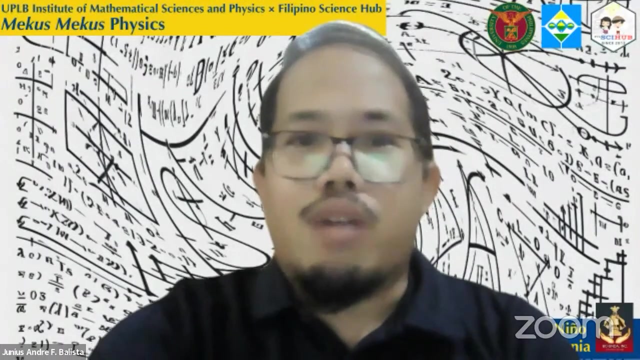 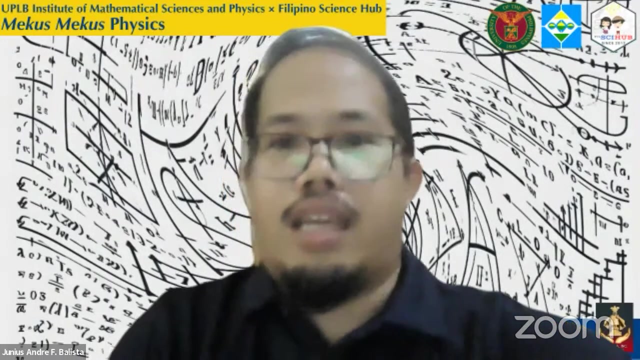 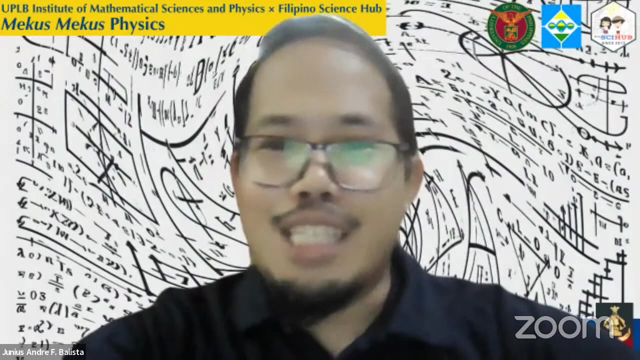 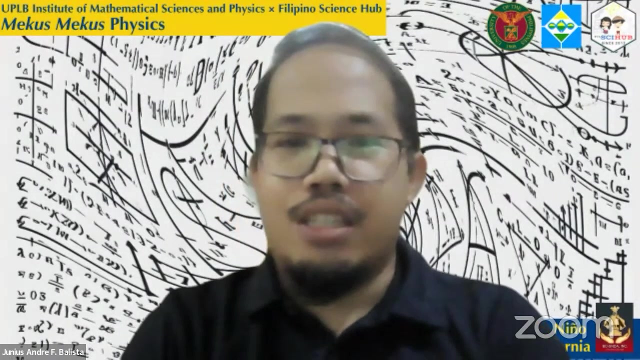 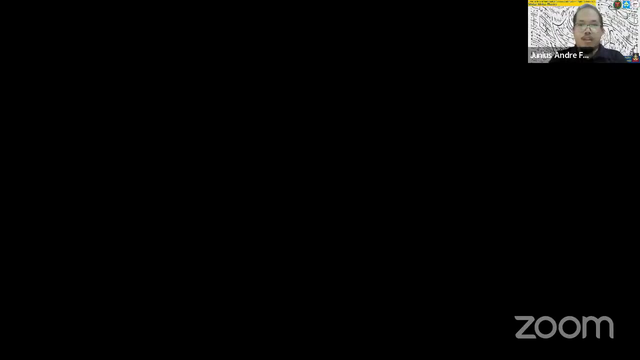 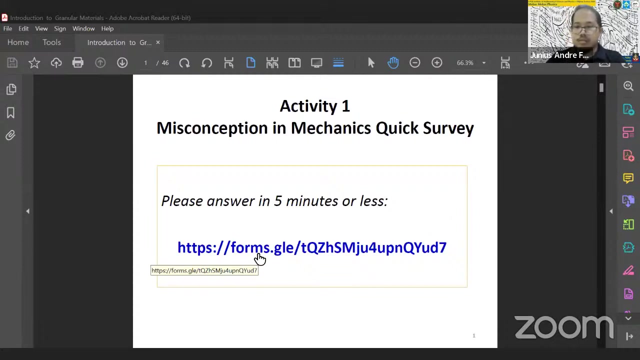 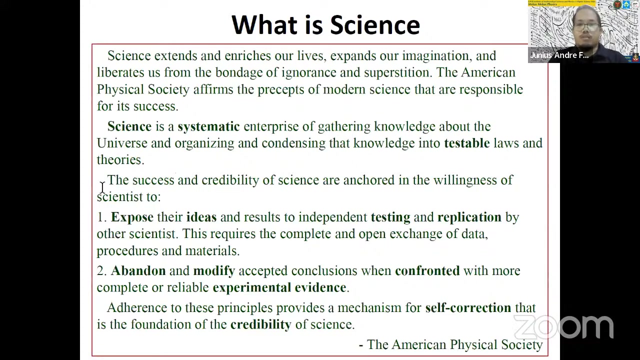 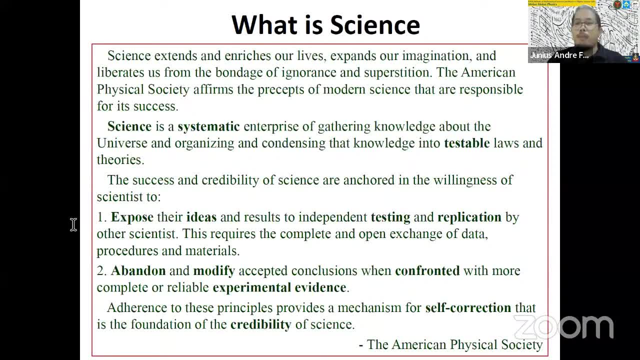 studying science. it's a good way to even approach our challenges in teaching and learning physics in a scientific way. So just to refresh you, I've defined the science. I find a good definition and I think it's applicable to the whole field of science. but I found the American Physical 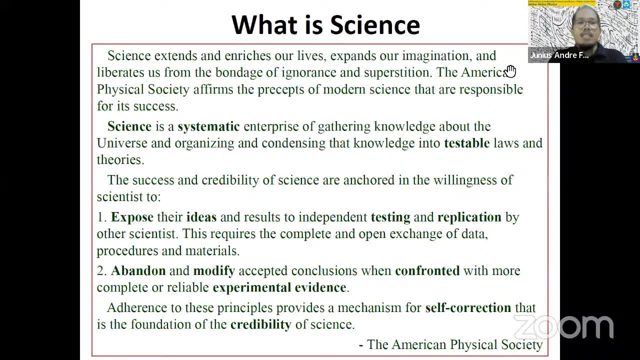 Society. nicely written. So science extends and enrich our lives, expands our imagination, liberates us from the bandage of ignorance and superstition. The APS affirms the precepts of modern science that are responsible for its success. So science is a systematic enterprise. 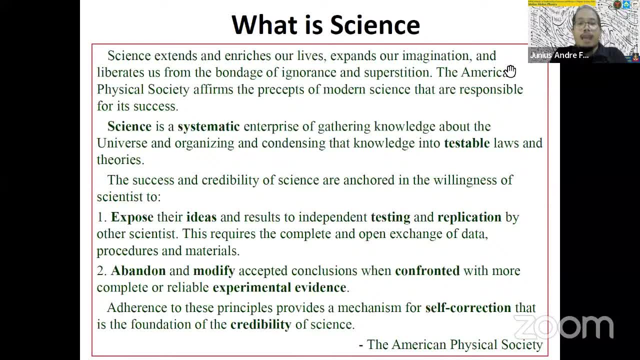 of gathering knowledge about the universe and organizing and condensing that knowledge into testable laws and theories. The success and credibility of science are anchored in the willingness of modern scientists to develop their knowledge so we can achieve the same of scientists and in this case, teachers and students. 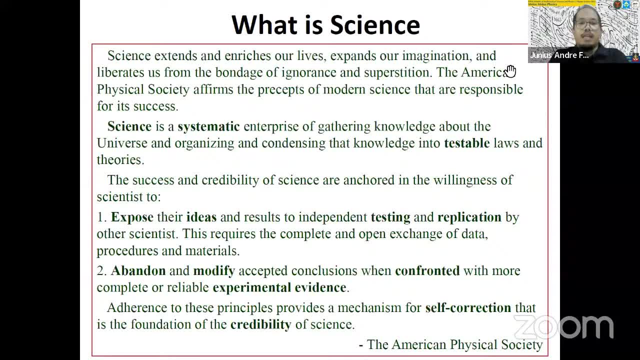 in science to expose our ideas and results to independent testing and replication by other scientists. This requires to complete an open exchange of data, procedures and material, and to abandon and modify accepted conclusions when confronted with more complete and reliable experimental evidence. okay, 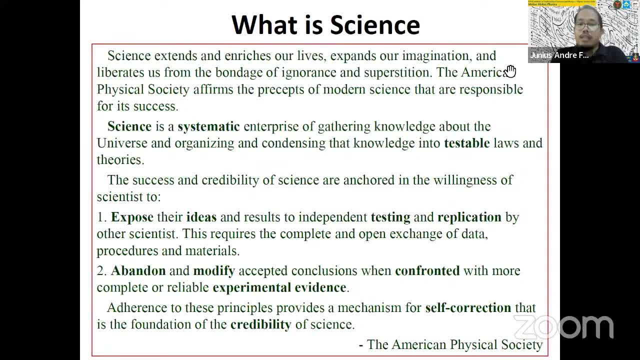 Adherence to these principles provide a mechanism for self-correction that is the foundation of the credibility of science. Of course, the teaching of science is still not a complete endeavor or finished endeavor, And this is just a little way of helping reach that goal. 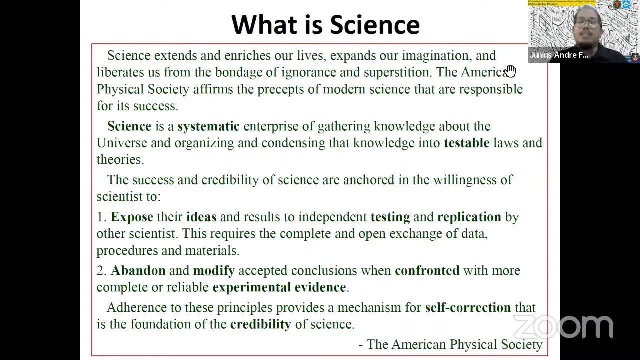 the goal of where in everybody thinks scientifically is our goal and we're not yet there. but this is our attempt And even this short conversation will not really remove- hopefully will remove- all our misconceptions, but we are humble to accept the possibility. 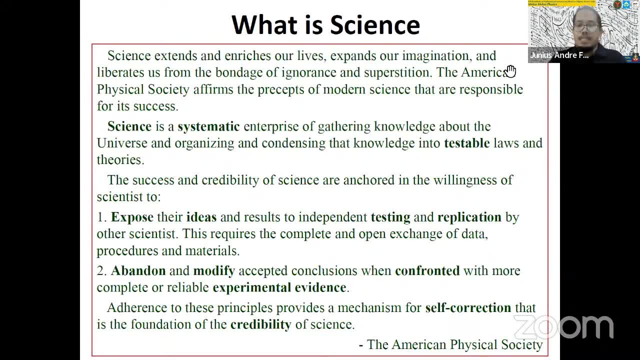 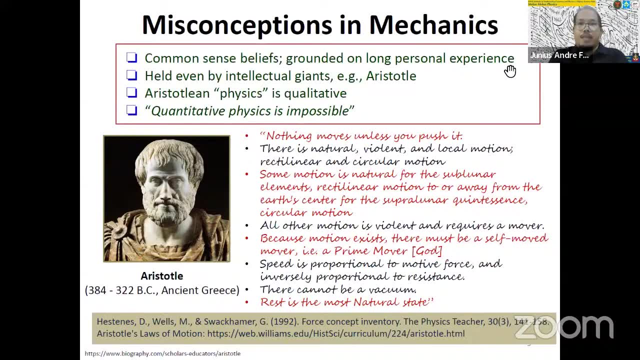 that this is just an ongoing process. okay, So now? so what are misconceptions in science? Are they real? Are they real? So let's start with the basic ones, okay. The first one is that we are a society that is based on a common sense belief. 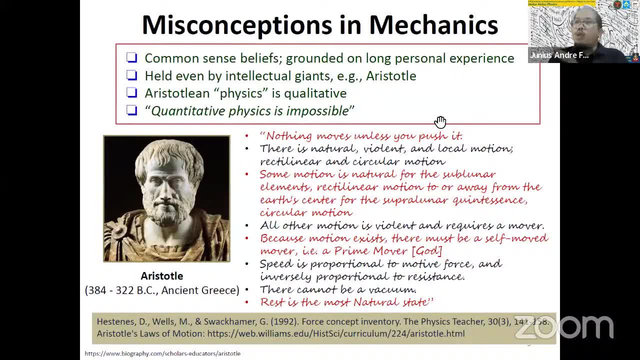 Okay. So we are very much based on a common sense belief. I mean, we have a lot of different beliefs, but we have a lot of ways of thinking about them, okay, and we have a lot of different ways of thinking about them. 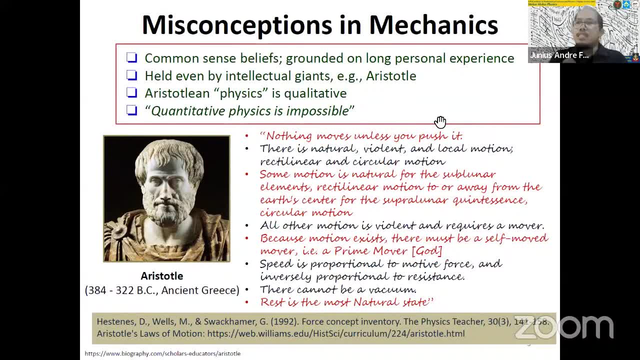 So the first one is that we are a society that is based on a common sense belief, like Aristotle and graduate students may have misconceptions. It's because you will see here that what is referred as misconceptions in physics are in fact from what? our view of the physical world, from our senses. okay, 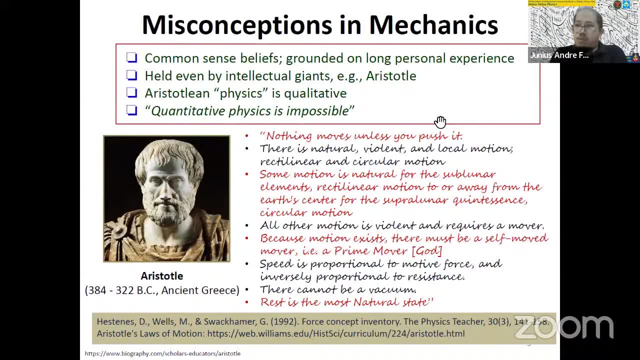 So that's why we recognize Aristotle as one of the fathers of science, because he proposed an important element in science, which is observation. So what we gain from observation, that is how we describe the physical world. okay, But we'll see later on that there are limits. 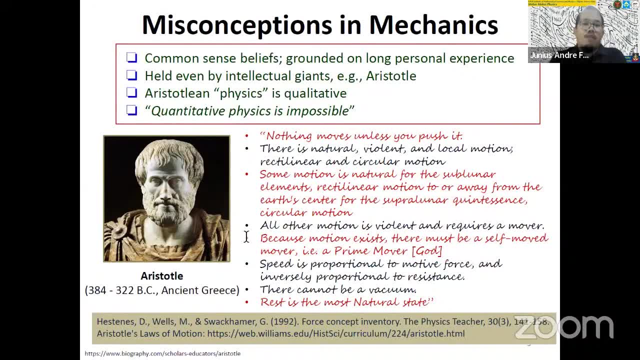 I'm not really going to go through the laws of motion of Aristotle, but these are the things that he expressed or he said about, for example: nothing moves unless you push it. okay, Sounds familiar. okay, Some motion is natural for the sublunar elements: rectilinear motion. 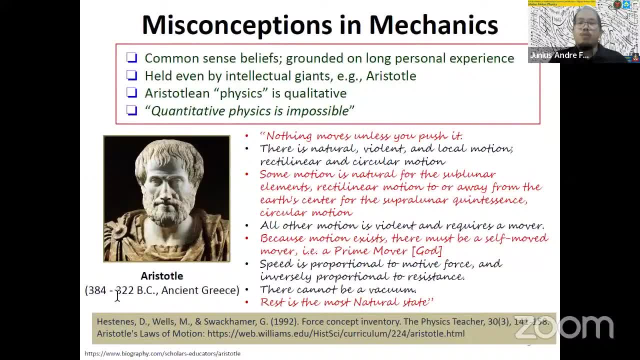 two or away from the Earth's center for the superlunar quintessence or circular motion. So since he has no mathematical law for circular motion, he accepts it as a given. okay, Then, And he believes that because motion exists, there must be self-move or mover. 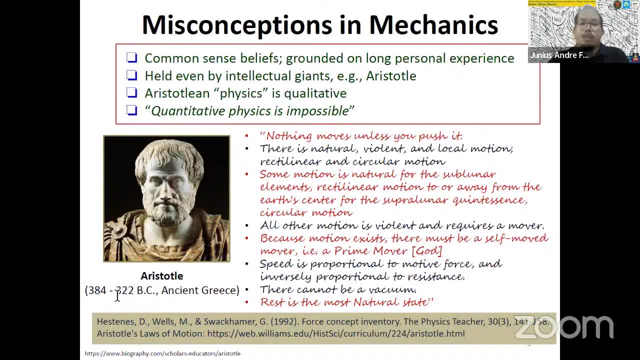 So in this case, maybe he entertains the God in the equation, in the equation itself of describing motion, And he believes that rest is the most natural state. okay, So this to us, to scientists- we know that this is limited or some would say even wrong- okay, 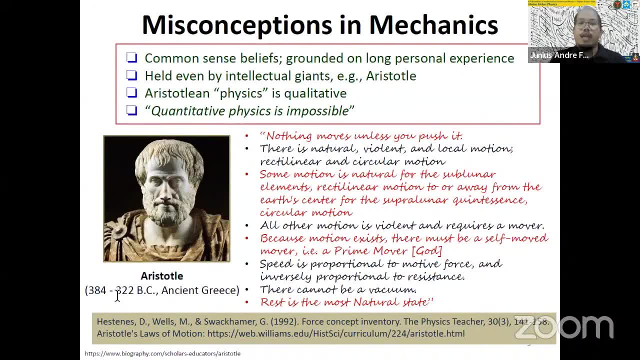 But it sounds familiar because it is what We observe. okay, As you can see, this is just an excerpt of what Aristotle believed, and it's very verbose and it's qualitative. So, in fact, Aristotle thought that quantitative physics is impossible. okay, 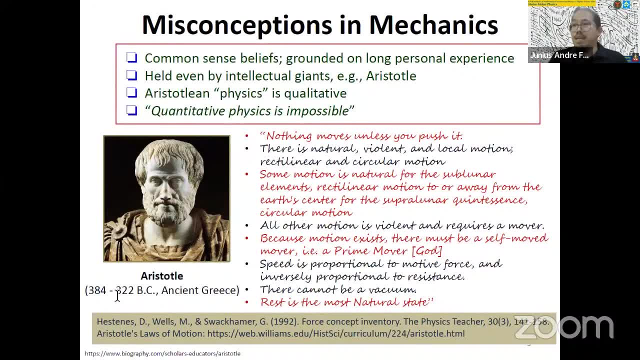 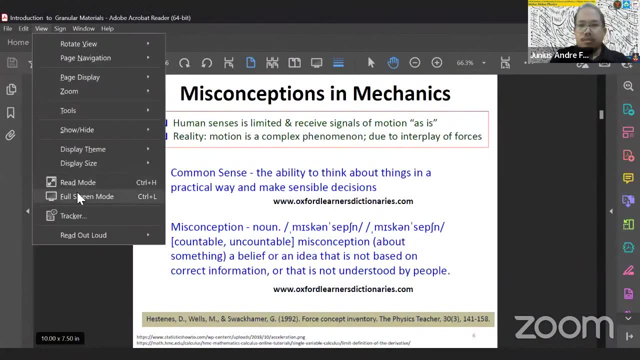 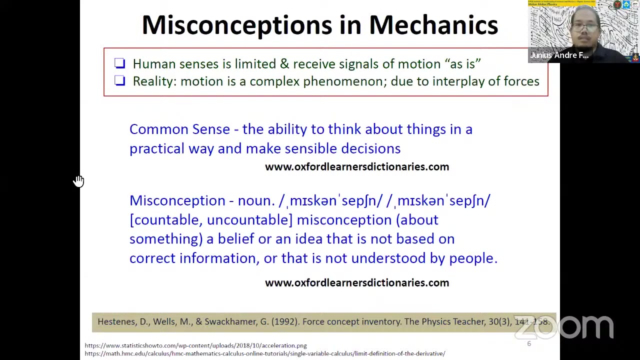 But note that his observation makes sense. We ourselves observe it. okay, Let's freeze. Okay, Okay. So what is scholars of misconception actually considered misconception? not in a derogatory sense, actually, they think of it as common sense. 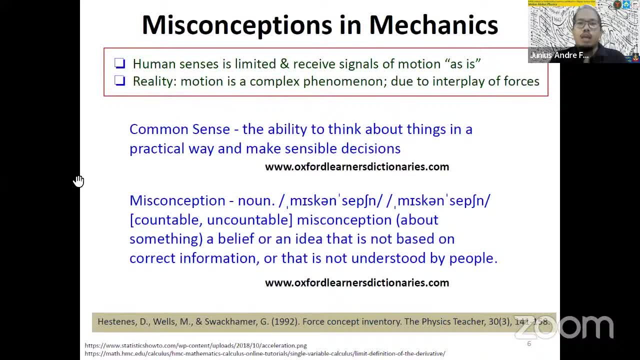 So just to review what is common sense: is the ability to think about things in a practical way and make sensible decisions, or it's a product of sense? okay, So we can do. We observe things and we do something based on that observation. 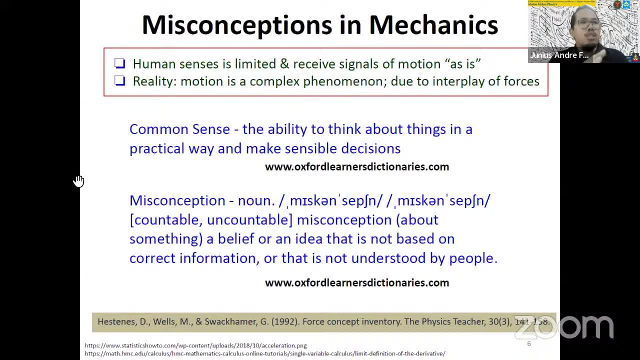 However, as we will see that if we use this common sense in describing motion, it can be limited, It can be severely limiting And, in a sense, we call this one as misconception. So misconception as defined misconception is a belief or an idea that is not based on correct information. 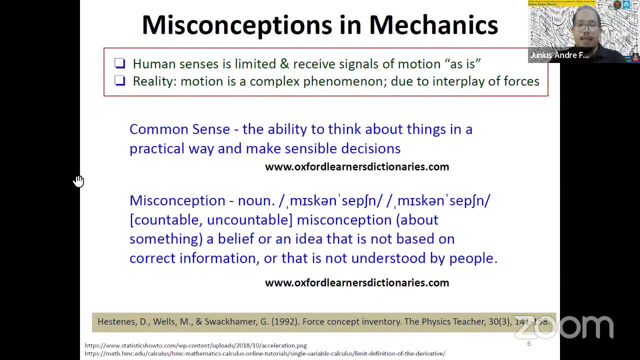 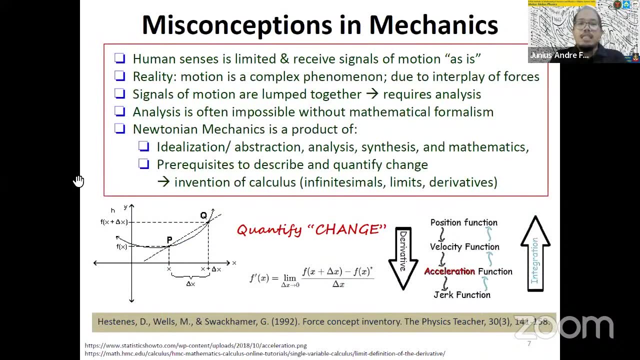 or an idea that is not understood by the people. okay, And you will see later on that this is relative to the Newtonian mechanics. okay, As we will see later. okay, As mentioned, human senses is limited and usually we receive the signal about motion, as is okay. 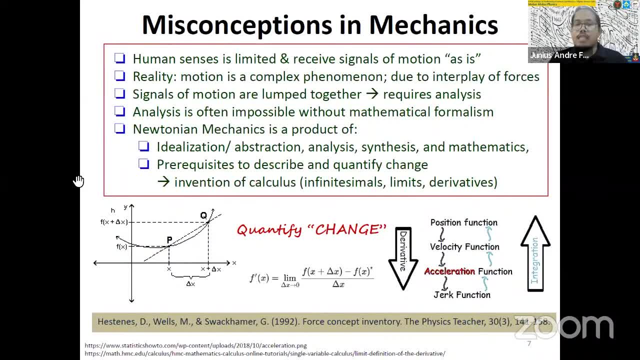 And, in reality, motion is a complex phenomenon. It's due to the interplay of forces. okay, And there is signals that we receive are lumped together such that it requires an active task. It involves action, It's an active task. 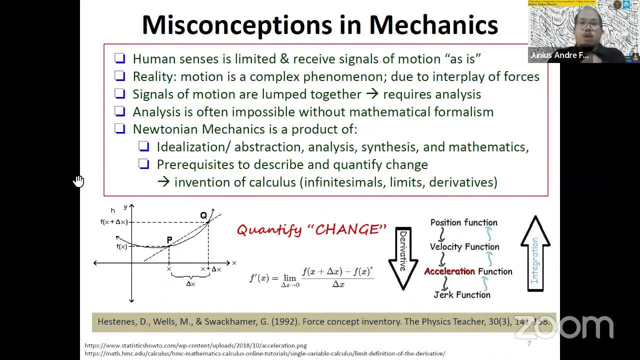 To really understand motion, you have to analyze it. okay, Analyze, in a sense, when we define analysis as taking a part or taking something part by part. okay, And it turns out that for us to be able to do this properly, 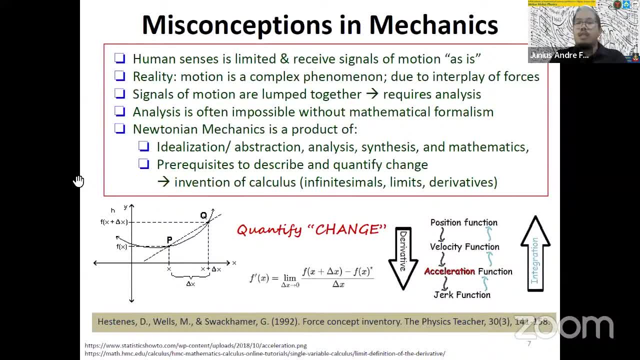 analysis often needs mathematical formalism, And it's no surprise that misconception or the Aristotelian view of the world persisted for so long, because there's an important ingredient that is missing, okay, And that is as we now know. 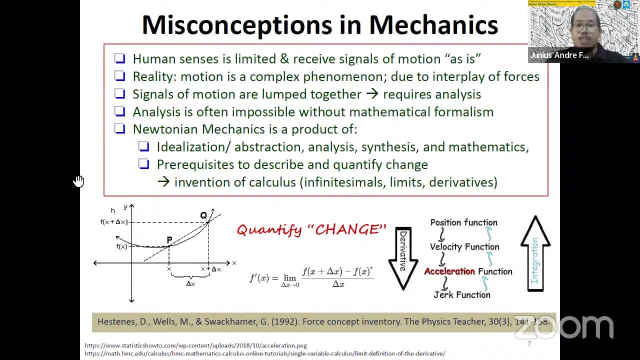 the correct way of viewing the motion is Newtonian mechanics, At least that's one We'll see later on that. actually there are other mechanics, like quantum mechanics, when you go to microscopic domain or phenomenon, But at least on the macroscopic scale. 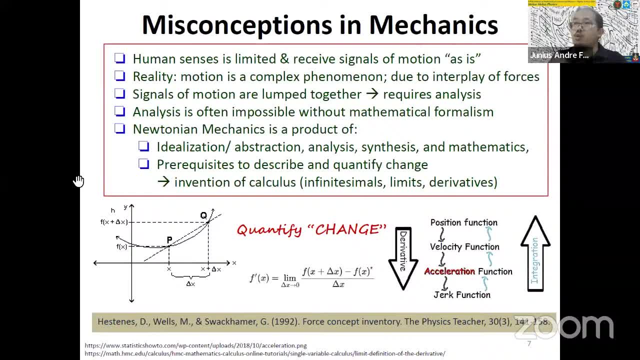 on the classical scale. Newtonian mechanics is a good way of viewing motion And it has an important ingredient: There is an abstraction. yes, Aristotel did that. He thinks, but Newtonian mechanics went deeper and I will explain that further. 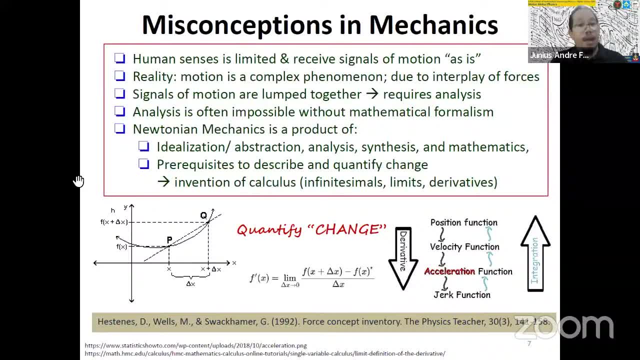 It requires analysis. So you have to identify parts, parts of of the phenomenon. So you have the object, you have the environment, So you have to take them apart, okay. So that's an active task, okay, And then you have to put it together. 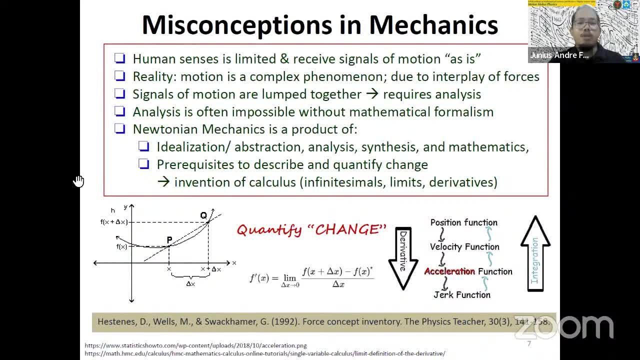 You have to relate things again, So you break apart components of motion, the elements of phenomenon, and then you conclude, you synthesize them And, most importantly, you need mathematics. okay, Mathematics is a prerequisite And, more specifically, the more efficient way of looking at motion. 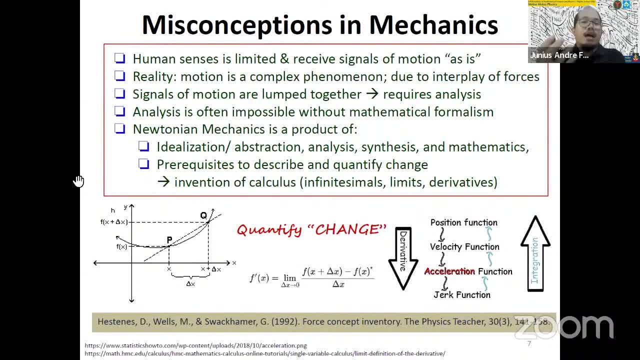 needs the invention of calculus. It needs the concept of things like infinitesimal limits and derivatives, Because the key element option is change And the best way to describe change is mathematically, And you need mathematics too for that, And the mathematics for that is calculus. okay, 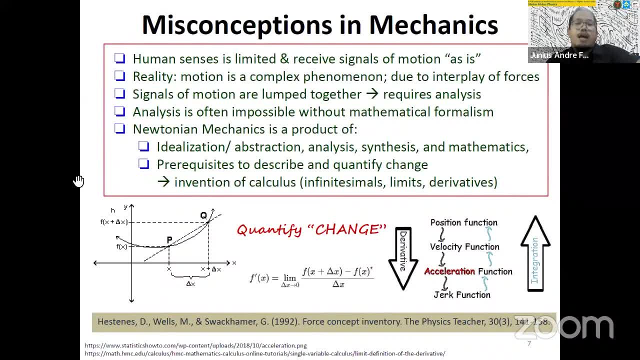 So you have these concepts of change, okay, And then limits: These things- limits or infinitesimal- are actually abstract concepts. They are not tangible in a sense that you can count them. In fact, yeah, in an ordinary way, you cannot really, you cannot touch. 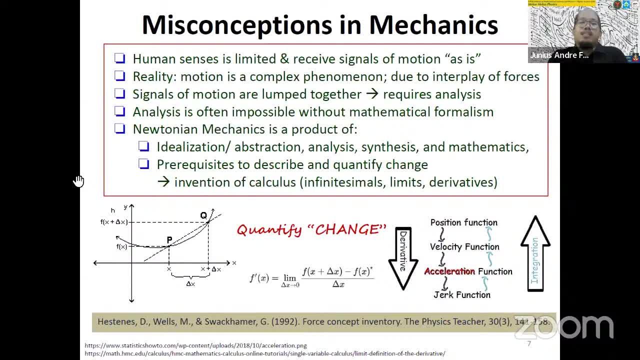 It's not intuitive, the concept of limits and infinitesimal. In fact, you will see that in even in college students- one of the brightest students in science- high schools, in UP, it's difficult to teach calculus because it's not a natural. 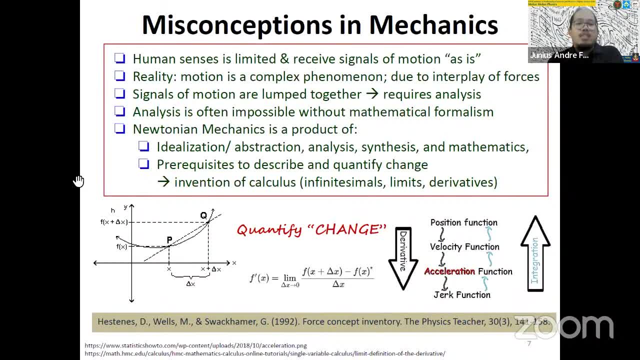 it's not a natural reaction or natural view of things- the concept of limits and infinitesimal. So Aristotle does not have that, while Newton invented that along with Leibniz. okay, And we know that mathematics is the most efficient language, okay. 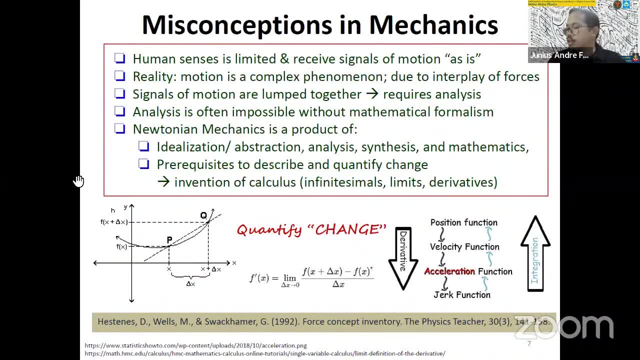 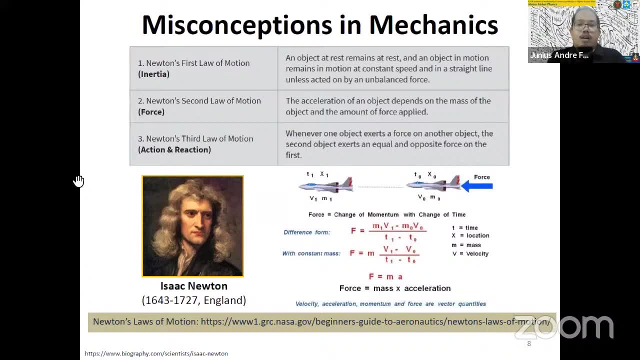 In the language. it's a language, so this is the core element of Newton's laws. okay, So, as you can see here, you're familiar with this. Newton's laws are three sets of equations or descriptions. These are descriptions that are related to each other. 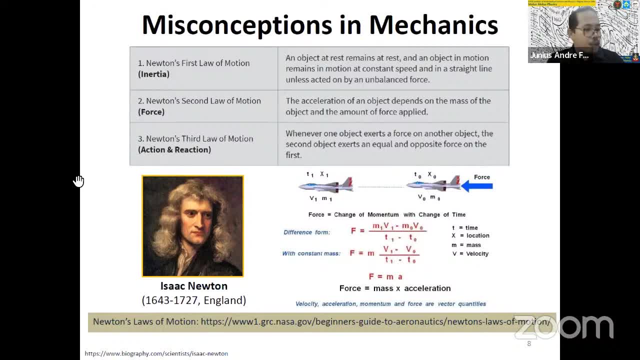 It's important to note that these three laws should be considered together, okay, Although we simply we listed them and we numbered them just for organization purposes. But basically, these three laws define what we now call as force, okay, And its relation to the quantity of motion, which is momentum. 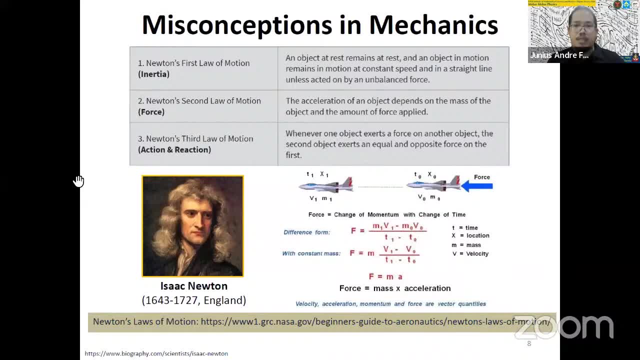 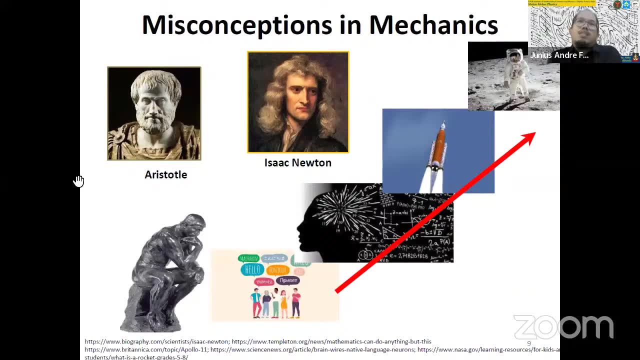 And for this to be practically useful, it needs mathematics. okay, So you will ask: is Aristotle wrong? In a simplistic way, it's a very oversimplified way of asking the question: is Aristotle wrong? okay, In a sense no, because he is simply describing what he observes. okay, 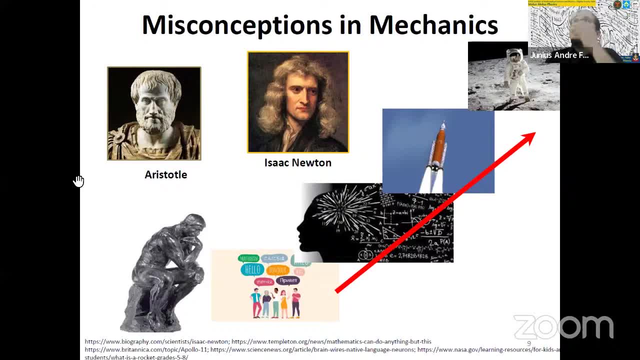 So, however, okay, my view of knowledge is because we need, when we knowledge has to, has to prioritize, has to compare or discriminate, okay, And some knowledge are more efficient or, in a way, superior than others- kind of knowledge. 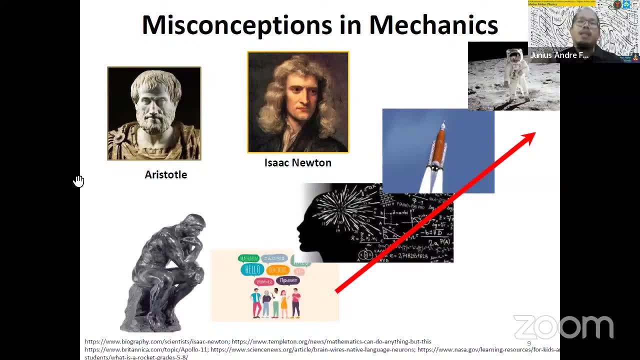 What do you mean by better or when we discriminate? knowledge I can offer this one: Aristotle is a product of well-thought, deep thinking. He taught us to observe And it has been successful in science And it remains the core activity or task in doing science: observation. 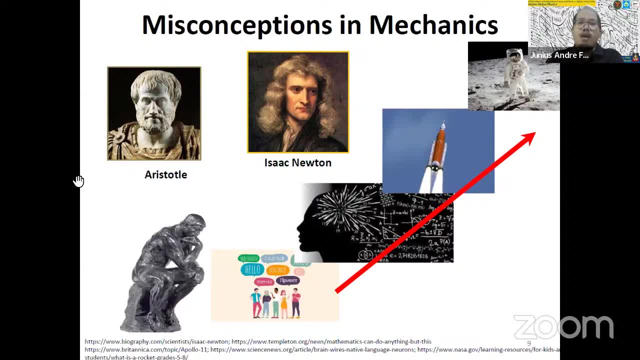 We use our senses. However, it's not enough because technologically, we see that we need technology to see further or to see smaller, or to see we need to extend our senses. So that's one. The other is we need to extend our senses. 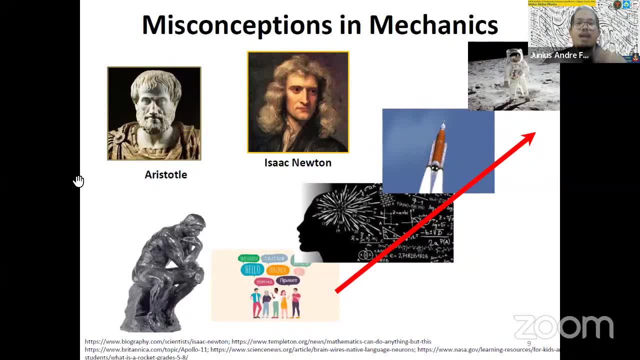 So that's one. The other is we need to extend our senses, So that's one. We need to extend our language. The words that we use are not enough, So we invented or we discovered. I will not go to that debate, but basically we need. 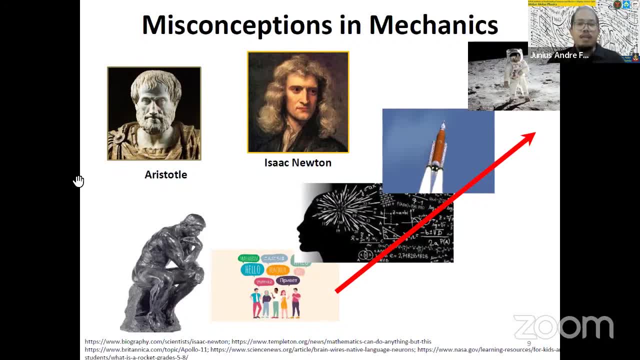 mathematics to extend our language, okay, And it is through mathematics that we're able to find, to learn more. I think the term there is generative. The knowledge that uses mathematics, okay, and technology, advanced technology, are more generative. it can lead us to further knowledge. in contrast with aristotle, it's, it's a it's. 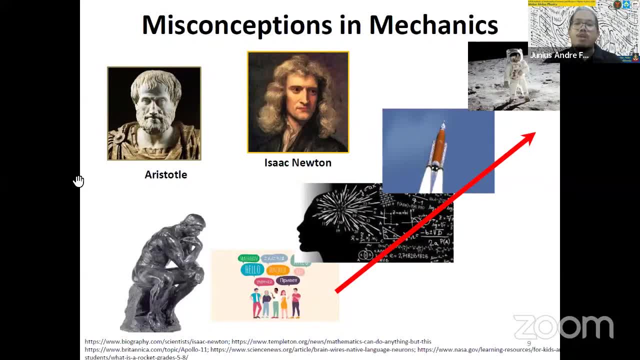 knowledge. however, it is limited, it does not give. allow us to go further. simply put, you cannot use, okay, you need newtonian mechanics to do that, okay, so that's, i think, that's, i think, that's, uh, uh, one way to to uh settle the debate, at least, uh, uh, for now, why newtonian mechanics is a, is a. 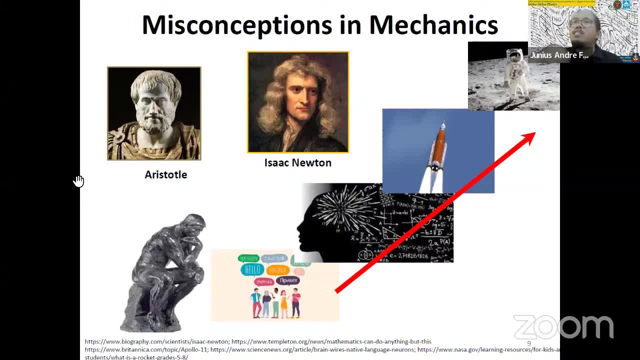 better alternative to aristotle- in fact, it's the only option relative to aristotle- uh, to view motion, okay, so with, again, with aristotelian thinking cannot send man to the moon, okay, so that's how, how i would end this discussion here, okay, and therefore, if we do not, uh, remove misconceptions aside, just we will. 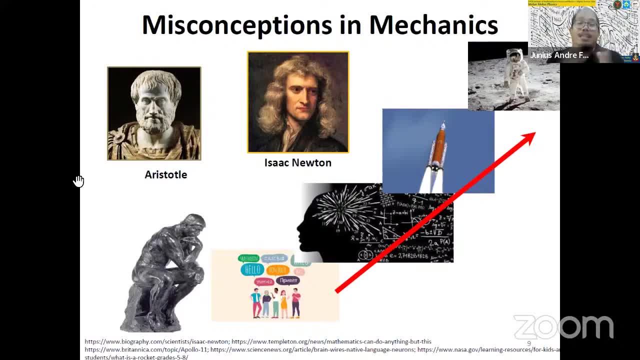 fail the exam. that's a very minor. the other is in the physics. okay, that's a very minor consideration, but the more important reason is that because aristotelian thinking, our common sense thinking, is limited, it will not take us far, okay, in contrast with a newtonian physics, okay. so that's. 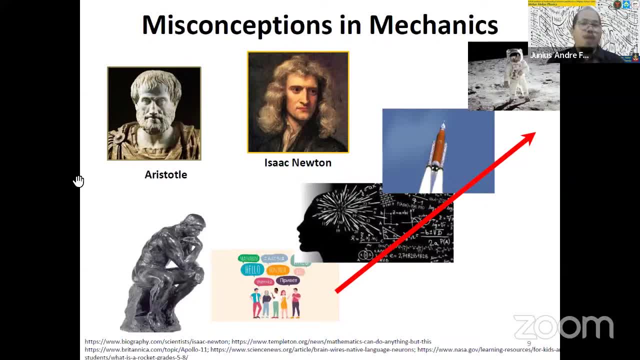 really important that we, uh, we resolve, we identify and resolve misconception. okay, so, uh, to recap the this first question: what are misconceptions in physics? basically, these are common sense, uh, observation, uh, good observation, but they are limited and they are, they do not, they they do not satisfy or they are not as good as newtonia newton's view of motion. so all of this. will likely, Mateo, take you through. haven't seen much of sport, though, in your heli past, or understand you only 양 show or race car. you don't kick a man. but i really enjoy looking at the dish right then, um, because you see a good. expression there. but though there's very much of a need for an framed game, not everything is most important to you, but total fire at 10, 90 percent of the word movement will seem rather bake and a good UK training device. yeah, i can see more like this and that's because even, but to me and some of my newtonian scientists are 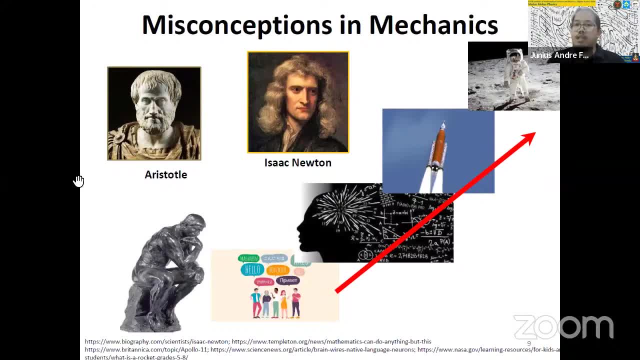 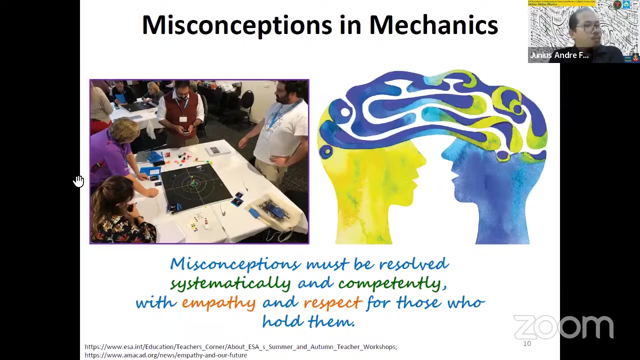 So that is how we define misconception here. So misconception wrong relative to Newtonian And Newtonian view of motion is in this metric is very superior is the correct answer to describe motion. It is important in this discussion. what I wish to also highlight is that misconceptions must be resolved systematically and competently, with empathy and respect for those who hold them. 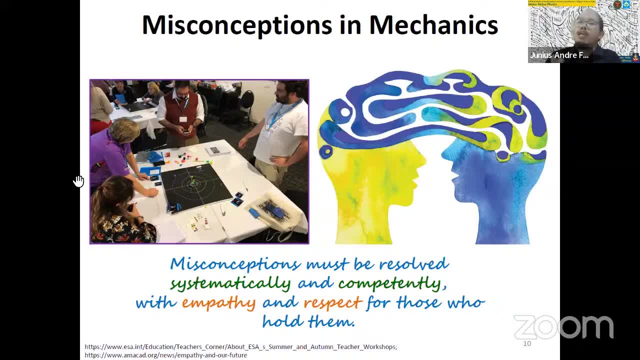 Because usually when we say misconception, yes, it's wrong, But sometimes it's as if it's a fault of a person. It's something he did something wrong, or there's something missing, lacking, And that person there's, that sometimes there's a sense like that. 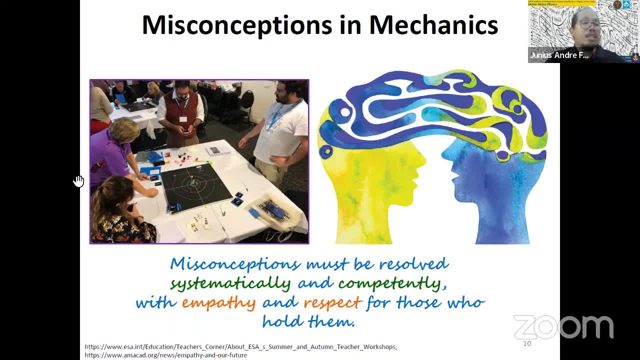 But actually it should not be the case, because reminding ourselves that, if intellectual giants like Aristotle have them, if graduate students or even us teachers sometimes still have misconception, how much more a person who has not studied physics or is just starting to learn physics? So there must be empathy and respect, because it is rooted on understanding. 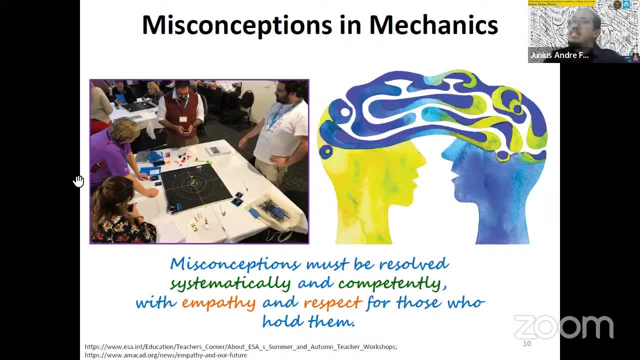 What is misconception? So it's not really out of laziness or you know, it's because the misconception is actually a natural reaction to our surrounding. So it's not simply just wrong, Okay, But it's, And we have to understand that the replacement is not, is not, did not just spontaneously arise. 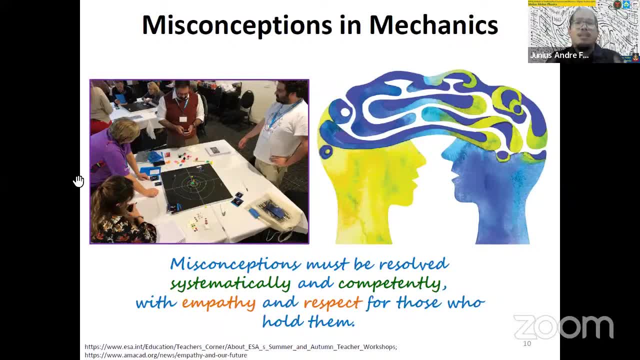 It requires an active, a proactive process. It's an active task to to think that way. We don't naturally think in a Newtonian way, So that's one. We do not think like Newton in the first reaction. We usually start from, from, from Aristotelian. 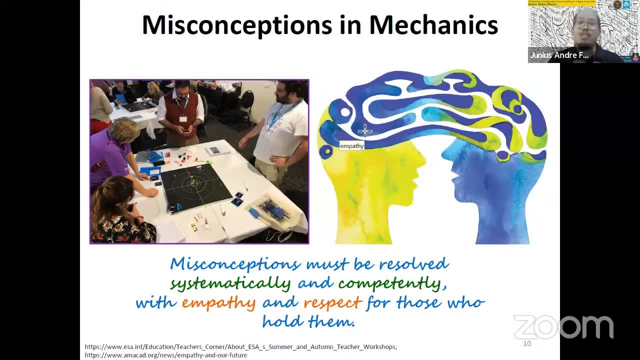 Okay. So, as they say, all of us have, We have misconceptions at the beginning. Okay, Because we use our. our first sensor for our surrounding is our senses. Okay, Our common sense. So that's that's why we have this misconception. 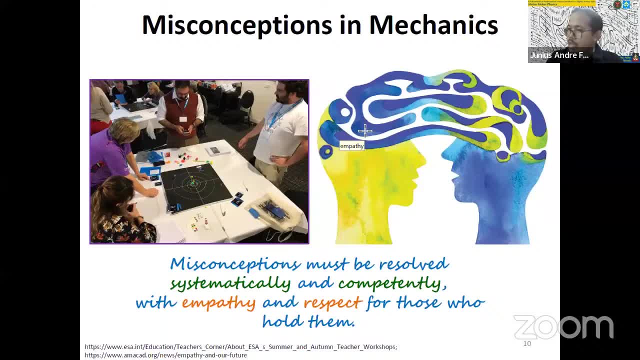 Okay. So hopefully after this, this lecture or this talk, the conversation, we have a more nuanced view of of misconception. But let me let me make myself clear. The correct way Of looking at motion is Newtonian. So maybe you'll say: ah, relative lang yan, and there's a sympathy for new Aristotelian. 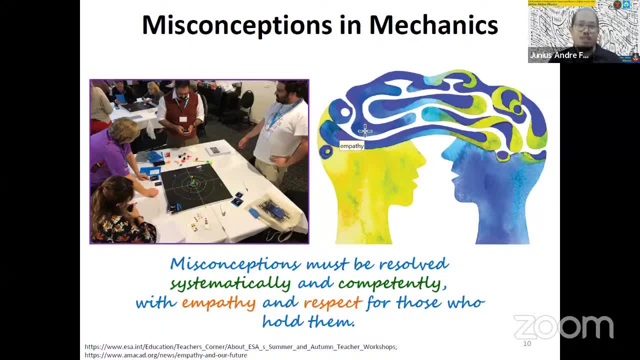 So, okay, lang, No, we really have to resolve the misconception. Okay, But we have to do it in a, in a, with goodwill And because we know what's what's our goal. We want to send man to the moon. 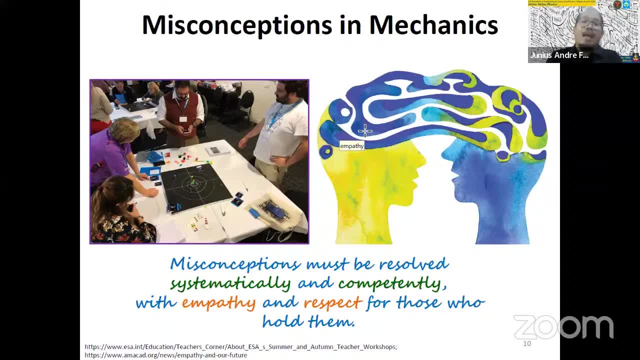 We want to send our cars to function properly, And Aristotelian physics will not, will not work If, if we, if, If it, if that's our choice, Okay, So it has to be Newtonian, Okay? Next, 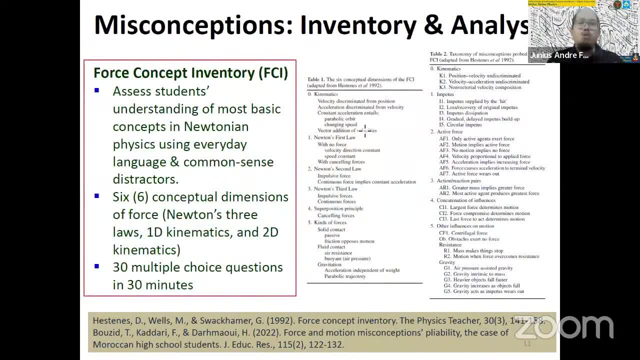 So if there's misconception, okay, How do we measure and analyze it? Okay, Ah, there's a long study since, I think ever since, uh, people had been studying or teaching physics. Okay, We have to contend with misconception, Okay. 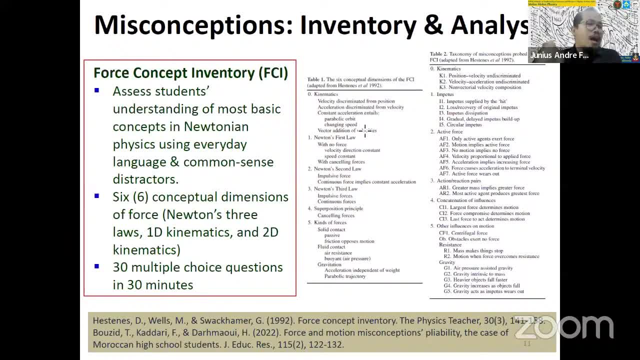 So I will not go through the long History of uh physics education, research or PR. Okay, I will just uh uh highlight here One of the uh successful- I mean very uh successful- efforts in addressing misconception. 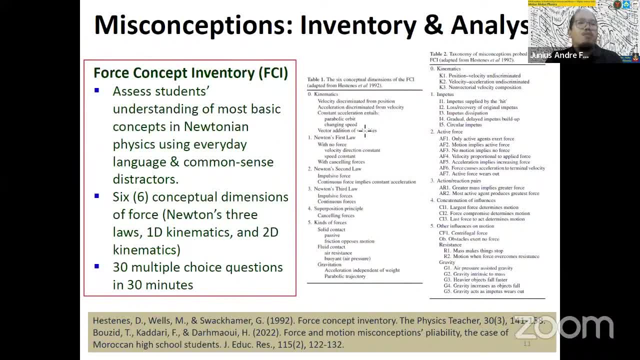 And this is the uh. one tool that was the product of this effort is what we call the force concept inventory. Okay, Actually, what I did, the survey that I gave you, is from uh, is from this one, But uh, because there's a need to maintain the integrity of that uh, of that quiz. 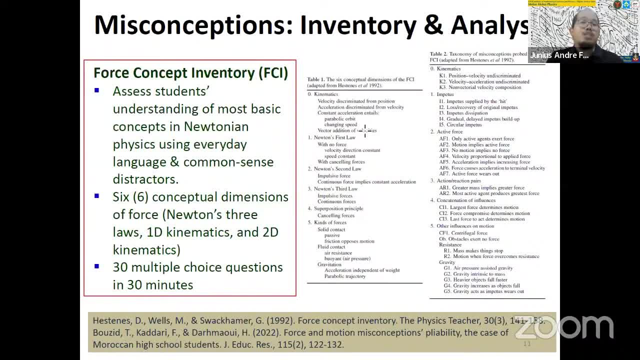 Okay, Uh, we, we have to change the question because, of course, if you will use this force, concept inventory- and I'm I have uh, uh, announced it to the whole world- uh in the, uh, the, the purpose will be defeated. 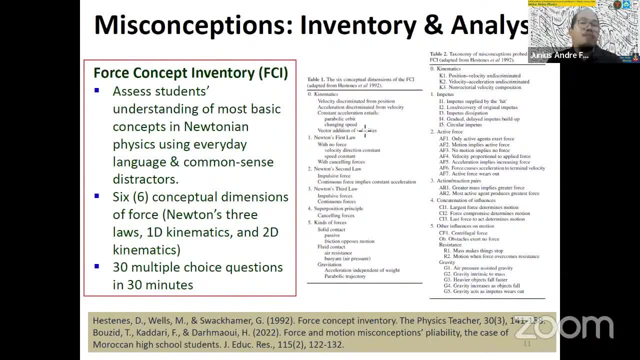 Okay, So actually what I gave you is an excerpt and a modified version of the force concept inventory. So now the force concept inventory is the Uh, uh, one of the just one of the many inventories. Okay, So it's uh, it's developed. it was developed by the team of uh Hester nest. 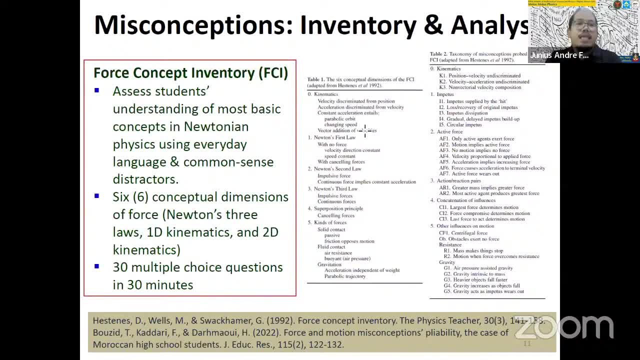 Okay, Um and uh. basically, it assess students understanding of the most basic concepts in Newtonian physics using as much as possible, uh, everyday language and and common sense disruptor. I will show you the parts of the cut and the basically they started. 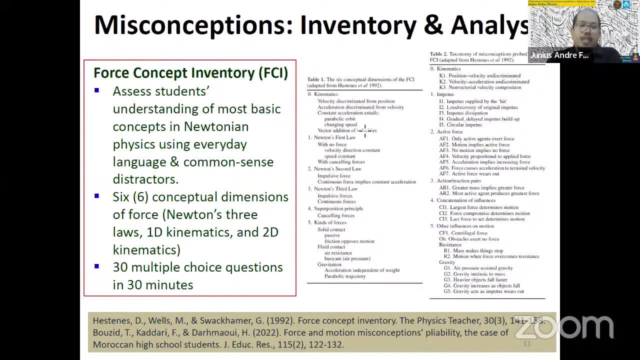 They identified six conceptual dimensions, of course, basically Newton's three laws, uh kinematics and 2d kinematics, And it's a 30 multiple choice question that must be answered in 30 minutes. So it's a. it's a standardized test. 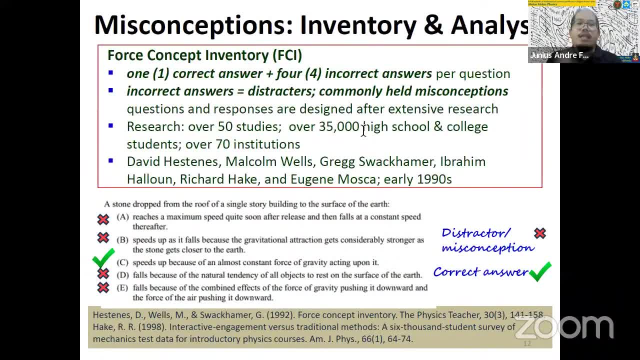 Okay, Standardized test. Okay, It's a. it has one for each question. It has one correct answer and four incorrect answers. Okay, What do you mean by incorrect answer? This is what is. It's not a track course or commonly held misguided uh questions. then, to convert it into a multiple choice question, they study the responses of the students that are wrong and they identify the common wrong responses. 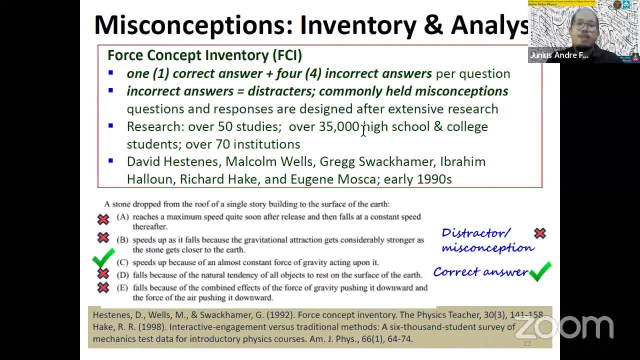 And that is what they use as the destructors. Okay, So this is uh one of the uh popular, most uh one of the popular Uh inventories, because- and well-studied uh inventories, it uh, at least it was a subject of over 50 studies involving more than 35,000 students in over 70 institutions, and counting. 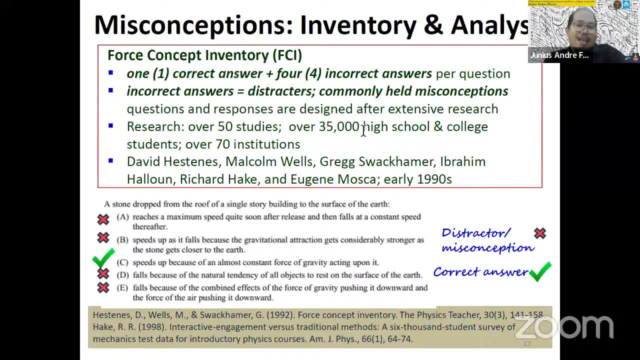 Okay, Actually, if you're a teacher, uh, when I I was able to have access to this and to the answer keys by having myself directed, and I have to ask permission, uh, to be able to to see the answer key of this. 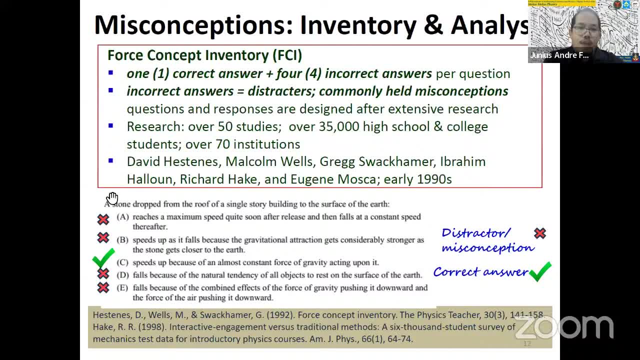 Okay, Um, just to show you an example. So you have your question and then you have only one correct answer, Okay, And then the four. the rest are wrong answers. And uh, what is usually studied is uh, is, uh, what are the most among the destructors? 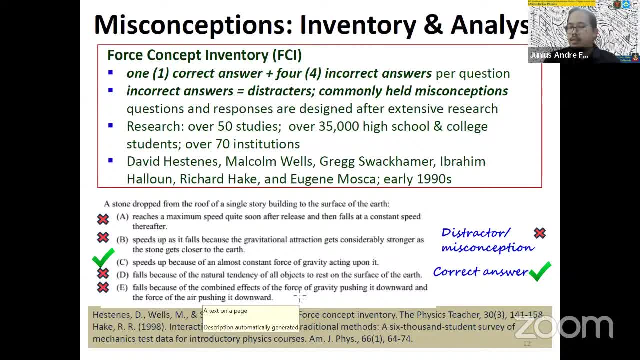 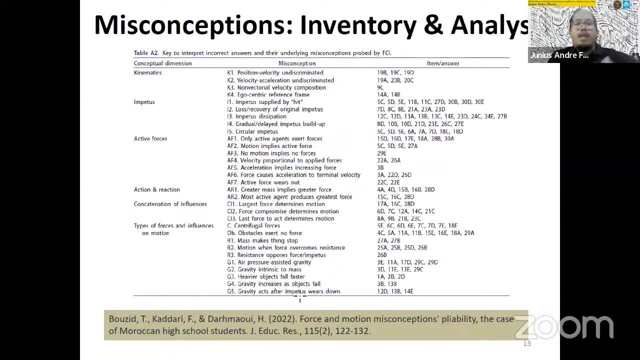 What's the common one, And this is what we will discuss in a short while. Okay, So Uh, this is a conceptual several dimensions where they identify what are the forces, Concepts that are the elements of Newton's laws of motion. 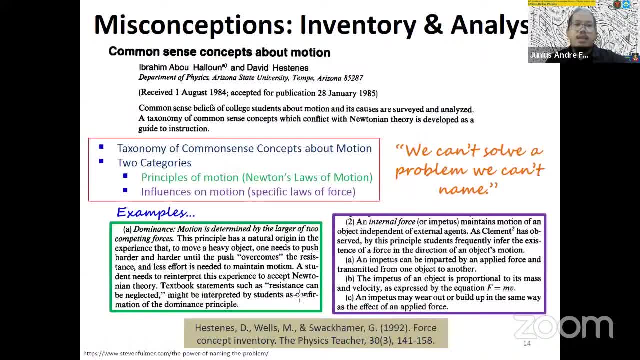 And then the types of forces. Now, of course, we need to analyze the result of this inventory, And many researchers have studied the misconceptions and they developed a taxonomy, Because you cannot solve a problem if you cannot name it. So develop a taxonomy. 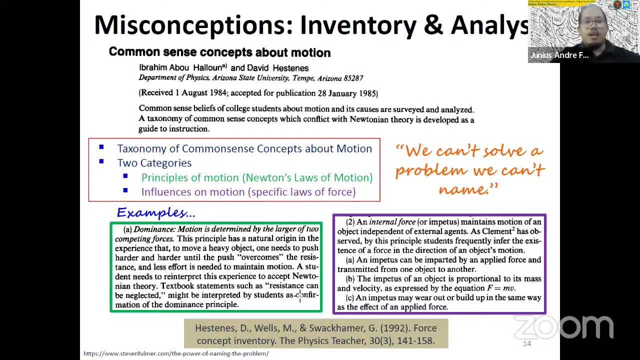 It consists of two categories: One pertains to the principles of motion And the other identifies influences of motion, And this is important later on when we discuss how to address one misconception in Newtonian mechanics. So just an example, You don't need to read this one. For example, 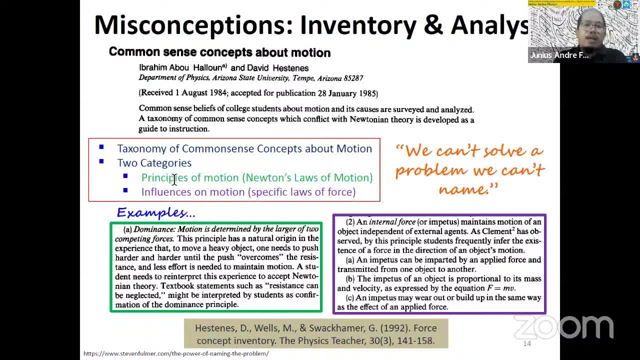 this misconception is under the category for principles of motion. So the misconception related to the Newton's laws of motion- The violet one, the purple one in the purple box- is a misconception about the kinds of forces. So these are two different things. 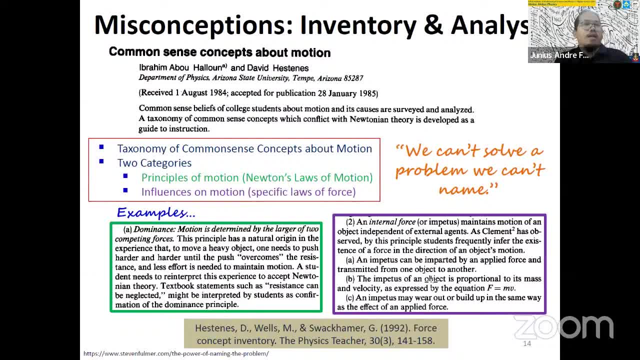 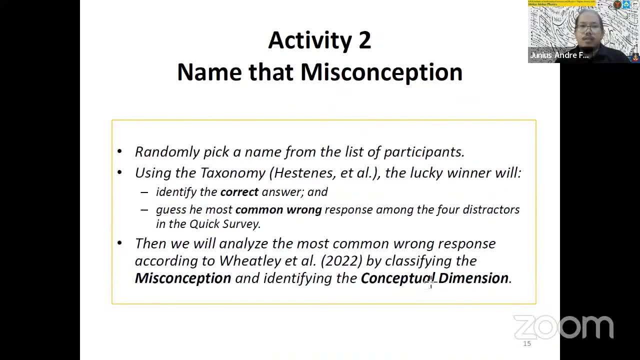 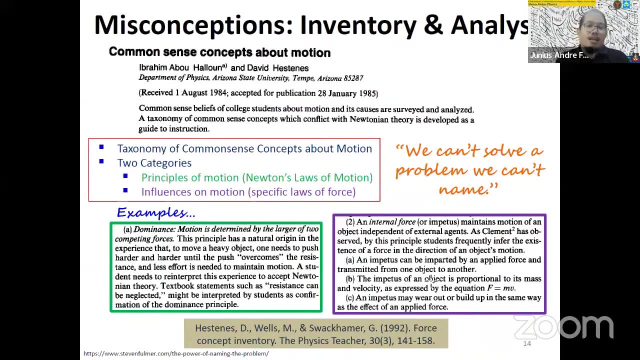 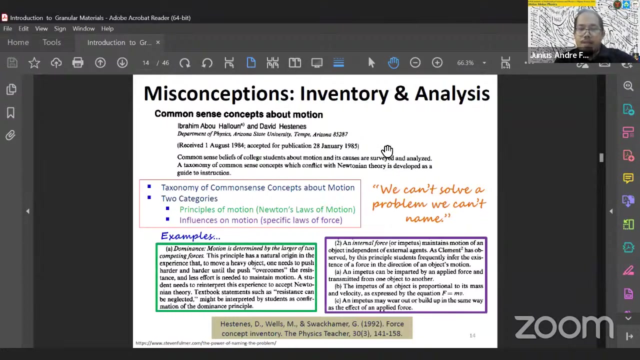 So they have this one, So they do item analysis. Basically, this is a product of item analysis. So just to up our energy a bit, we now have a next misconception, Next activity, rather talking about misconception. So, by the way, 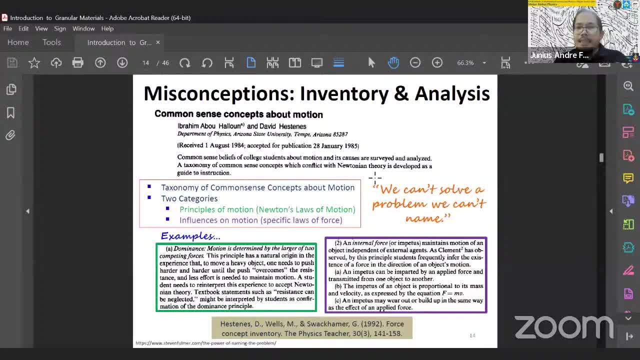 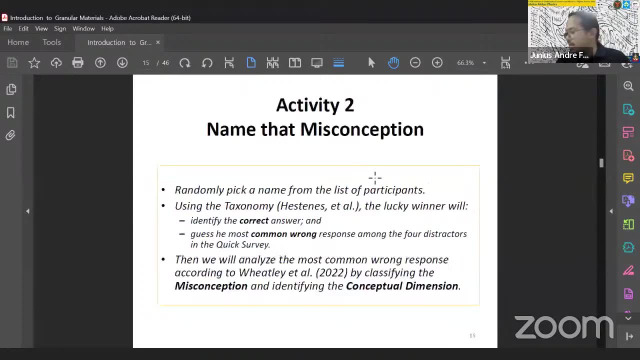 we'll pause a bit. Ma'am Ella, Ma'am Ella. Yes, sir, Can you help me identify volunteers or lucky winners? Five people who will help. This is the next activity. Okay, So Ma'am Ella will randomly pick a name from the list of participants. 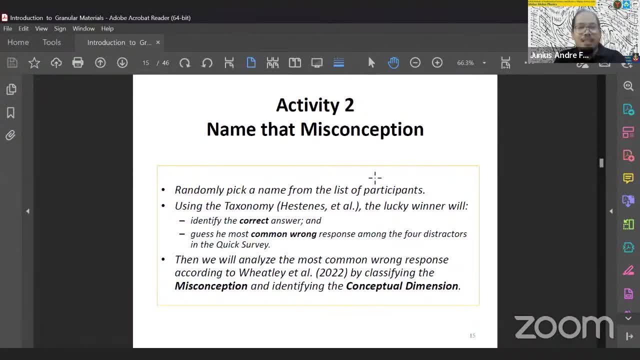 And I hope, a good sports and participate. Sir, should they be students Or may there be instructors? So what we're going to do, we're just going to ask you to okay. So then, using the taxonomy, okay, the lucky winner. 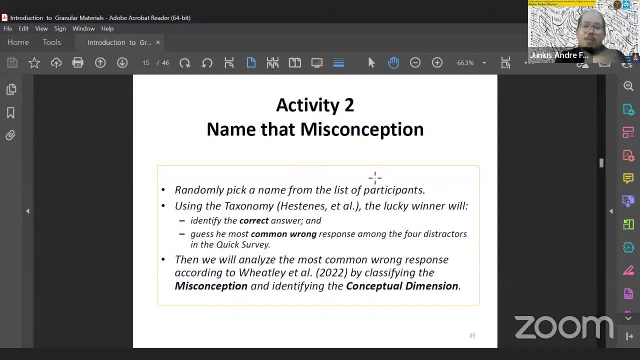 actually you don't have the list of taxonomy, but basically I'll just ask you to identify the correct answer and then, among the wrong answers, guess which of which one is the most popular wrong answer. Okay, So the correct the answer. 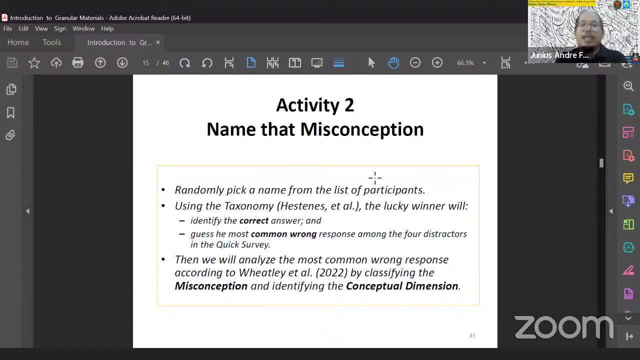 will be revealed in the work by Wheatley. Okay, So using the taxonomy, the lucky winner will identify the correct answer and identify, I guess, the most common response among the four disruptors. Then we will analyze the common wrong response according to Wheatley. So I have. 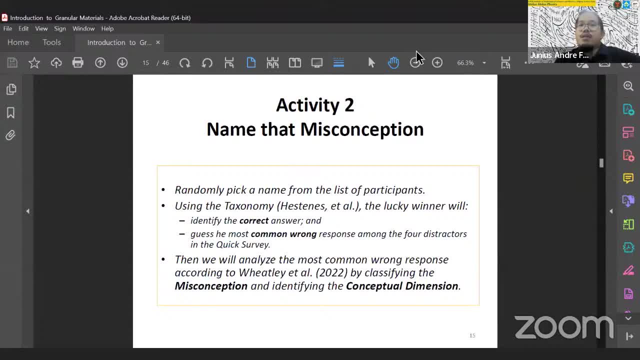 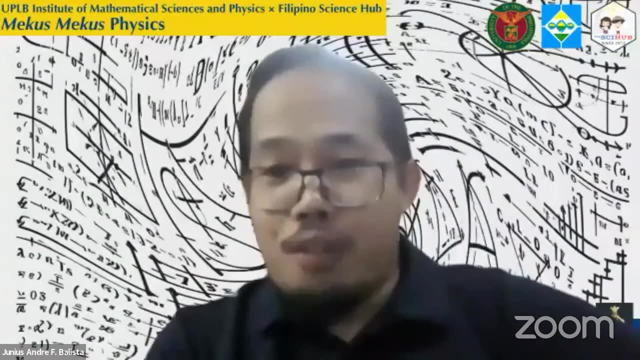 I will flash the answer also. I will stop share a few moments. Ma'am Ellen, you're already identifying, right? Yes, sir, Okay, They're chatting. Okay. Okay, Just a moment, Stop share. I'll look at our survey first. 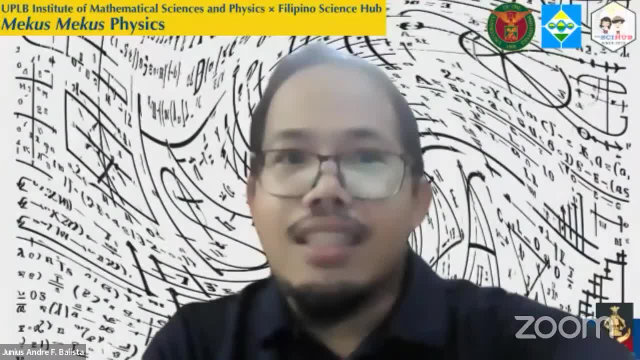 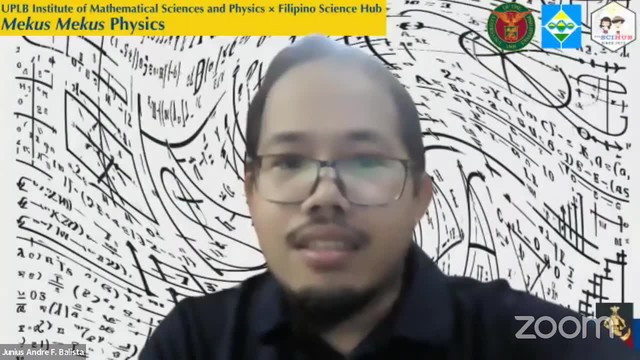 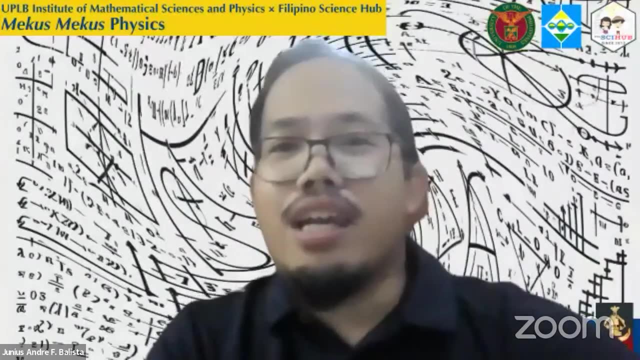 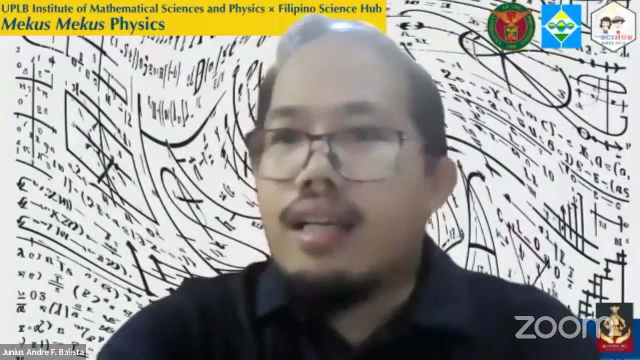 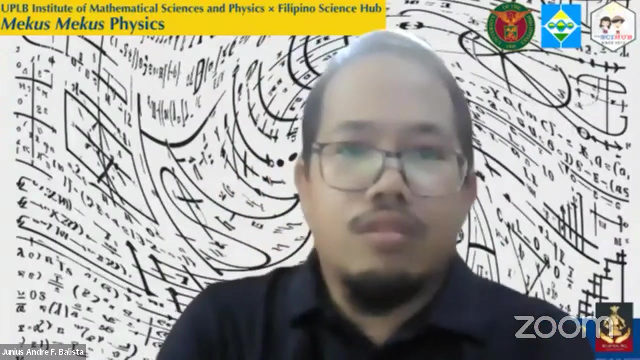 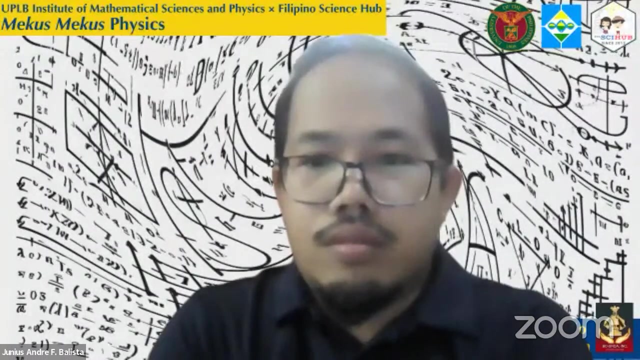 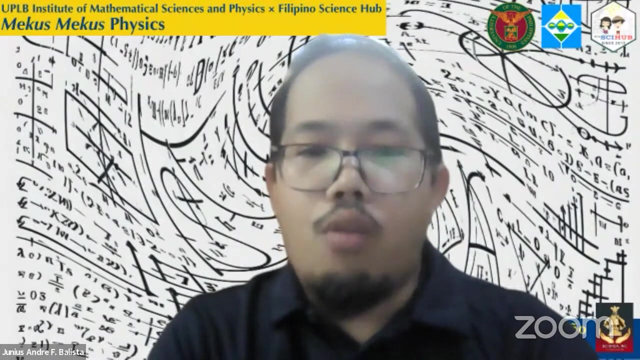 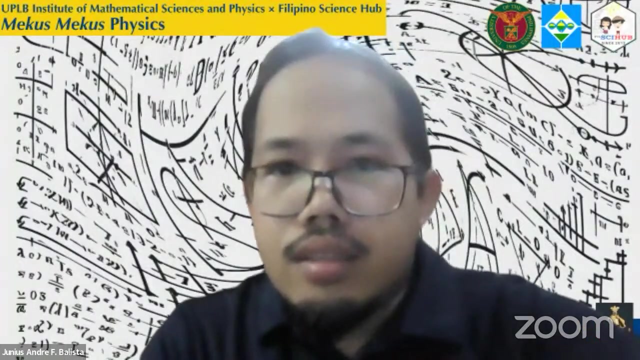 If our survey is okay, Okay, Okay, I will flash, I will share this, the result of our survey after our activity. So yeah, 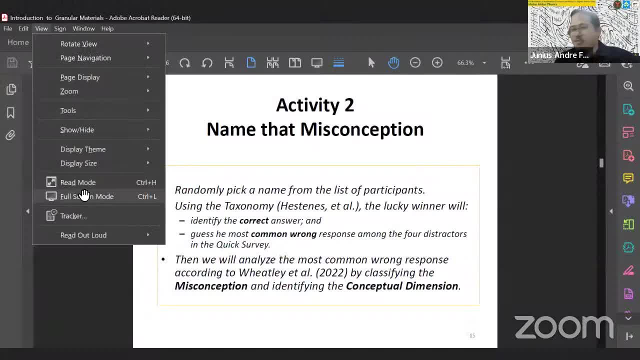 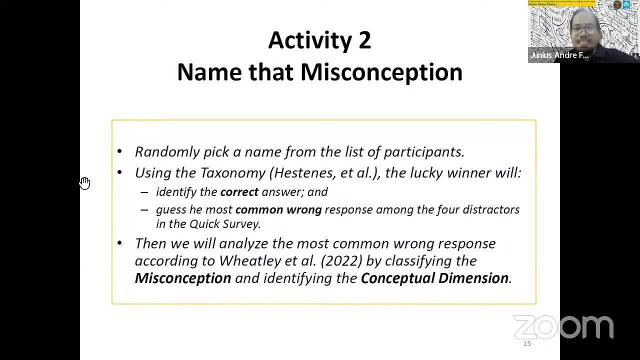 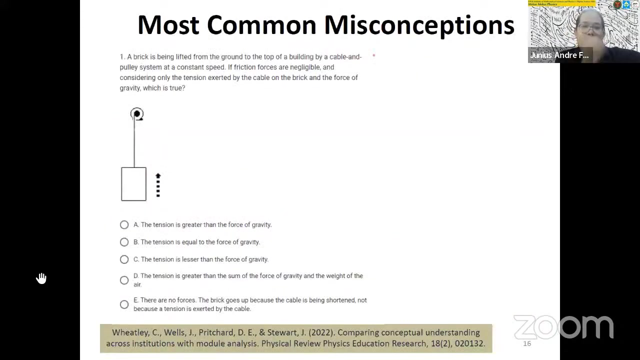 Ma'am Ellen, who is the first lucky winner, The lucky winner of the list, um, um, can we, can we hear kristin kate, eliorin, kirsten? hello, miss eliorin, miss kate. um, okay, so a bridge is being lifted from the ground to the top of a building by a cable and pulley system at 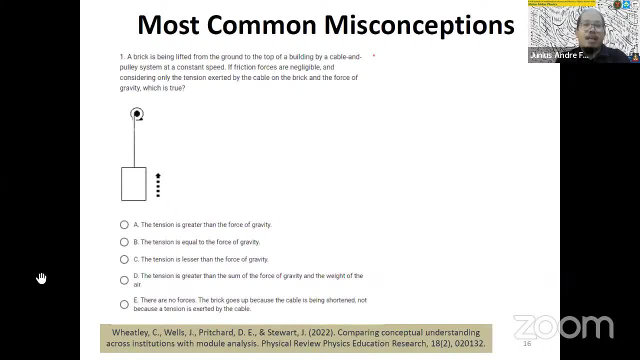 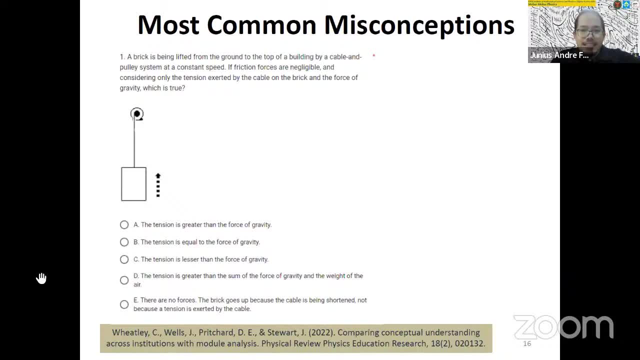 um, um, um, letter c c. okay, letter c. so the correct answer is a. a bcd is wrong. but what he usually thinks is that the wrong answer is letter c. is that right again? yes, sir, okay, thank you, so let's see what the answer is. okay, thank you. so let's see what the answer is. 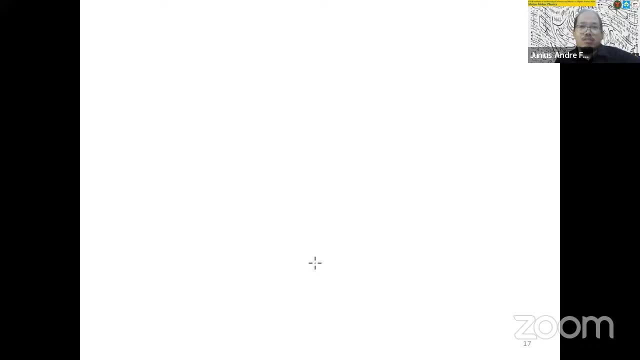 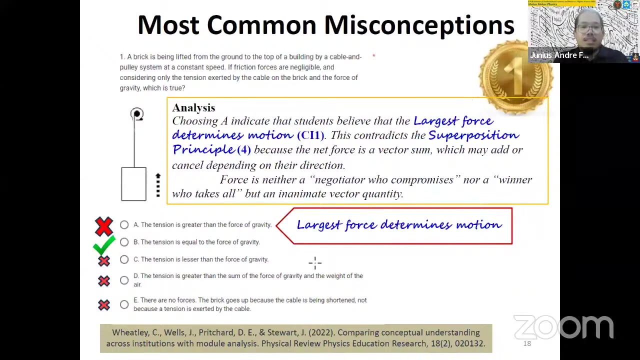 okay, thank you. so let's see what the answer is. um, according to this, to the study of whitley. okay, so ito. so yes, the correct answer is equal po, yung tension and force of gravity, zero. okay, so, uh, okay, so, uh, so no change. 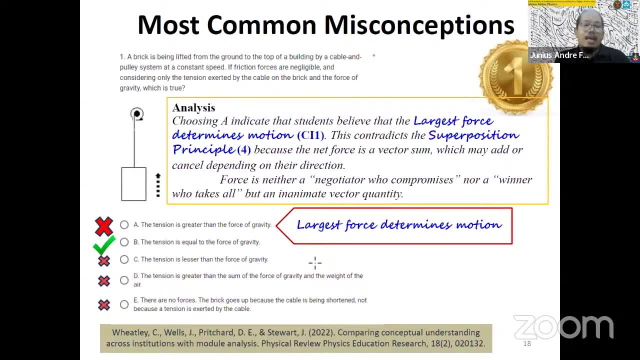 so okay, however, you're in good company. so correct answer is b. okay, however, you're in good company. company Kasi marami din yung punupili Tama ba John Yung pinili mo ay A Yes po sir. 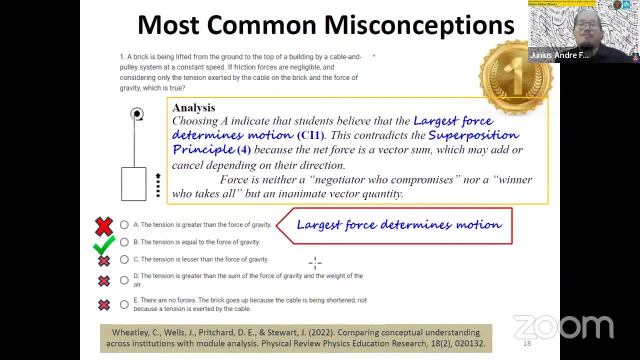 Okay, so you're in good company. Not good kasi misconception. eh, Marami nag-iisip. So choosing A indicate that the students, like John, believe that the largest force determines motion. Okay, This contradicts the superposition. 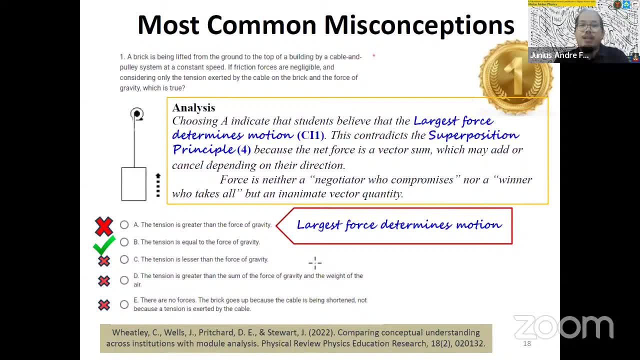 principle, because the net force is a vector sum which may add or cancel depending on their direction. So nakaroot ito sa pagtingin na yung forces is negotiating, Tapos yung kung sino yung medyo malakas. 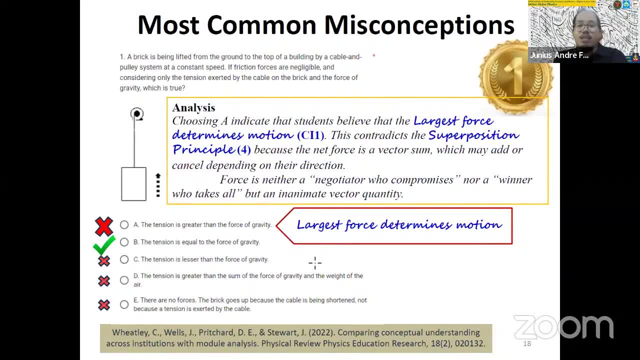 siya na lang yung susundin. Hindi po ganon, Because force is the net, force is a vector sum. Okay, So the answer is zero. yung force kasi Pareho Kaya walang change in velocity, Walang change in. 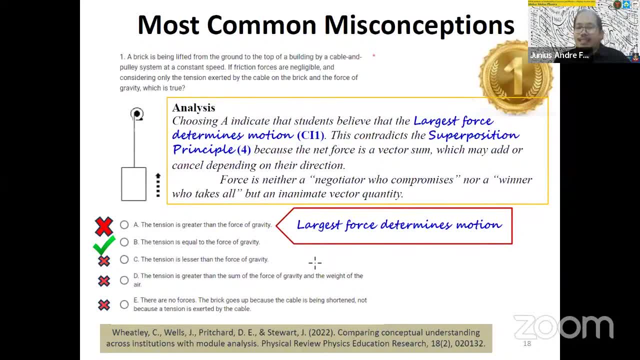 momentum. Okay, Mamela. thank you, John. Okay, Next, Mamela sino ang ating lucky volunteer Alin Lea Yatko. Hello Alin, Good morning. Good morning, Alin, Alin. 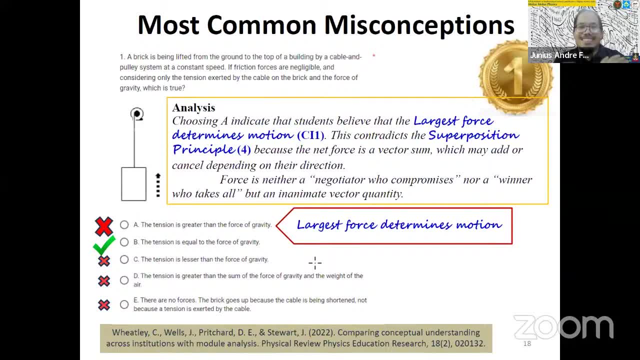 Adjoining. Ah, nawala siya, Hi sir. Maybe sir pwede muna natin tawagin si Christian Villareal, Christian. Christian. good morning, Hello Christian, Good time, Okay lang yan. 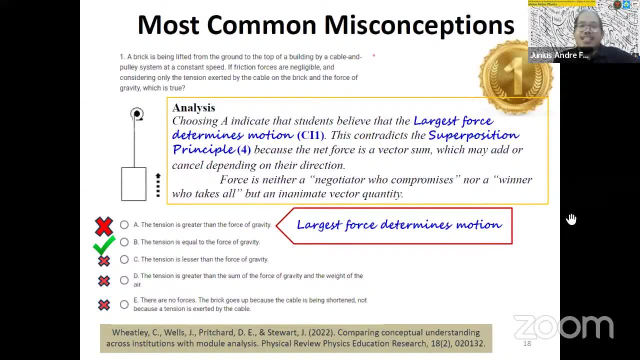 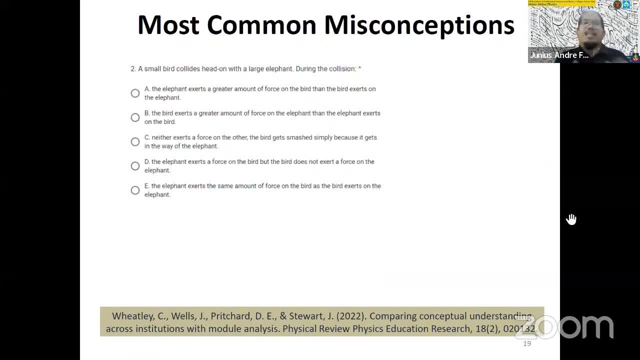 Or si Alin Ayan Ayan, si Ian, Ian Sige sige: Ian go Number two. na po no Sige. Yes, eto Number two. Hmm, A small bird collides head-on. 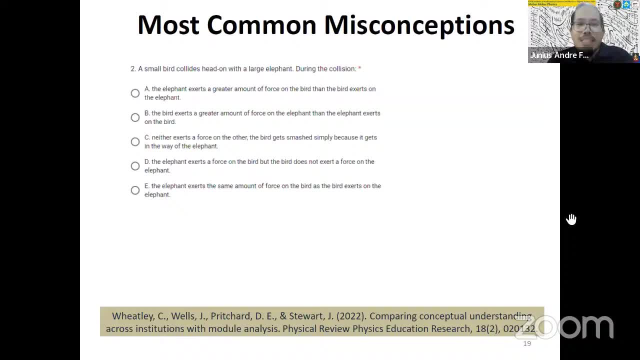 with a large elephant. Sige nga Ikaw, please read. A small bird collides head-on with a large elephant during the collision, And I think po ang tamang answer. ay, hmm, Letter E: the elephant exerts the same amount of force on the bird as the bird exerts on the elephant. since that's the correct answer, I think. 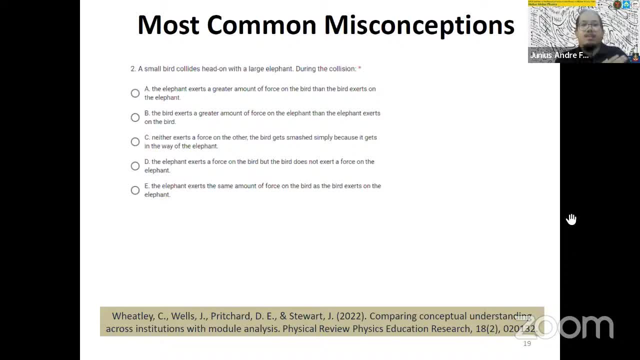 And then yung pinaka, siguro most common na answer dito ay letter A. Okay, so The elephant exerts a greater amount of force on the bird than the bird exerts on the elephant. Okay, let's see. 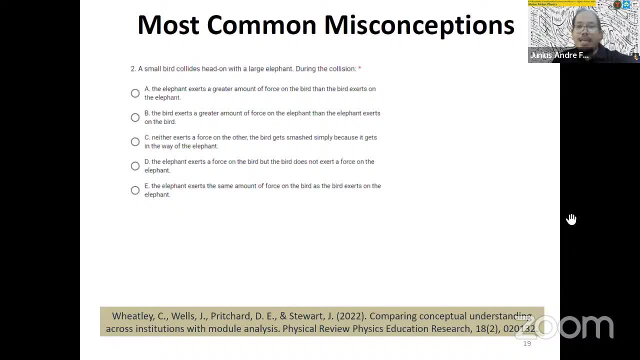 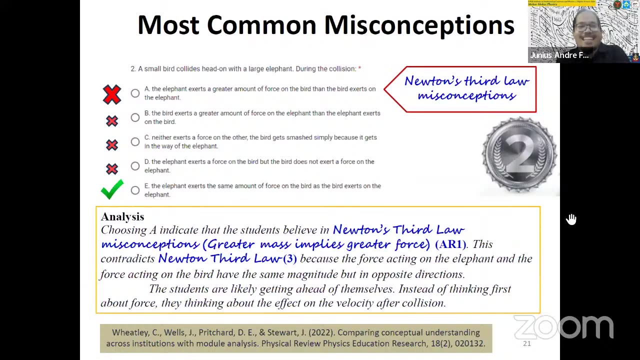 So E is the right answer for Ian. Is it right, Ian, or Ayan, Ian, Ian, Ian? And the common wrong answer is A. Let's see, Okay, it's right. Okay, congrats Ian. So the correct answer is the same. 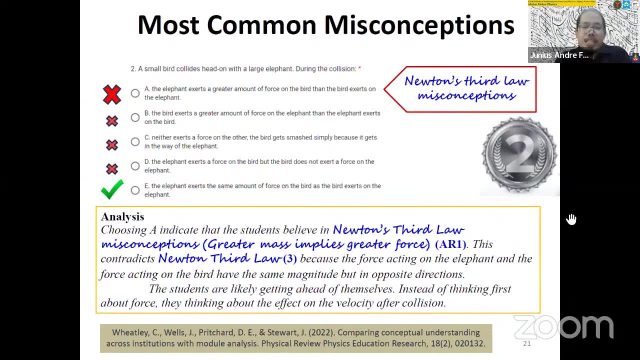 And choosing A indicates that the same dapat the same lang. okay, But opposite. equal in magnitude, but opposite okay When they collide: okay. However, ang common, more commonly common wrong answer is letter A: okay. So choosing A indicates that the students believe. 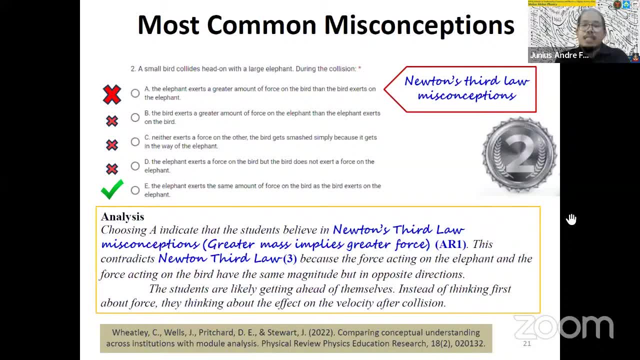 in Newton's third law's misconception such that greater mass implies greater force, AR1.. This contradicts Newton's third law, because the force acting on the elephant and the force acting on the bird have the same magnitude, but in opposite directions. okay, I think the students are likely getting ahead of themselves. 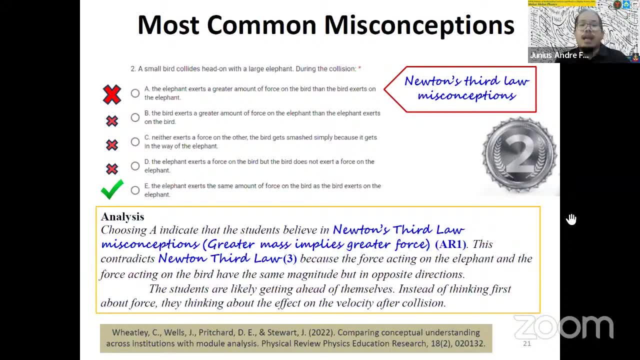 instead of thinking first about force, they think they are thinking sorry, thinking about the effect on the velocity after collision. Nila lump together nila yung force sa momentum or sa velocity. Okay So, but force muna and then. 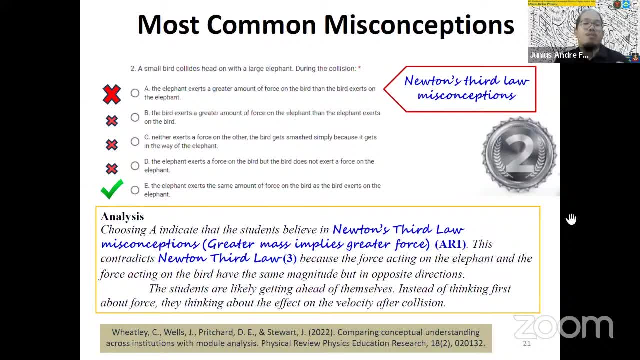 but ang effect nito is sino ang mas malaking merong, malaking change in ano in, in tawag ito in in momentum And you will see, actually, kung momentum naman. 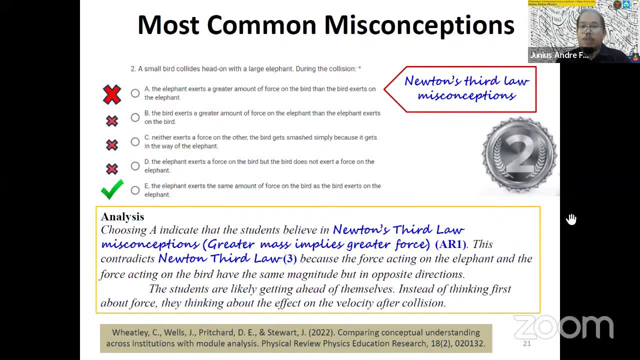 dapat ang bird yung may mas malaking change in in momentum. okay, So next, thank you, Ian. Next is Ma'am Ella sino, ang ating ating volunteer. Andito na ba si Aline Yatko. 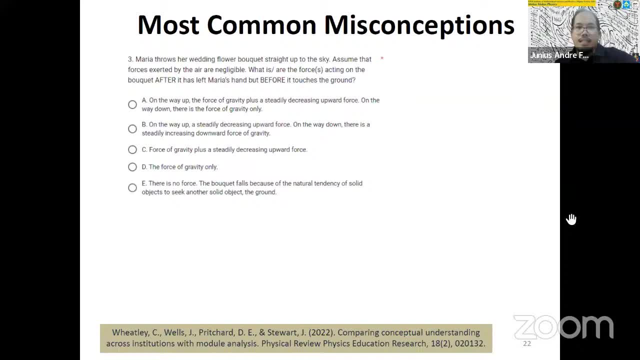 Yes, Ma'am. Good morning, Good morning po. So please read the question, Okay. Maria froze her wedding flower bouquet straight up to the sky, assumed that forces exerted by the air are negligible. What is, or are, the forces acting on the bouquet? 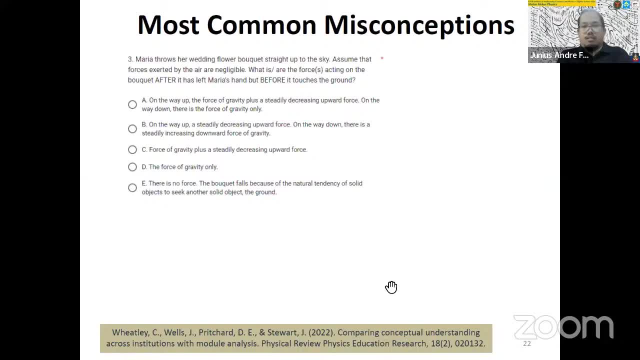 after it has left Maria's hand, but before it touches the ground. My answer to this question is letter D, dog D as in dog, the force of gravity only, And then, sa tingin ko, po the more yung the answer that is most likely to be chosen would be: 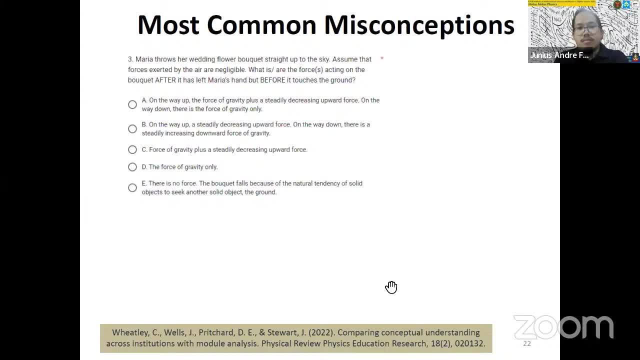 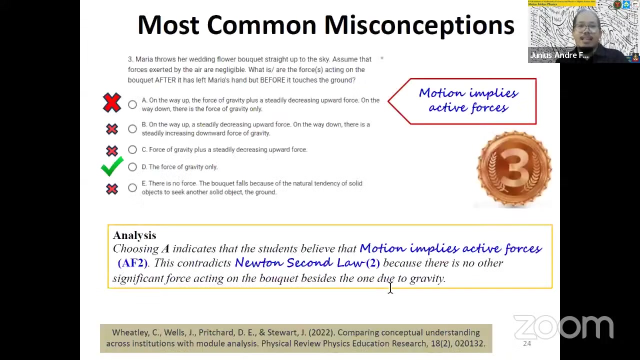 Letter. Letter of letter E- most most common misconception- as the answer letter E. Let's see, Ms Aline naman, yeah, ang correct answer is yes, letter D. pero let's see, Ms Aline naman, yeah, ang correct answer is yes, letter D. pero 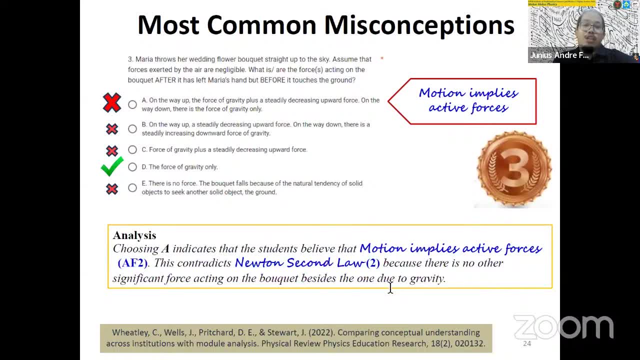 ang mas maraming pumili ng wrong answer, yung letter A. okay, So choosing A indicates that the students believe that motion implies active force. okay, This contradicts Newton's second law, because there is no other significant force acting on the bouquet. 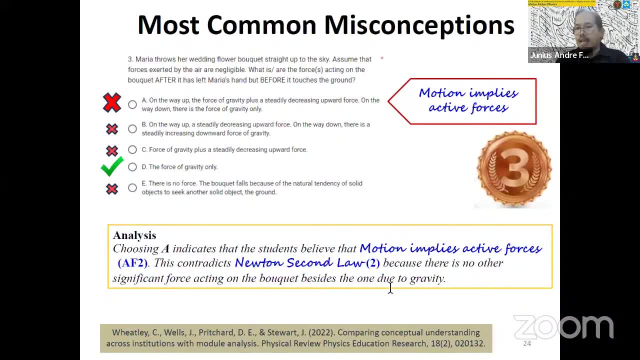 besides the one due to gravity. okay, So thank you, Ms Aline. Thank you, din po sir. Next, Thank you Ma'am, ma'am Pamela, ma'am, Ana, sinong. next, nating volunteer. 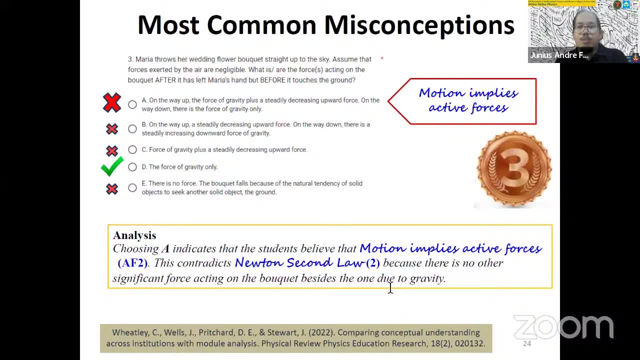 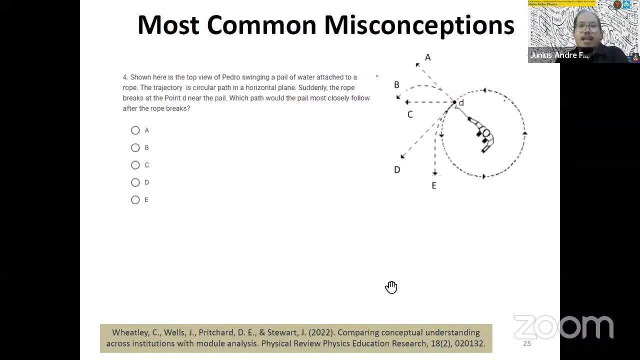 Robert Morante. still here, Robert, Mr Robert Morante? Ah, Robert, sir Robert, Yes, ma'am here, ma'am person. Okay, yeah, can you please read? Okay, sir, Okay, ma'am. 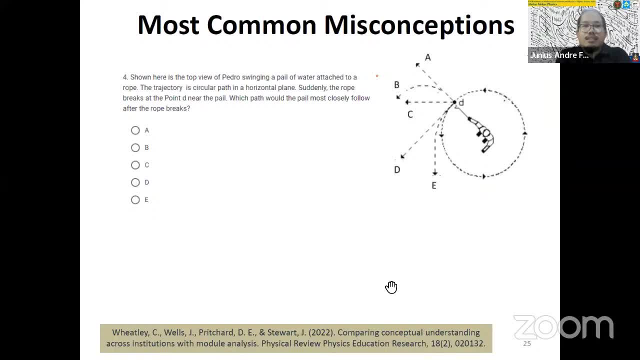 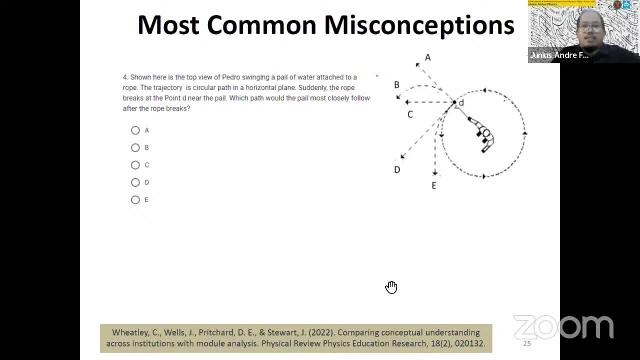 Okay, so Professor Watson and I want to ask you two questions about this question and also about the time we have left. So let me start over. So we have two questions. We will start with this question. We have one question from Joanne. 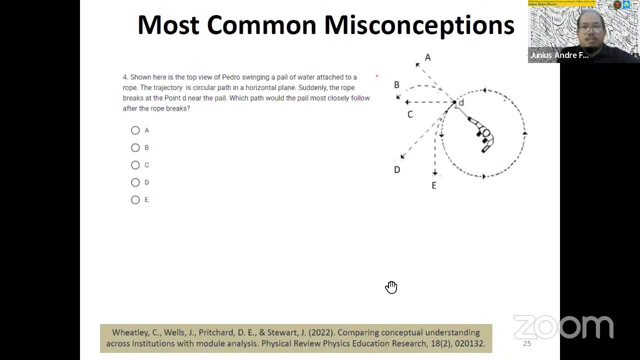 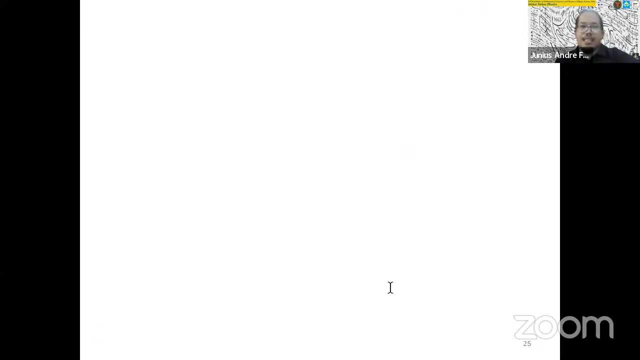 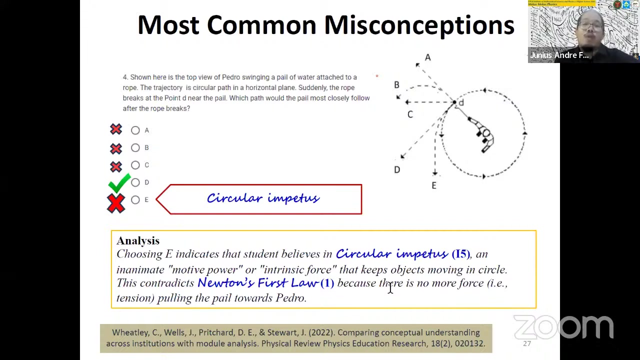 Okay, Joanne, go ahead. I think the correct answer, sir, is a letter E, And the most common answer chosen by students is a letter C, And the most common answer chosen by students is a letter C On the horizontal plane, so dapat zero na yung force. 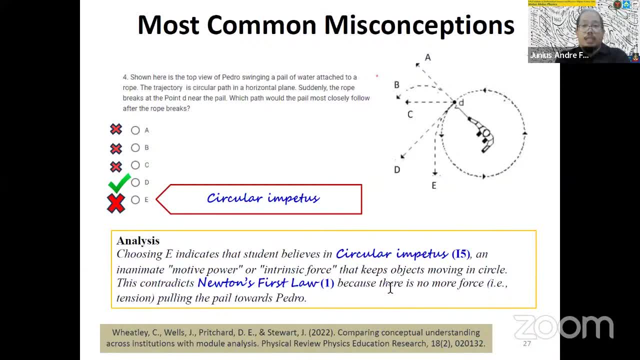 So hindi na mag-change yung velocity, You're in good company also. So choosing E indicates that the students believe in circular impetus. So it's an inanimate motive, power or intrinsic force that keeps the objects moving in circle. 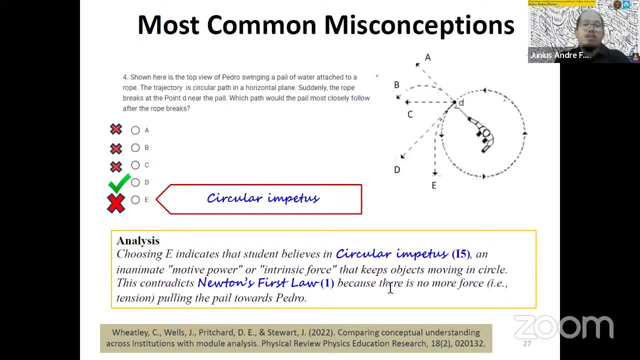 But there's no such thing. So this contradicts Newton's first law, Because there's no more force pulling the pail towards Pedro, So hindi na mag-change yung momentum dapat, So dapat straight line na, at least on the horizontal plane. 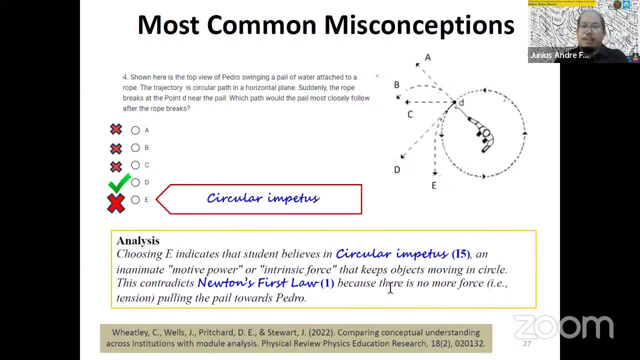 So yan po ang sagot: So common ang E na misconception. The last but not the least, Ma'am Anna. Hello, sir, We can hear from Ruben Cadayona. Mr Ruben Cadayona, Yes, Ruben. 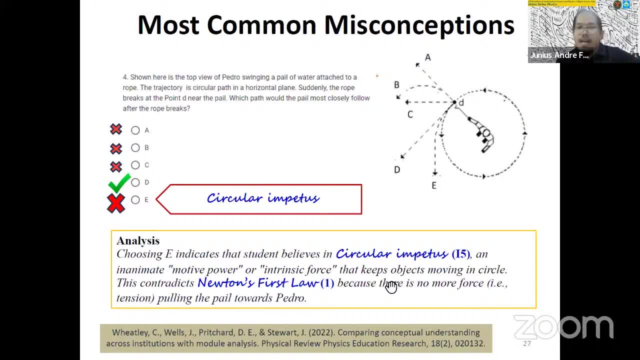 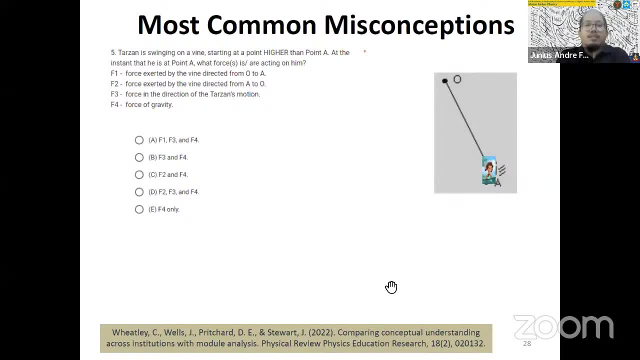 Good morning, Ruben. okay, So, Ruben. good morning Okay. Please read the question. Tarzan is swinging on a vine starting at a point higher than point A. At the instant that he is at a point A, what forces or forces? 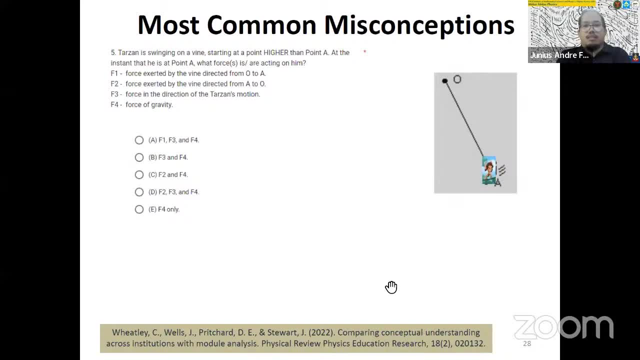 what forces are attracting him on? A? F1, force exerted by the vine and directed from zero to A. F2, force exerted by the vine directed from A to O. F3, force in direction of the Tarzan's motion. 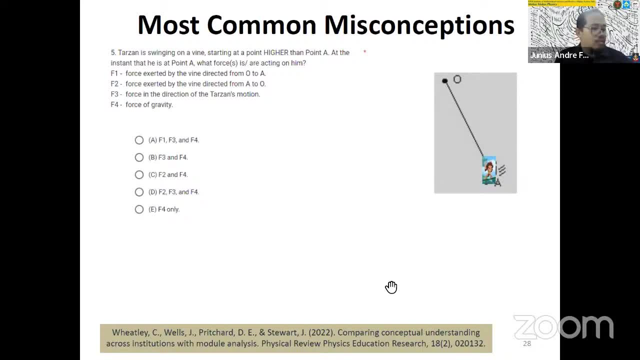 F4, force of gravity. Ang aking answer po here is C, F2 and F4. And I think the most common answers of the students would be A. po Okay, Tingnan natin kung lucky answer ang last question si Sir Ruben. 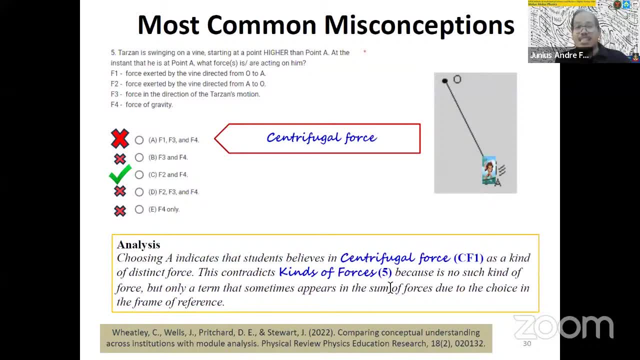 Tama. So the correct answer is F2 and F4. And the common misconception or chosen wrong answer is A. Okay, Choosing A indicates that the students believe in centrifugal force, say F1, as a kind of distinct force. 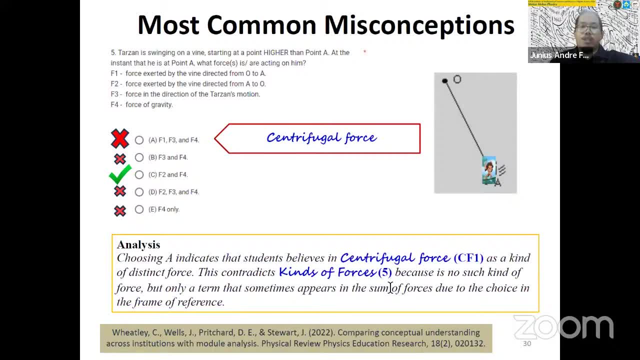 This contradicts kinds of force, the conceptual dimension. kinds of force: number five, because there is no such kind of force, but only a term that sometimes, friends Medyo advanced na to yung pag nagdiscuss niyo, Medyo advanced na to yung pag nagdiscuss niyo. 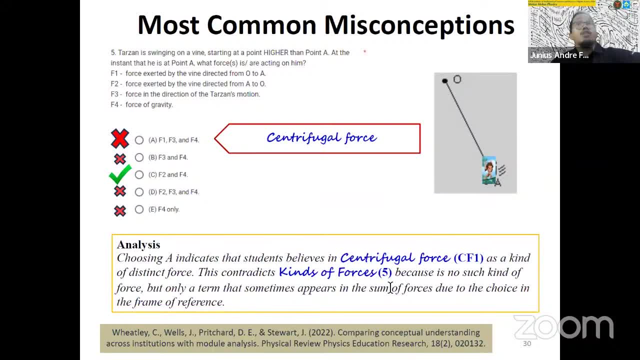 Nagdiscuss usually ng centrifugal force, pero hindi siya totoong force in a sense na may mga force laws siya Dahil lang yan sa choice of reference, So medyo advanced, pero ang centrifugal force is yun nga nage-exist. 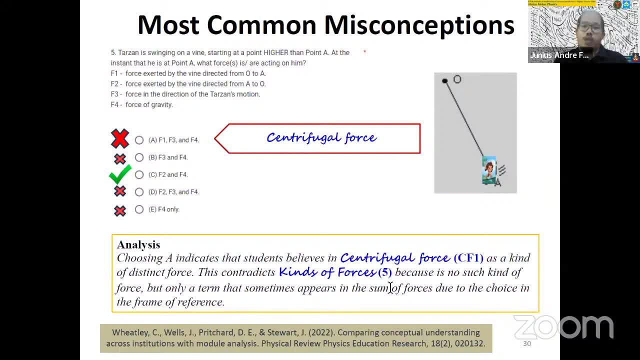 They thought sa basic physics. they thought there's such a force, okay So, but there's no such thing. Ang force nang nag-a-act ay yung gravity, At saka yung tension, At saka yung tension ng rope, which is in the direction from Tarzan to the peg saan nagkadikit yung rope. okay, 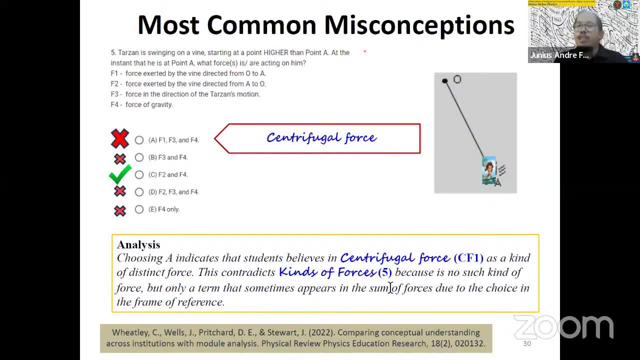 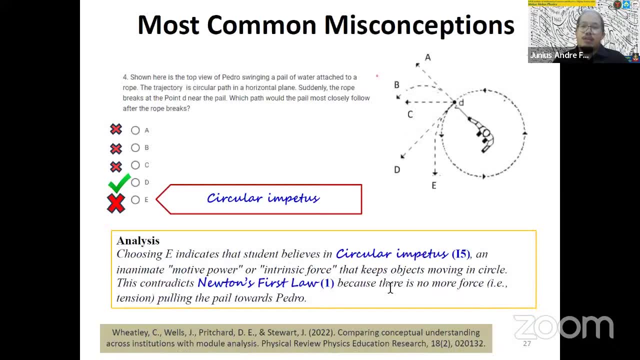 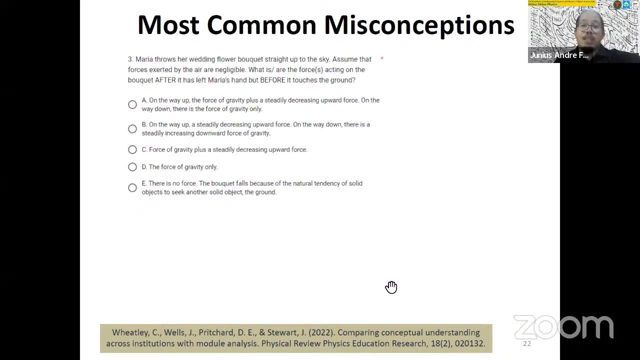 So thank you to the five volunteers. okay, So yun, this is pag nakikita niyo sige. So we will see May naka first, second third. So the first three, ito yung top three, okay. 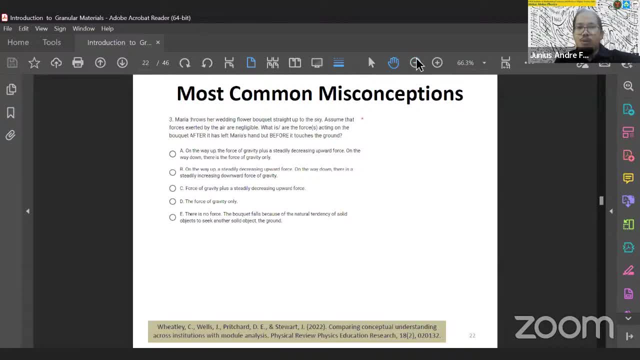 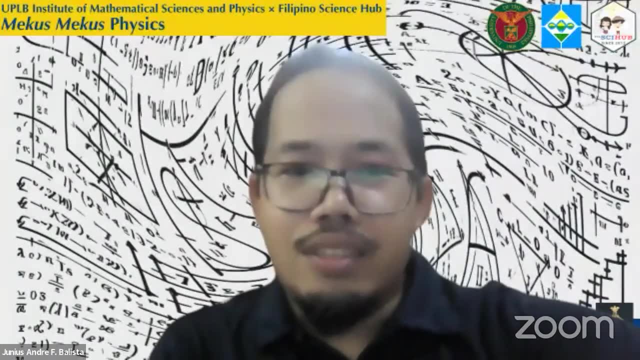 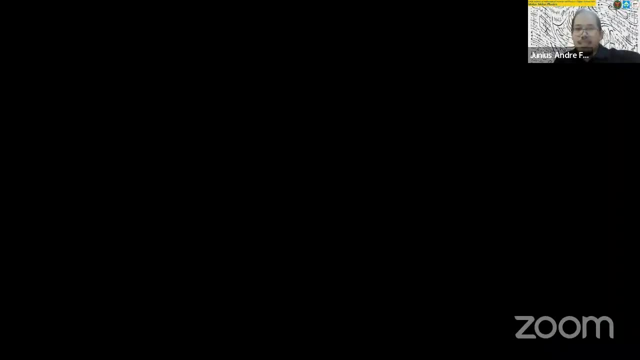 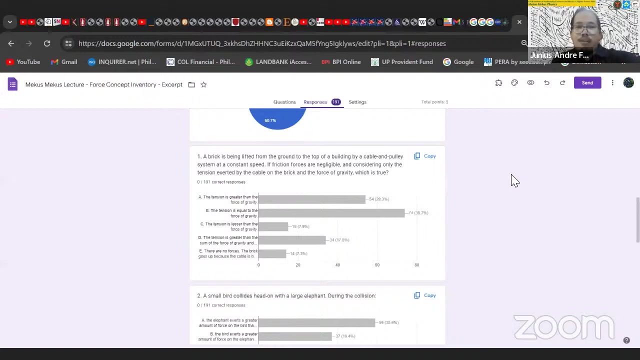 Tingnan natin yung. I will go to our survey, tingnan natin kung ano yung result ng ating survey. Kikita niyo ba. Kita niyo po, Mama Ann, clear po ba yung naka-flash sa screen? 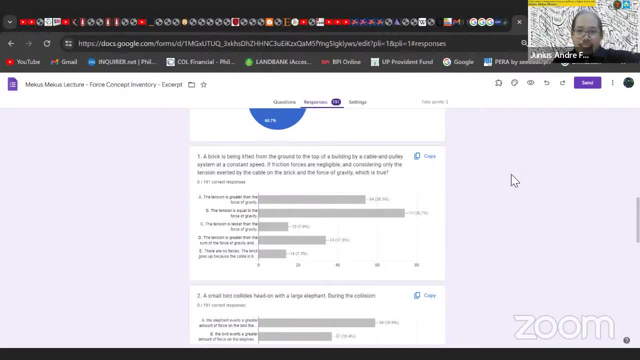 Yes, sir Clear, naman po Okay, So sa number one, kahit tama namang nakakuha yan 74%, yeah, 39%, pero marami rin yung mali, So A ang common misconception okay. 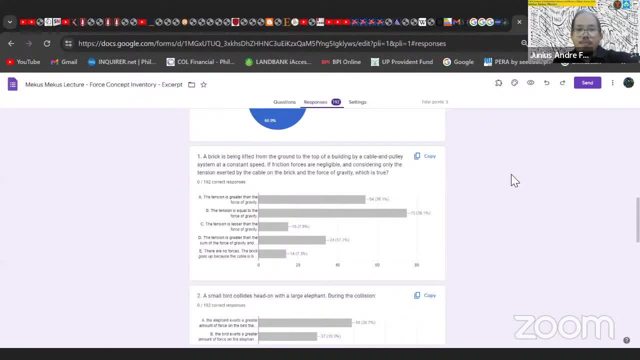 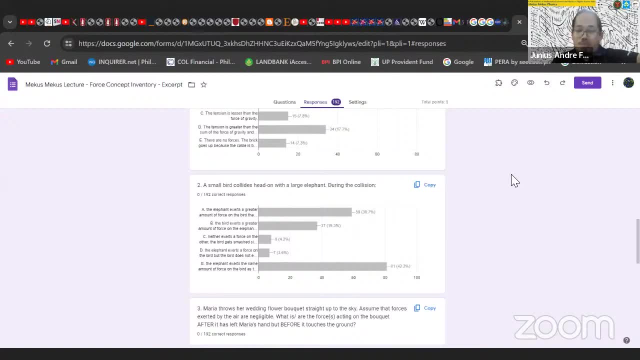 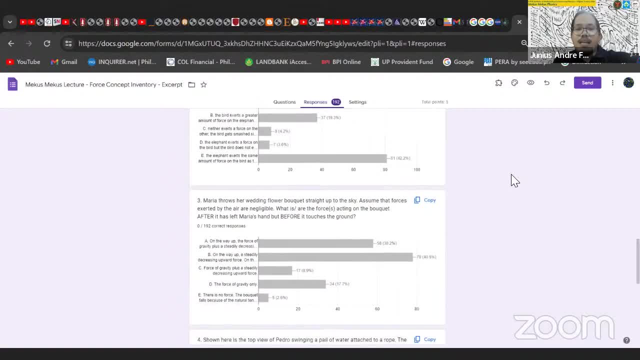 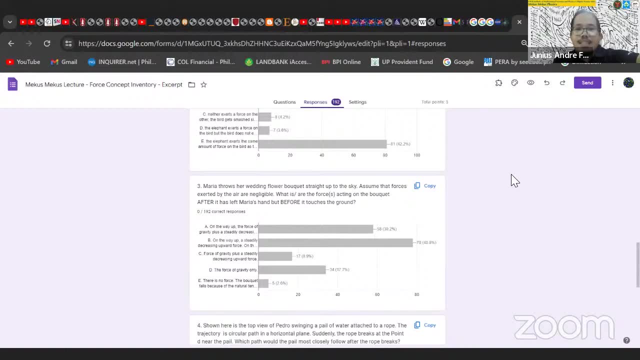 Tama ba, Ayan, So number three, ito medyo malungkot. Ang tamang sagot ay letter D. It turns out ang misconception natin sa number three, number three, Medyo iba dito sa. 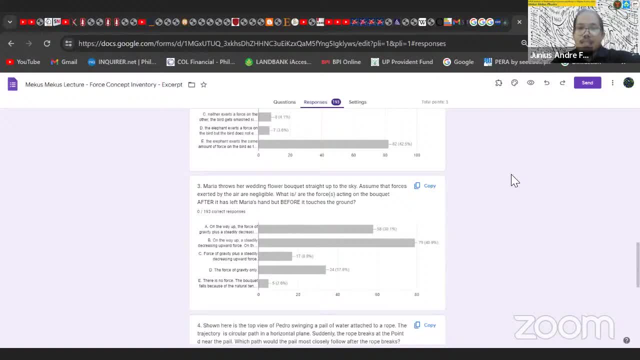 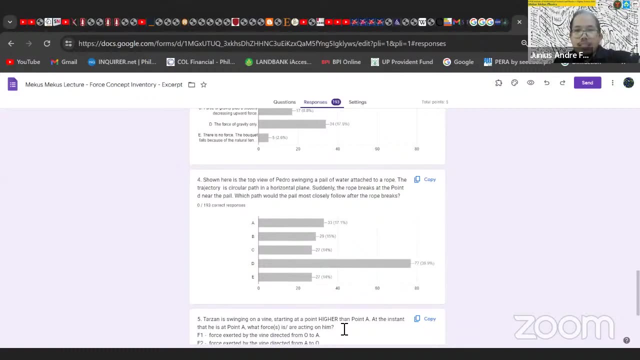 Iba, I'm sorry, Iba ang ano. Okay. Sa four naman, Ang tamang sagot ay Sa number four, Letter D. ang correct answer Tapos letter E: Okay. Medyo iba sa research, Ang result ng ating Survey, Pero ang tamang sagot D. 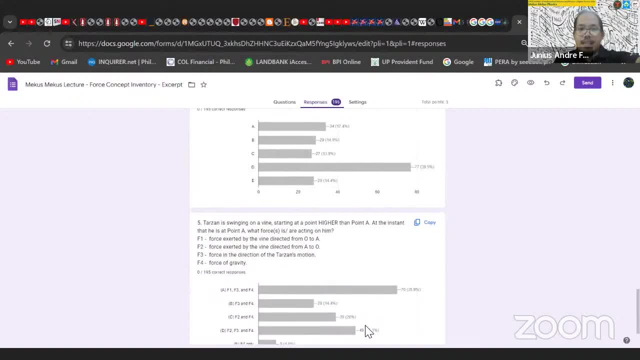 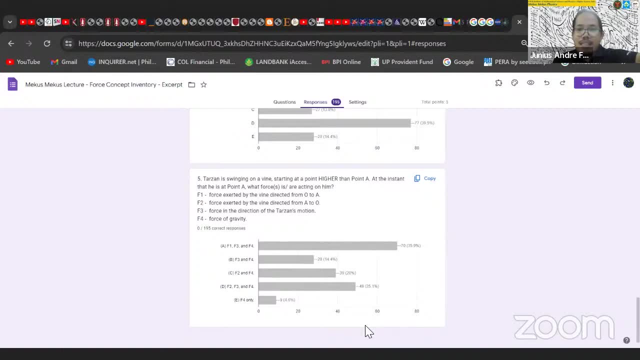 So in here most of us Got it right. And number five Ito? Ang tamang sagot ay C, Pero ang karamihan Mali, ay tama. Ang misconception din dito, Similar to the Research that I will talk about Later on, Is A. Okay Ang daming na. 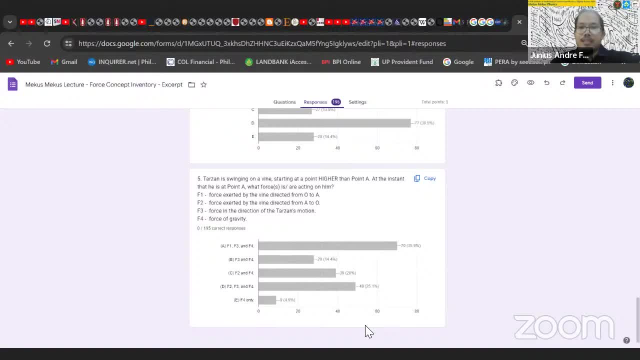 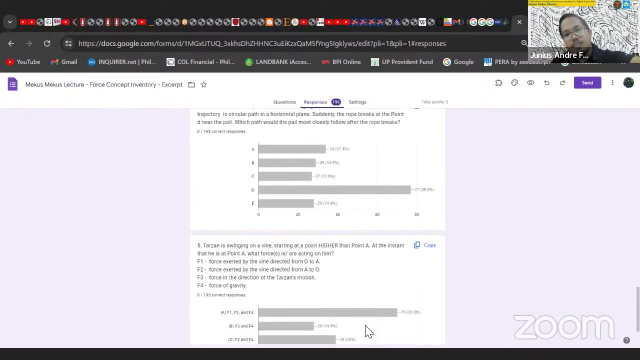 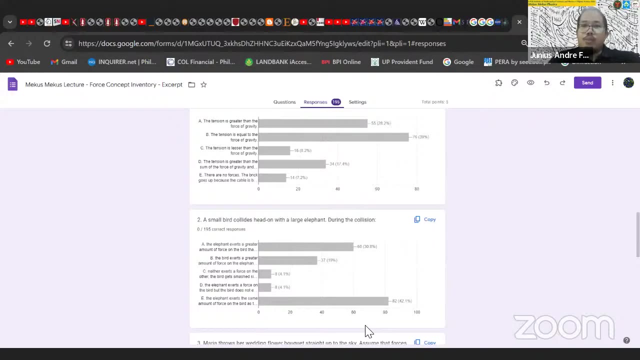 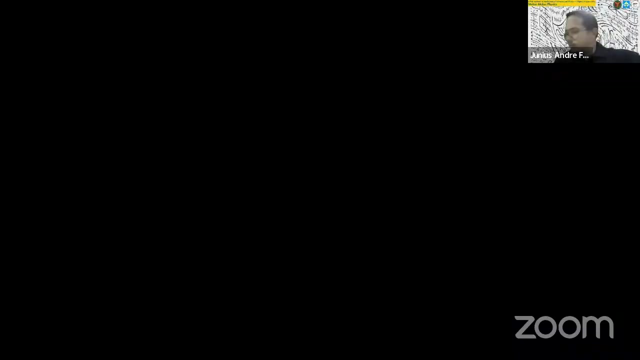 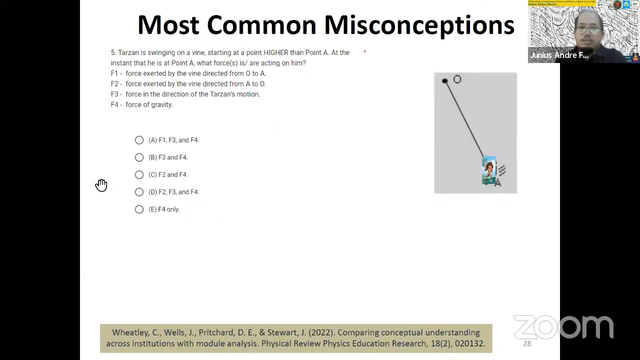 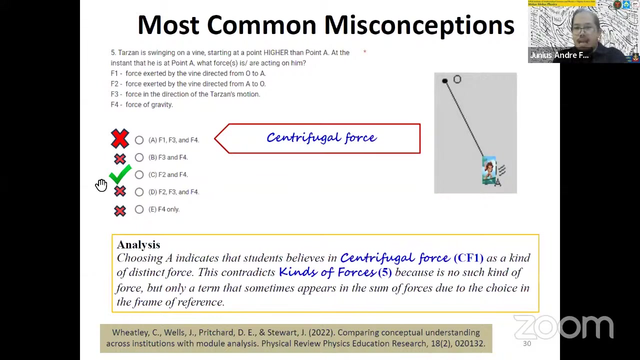 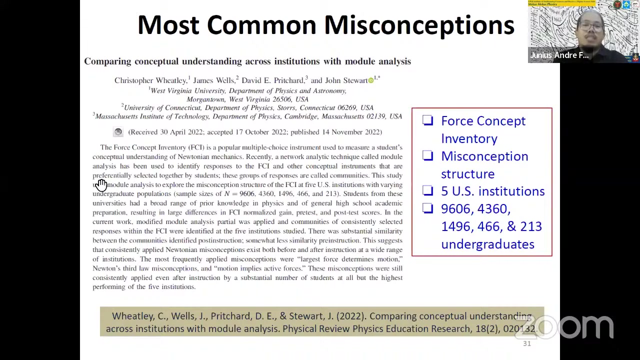 Ang misconception dito. Okay, Okay po ba. So ito po yung ating result Yan. So that's the result. Okay. Now, Going back to similar study, was done recently, So this is 20 year. last year, Okay, Done by Wheatley et al. Okay, 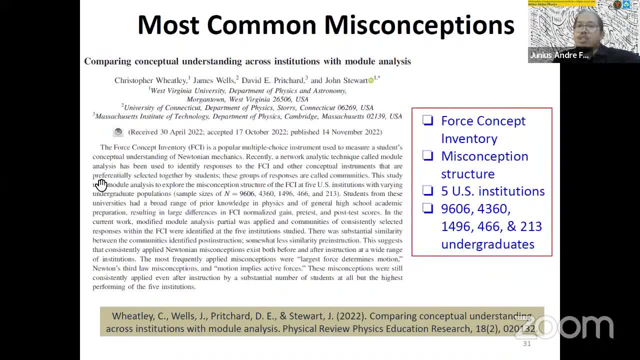 So basically It uses the force concept inventory To study the misconception structure of Five Of students from five US institutions. Okay So I think I include dun yung MIT, So mga top universities din Sa Sa US. Okay So, Nine thousand Four thousand One, five, Four hundred And two hundred. 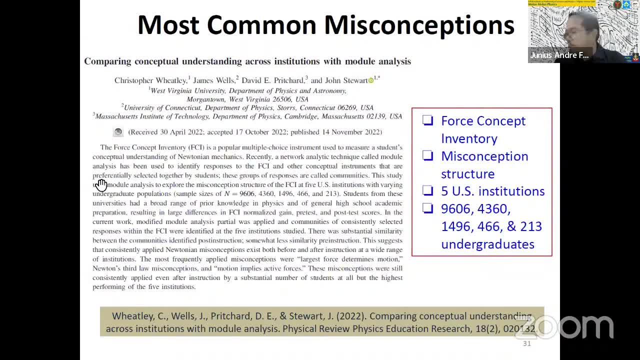 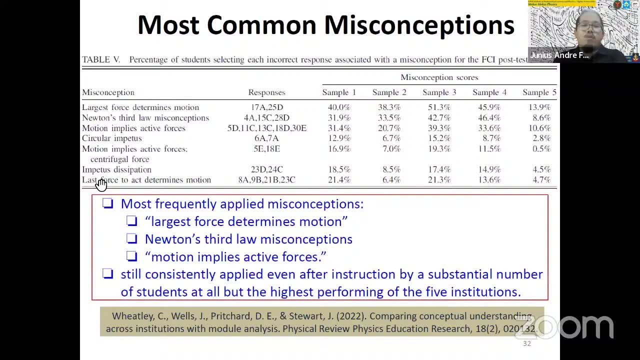 Undergraduates. Okay, So this study Did a similar And ito po yung kanilang result. Okay, So What they identified is the most frequently applied misconception is that The largest force determines motion. Then yung Newton's third law- Okay Misconception. And then motion implies active force. 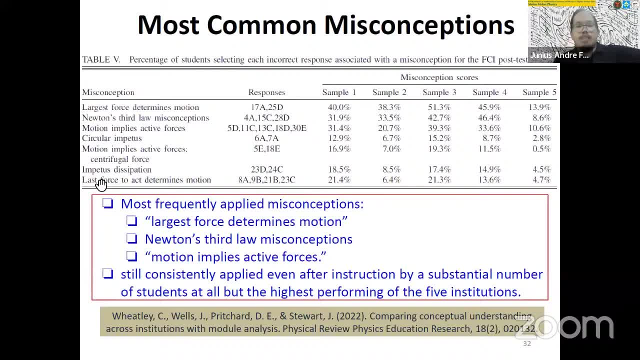 Okay, Misconception. and then motion implies active force. Okay, So, using the taxonomy Yun, These are the top Three, Okay, And what is notable is that It's still consistently applied Even after instruction, by a substantial number of students At all, But the highest performing Of the five institutions. 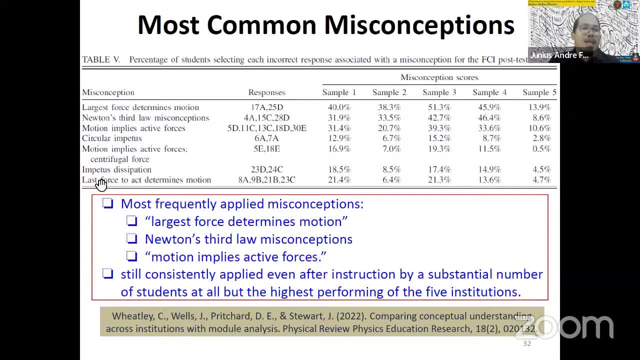 Okay So, kaya sabi ko, yung good company, kasi Marami Yung sa top three. Yun din yung common na Na misconceptions ng Mga Sujante. Okay So, ito po yung Top three. Okay So, anong kagandahan po nito? 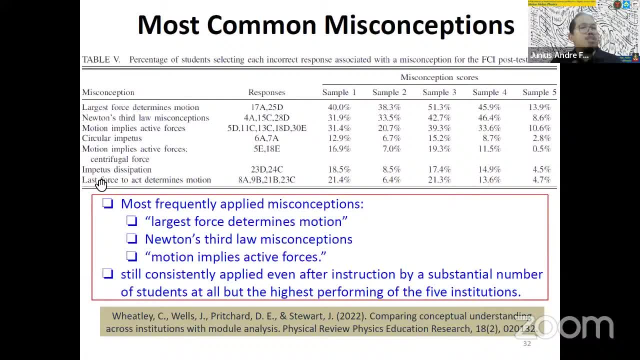 Kasi Diba Dapat. the way to address Misconception is to To be methodical, And We don't have the luxury of: Yes, dapat nag item analysis yung teacher, Okay, But it's a good thing Na Nabe benchmark natin. Tapos na nakaka. 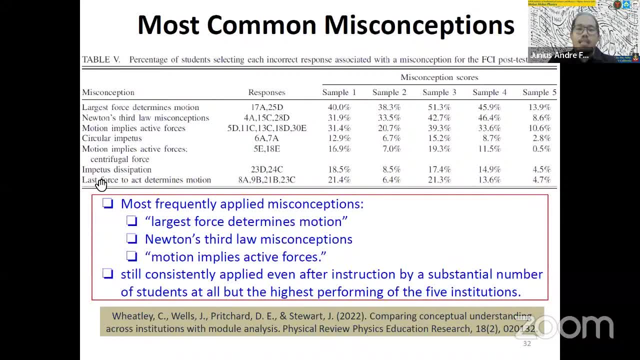 Relate tayo Sa Sa Sa challenges Ng ibang institution, Okay. So it's also good thing that we can benchmark it. So it's also good thing that we can benchmark it To know what the And Studies like this, Okay Will guide us on how to Address. 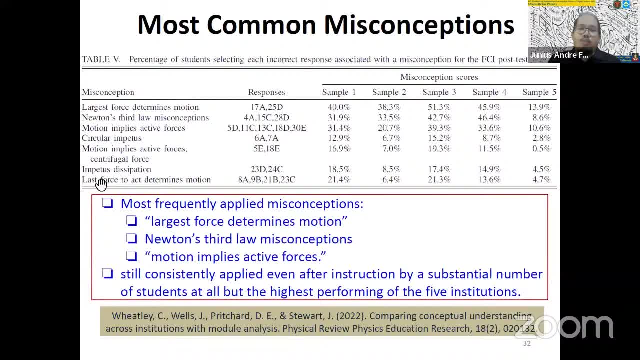 What to watch out for. Okay, So It is important to, To To know this: What's happening In other institutions, What's the experience of other students Or other teachers? And Hopefully, If we We identify what are the most Common, Okay, We can Preempt, We can Make Preparations. 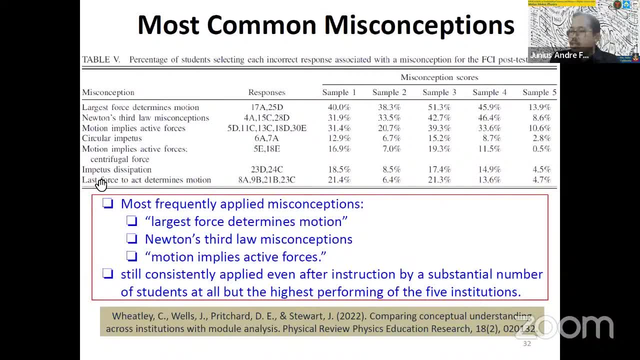 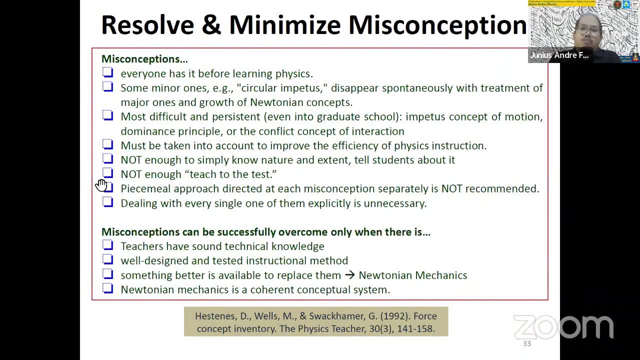 Okay, So The last part of the This Talk, This conversation, Is Basically Just an offer Of Some Suggestions On how to To To Deal with Misconception. First is that we have to Again to recap, To understand That. we have to understand That Everyone has it Before learning. 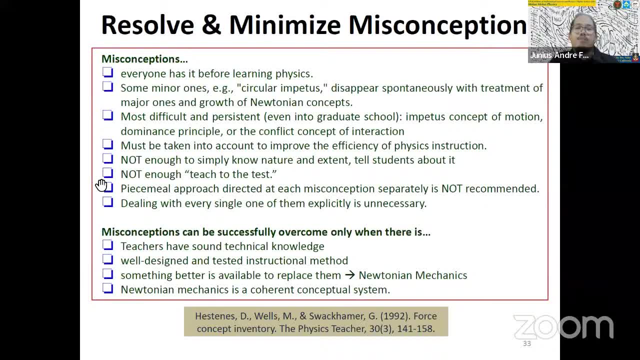 Physics. Okay. So Because, as I mentioned, We, We, Our natural reaction Is to use Our senses And, Like Aristotle, We describe Things as we see it. Okay. And Misconceptions Persist, Some minor ones, Like circular Amplitudes. They disappear Spontaneously with As we study Physics. 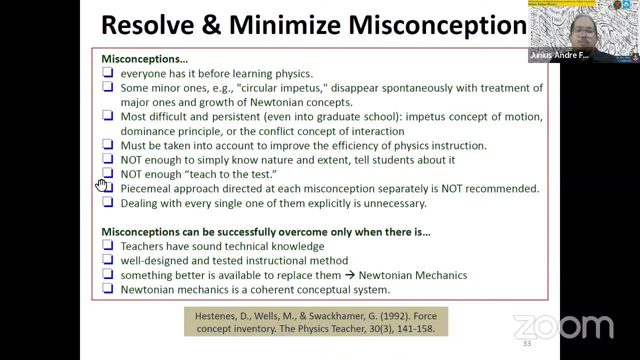 Okay, But there are More difficult ones, Most Difficult And Persistent, Such that even Into graduate school- Or You can Deduce from here That even teachers Will have it, Because let's say: Teacher, Hindi naman, Hindi pa Nag PhD Or hindi nag Masters- We now teach Into high school. 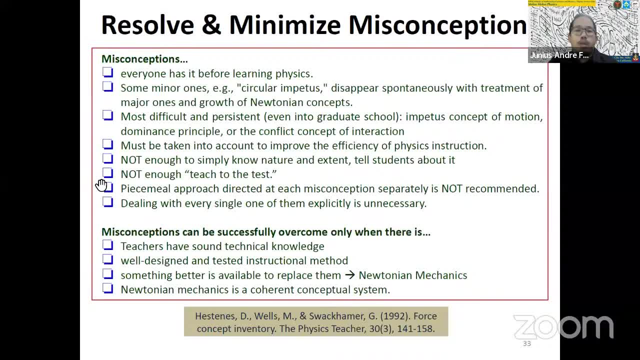 So kung If some of us Go to grad School And still have Misconception, How much more Those who don't Go to grad school? Okay, So Ito nga Yung Common Is Uh Impetus Concept, Dominance Principle Or conflict Concept Of interaction, Yun yung. 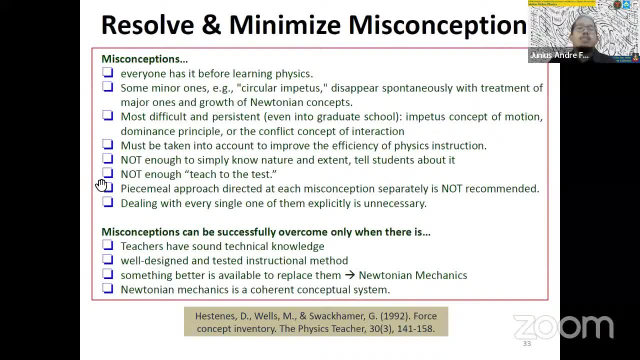 Binigay kong Example: Kanina, Yun po yung mga Persistent Okay, So Don't despair. Of course We are not happy. Kung baga Hindi, naman We don't say na We are happy, Kasi marami tayong At least Marami kang karamay. 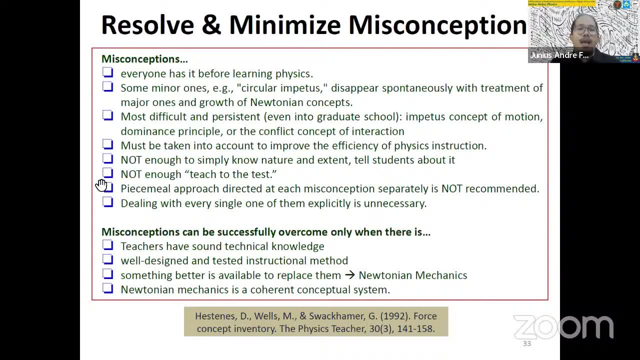 So this: When we know That many are Suffering Or carrying This misconception, We know where to focus. Kasi ang daming Kailangan gawin, Pero at least Kung na-identify mo Sino ba Alin ba dito Ang kailangan pa. 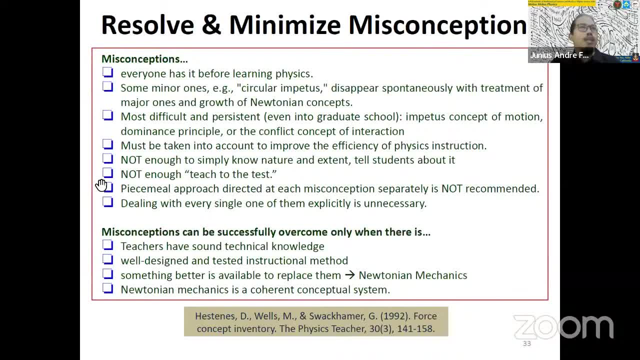 Ng more attention. So ito yun Okay. And don't really feel bad Kasi. even Uh The best of us Uh Still suffer From misconception. So don't really feel bad About it, But let's do something About it. Uh, sorry, Ma'am Ana, I'm still okay. 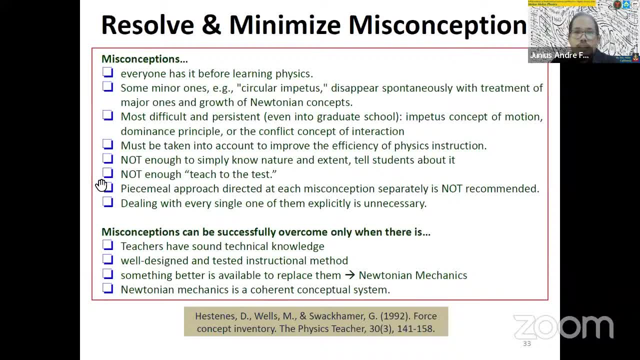 Yung sound ko. Yes po, sir. Okay, Medyo nag Plucked fit kasi Okay. So ito Not enough to teach the test. Okay, Isa, kasing One. One temptation is Ang gagawin ng teacher: I-access niya yung First concept inventory, Tapos i-review niya yung. 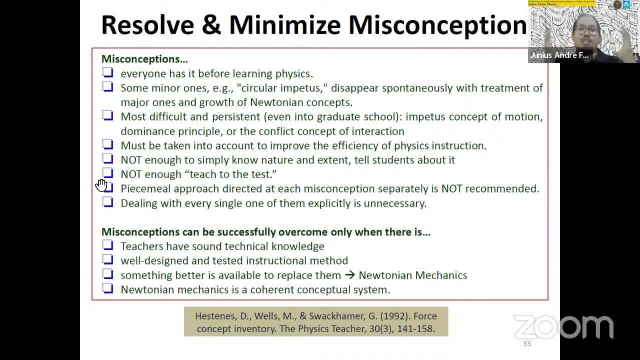 Students doon, Isa sa Pwedeng maging Temptation natin Okay, Or lalo na, For example, Malaki Yung pressure Sa mga standardized exam, Ang tendency natin Ipa-practice natin, I-review Center natin Yung Yung Yung. 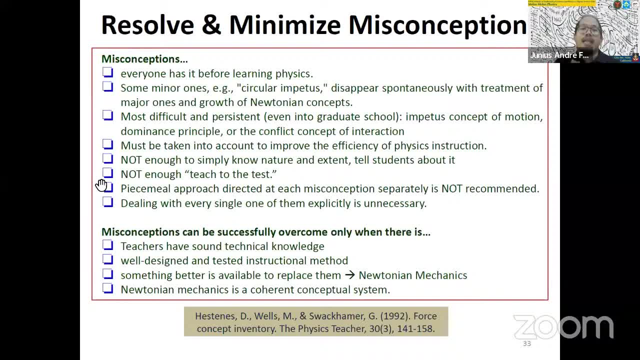 Uh Yung exam Para to Ma-address natin. That is not advisable. Aside from Siyempre Lalo na sa First concept inventory. Uh, Sinasabi talaga Ng developer Na wag natin I-proliferate, Wag natin I-test doon. What do you mean? 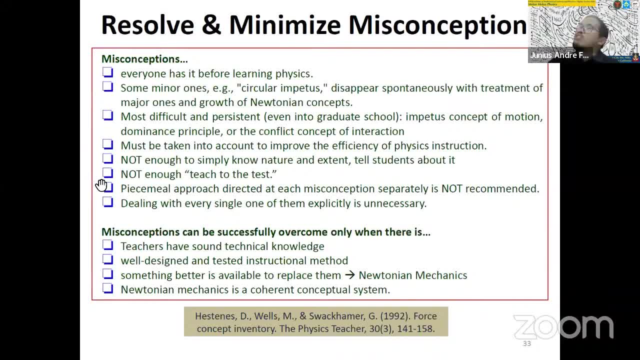 Teach to the test Yung exam. Tingnan natin Tapos Arali natin Anong correct answer Tapos I-review Review natin. Okay, You may get there. You may After a while Your students will get A high score In that inventory, But that will not. 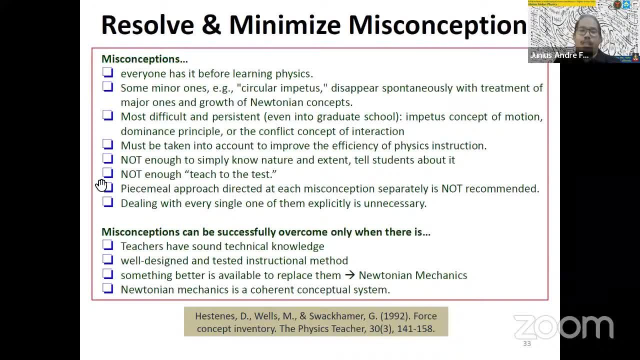 Remove the misconception. Okay, So, yeah, That's why Then? Uh, Piecemeal approach Directed at each Misconception Separately Is not recommended. So, although We identified The misconception, Okay, Uh, We, I'm not Suggesting that We We Treat them Individually, Because 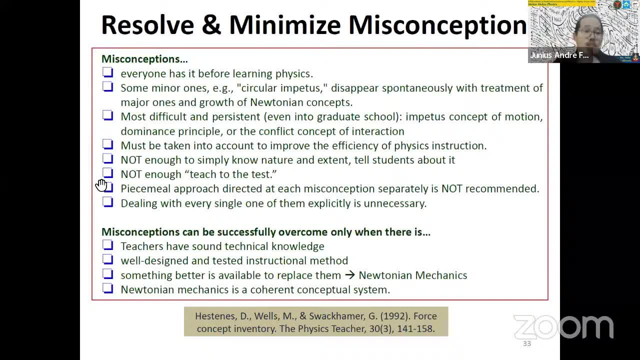 As I mentioned, The Newton's Laws of motion. Yung three laws Na yun. They're talking about One thing, So you must look at them Together, You must consider them As a whole, Defining Force Okay, And so It's not necessary To deal with them One by one. 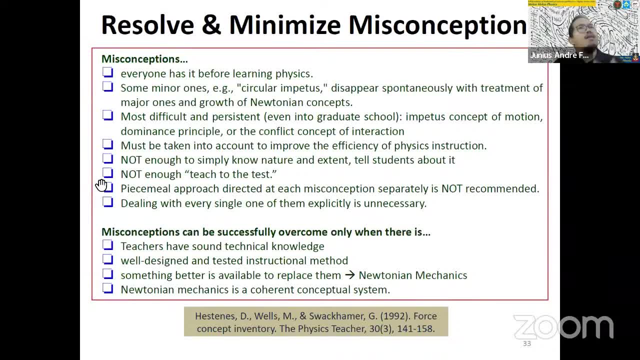 But rather To To To have A More methodical way Of teaching Newton's laws. Okay, So misconception Can only. I will. In closing, I will Discuss At least Some one way To do that. So misconceptions Can be successfully Overcome Only when there is A teacher, When teachers 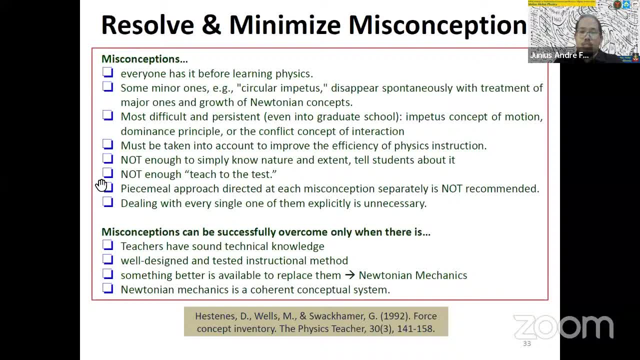 Have sound technical knowledge. So of course We must know Newton's laws, The one that teaches Okay, And you have Well designed And tested Instructional method. And We must keep in mind That We are replacing Something. There's an existing Worldview. The students, The teachers Have existing worldview. 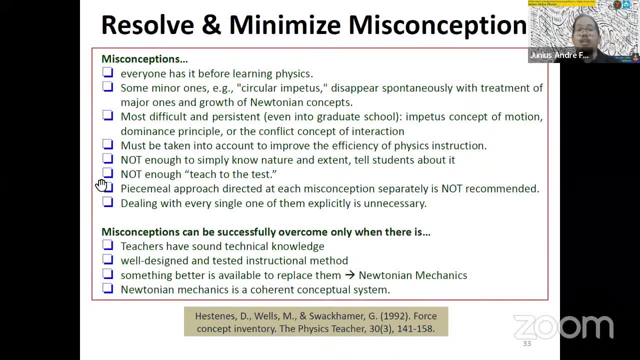 We have a default Aristotelian view And To Remove These are- We call These things As Maybe Misconceptions. So It needs to be replaced. So there's a replacement And the replacement Is Newtonian Mechanics. Okay, We must understand That the Newtonian mechanics Is a coherent. 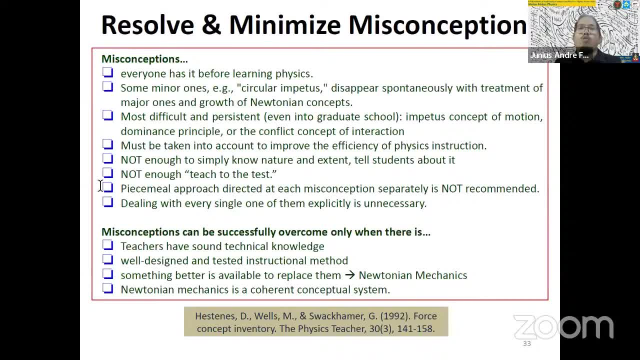 Conceptual system. Okay, So We must Accept That Newton Is correct, Because You can't Teach, Because You can't say Aristotle is wrong. Then what do you replace? Okay, So You must replace And show That It's superior, It's correct. You're replacing What's correct. 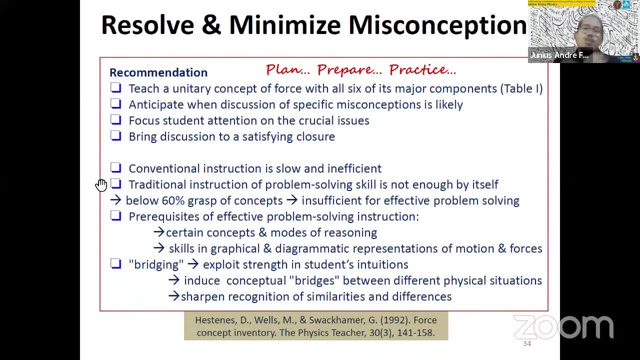 Which is Newtonian mechanics, Okay. So Recommend With each A unitary, Unitary concept, Of course, With all the six Major components. It means Teach it as a whole, Emphasize That the three laws Are interconnected And This, This lecture, For example. We now, We know, We are aware. 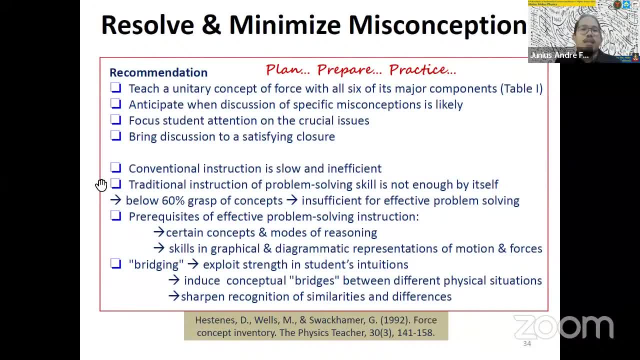 Common Misconceptions. So you anticipate it And then You. This will Allow you to Lead the Lead students To focus on the Crucial issues. We don't do it Piecemeal Or separately, For at least Identify Where most likely It's wrong. Okay, And Bring discussion. 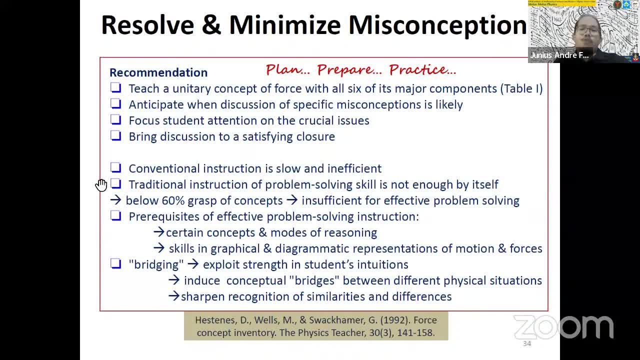 To a satisfying Closure. Okay, Conventional instruction Is slow and efficient, Just the lecture. So Actually, this one. That's why This one, Like what I did, is I tried to Interact with the students. This is not satisfying, Just the lecture, But Yeah, We have to start somewhere. 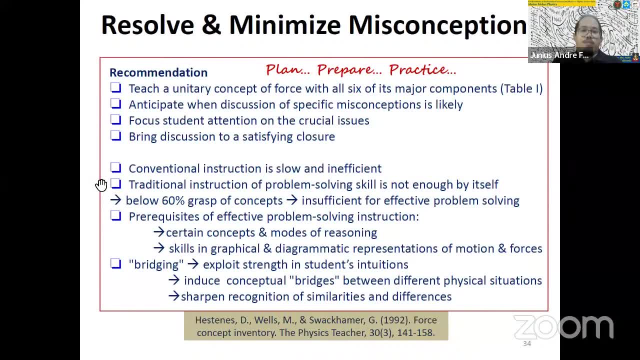 But It really should be, I It's not just a lecture Then. Yes, We teach problem solving, But there are- We have to understand That- If there are Misconceptions, Especially Problem solving. So there are prerequisites To problem solving. You should Learn Your students To Graphing Diagramming. 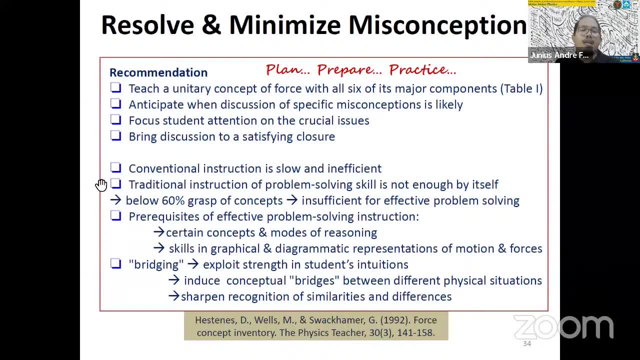 Then You don't throw Away everything, But you Try to use What's available. The student knows. Try to Salvage, Build on it, Identify Which is wrong, Then The newtons, The correct, You will breach That. So you don't really need To start from Zero, Because that's not possible. 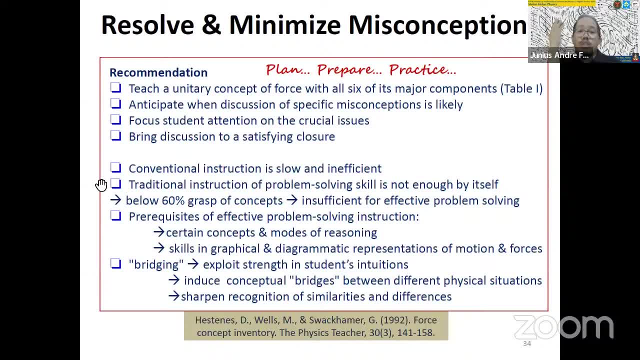 You cannot erase The, The memory Of Our memory, Or the, The memory Of your students. So that's where The Aristotelian. But when you identify The misconception, You know This portion Of his idea Will be removed. Then this The newton. So you breach What is good. 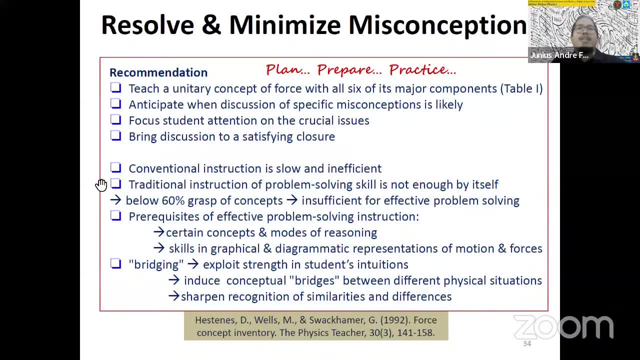 And then the newton That The- Because the observation Is still important- The There are aspects From Aristotelian view That are still useful. Okay, So that's what Builds. We call that one Intuition. His intuition Is from his senses, His intuition. And then the newton. 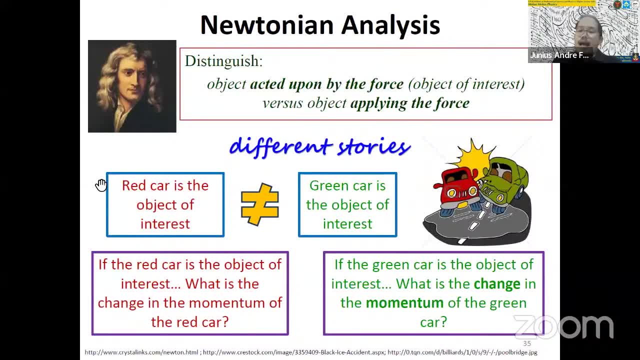 Okay, So We only have a few One hour, But let me leave you With this, Somehow, Some key points That I think Are notable In Aspect of the problem. So I think it's important To emphasize That Aristotelian worldview Is a bit passive. A, A, A, A. 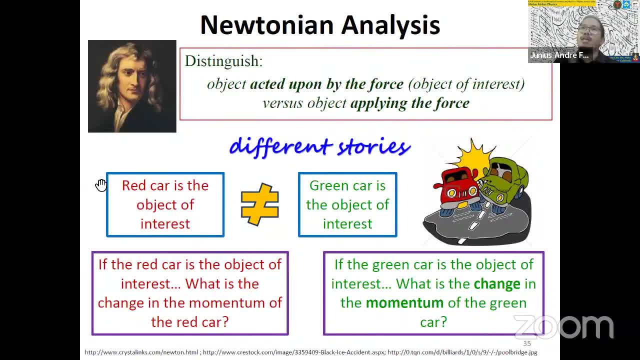 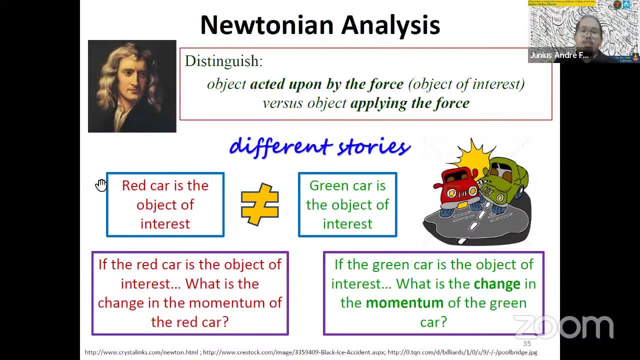 Eyes Smelt, et cetera. You need mathematics, so it's more, more proactive process. and by doing a more proactive process, okay requires Newtonian analysis. how did Newton think okay? Newton think okay. it's important to emphasize that when you look at interaction or motion, for example, the interact 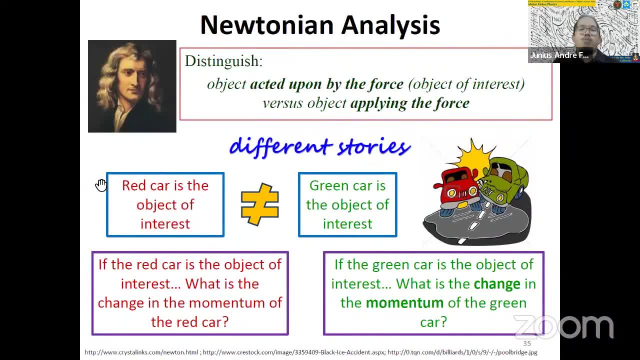 moving objects that interact sila, you have to distinguish the object that is acted upon by the force and the object. so yun po yung tawag natin object of interest, then, versus the object applying the force. so we must keep in mind that when we do, 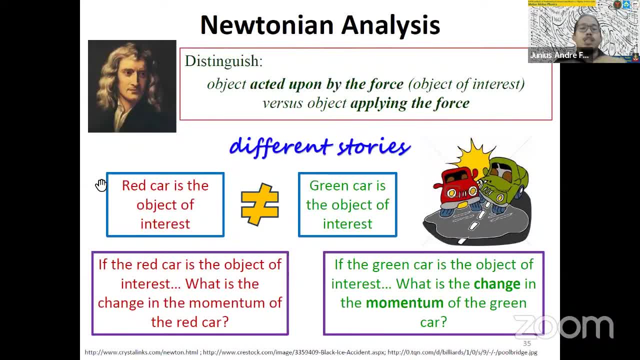 Newtonian analysis. there's an, there's a decision to be made. okay, because in one equation you cannot talk about, in this case, dalawang car. Hindi mo mapag usapan sabay sabay yung momentum ng ng red car at green car. in one line of equation you have to decide sino ang magiging object of interest. when you say object of interest yung object na gusto mo pag usapan, yung momentum, the object whose momentum you want to measure the change. okay, so if you say green car, that is the momentum of the green car, is the momentum of the green car. 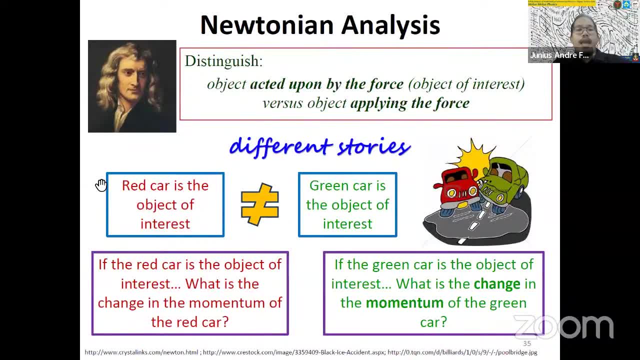 you're going to measure over and then treat the red car as the one applying the force. okay, so you there's. this is related to the next item, though, but let me recap this slide here. we must be conscious that there is a decision to be made. okay, when you are talking about motion, especially when there's an interaction between two objects. 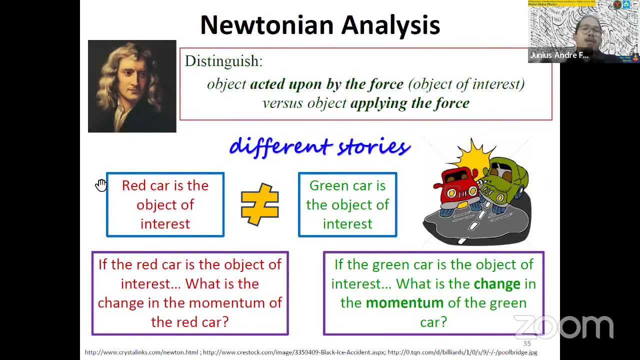 you have to decide which one is the object of, identify what's the object means. but i think it's important to to tell the students or ourselves that, no, we are making a major decision here. we're just starting to solve the problem, but we're already making a decision. we are choosing the object of interest, okay. 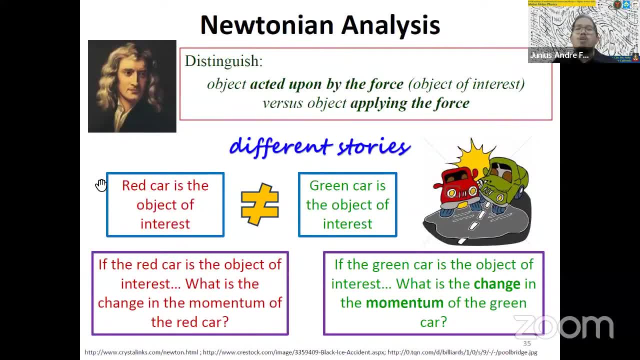 that we made a decision, okay. so there, so you're conscious thinking, conscious that we are thinking we are making a decision. okay, so we're not yet solving the problem, we're not yet setting up the equation, but we're making a decision. so the students should be aware. 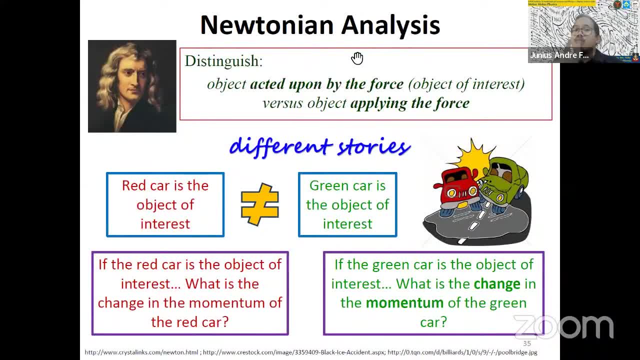 that we're making a decision. okay, so we're not yet solving the problem. that we're making a decision, okay, so we're not yet solving the problem. actually, my active, my very important event, or, uh, action, that the making of the decision to identify which is the object of interest, okay, so, 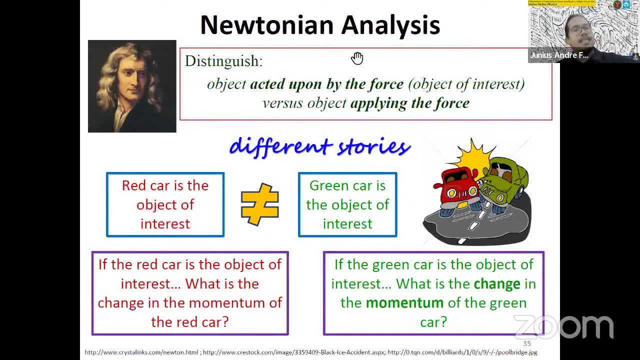 okay. so in this case, if the green car is the object of interest, the question is: what is the change in the momentum of the green car as a result of the interaction, different behavior and interaction and variety phenomena, if it's a red car. if it's a red car. 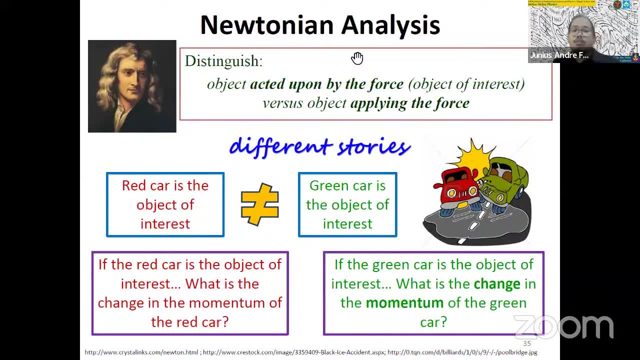 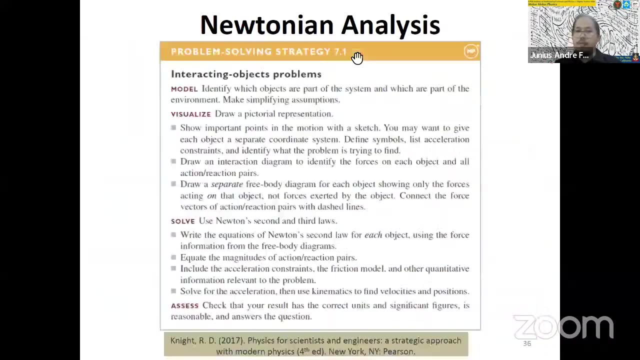 the momentum of the red car. so it means the force is due to the green car if red car is our object of interest. okay, so that's a conscious. it's not natural to think that you have to, to be aware that you're doing that. okay, actually, you. 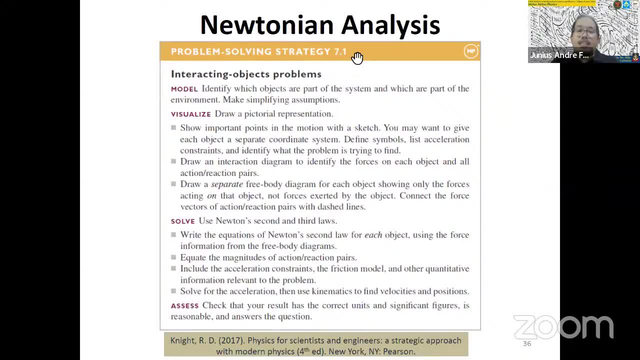 will see, this is common strategy advice in the strategy book. so this one Light Fiction and Diction of Test lastingumuz loy invit printed, and this good textbook called Amitav and Ethic Angie, how's it going? so let's review the feed there structure, and that this is the example that the research, uh, the tools, are you the strength of a strategyと思offin. 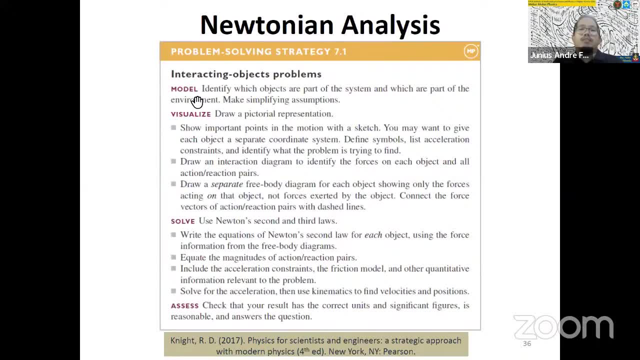 So this one good textbook, Tingnan mo dito Model: Identify which objects are part of the system and which are part of the environment. Tingnan nyo Hiwala binigyan po ng separate na section sa problem-solving advice. 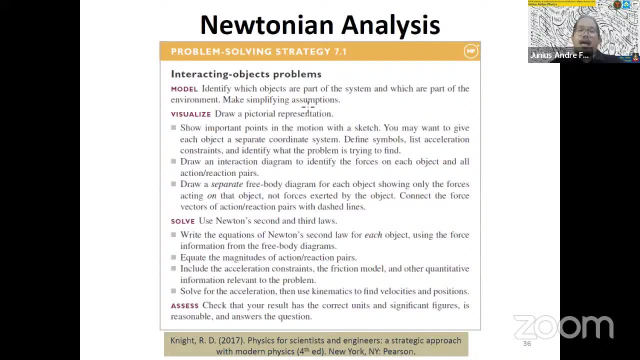 So importante po yan, Okay. And then sabi to proceed with the problem-solving: we need to draw, Draw, We have to draw. So tingnan nyo. These are active, proactive processes. Kung Aristotelian lang, titignan mo lang yung may gumagalaw yung car, ano sila. 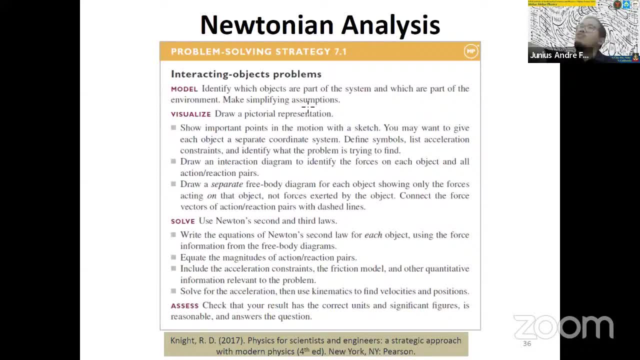 Pero pagsabihin ay teka lang decide first sino ang pag-usapan natin ng momentum. So that's an active. Next, you draw, You draw. Ah, i-isolate mo siya. 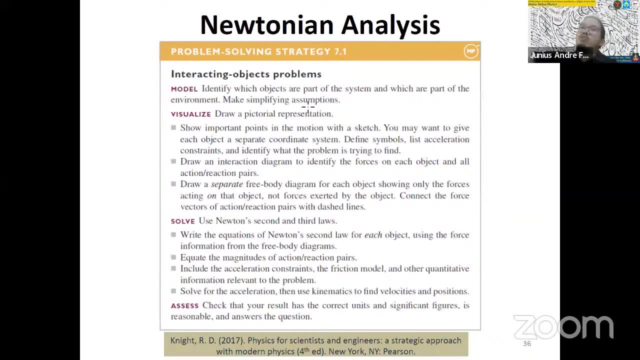 So na-isolate mo na yung object of interest, Sino yung interest Environment. Ido-drawing mo pa You have to draw it. These are active, proactive processes. Okay, Then saka, after you've done this, saka muna iset up yung equation at saka isosolve. 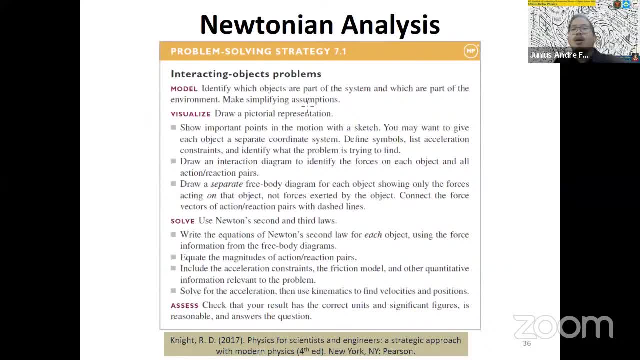 Tingnan nyo lang visually yung box na to Kalahati po ay sa ano pa lang, hindi pa yung pagsosolve ng mathematics, ng equation, ng Newton's law. So kalahati ng process ay ano siya. 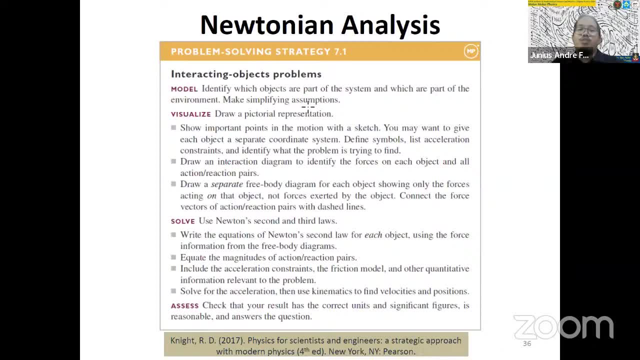 Yung proactive process. Okay, Hindi yung, kasi ang misconception na physics is mathematics, Simple math. No Physics uses the language needed, mathematics, Mathematics, as a basis or a tool for thinking. Okay, So ang first part is: mag-isip ka muna. may creative, may active process. 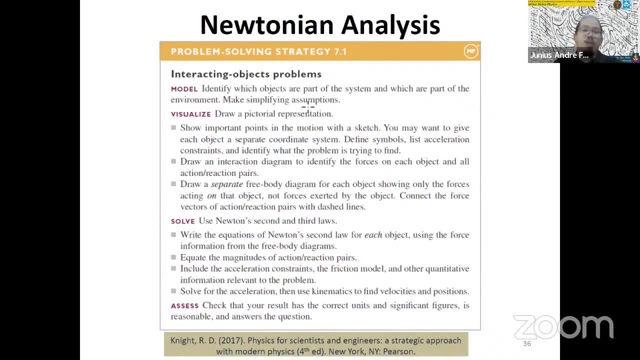 You have to model, you have to decide, you have to draw, Okay, So yun yung kalahati. So dito nyo lang makikita Yung importance ng itong action na to Yung modeling and visualizing yung drawing. 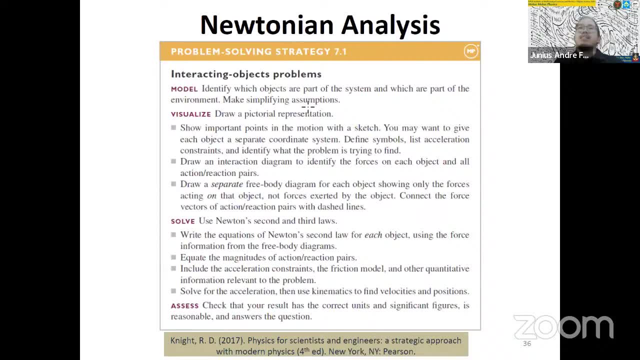 Okay, Hindi pa. So sa dulo pa yung i-describe mo na ano yung conclusion. Kasi yung sa Aristotle yan i-describe mo lang anong nangyari May dalawang objects na nag-collide. 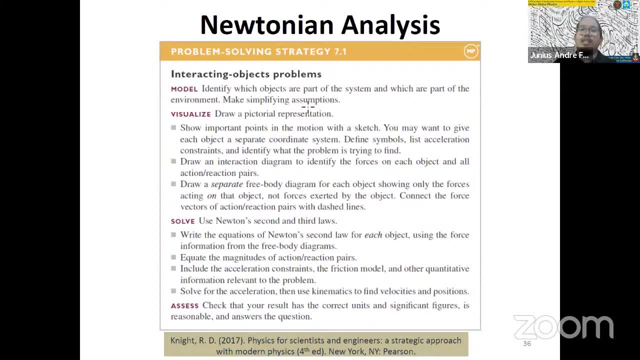 So sino ang mas malayo, yung tinapon. So dun lang, Walang modeling, Walang. hindi ka pa nagdo-drawing, Tapos i-analyze mo. Analyze when I say analyze again is take the components of the phenomenon part by part. 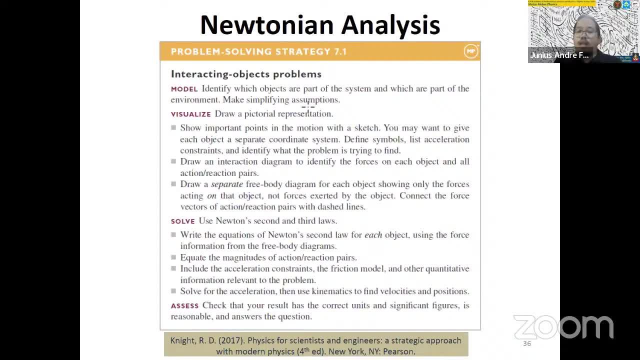 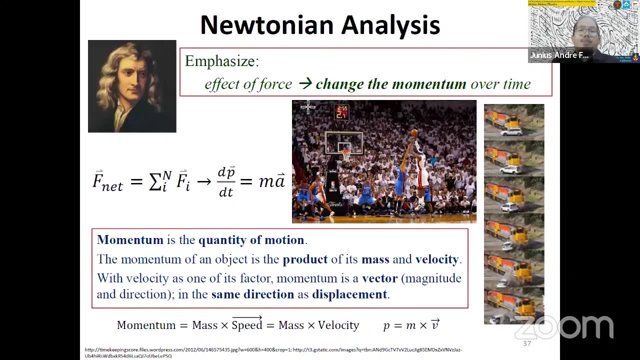 Usually Aristotelian view does not do that. Okay, Now, kasi yun nga At saka importante na i-emphasize, kasi madalas natin, when I say Newton's Laws of Motion, actually ang primary na pumapasok sa isip natin what comes to our mind first is the second law. 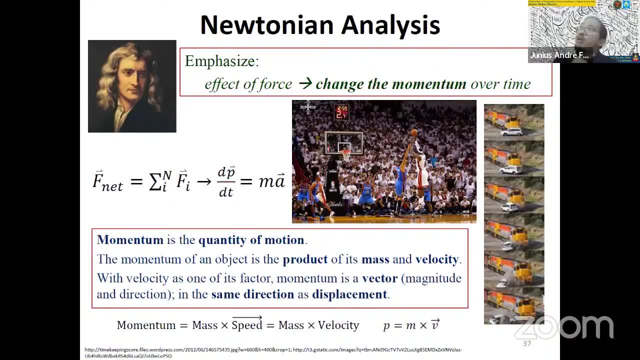 F equals m A. I would advocate: Okay, Nasana, we emphasize emphasizing momentum, Because momentum is the main quantity of motion: mass and velocity. So it's a better way to state Newton's Law. We're not changing Newton's Law. 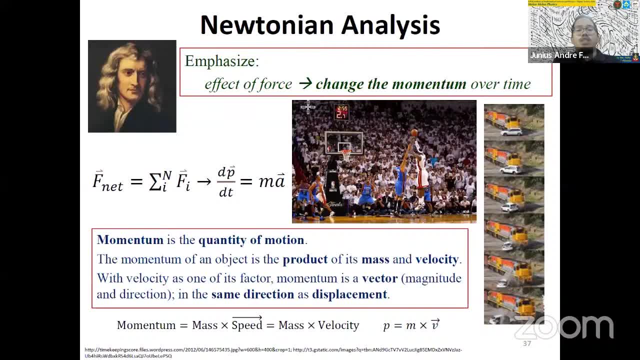 Rather yung focus natin. we're changing the focus. We're looking at Newton's Law, as force will cause the momentum of the object of interest to change Force from the external force. okay, So we identify the object of interest. 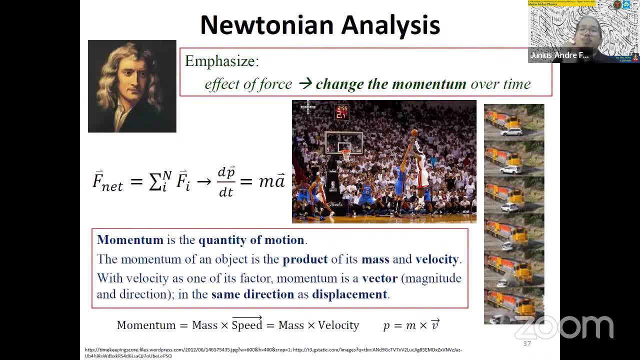 Kunwari ball. That's our object of interest. So it means that we have decided that our ball is the object of interest. By that also means that we decided not to talk about the force of the ball, Rather the force of the. 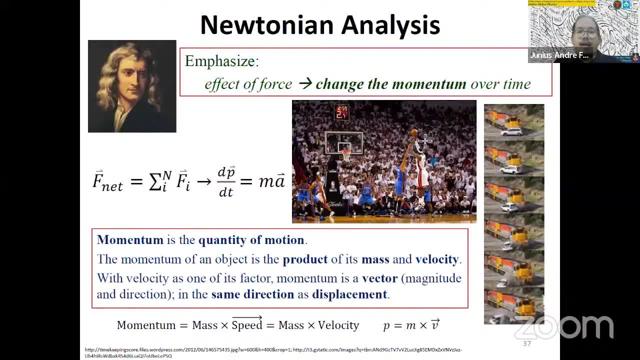 Of the external force, in this case the hand of the basketball player. okay, Yung, momentum. the momentum that we're going to talk about is the momentum of the ball. okay, Now, I think the better way to emphasize Newton's Second Law is: 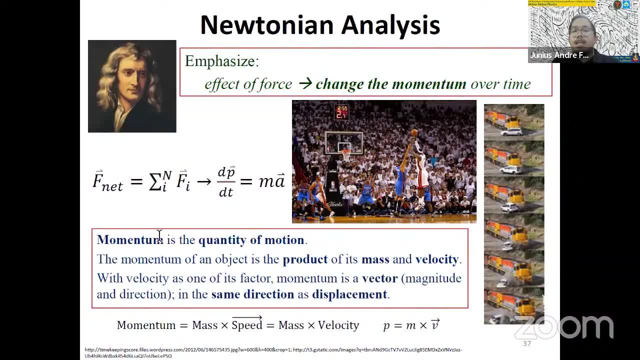 if there's a force, external force, acting on the ball, the momentum of the ball will change, okay. So, Sir Eddie, common naman acceleration, yung sinasabi. Saka natin i-i-i-i-i-i-clarify na. 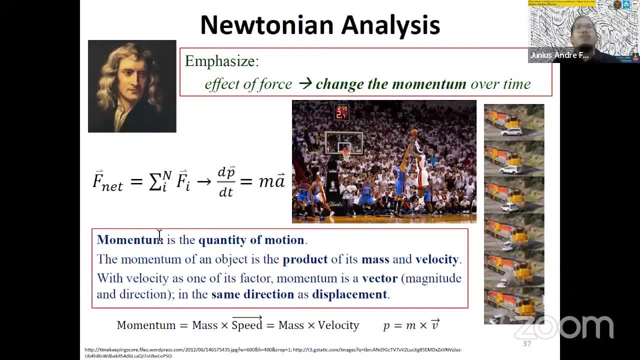 actually the momentum will change. So what are the ways that the momentum will change? Either the mass of the momentum will change, the speed of the momentum- the speed- will change, or the direction or combination of both. Usually, mass is constant. 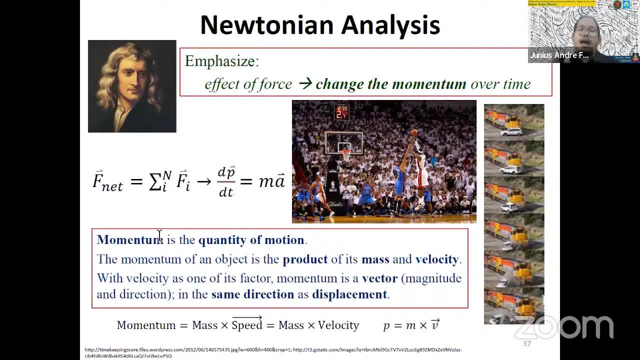 In classical physics, the mass does not change, okay, And so what changes? what changes is the velocity or the speed and and or direction of of the object. okay, so acceleration done. acceleration is the change in speed. okay, so, maganda na dumaan tayo muna sa we pass by. 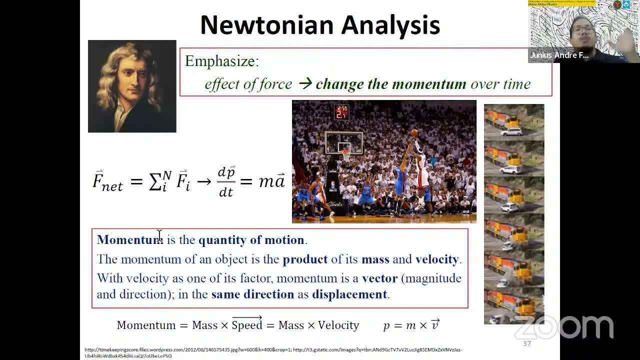 we pass through first with the, with the statement that if, if there's external force, the momentum of the object will change. what, what part of the momentum in this case? oftentimes is a velocity, the mv, so the velocity will change. so what is the change in velocity? that is, acceleration. 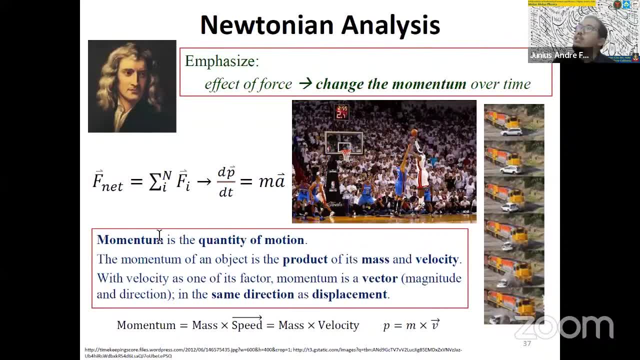 okay, so even the, even the way we state the, we're stating the same thing: f equals m, that's correct. however, if we are more nu once, we more be more systematic in phrasing or in stating the law of motion, i think we can avoid a lot of misconception. okay, so that's one of my 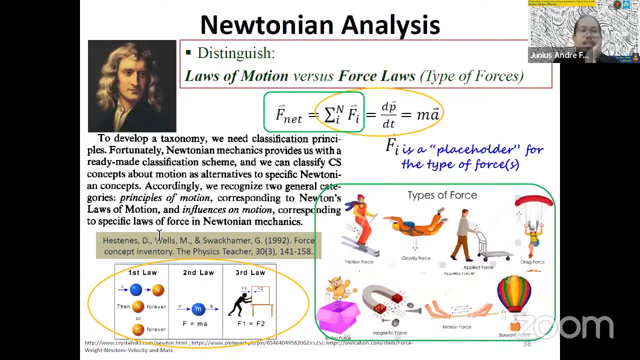 suggestion. okay, and here's an important thing. that's why uh hestanis and his and other scholars of misconception, uh emphasizes the, uh categorize the misconception into two. one is misconception in terms of of the principle of motion and the misconception about the influence of motion. so it's important to distinguish what's the law of motion and the force laws. okay, so the 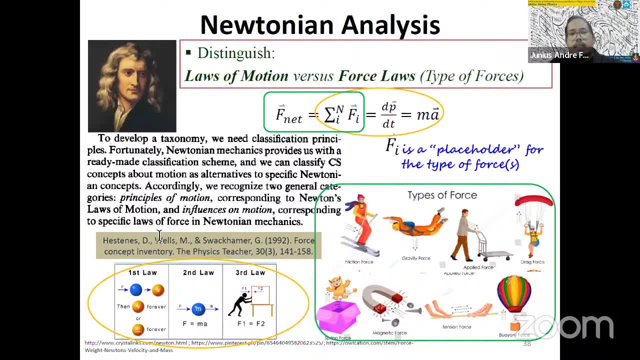 way to do this is- i think is uh, related to the previous discussion also, we have identified the object of interest, okay, and then the f there, the force. when you say force it can we still have to clarify what kind of force it is, but it's good to think of fi here. 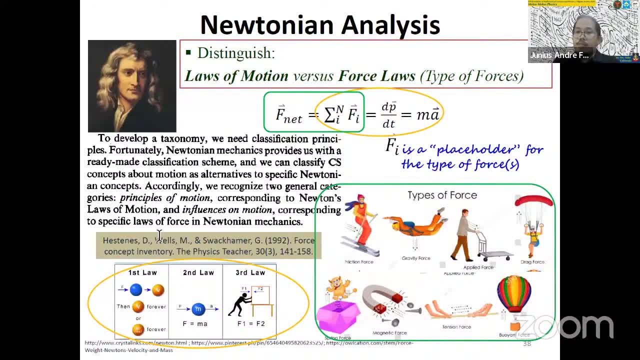 as a placeholder for the type of force. okay, so the change in the change in velocity, that's the effect. okay, so, uh, it's a bit unfortunate that we have to you. of course the equal sign is necessary of the equation, but we have to have a nuanced view of the equal sign. they're not really mean. 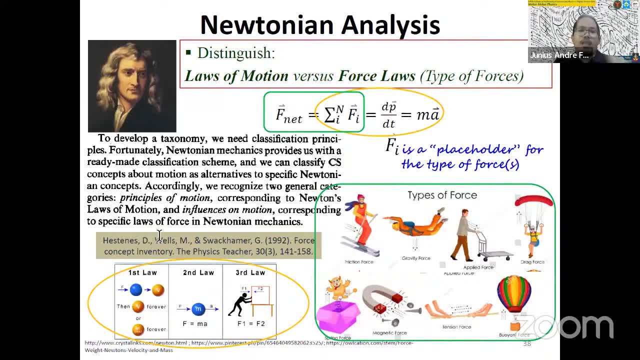 they do not mean here that they are equal, equal in the sense that they are the same thing. they're not the same because the equal sign here talks about what will be equal as in the same, but rather f will lead to ma or will lead to change in momentum with time. 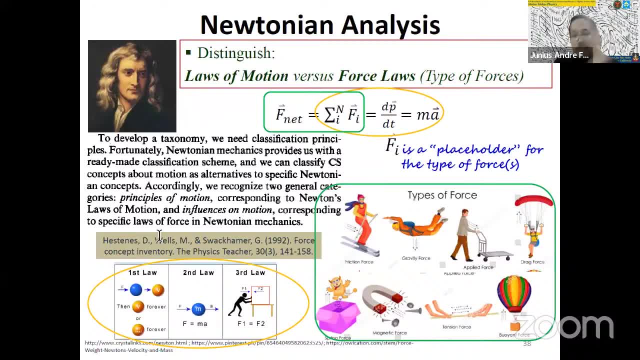 so we lead to so young f. it's a different entity. yes, where there is child, you need the, the, the, the people, you men AB. So let me just recap here When I say principles of motion, ito po yung three laws of motion. 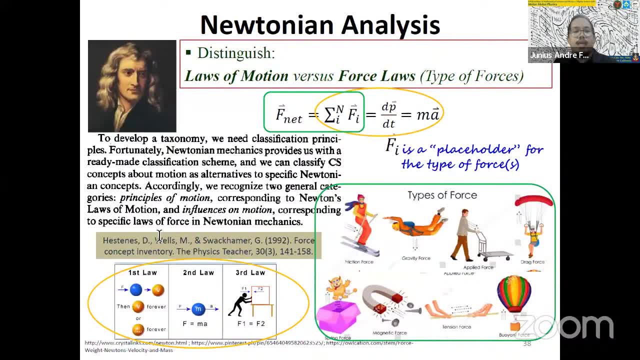 So, in general, as long as you have force, any force, it will. if it's zero, first law of motion, the momentum is the same. If there is non-zero, if the F is non-zero, the F net, the net force is non-zero, then there's a momentum change. 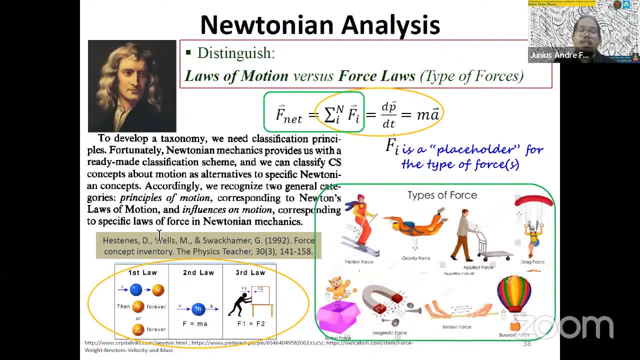 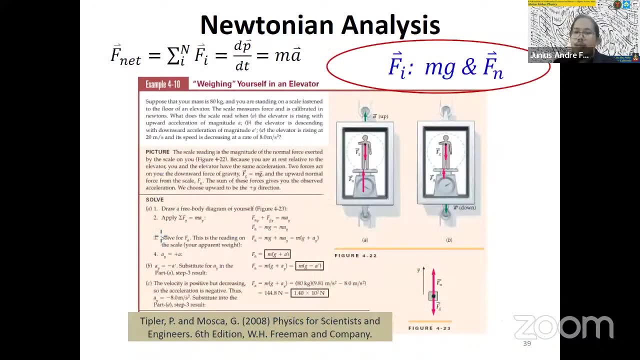 And then the forces in the interaction are equal in magnitude but opposite in direction. So this is a general principle. So yung F, the F, there is a placeholder and it depends on the type of forces. So halimbawa eto: 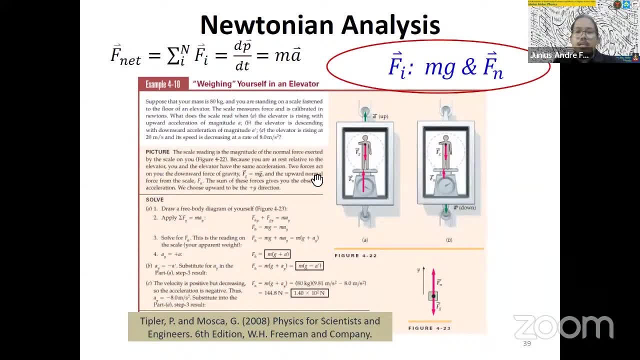 We're talking about. our object of interest here is the person. So what do we do? So we have decided that The object of interest is the person, So it means that we're going to talk about the momentum of this person. 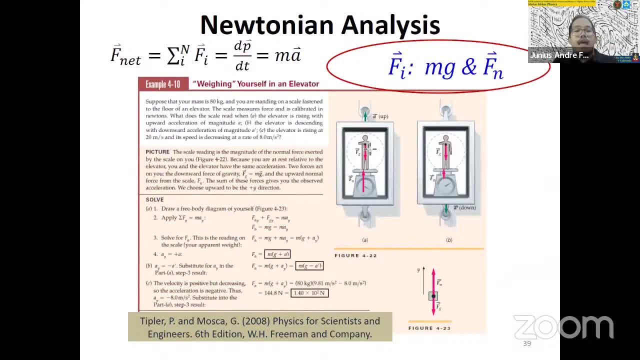 So the next thing to do is to identify what are the forces acting on it. So, the external forces. So we're not talking about the force exerted by the person, but the force exerted by the external force. Now, what are these F? 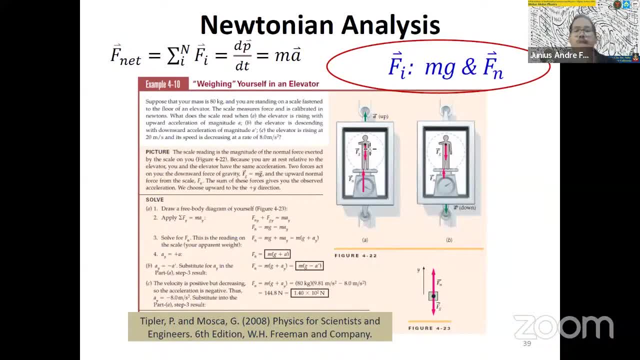 So dito napapasok po yung force laws. So in this case it's the normal force and the gravitational force. So the FI here is Mg and Fn. So now we set up the equation of motion, So applying the second law. 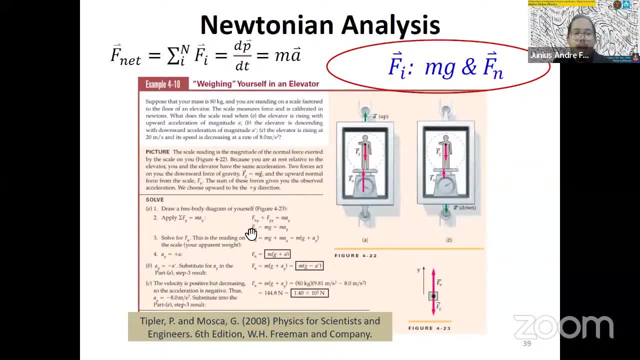 So tingnan nyo F net equals Ma pa rin. But now, this time, we put in the actual force, the detail of the force, So normal force, and then the weight or the force due to gravity. Another example, this one: 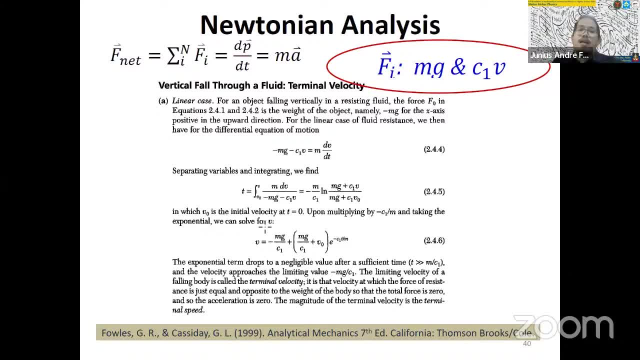 So a ball, I think, an object falling in a damp resistive fluid, So anong na-identify. Still, F? net equals change in momentum, But this time here the F. here there are two forces identified: One due to the fluid, the damping force due to the fluid where the object is immersed. 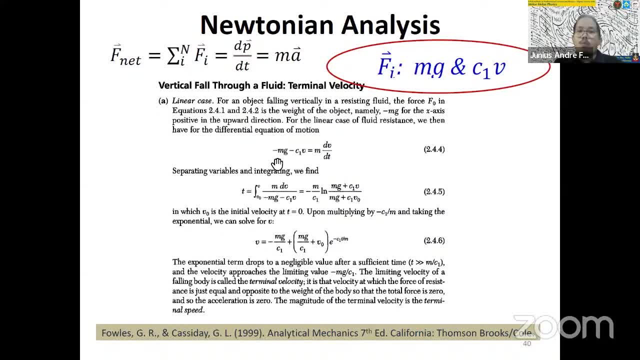 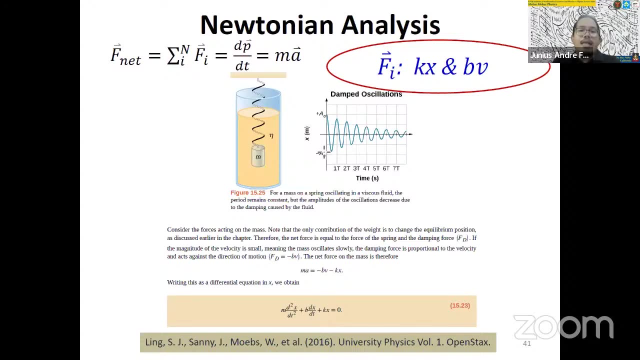 And then again the weight of the object. So dalawa po ang Ang incident, yung force that is acting on the object of interest. Last is, eto, Let's say, an oscillating mass. here, In this case we decided that the object of interest is the mass M here. 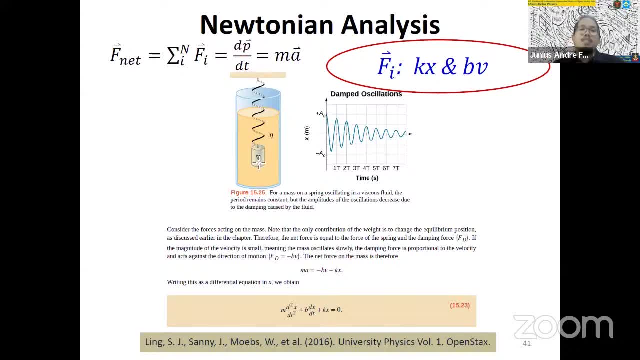 We're not talking about the spring itself, but about the mass. So what are the forces acting on the mass? So F1 on them is the spring Force of the spring, And then the other is the resistance of the fluid, the liquid, the viscous fluid. 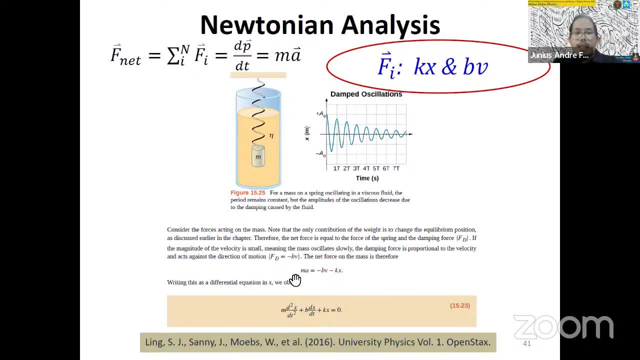 So, as you can see here, F net is the sum of the fluid damping and then the spring, And then this is your M? A. Okay, The equation may now look different. They are different, The previous one is different, et cetera. 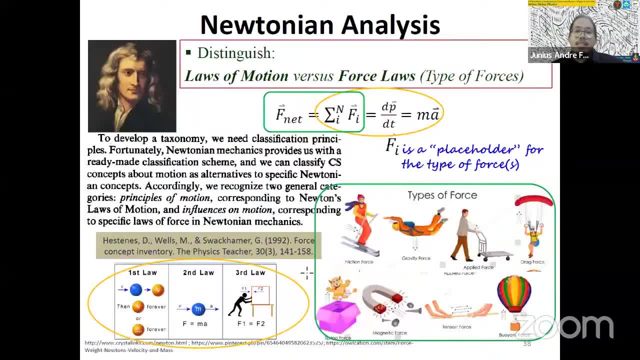 And this one. But you must recognize that this is still F. net equals M A. Okay, So the type of force will vary depending on the situation, But it is still the cost Dito siya sa side na to Cost siya ng the cost of the change in the momentum of interest. 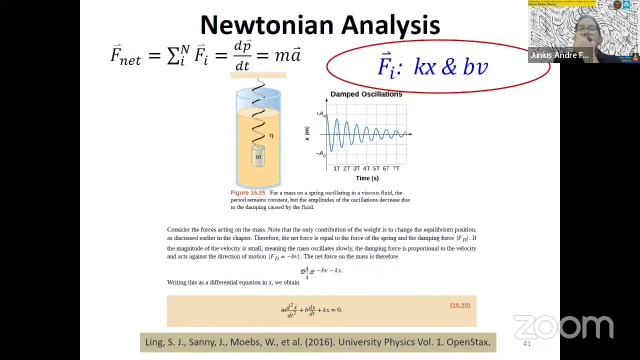 Okay, Okay. So basically, what is Okay, So important in? As you can see, what is important in dealing with misconception is the awareness of our thought process. Okay, Aware, One of the. I think one of the key way to address misconception is the awareness of our thought process. 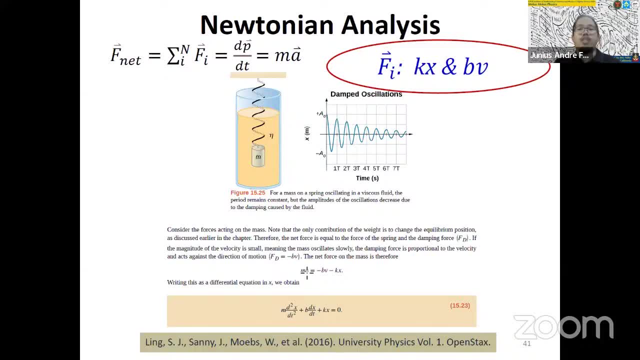 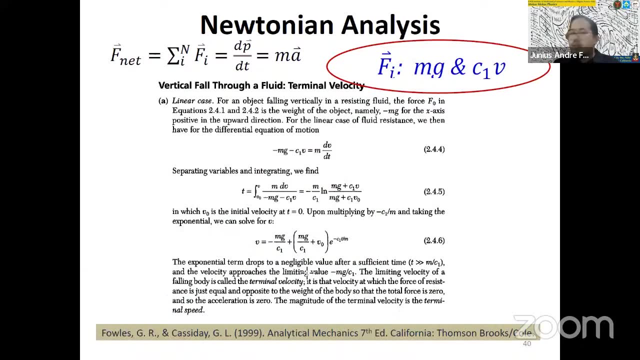 So my metacognition- I think that's the term here- is metacognition. You must think about your thinking. Okay, So this way, yung mga misconception, like in the third law of motion, action-reaction, it will. 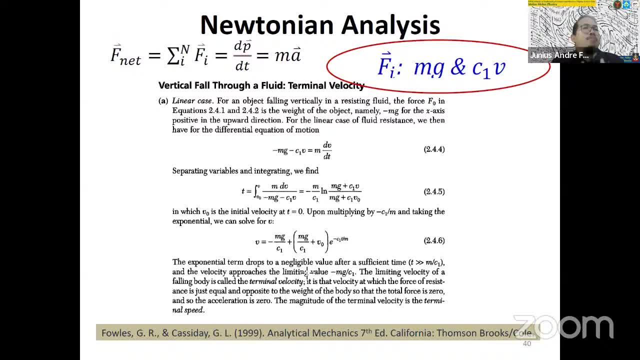 If you are conscious of your decision at the beginning, who is your object of interest? you will identify that. I think you will. The chance that you will have a misconception about the third law will already be minimized Because you're aware that there's a decision that was made at the beginning. 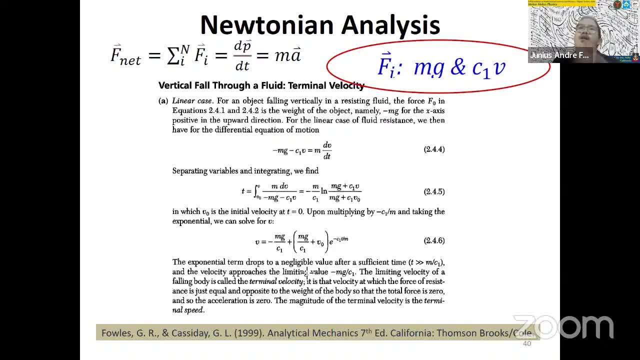 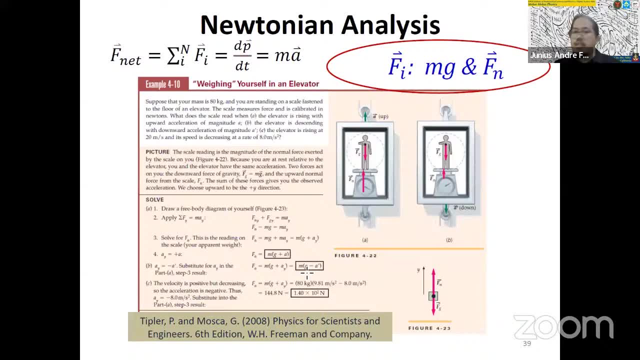 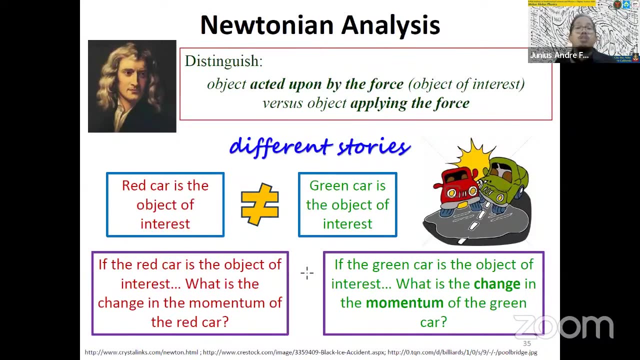 This is the object of interest. When you talk about the other object, we are aware that we have shifted. We have made a second decision, Like, for example: dito Yun Sa car na to Okay Kung mag third law ka na. you know that you're making two decisions. 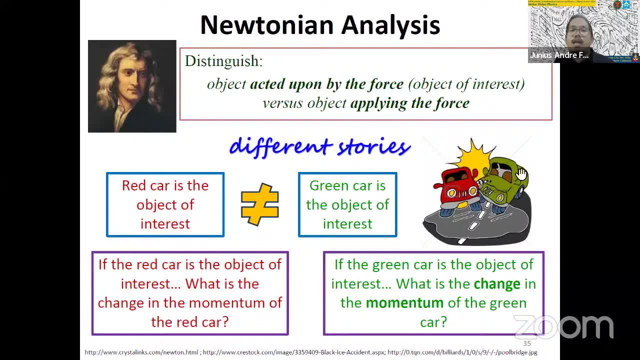 One. first, you're going to talk about the green car. So anong force in it? So that's your object of interest. When you talk about the green car, When you talk about the force on the red car, you are aware that you're making another decision. 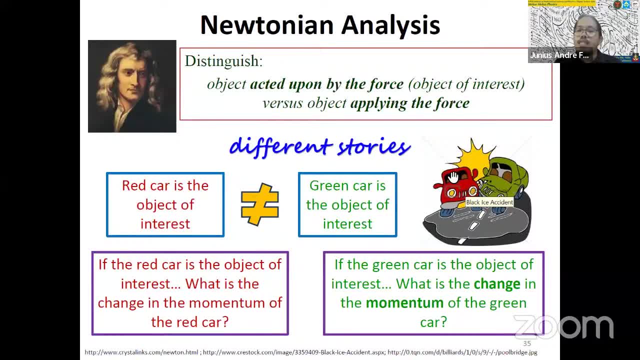 On this instant, you're deciding that your object of interest is your Is the red car. Okay, So that is important. The consciousness that you are making a decision, Okay. The consciousness that you are thinking: Okay, So yun pa. 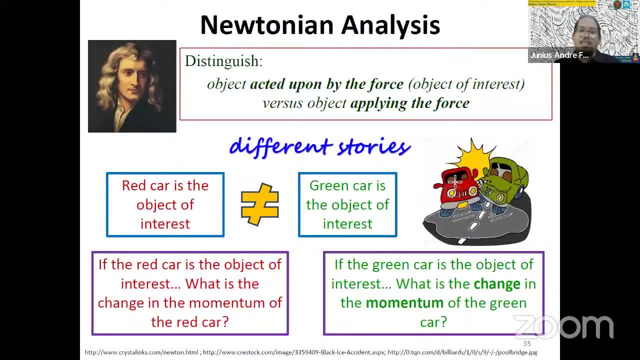 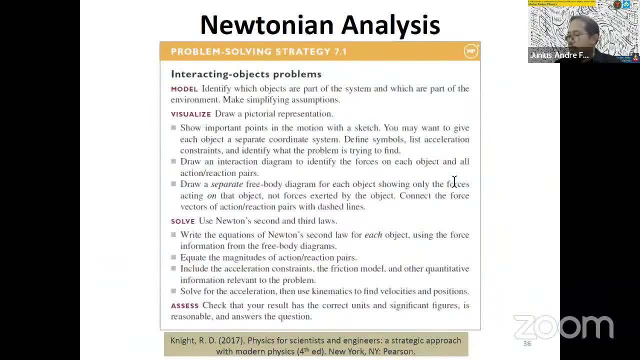 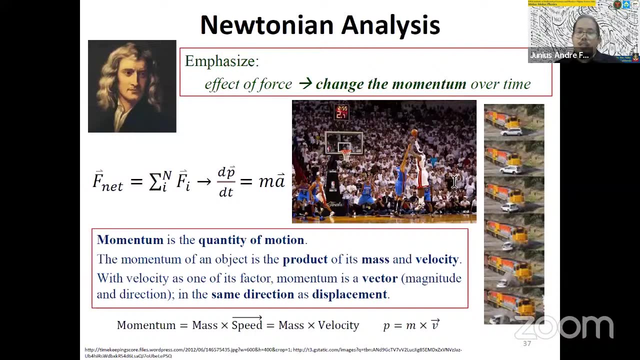 So, in Hopefully, this few tips, This- This is not so obvious about misconception- But hopefully, in this few tips that I gave you, I have given you, There's something to start or to work with. Okay, So I think this ends my discussion. 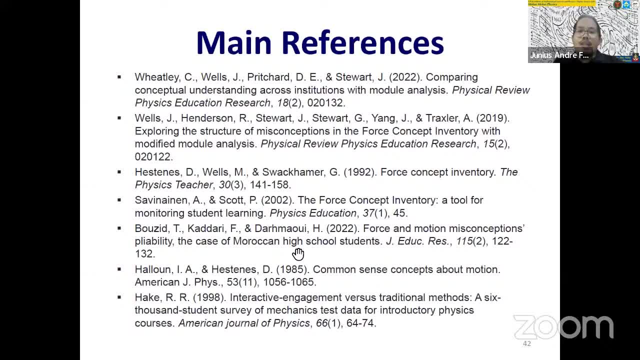 So here are my main references. Please note that Note the years of the publication: 1985. 1992.. 2022. Okay, So it's a long process And up to now we're still studying it. 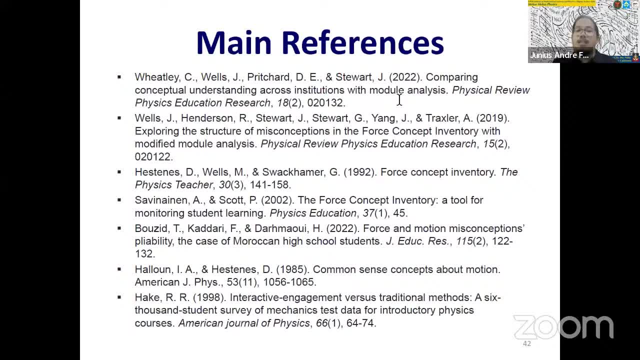 And what we've talked about is, I can say, recent development or update on this topic. Okay, So hopefully it will give you confidence and hope, Okay, Confidence that this, This, This, This effort to address misconception has a long history. 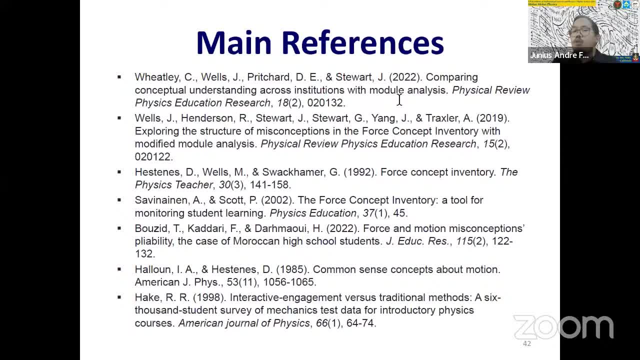 And we can trust the tools that are being offered to us, For example yung forced concept inventory. We should be happy to know na matagal na siyang inaaral, So medyo we can rely on it And we follow. 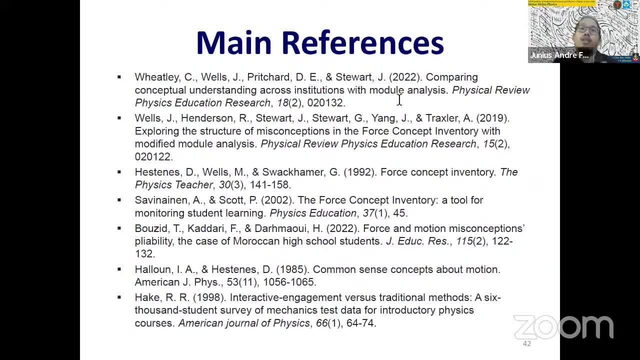 We try to follow the recommendations of the developer of the forced concept inventory, So we try to maintain its integrity And we try to use it. So, teachers, I encourage you to use it, And use it properly. Okay, And then we're in good company, because these things are fresh. 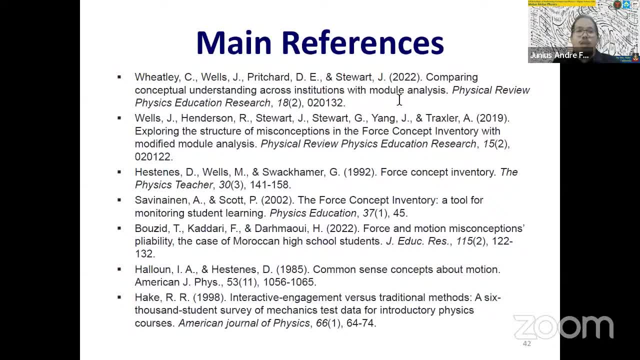 Okay, So again I would like to acknowledge this researcher. This is not my work, But my contribution perhaps here is simply to curate and to synthesize them to So that we have a conversation that lasts for about more than an hour. 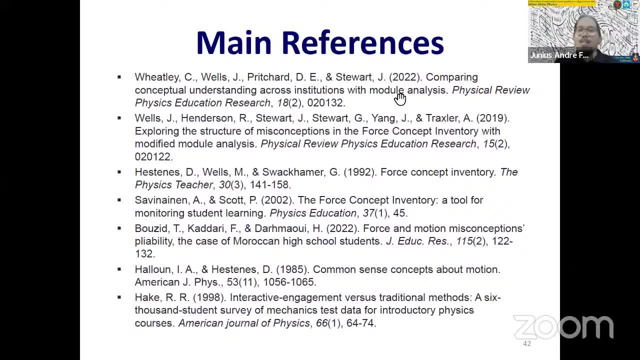 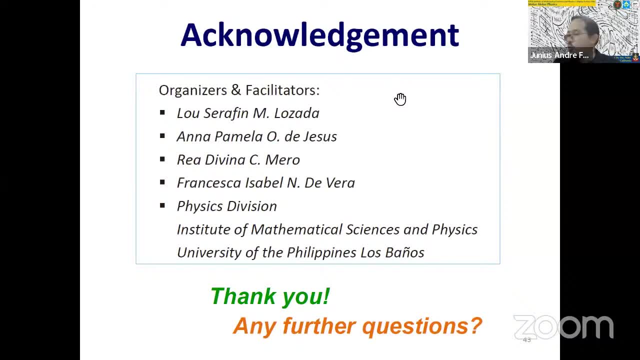 Medyo over 11 hours. Medyo over 11.40.. Okay, So thank you very much. I would like to acknowledge my assistant professor, Lucerfine Lozada, who gave some corrections on my slide, Miss assistant professor Ana Pamela De Jesus, for facilitating our discussion. 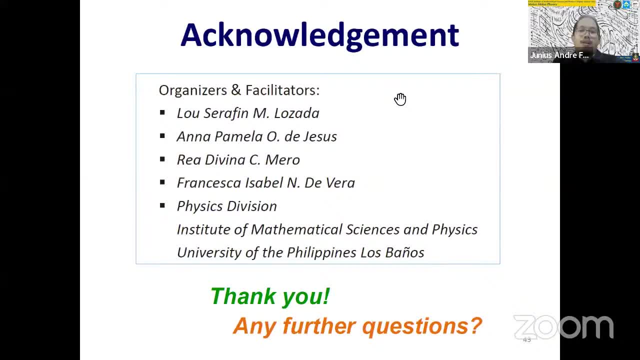 And, most importantly, to Dr Maria Mero and Dr Francesca Isabel Devera, who are the organizers and the facilitators And who invited me to be the first speaker for this lecture series, And finally, the physics division, headed by Dr Ivy Colombo. 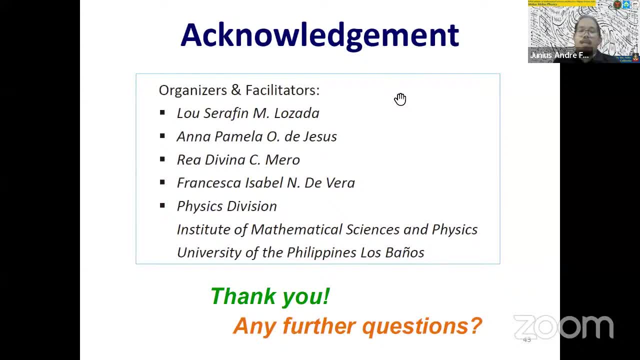 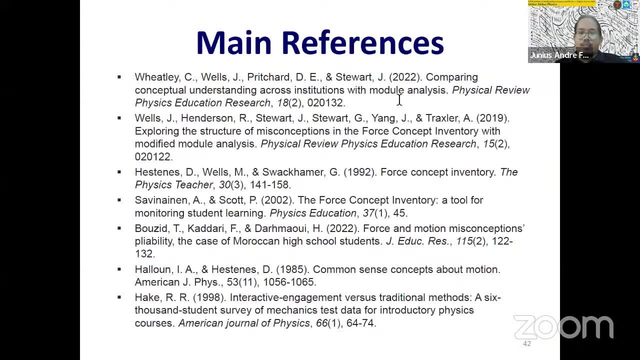 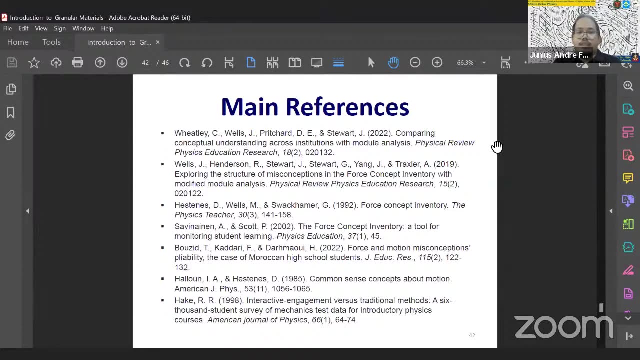 And the IMSP headed by Dr Edita C Jose. So, thank you And any further questions. Okay, Hello, Ma'am Ana. Hello sir, Welcome. All right, Thank you, sir, Yes, welcome. 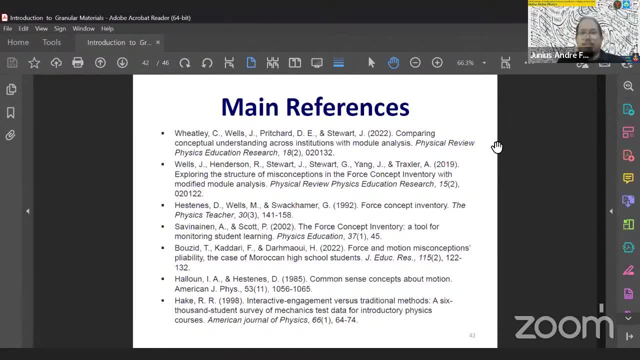 Thank you, sir Junius, for that wonderful presentation. For today we're going to have a Q&A, as Sir Lou Lozada was mentioning in the chat box, So if you have questions para sa ating mga participants, you might want to unmute your. 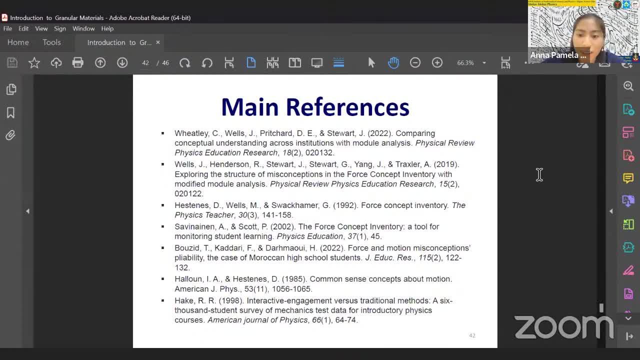 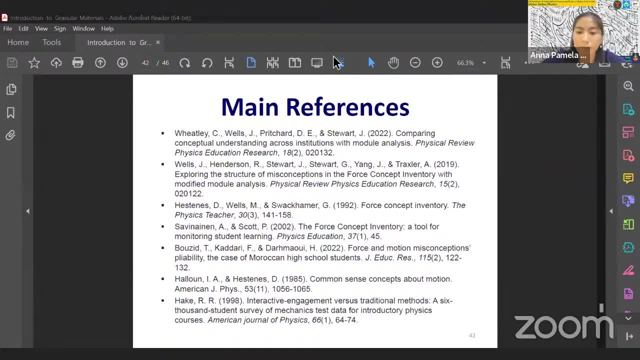 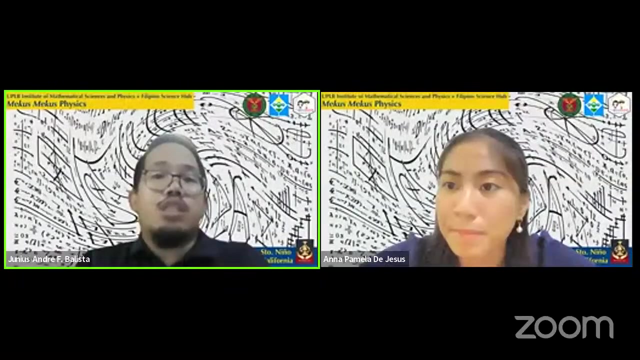 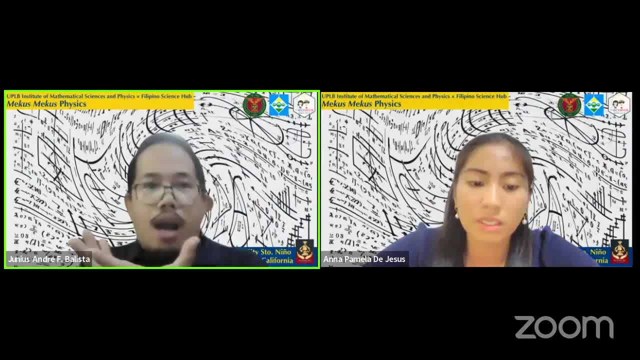 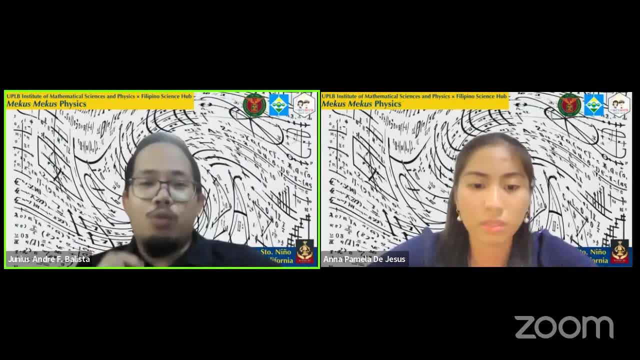 Okay, Okay, Okay, Okay, Okay, Okay. So I have to wait actually three, no, no, no, five days before I got approved, Because one is, of course, it's not available for the students. It's not available for the students. 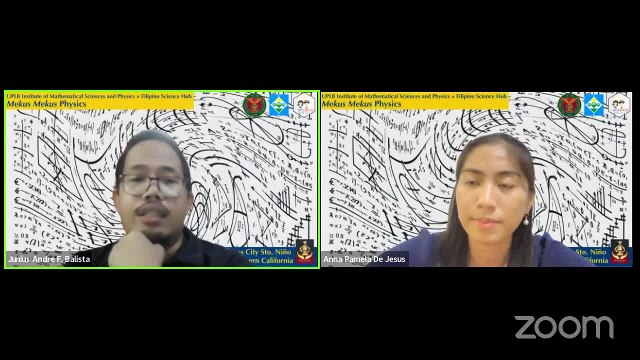 And once the teacher gets it, the developer really implores that you take care of the exam And you don't teach it. you don't use it Like this. I have to change the question And I hope- hopefully- I was able to change it properly. 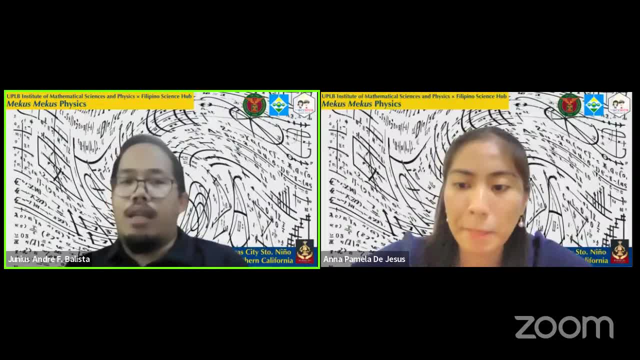 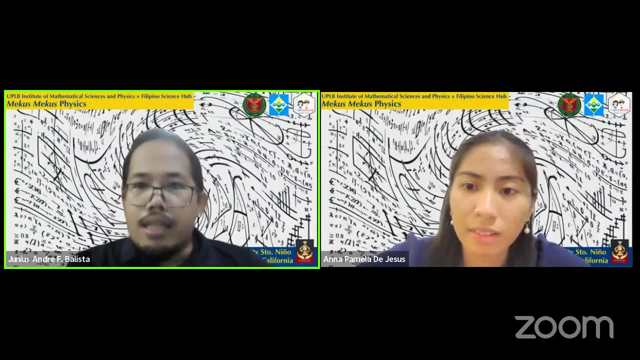 Okay, So yan Hindi siya available for everyone. It's downloadable, So yeah, But there must be access. Okay, A question pa. Okay Teko lang Hindi ko ma-ask. Another question Para si Sir Adrian. 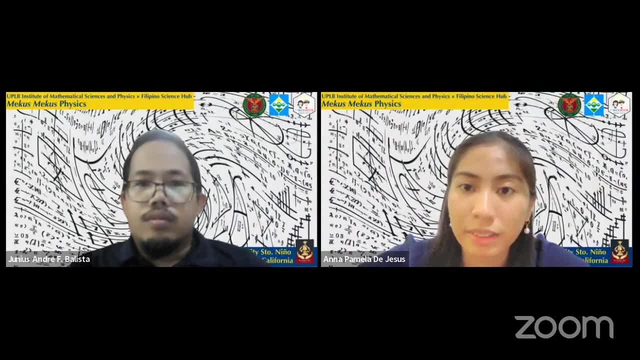 Ah Okay, Hello sir. Hello, Rinding po ba ako sir. Good morning Apo. Good morning po sir Yung. question ko po, sir is base doon sa question na pinapanser mo sa amin. 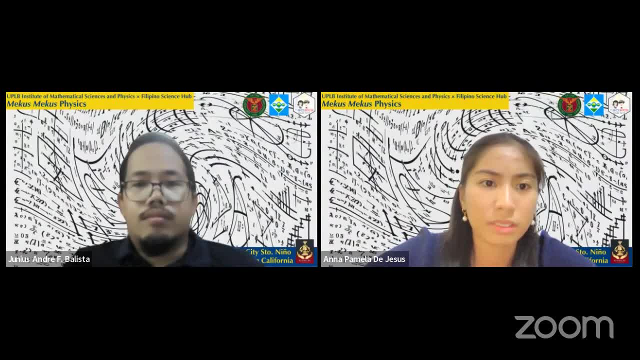 Yung tanong lang po is how to practice these types of questions, which is misconceptions, Kasi yung tinuturo lang ng physics teacher namin is how to solve certain problem, solving omni. Tapos, first time ko pa na-encounter yung ganun na mga questions sa physics. 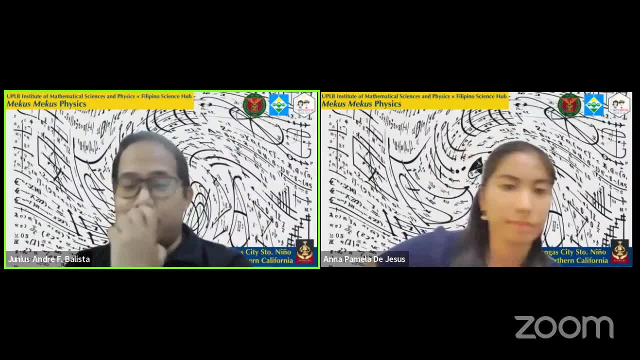 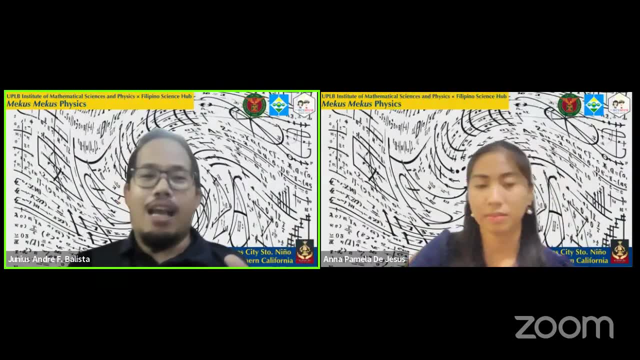 Thank you po, sir. Actually, una clarify ko lang ulit. Dapat hindi po ipapractice saan yung question na yun. So ibig sabihin umaga yun nga. Let's say, yung teacher may access na siya sa question, huwag niyang ibigay as one of the. 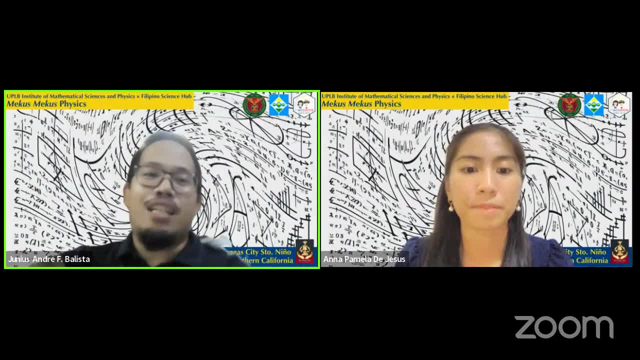 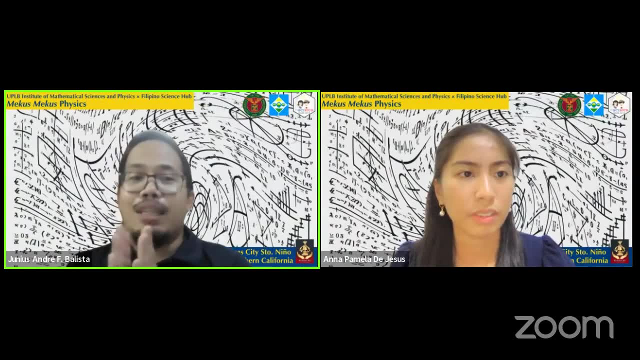 items in the exam. Okay, At saka, huwag niya rin gawin. actually ito nga medyo limited. ito na yung ano na hindi siya dapat. Pero yeah, On the other hand, yes, dapat, hindi nagja-jump. 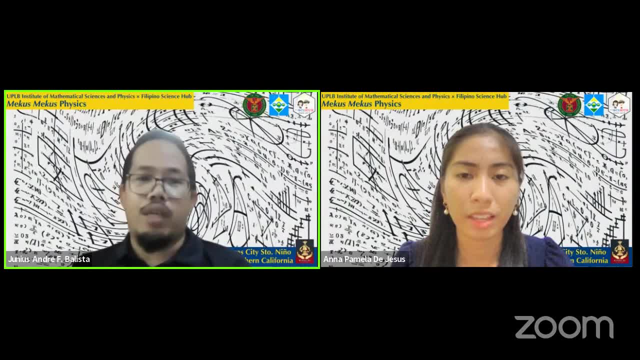 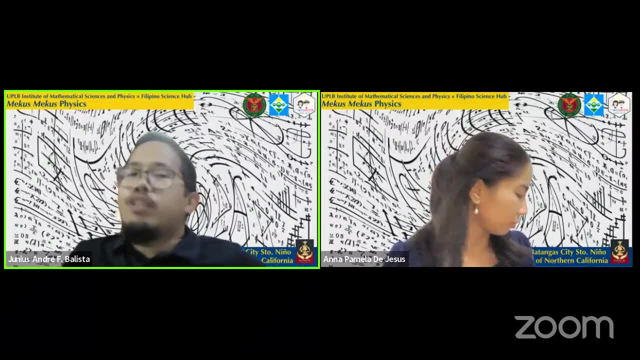 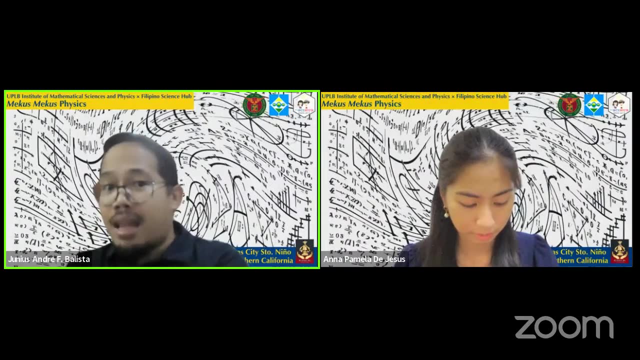 We don't jump right away to the problem solving, teaching of the problem solving. Notice, these are conceptual questions about the concept. So they really advocated that you give time to discuss the concept, Kasi madalas nga yung misconception is math, physics is math. 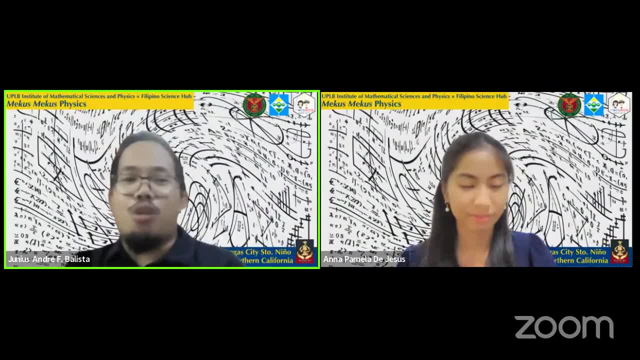 So kasi ang nakita mo doon nagsusolve ng differential equation, nagsusolve ng vectors, These are. So, kahit hindi pa naintindihan, ang physics ay nagsusolve na ng problem. 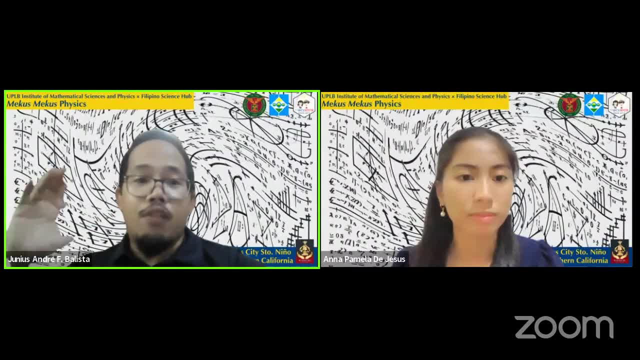 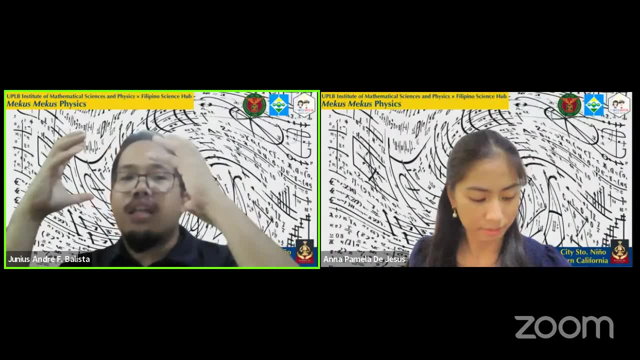 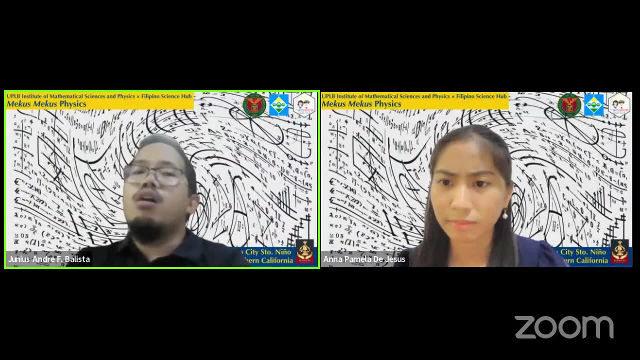 So that's the problem, Dapat. we must understand that physics is a story, Okay, And there's a creative process there. Yun nga, there's an active thinking. Yun nga dapat mag-decide ka Hindi siya novel na. okay, I'm just watching the objects collide and I describe them. 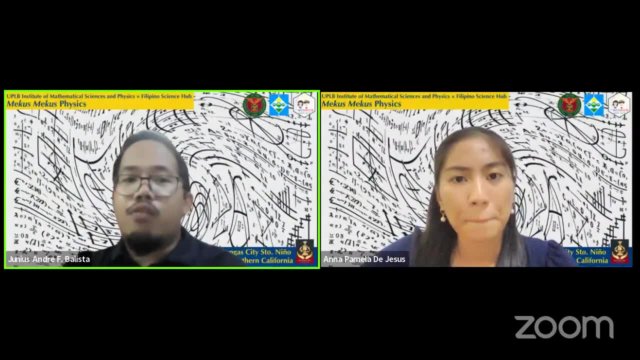 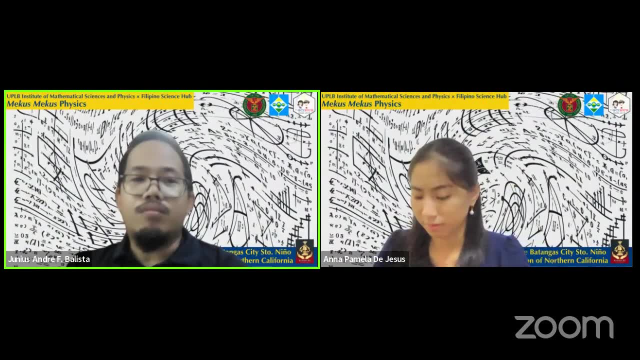 No, There are The mathematics. you have to identify, you have to analyze. When you say analyze, take apart the components. So ang environment iba ang environment sa object of interest. Okay, So that's not yet the mathematics. 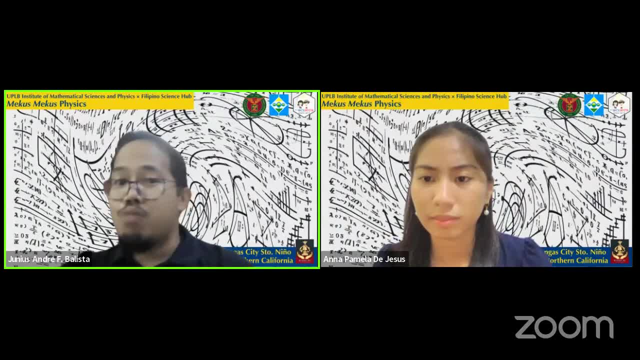 Wala pang math doon. eh, Nag-decide ka palang kung sino yung object of interest. Okay, Tapos you decide na iba pala. When you choose the object of interest, you're basically telling: I will not talk about. 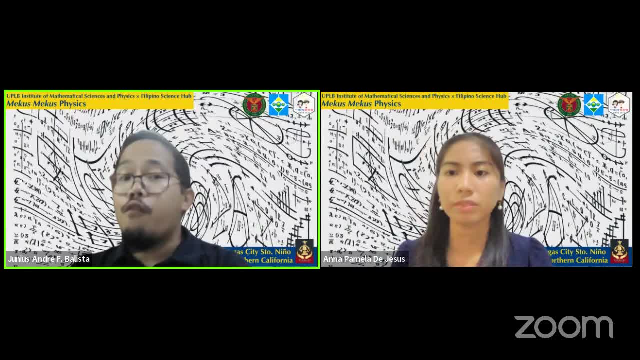 In this equation, in this part. here I will not be talking about the force of the object of interest, Right, Hindi natin pinag-usapan ang force na in-exert ng object Kaya sa sariling niya Diba. 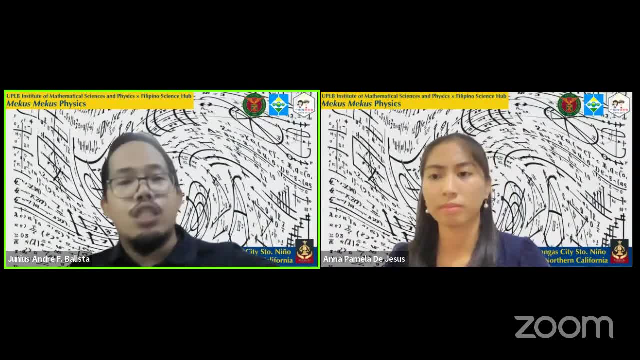 Object of interest. Nag-decide ka na: ah, yung force due to the external force, So that's a decision, Hindi, So wala pang math doon. You're not solving a math problem yet, So story. 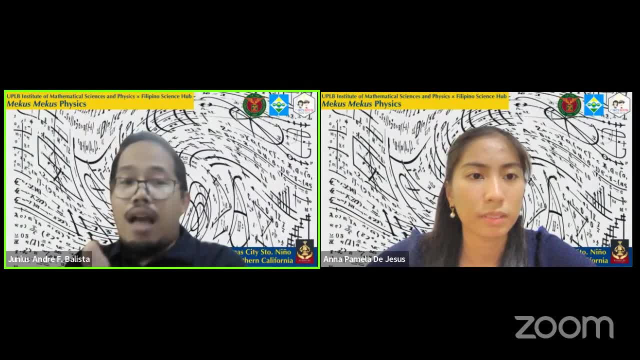 Kaya nga, ano din Like ako, even in my teaching sa aking majors, kalahati or one-third ng exam ko ay essay. I want students to tell a story, Kasi kung problem-solving lang ang wrong impression is. 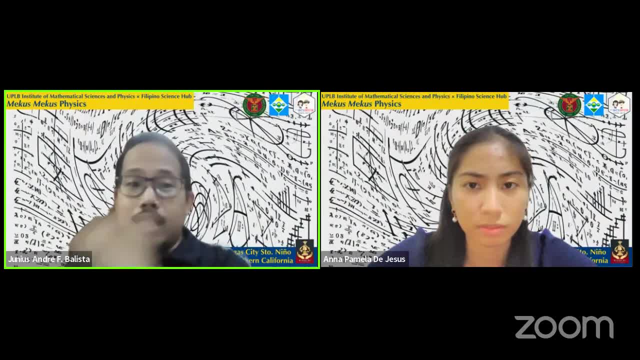 nagsosolve ka lang ng differential equation, which is correct When you solve once na-set up mo na equation, that's simply solving the differential equation, or the arithmetic, or the set of equation. That is mathematics, Mathematics, na lang Yun. 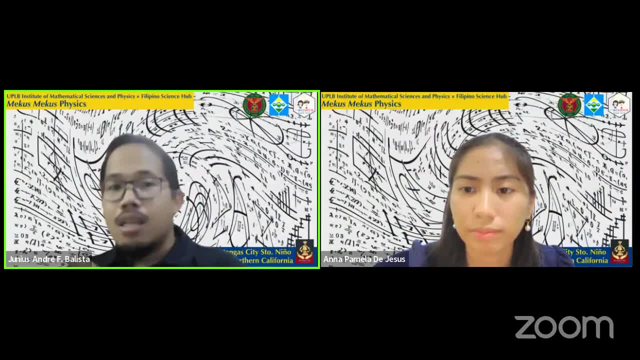 Okay, The physics part, the conceptual part is important, So dapat at least kalahati ng discussion natin, ng exam natin. ay may essay talaga Of course mahirap sagutin, Pero kaya nga, yeah, pwede gumawa ka ng parang. 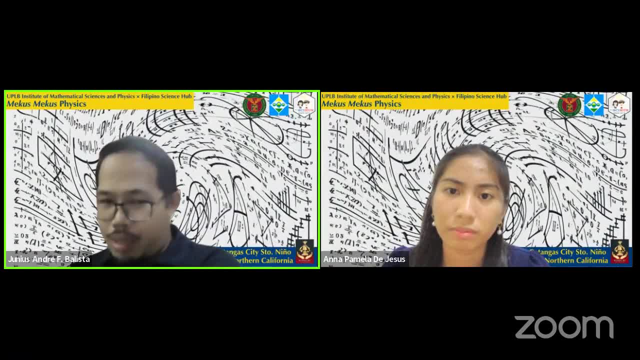 force concept inventory na style. But it takes effort, I have to admit mahirap. It takes effort from the teacher And it takes effort to convert a concept, ah an essay, A question, into a multiple choice Kasi kung essay may 40 students ka 60 students ka. 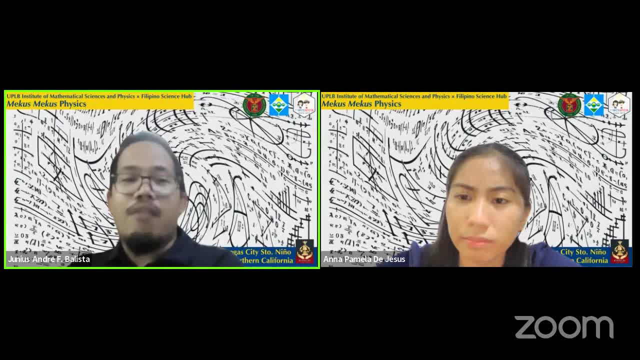 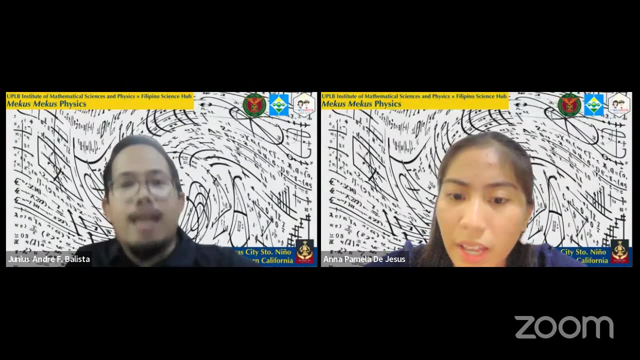 Imagine how will you check it? So mahirap, It takes effort. Kaya maganda na teamwork. kayo yung maglagturo ng physics. Okay, Other questions? Thank you, sir Ayaya. Thank you. 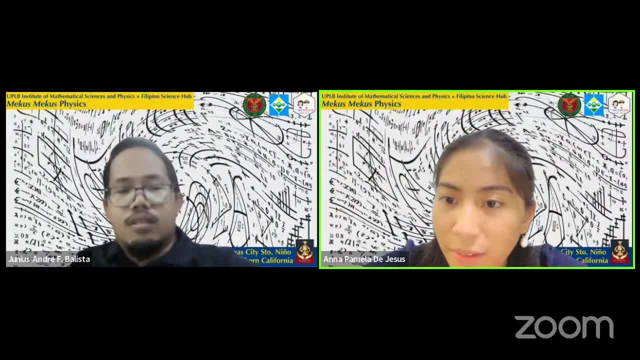 I think nandito na po sa chat box yung mga questions. Ano ho, Ito po a question from YouTube. Can you give us some tips how to encourage more students to take up course or make physics more interesting for learners? 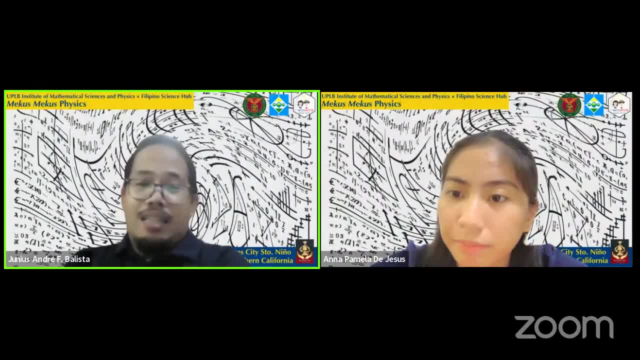 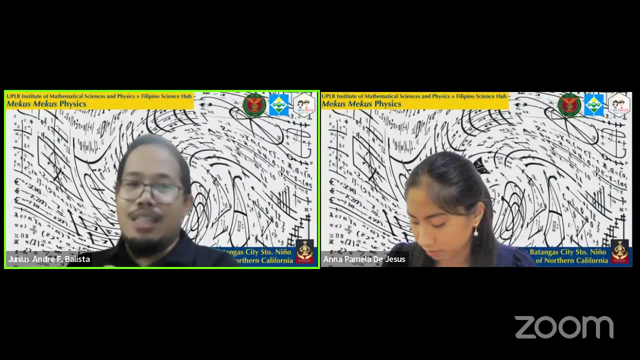 Hmm, One is una ang the ah siguro actually medyo parang age-old question yun eh Una, ang motivation to take to study the physical world is medyo self-driven. eh, You can do motivations like economics or technological. 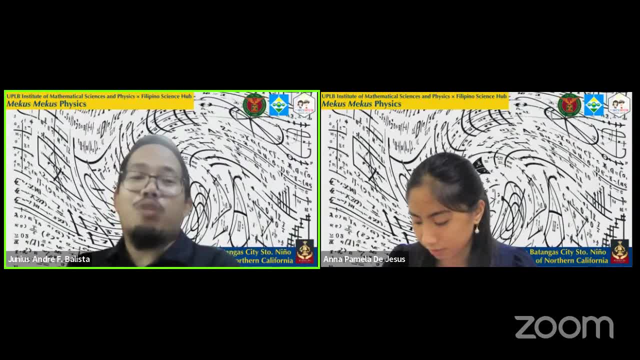 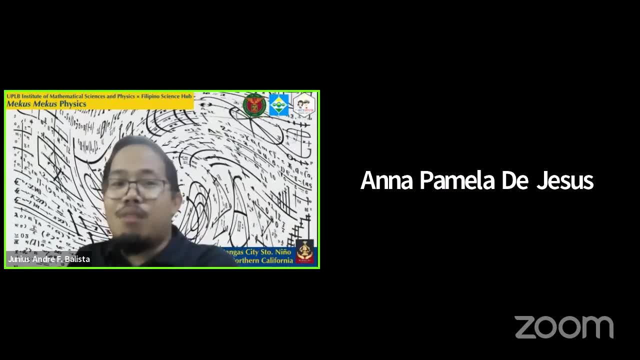 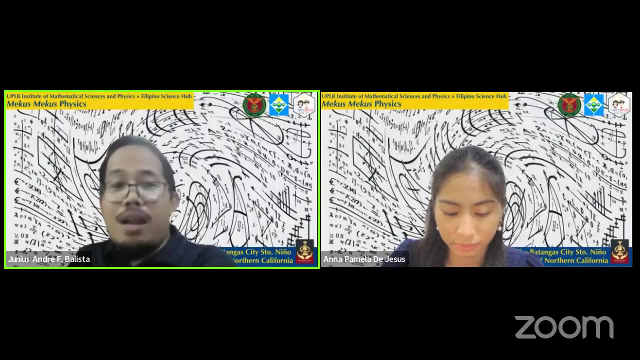 I would say the best way to invent technology, to make technology, is to get to do the physics right. You cannot send man to the moon using with misconceptions or other view worldview, Physics. so far ngayon palang tala. 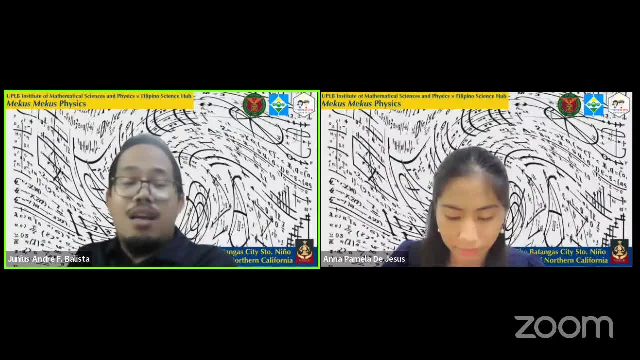 engineering, physics. yun lang po ang makakapa maka-invento ng ano. You cannot use Aristotelian view to invent. Let's say: ikaw, anong gusto mo sa buhay? Ah, gusto ko mag-invent ng flying cars. 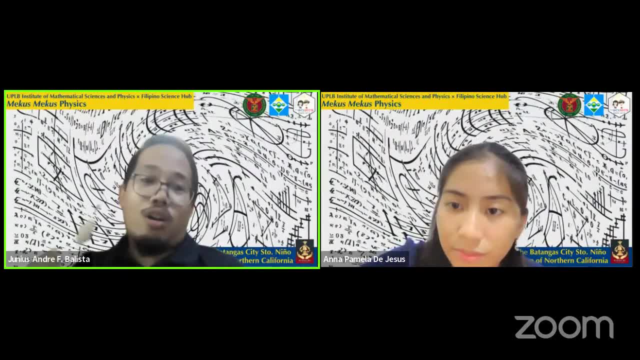 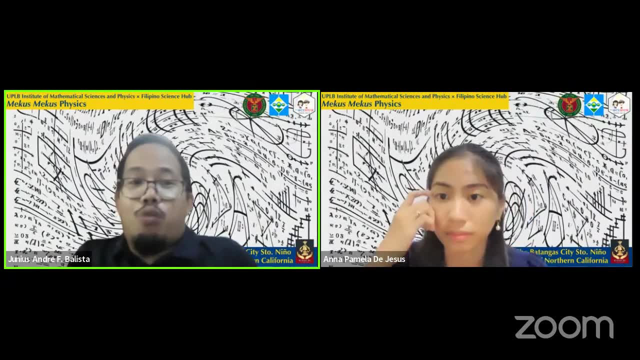 or, gusto ko, magiging astronomer, or, or, or ano ang astronoma or astronaut. okay, you have to do physics, okay. So curiosity, yeah, At saka yun fun, Siguro, yeah, like ito. 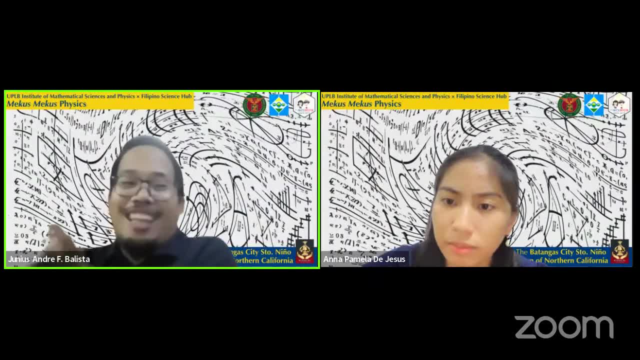 siguro one. the teacher should smile when they teach you physics. They should be happy. iba Hindi kasi ah yun nga dapat nanggaling na. physics is math, so dapat math should be fun also. 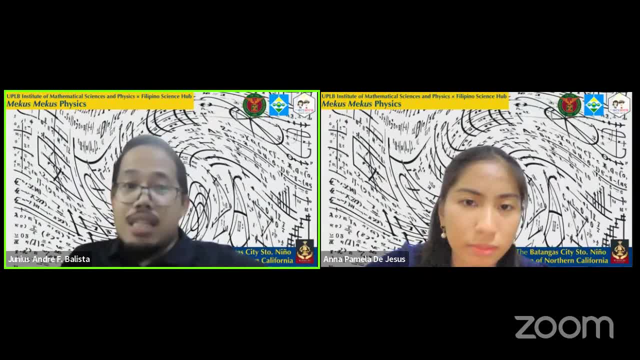 Then, so i-emphasize- dapat masaya ang math. Hindi tayo, tayong mga teacher or mga science students, na medyo gusto natin parang kailit, tayo na ay ang hirap-hirap ng physics. 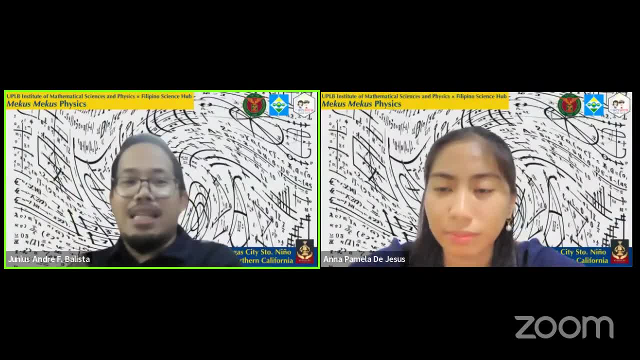 so ang galing-galing ko talaga, dahil scientist ako dapat medyo bawasan natin yung ganun, because it will turn off other things, It will turn off other students, So it's, it's hindi pabilisan. 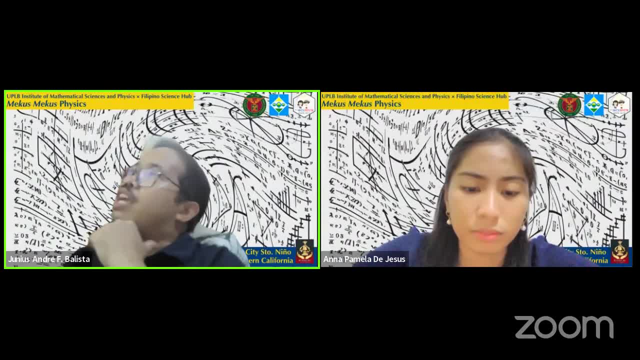 For one. yeah, ito yung, ah, ito pala. speaking of, in that sense, hindi ko gaano in-encourage yung quiz B show. Yes, it's a good way to promote science, mathematics, engineering, STEM. 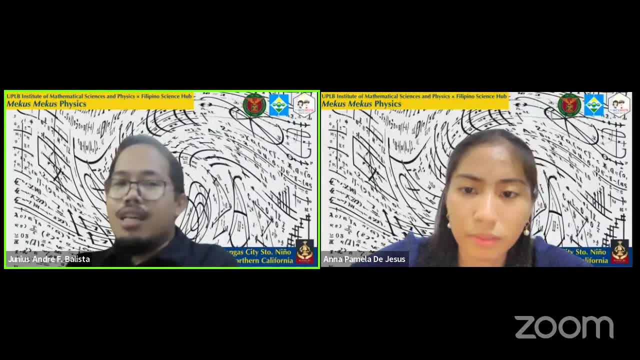 pero sometimes it has to be clarified: Hindi kailangan mabilis ka mag-buzzer or mabilis ka mag-compute to be a physicist Nagkakamabagal akong mag-solve ng problem ng mag-solve ng mathematics. 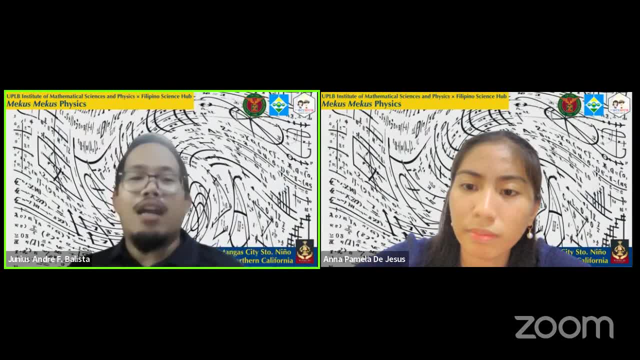 Kasi hindi naman pabilisan yan, eh, So katuwaan lang. So clarify quiz Bs as katuwaan lang, but it doesn't mean na pag natalo ka sa quiz B ay hindi ka na pwede maging scientist. 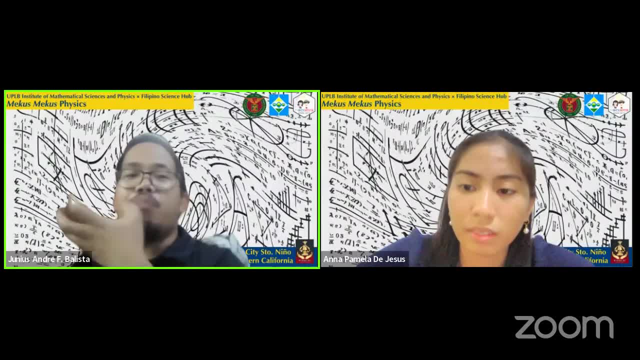 Kasi iba po ang scientist Hindi pabilisan, hindi pa-memorize na mabilisan, because scientists, when we do research, like kami dito from IMSP, we are researchers. when we solve math problem, we use calculator. 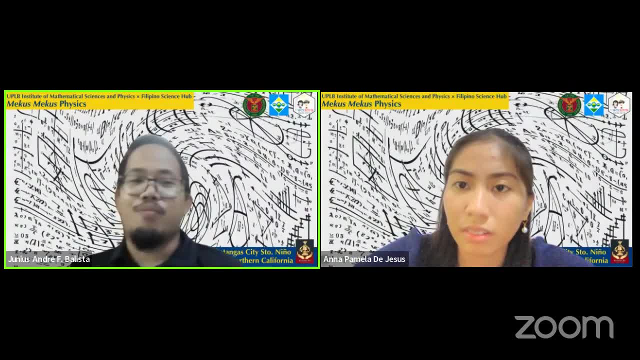 we take time to check our answers mabagal At saka. yung memory namin hindi extraordinary than the rest of the human population. I think Okay, So yun We promote quiz B shows as katuwaan. 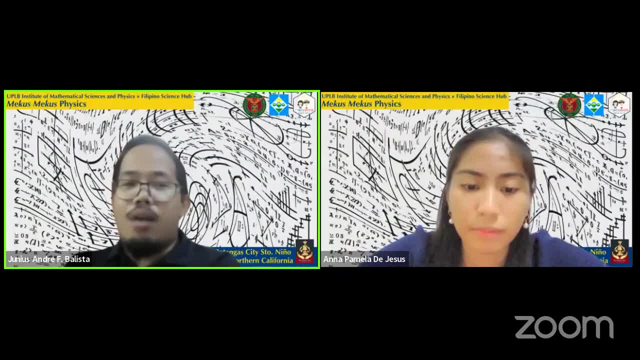 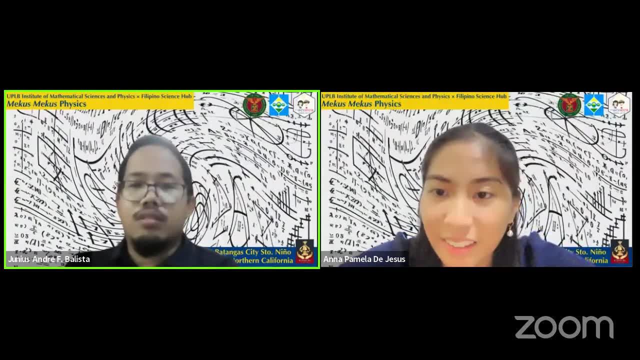 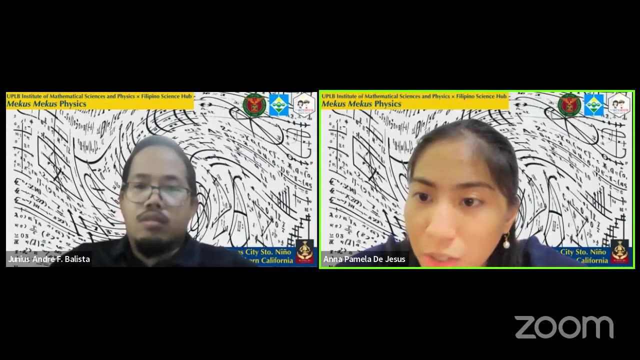 not really as a measure of kung pwede kang maging scientist or hindi. That's one, Sir. We have one question here In solving word problem: is it true that we need to check first the units and number before proceeding to the solution? 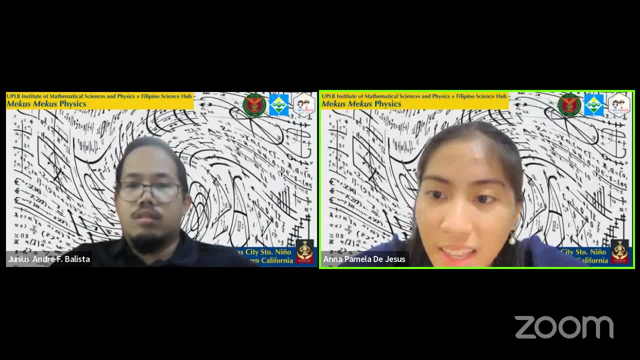 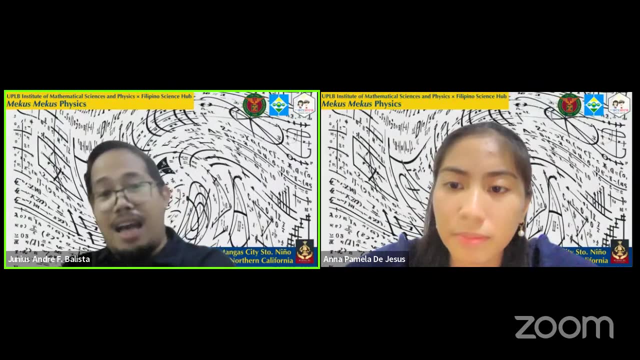 Or is it the what is asked in the problem? Can you prescribe or provide a short and effective mnemonics so that the solving process can be accurate and fast? Una syempre dapat. accurate and fast for the exam? yes, But yes. 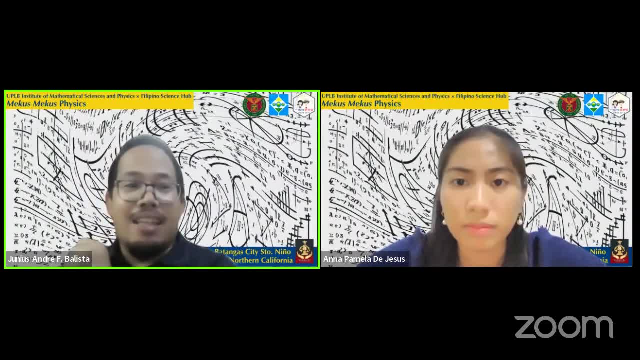 Sorry, Teka lang, Wala naman kayong na-spot na error doon sa dimensions ko. Wala pa naman yun. But it's a good advice to take note of dimensions, Kasi usually that is your first screener kung may mali sa problem mo. 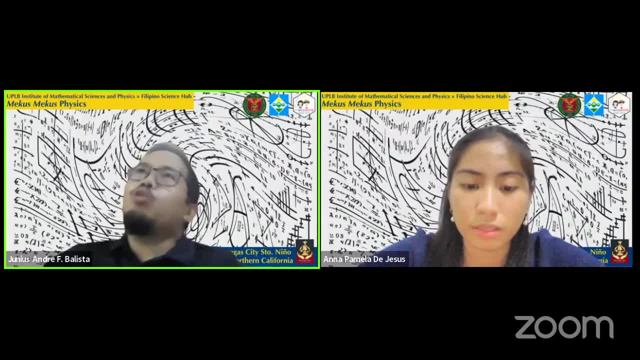 Yung dimensional analysis Kasi tinuturo sa atin, pagkita mo ng problem, tingnan mo muna medyo, i-visualize mo siya, So dapat yung mga quantities doon consistent, So yung mga units. 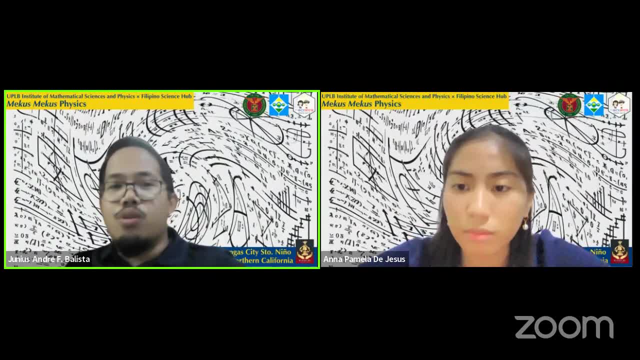 So it's a good exercise. So at the beginning, pag word problem, yes, pasahin mo muna. Tapos, kung aso ang tanong mo, kailan i-check yung dimension, Usually sa start, tingnan mo muna kung complete yung information. 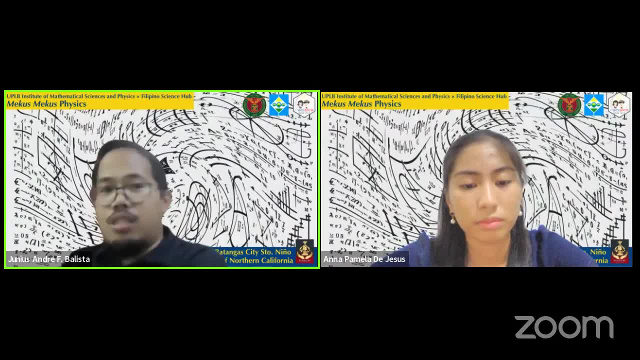 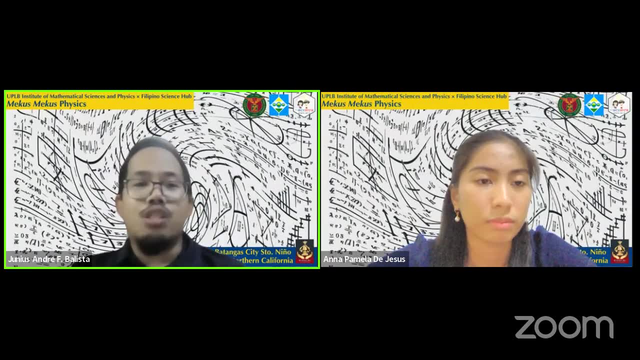 If the information is not complete, you state your assumptions, Kasi sa totoong buhay naman, yung physics problem is hindi lahat given, So you make your assumptions. Kung may assumptions ka, i-articulate mo na may assumptions ka. 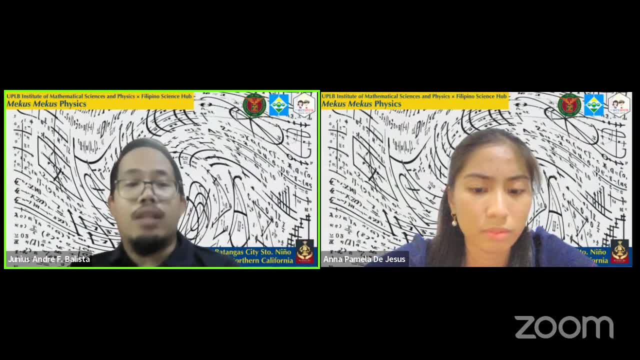 So alamin mo anong available na information, yung quantities, And you check. Siyempre careful ka sa dimension, So you check your calculation And at the end, pag solve mo ng problem, usually let's say may specific answer. 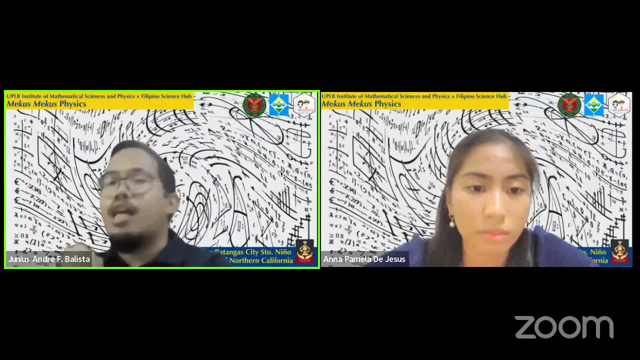 You ask yourself: does it make sense? When you say: does it make sense, Yan doon papasok Tama ba yung dimension. That's the first questions that you can ask, Dimension. Pero yun bago mag-problem solving, make sure that tama muna yung concept mo. 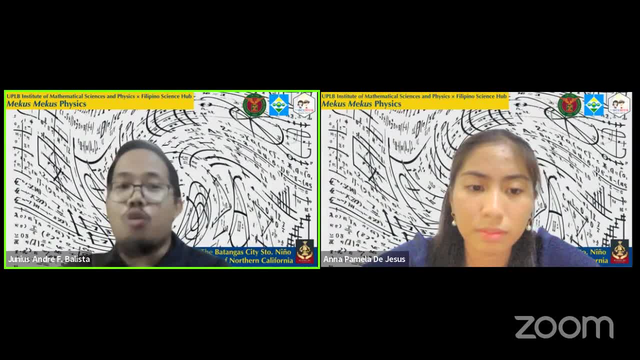 Nakaintindihan mo yung story muna. Bago ka mag-set up ng equation, Tapos pag solve mo na saka mag-check din yung dimension. I cannot really give you parang recipe, Nandiyan na yung common na recipe naman. 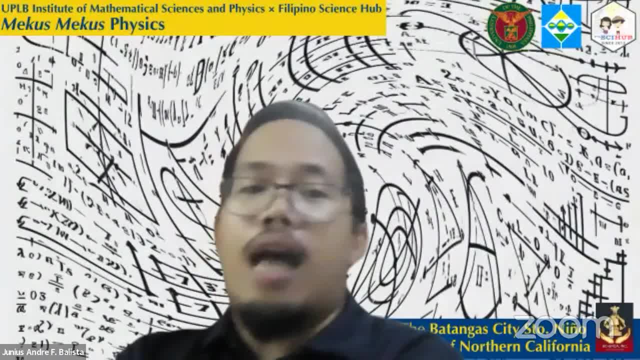 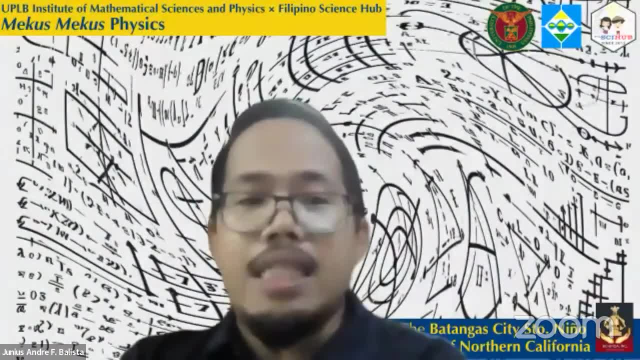 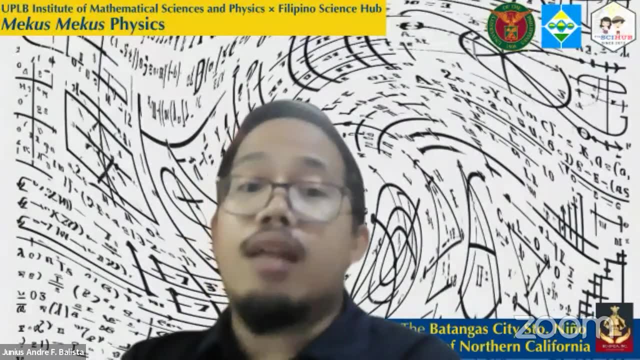 Identify the given. Draw the equation, Sorry. Draw the situation. Draw the force diagram. Yun nga Decide what is your object of interest, So that doon mo ilalagay yung i-draw mo, yung forces acting on that object of interest. 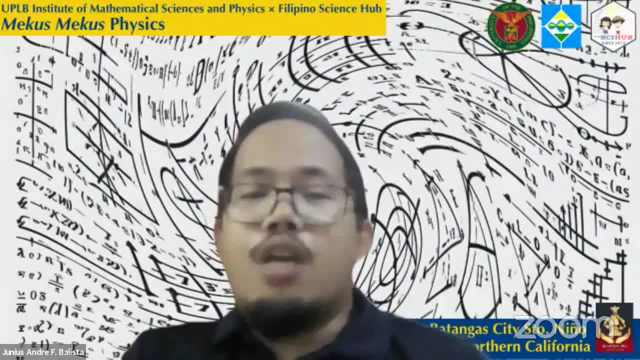 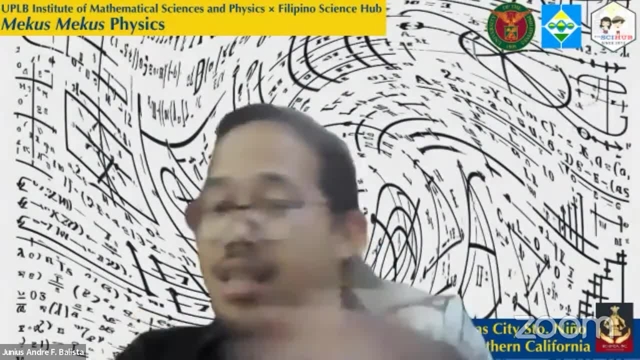 Saka set up mo yung forces And then solve Yung mathematics, kasi sa tingin ko pag na-set up mo ng equation medyo straightforward na yun. eh, At kung nahirapan ka sa math, hiwalay na problem yun. 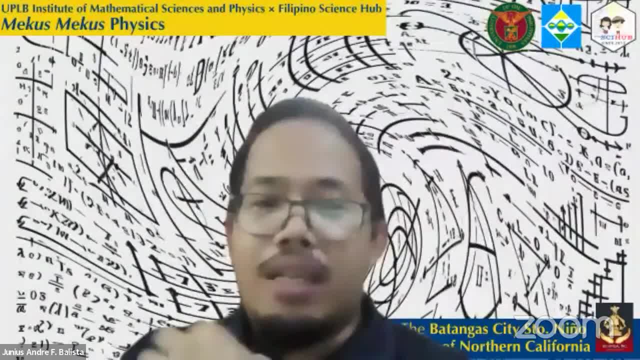 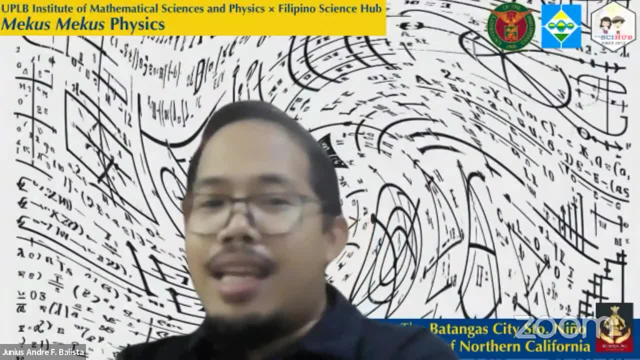 So important din yun. Minsan sinasabi ko sa studyante ko: Pag nahirapan, ano, Alin, ang problema natin? Dapat identify muna Yung physics or yung math? Hindi mo ba na-guess? 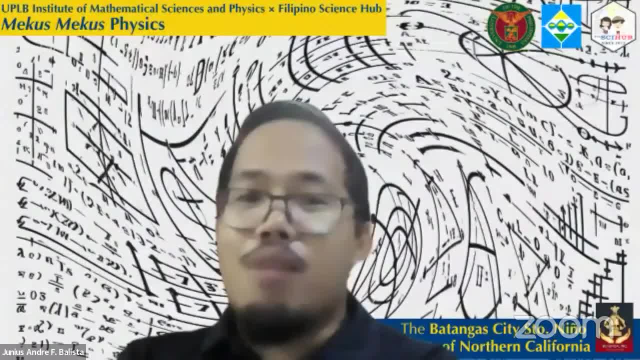 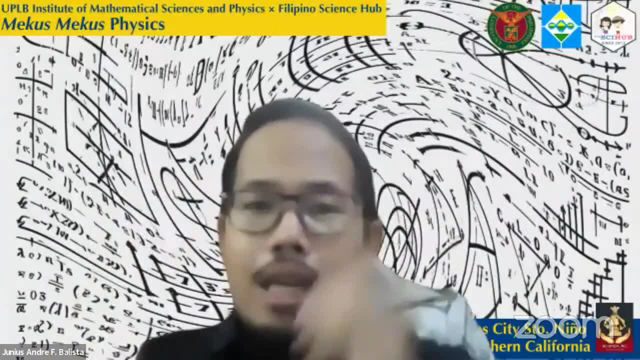 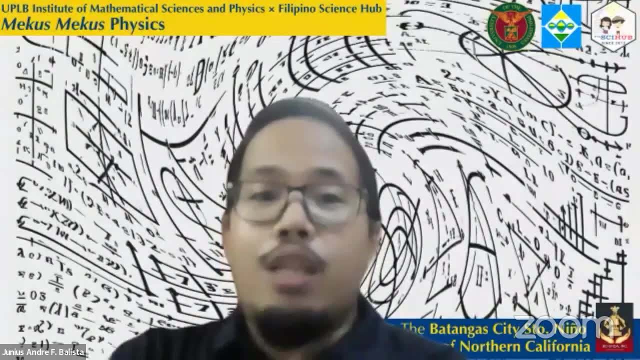 Tingnan natin Yung Newton's law ba O yung pag-solve ng pag-transpose, pag-substitute, pag-multiply. So identify natin yung problem, So and differentiate, distinguish. Iba ang physics sa pag-solve, part na yung the mechanical. 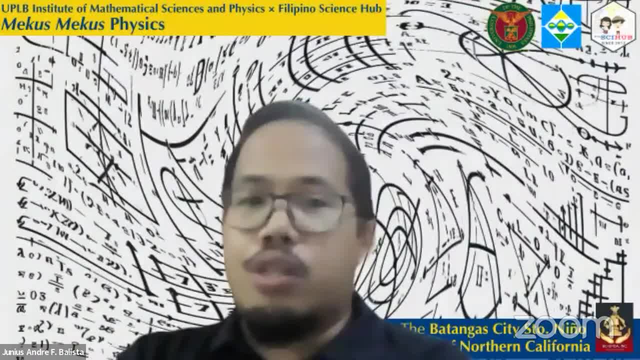 The mechanical part of solving the equations. Okay, So importante sila pareho for make sure na na-distinguish natin. Eto get the story straight: muna Bago mag-problema, kung paano mo i-solve? 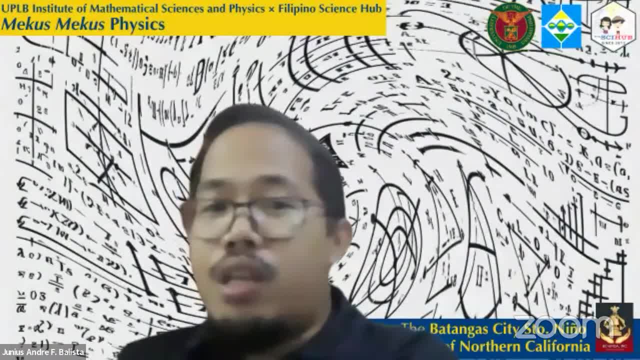 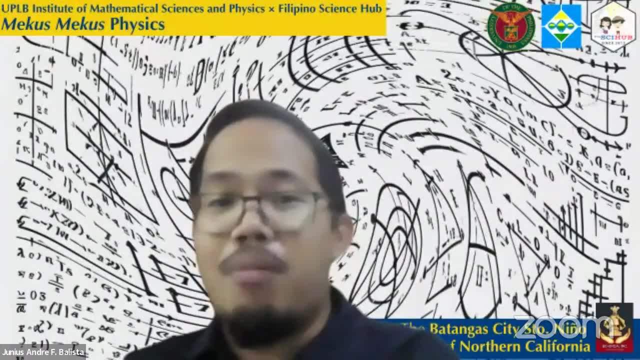 Kasi, minsan, by just simply guessing, even if you don't understand, but you substitute it right, you will get the correct numerical answer. But you still haven't solved the problem, Okay, So, yes, importante yung dimensional analysis, Importante na tama yung math mo. 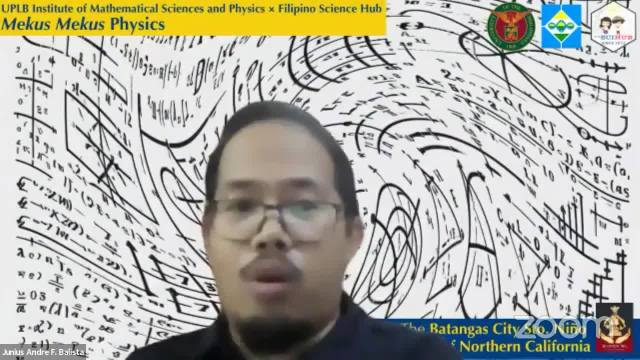 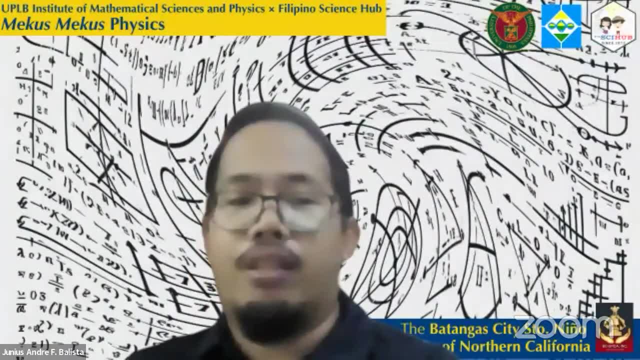 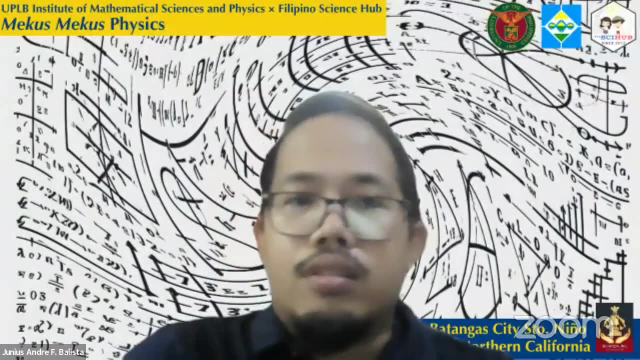 But on the physics side, importante dapat yung kwento. Claro, kung sino yung object of interest, sino yung external, Sinong pinag-usapan natin Yung basically ganun, Okay, Next questions. Hi, Sir Junius. 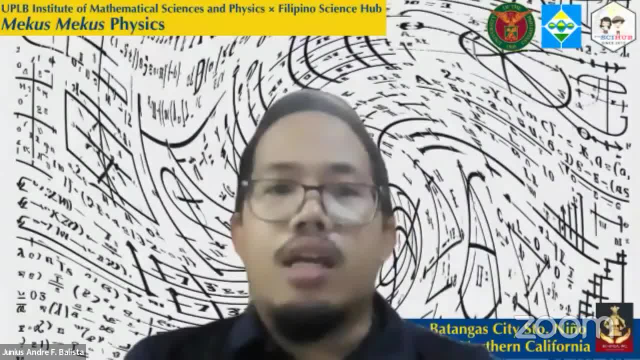 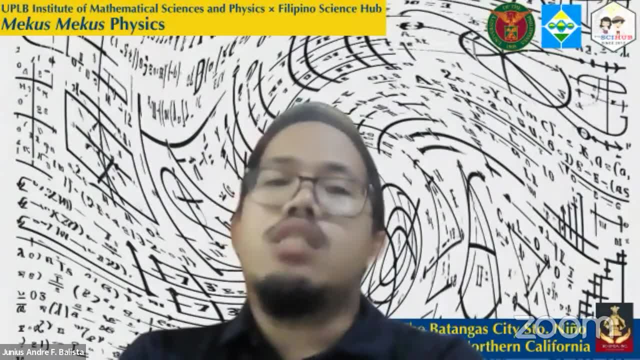 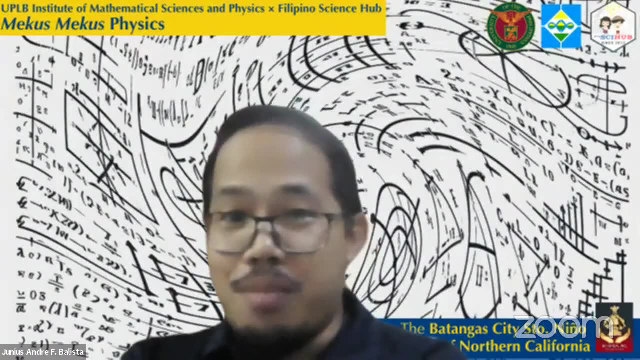 Sige po, Which lesson do you think are the most essential to teach to fee senior high school in their Gen-Phys 1 and 2,, given that their school days are shortened? Okay, I really understand, Actually, kasi isa kami sa tumulong sa paglagay ng silabus. 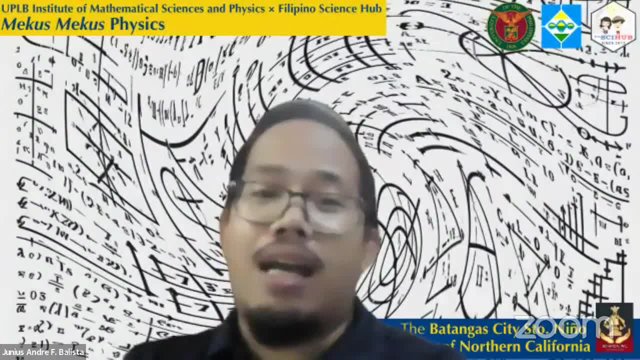 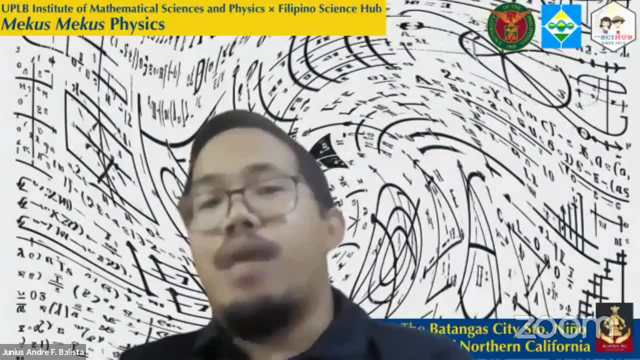 Okay, At saka pinagbabawasan yan yung mga item. Ah, hindi akong, Kung ako i-recommend siyempre yung basic. When you say basic, edi yung Newton's Laws muna, The Laws of Motion muna. 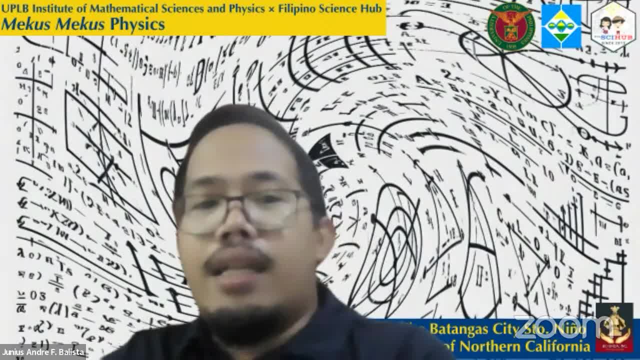 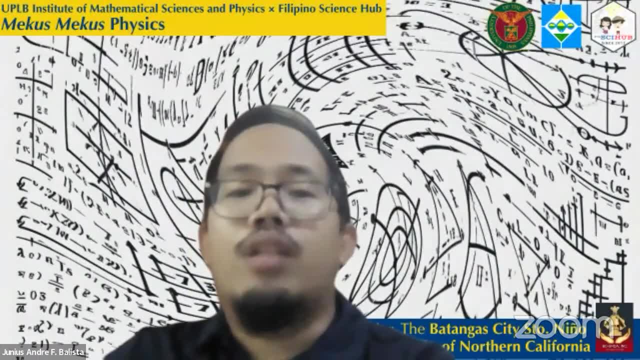 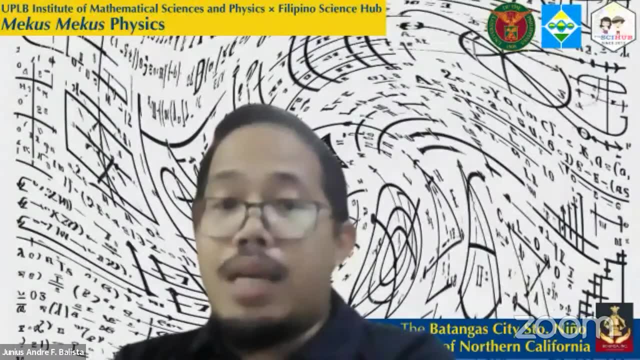 Yung unang pinaproblema ng, ng course, concept inventory, So yung tamang pag-intindi ng Newton's Laws, Kasi baka naubos na, For example, we have to recognize na ibang topic sa Newtonian because it's already the application of Newton's Laws of Motion. 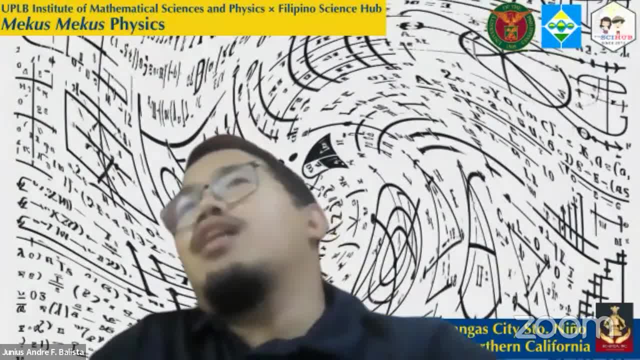 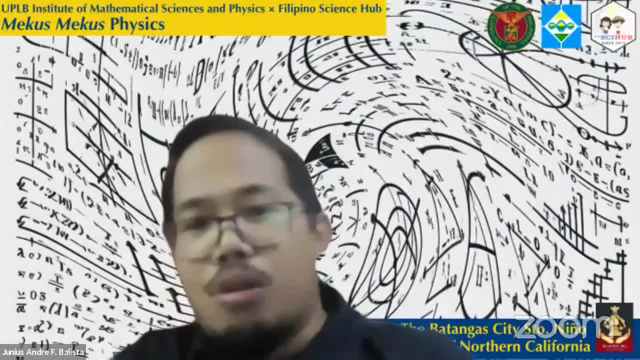 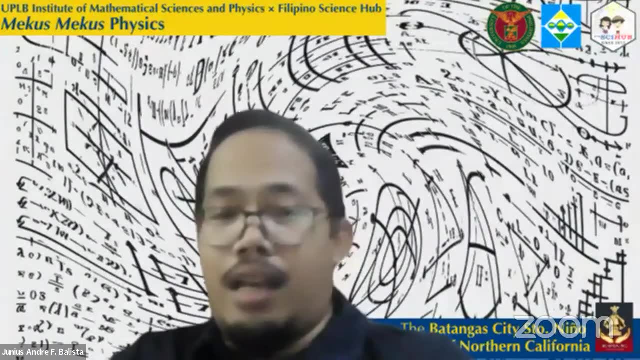 Diba, Lahat yan. So, kung limited yung time ang dapat na-emphasize, mo dun yung Newton's Laws of Motion, Kasi yung mga spring oscillation, Yung aerodynamics, yung fluid dynamics Application, yan na lang, yan ng Newton's Laws of Motion. 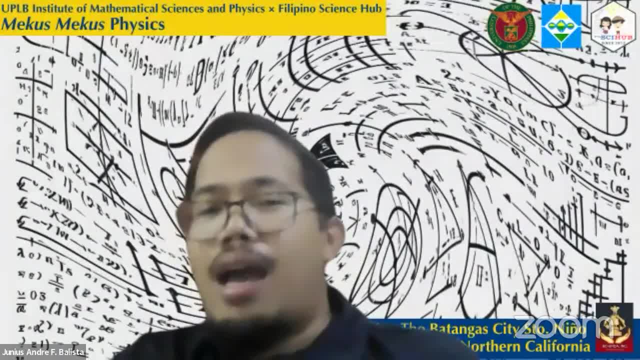 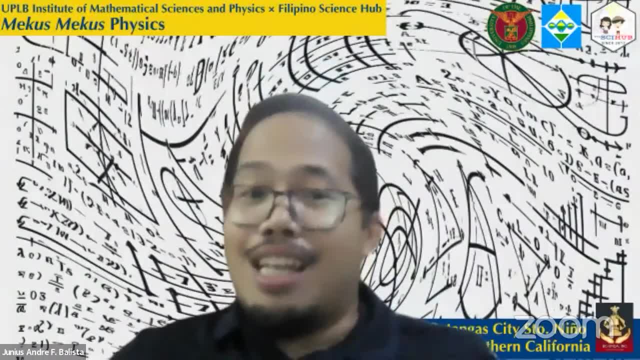 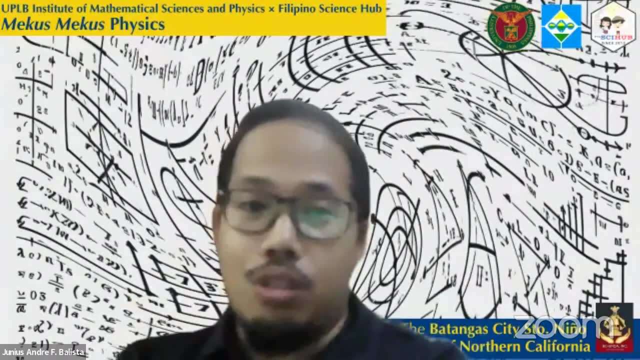 Okay, I have to admit I cannot really make a recommendation kung ano dapat ang mag-specify, Kasi kung ganun sana sinunod, Sana we have a more free reign sa silabus, sa curriculum. So 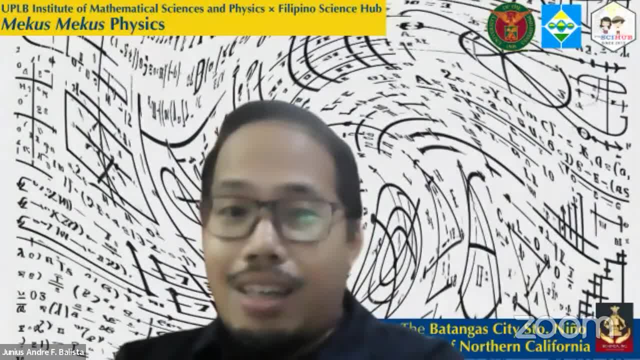 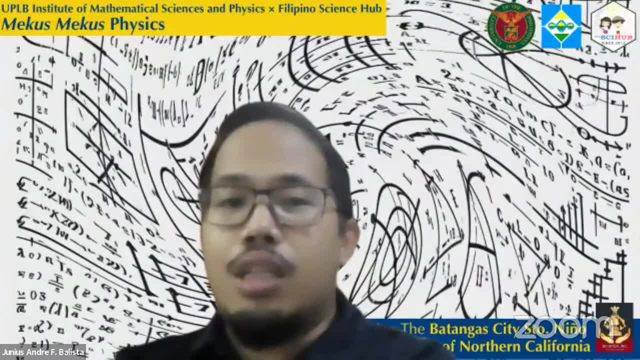 You have to consider kung anong na-require ng DepEd or ng school natin. Yun yung emphasize. So siguro communicate din natin sa administrator natin Or sa ano na ay kinukulang tayo ng oras. 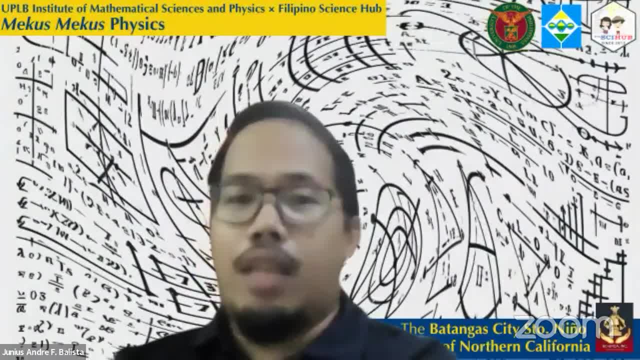 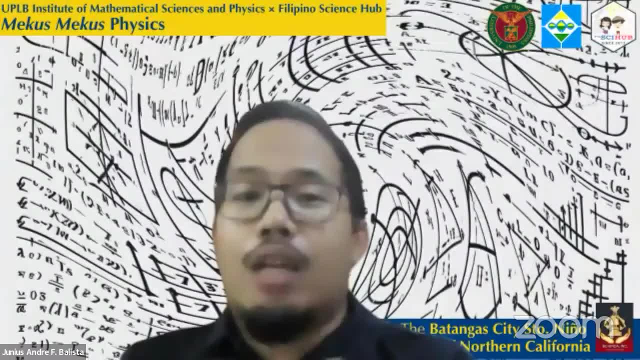 So dapat mag-decide tayo kung alin yung i-prioritize natin. So we have to comply with the regulations of the school. Pero kung on the conceptual side, kung akong tatanungin mo, 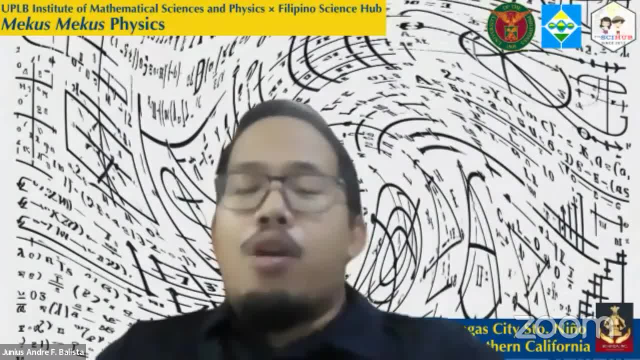 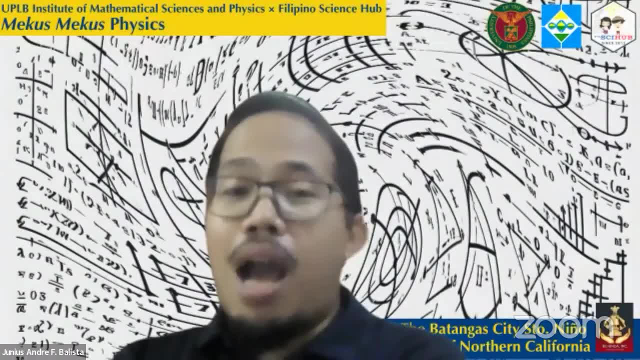 eh di yung Newton's Laws of Motion. Kasi once you get correctly you understand properly the Newton's Laws of Motion. Tapos hindi mo na-discuss yung mga application, Kahit konting application lang, iba pwedeng later na lang yan. 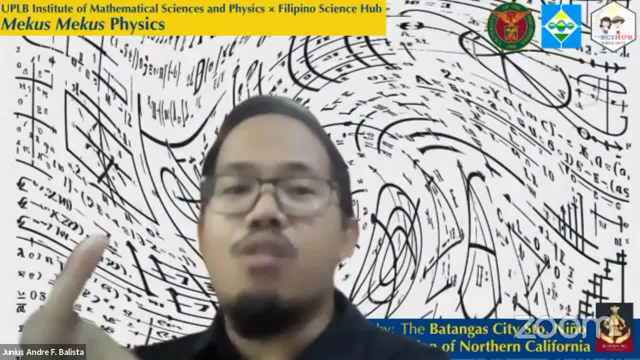 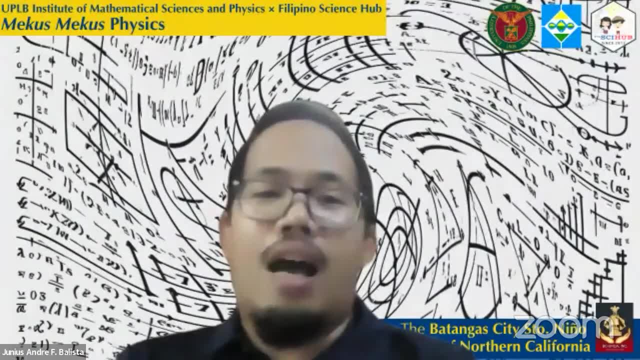 Sa next grade level na lang. Mas importante, yung Newton's Laws of Motion, Yung tamang pag-intindi ng Newton's Laws of Motion. But I have to admit may mga maraming factors in deciding. One is: siyempre we have to obey. 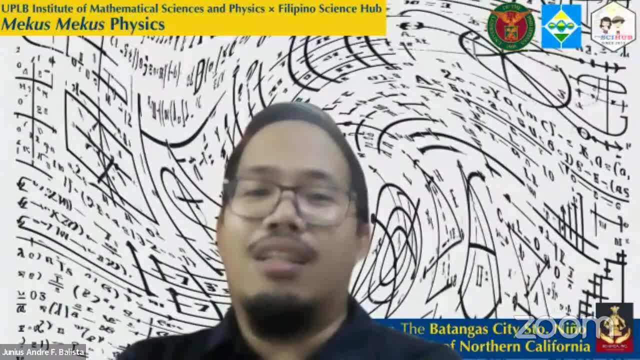 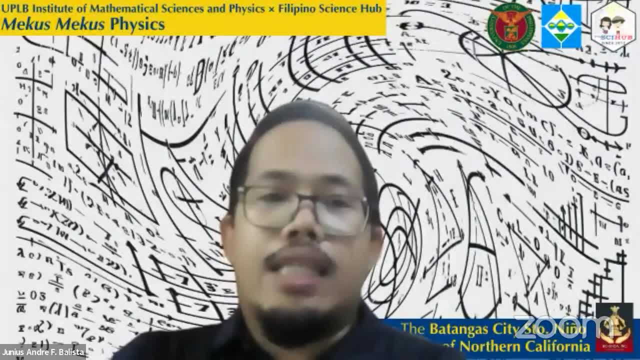 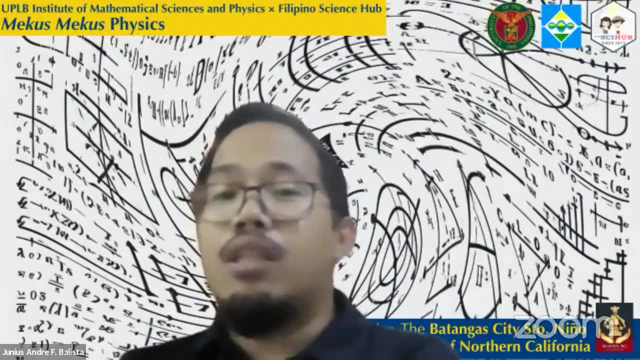 Obey, kung ano ang rules sa DepEd. Sa klase po namin nakita una po yung kinematics. Nauuna yung kinematics, Kasi usually nagde-define ka pa ng mga quantities na gusto mong ituro. 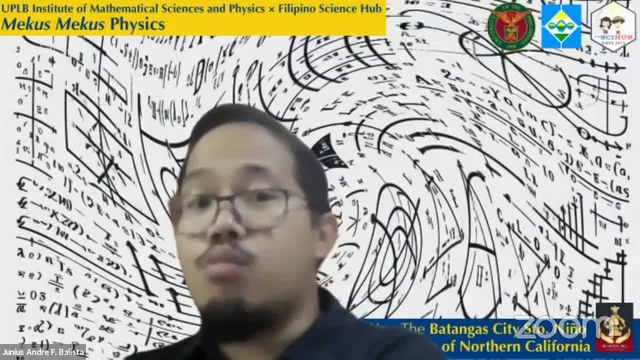 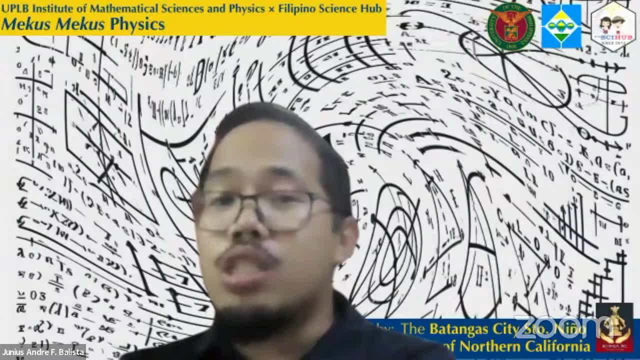 Kaya tinuturo yung kinematics. Kinematics describes the motion, not the cost, Kasi yung cost It's the force right, So the acceleration, So kaya siya nauuna madalas. Yes, Ma'am Anna. 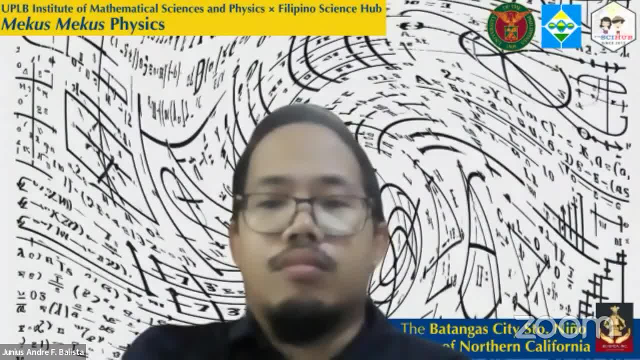 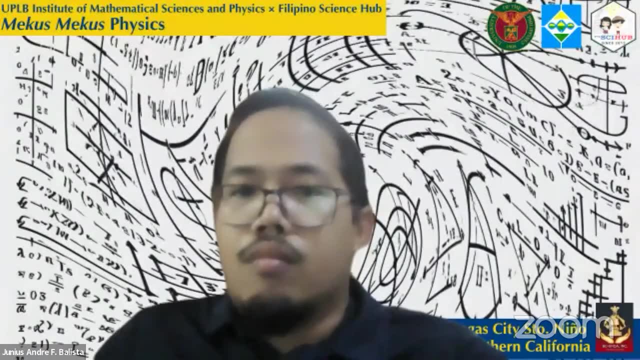 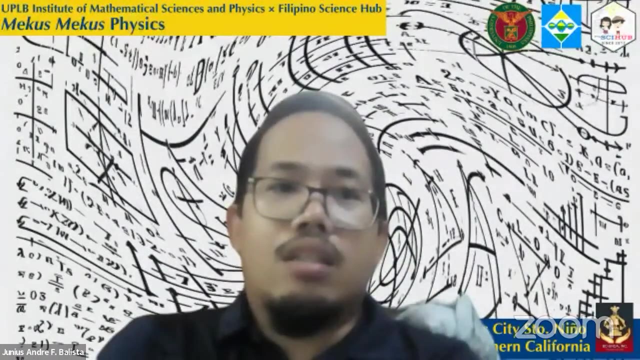 Sir, we can answer one last question po Question from YouTube, from Ryan Wong. So, based on your personal teaching experience, how do you assess the level of physics knowledge of entry-level or freshman college students? Siguro, Sir, bigyan po natin ng perspective from pre-COVID and COVID era or post-COVID era. 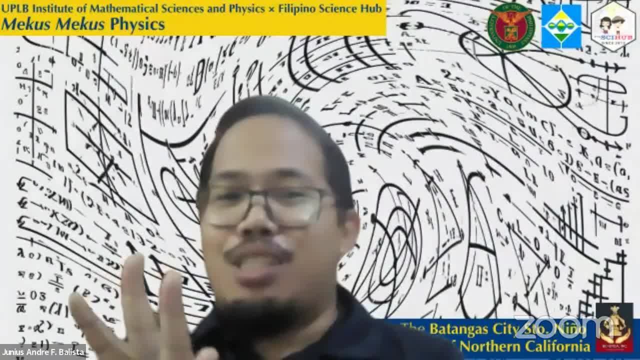 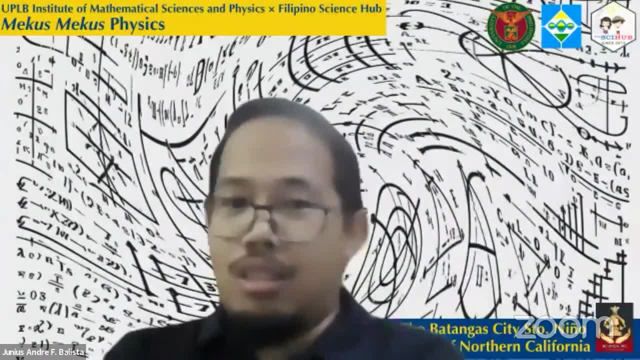 Actually una. the short answer is: I don't know, Because kaya nga actually, kaya ko ginamit yung I use with least result? Because we do not, unfortunately, many people. I have colleagues na nag-aaral ng doing physics research. 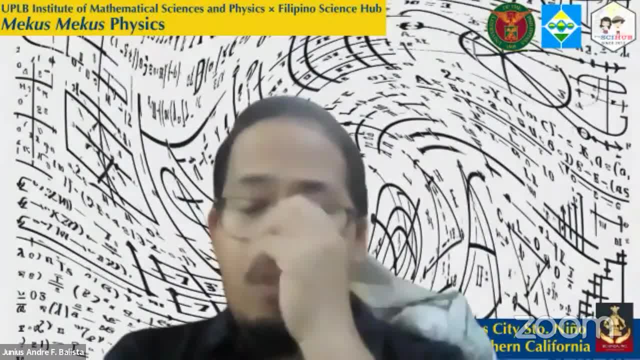 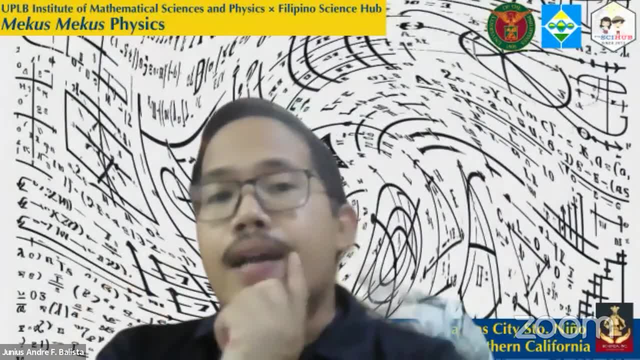 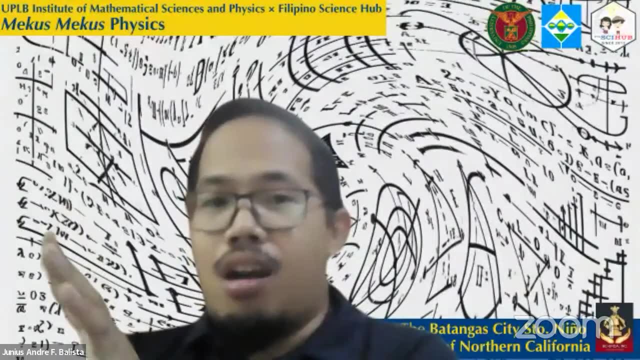 They have their results. Pero recently we don't have that fresh result. But based on that, ito the Whitley's response. the study give us a glimpse of what's the problem. So maraming misconception. 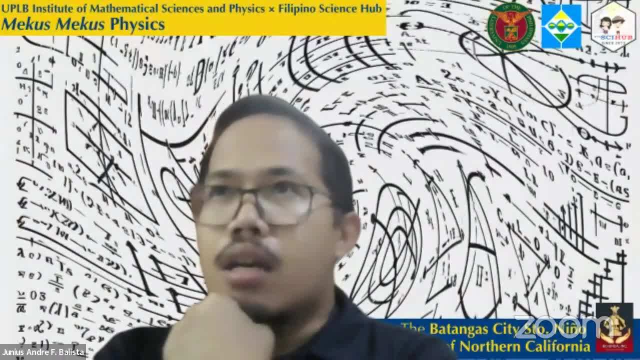 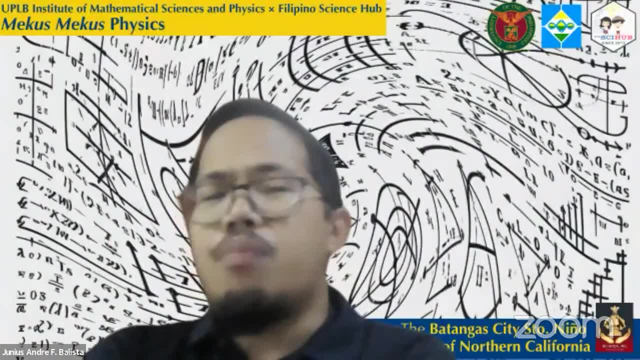 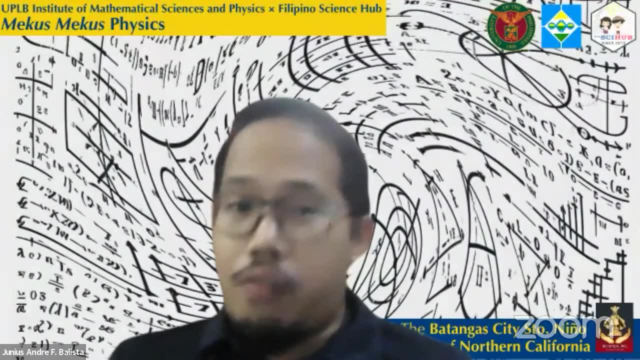 And usually ang sabi nila is unfortunately yung result ng force concept inventory. most of the students there is 60% and below mababa, Which is not really surprising, because pag-start mo first time mag-turo ng physics or mag-aaral ng physics, ang alam mo is Aristotelian, eh. 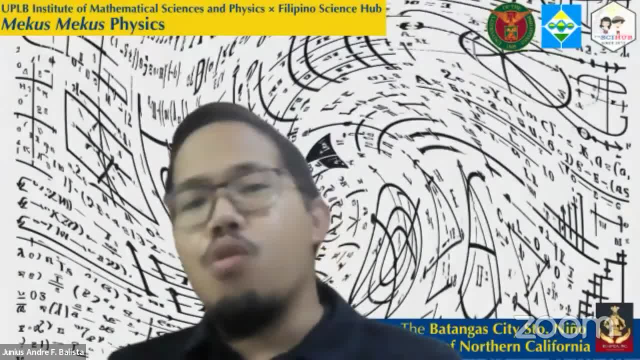 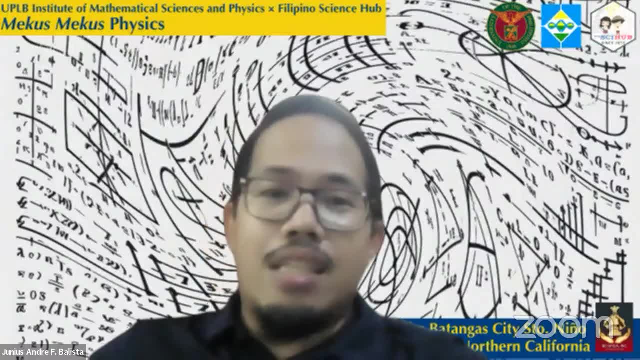 So marami ka talaga ng misconception. So I can say most likely sa Filipino students baka 60% or less din yung ating understanding ng Newtonian mechanics. I come from a high school physics special science. 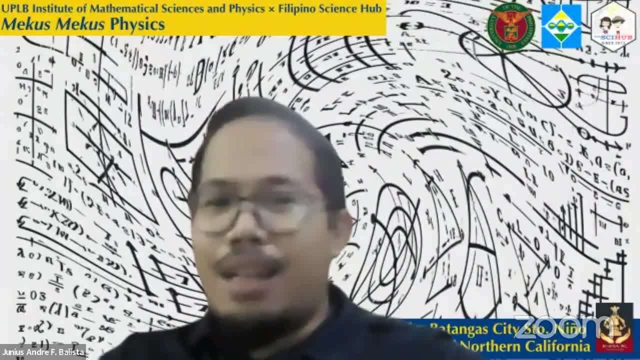 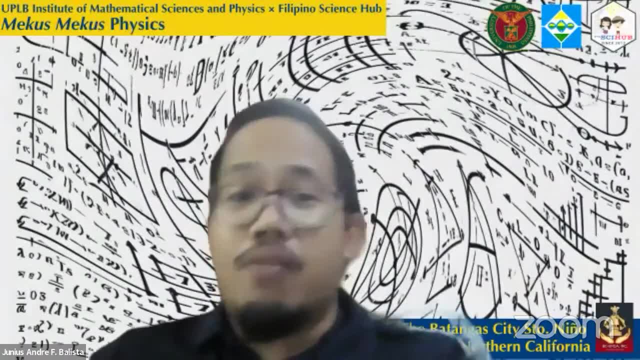 I graduated from Philippine science And I can say now, when I started sa college, I can say na parang feeling ko wala rin akong medyo mahina, ako pa rin sa physics, eh, So kung how much more yung? yeah, this is not really negative sa physics. 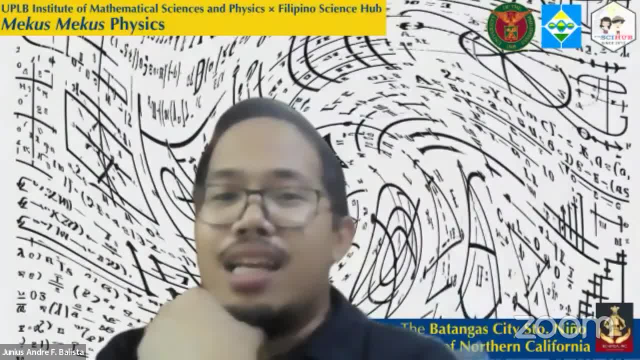 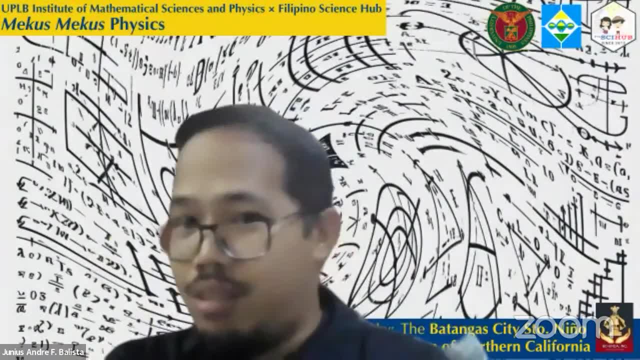 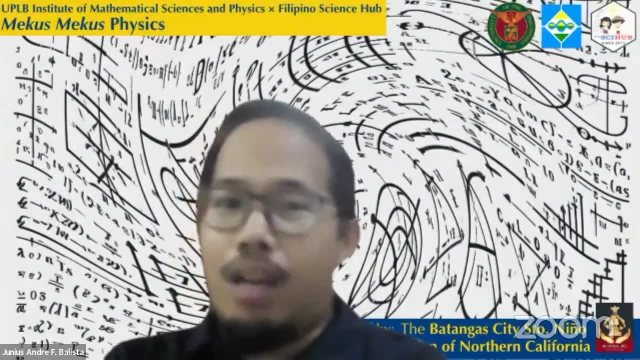 Natural lang medyo hindi marami pa rin akong misconception sa physics, eh, So most likely the same din yung iba or even worse, Yung ibang students na hindi from Philippine science. So 60% or less. 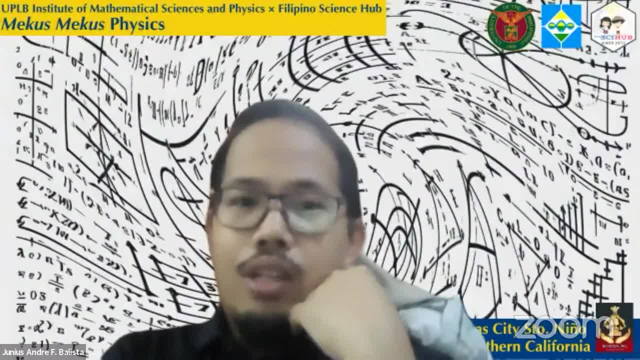 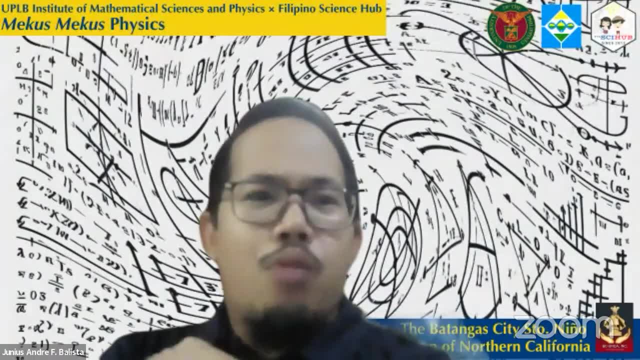 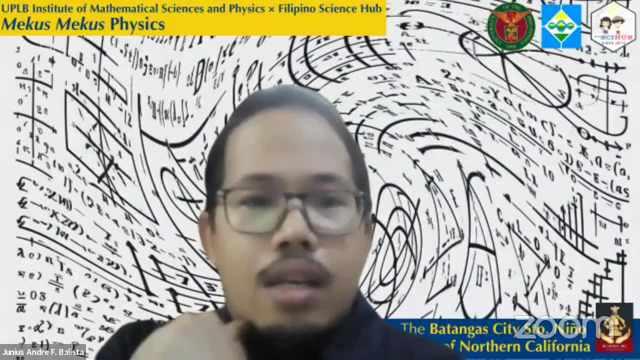 So maybe you can gauge it from there, But we don't have a figure. I don't have a figure, Probably I don't have a figure from the Philippines. Yeah, Maybe one more: Isa pa Sige po sir. 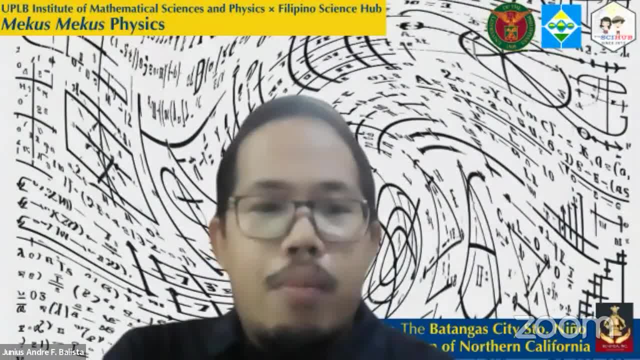 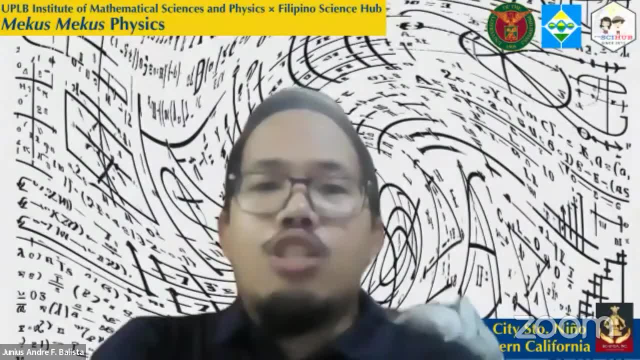 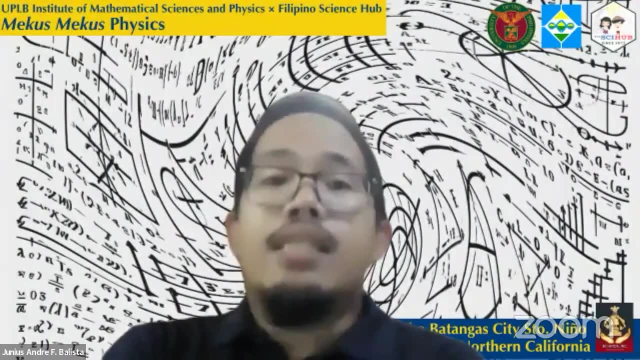 Sir, last question On what lessons po nababangit ang delivery At integrals sa. sorry, Hindi ko nababasa. Ah, okay, At what lessons po na nagagamit ang derivatives at integrals sa physics? Kasi grade 11 ko na siya, hindi pa kami behind sa klase. 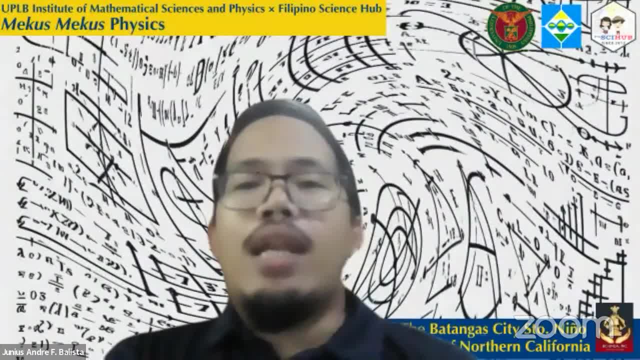 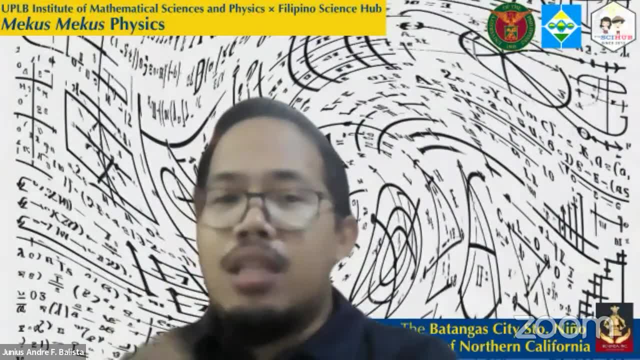 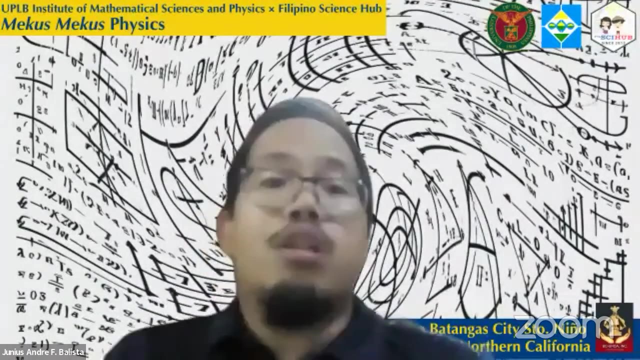 It's okay po. Ah, okay, Sige. Okay When I say pwede pong walang derivative or integral. Sorry, let me just clarify: Derivative is change Diba, So ang pag diba Momentum, initial moment final minus initial momentum over change in time or time interval. 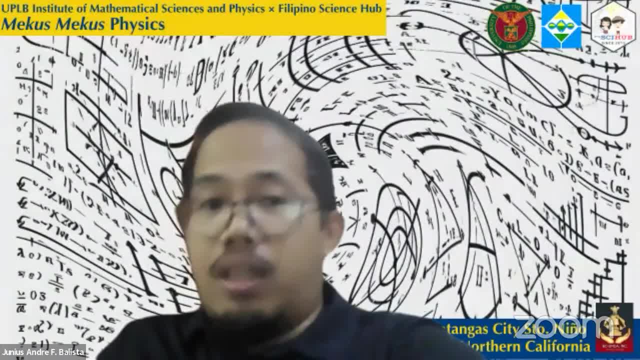 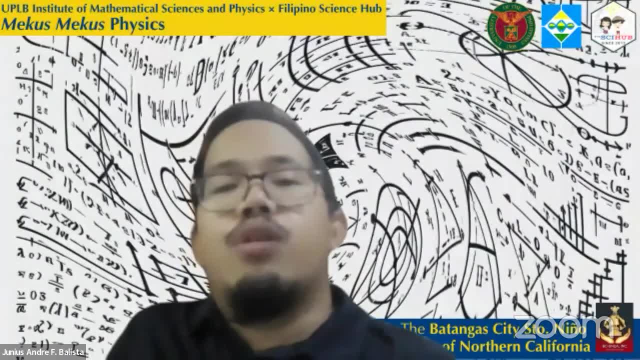 So basically, when you get its limit, that's the derivative. So pwedeng hindi pa na-discuss. Pero you don't need to say it's a derivative. But at the level of grade 9 to 11, kung hindi man nag-calculus or hindi pa gumagamit ng. 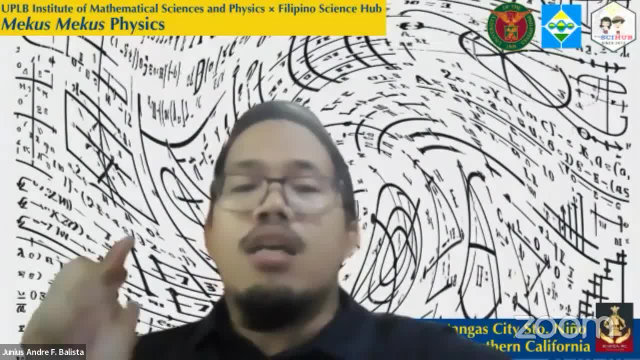 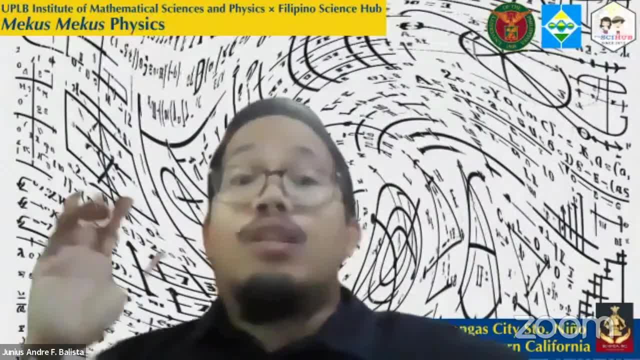 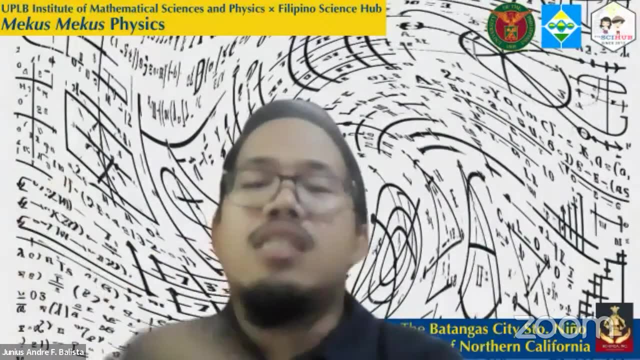 calculus. Sigurong isang kailangan lang. i-emphasize that Newton's laws of motion ay it's about that change in momentum. So dapat i-emphasize, siguro sa akin, kung ako in my opinion we emphasize that force will. 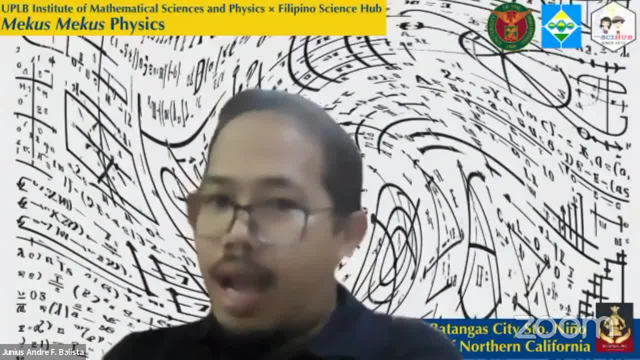 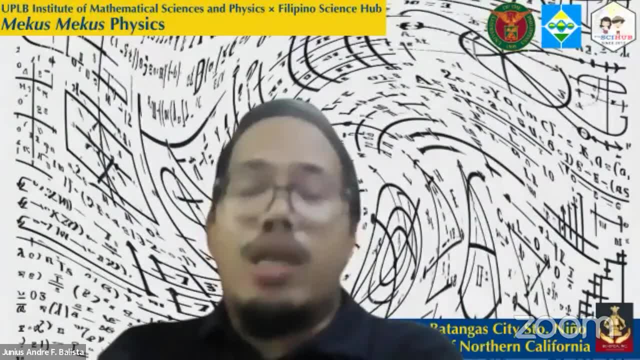 lead to a change in momentum over time. If you cannot say it's a derivative of the momentum with respect to time, force will lead to derivative. We can say that force will lead will cause the momentum of the object of interest to change over time. 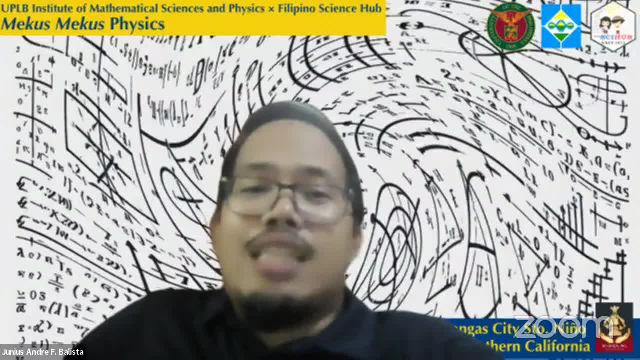 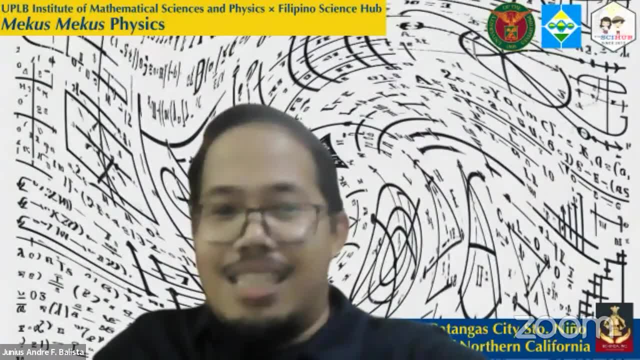 So change. So okay lang yan. I understand pala baka nga sa high school hindi pa wala pang calculus, But there's a name for it: Change, Change, Change po Change with time. That's the, that's the derivative. 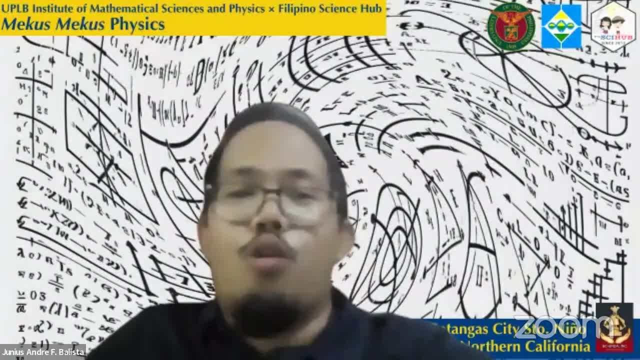 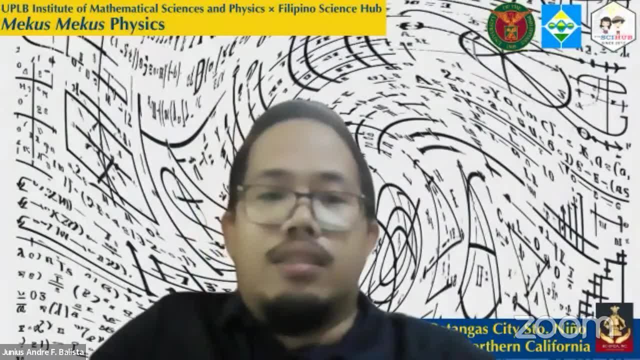 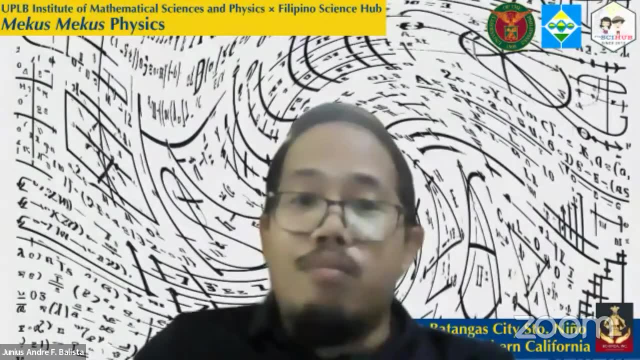 Yes, Slope, Slope, Slope. Or change with time, Or slope with respect to time of the graph with respect to time. Okay, Ayan tama Sabi ni Ma'am Anna is: yeah, If you plot the position versus time, you will see that velocity is the derivative or is. 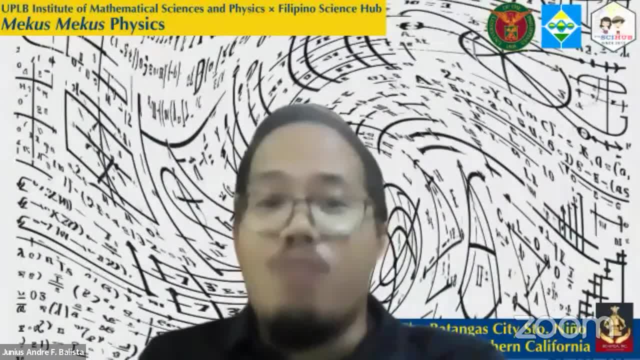 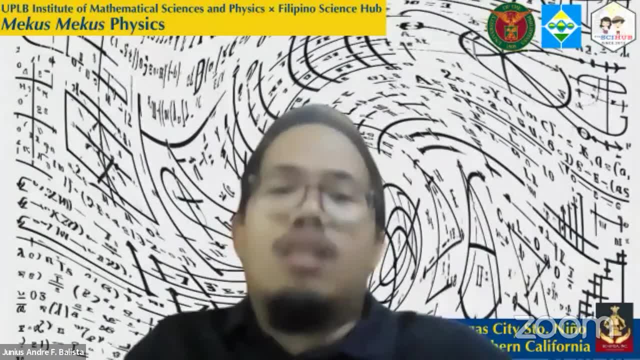 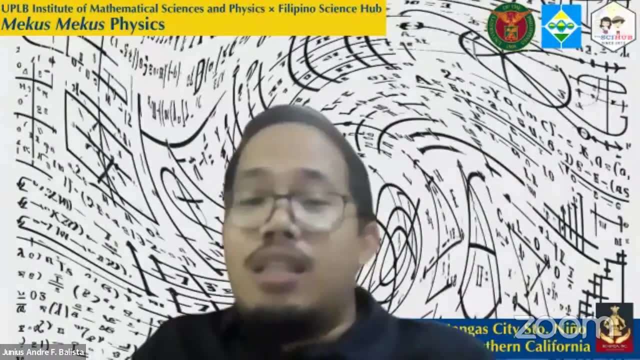 the slope Acceleration is the slope of of velocity plotted versus time. Okay Yun, yung instantaneous velocity, Yan Kailangan Yun nga, Ma'am Anna. Kailangan natin ng yung concept ng instantaneous. It needs the, it requires the concept of finite, infinitesimal rather. 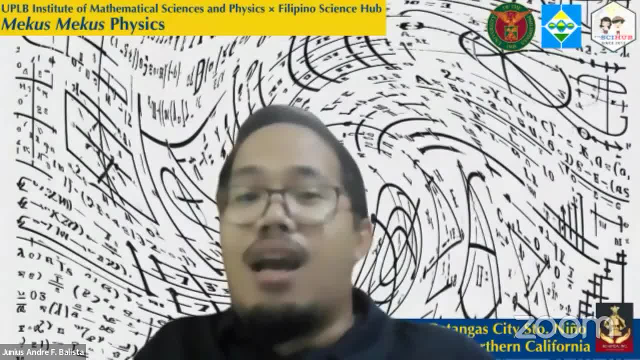 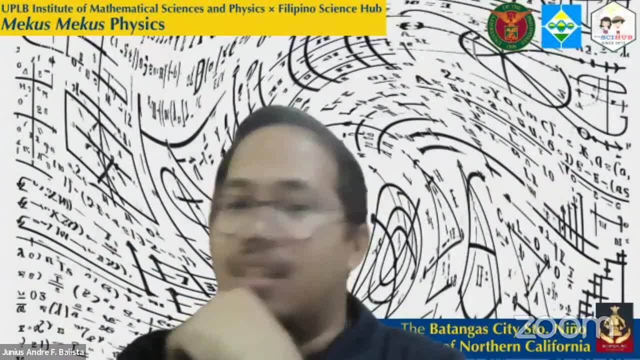 So that's why ano din nagkakaroon ng misconception. But ito rin sa akin: Sometimes you just have to accept na at a certain level nandyan pa yung misconception, So don't feel bad. 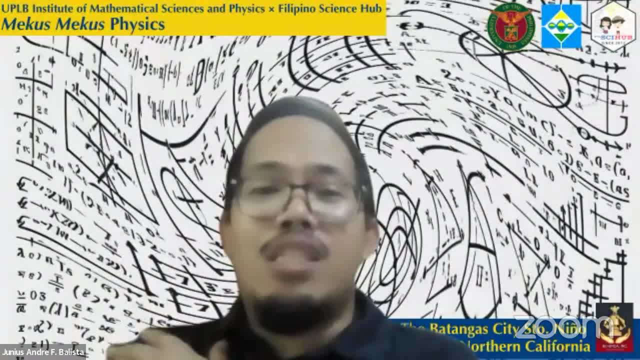 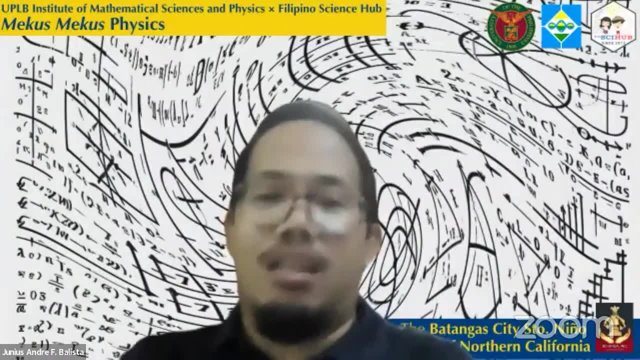 So akin din dun siguro sabihin sa estudyante: don't stop learning physics, But rather if you have misconception, that's all the more that you should take physics next year. Okay, Kasi yung madalas sa atin. ah, maraming kang misconception, huwag ka nang mag-physics. 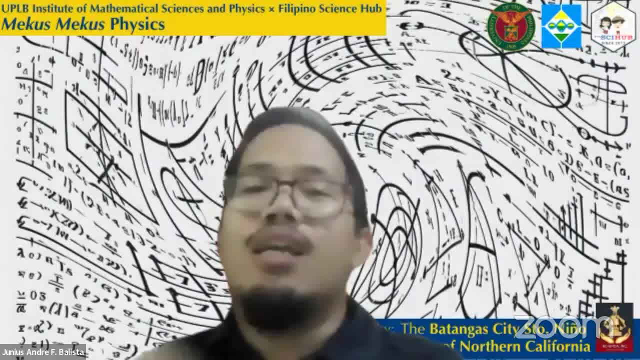 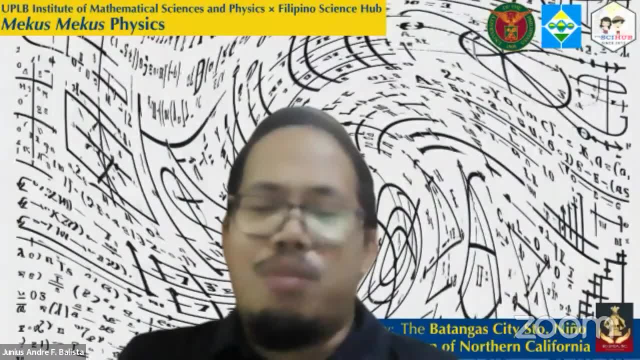 Baliktad, Most likely at grade 9, ang daming misconception. okay lang yan. Make sure lang na huwag namang bumagsak sa exam. Pero it's okay. To me it's okay. Don't really feel bad about it. 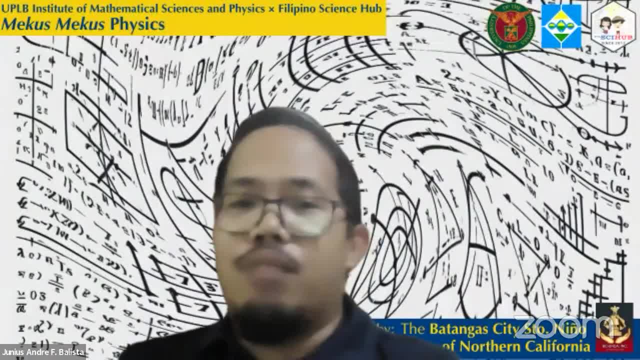 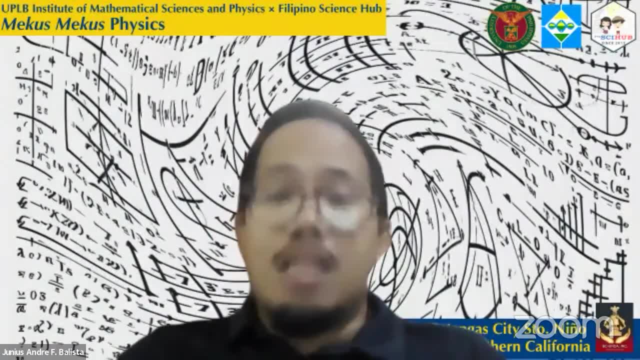 Just try to remove it. Keep on trying lang, But don't don't stop and don't feel bad about it. Okay, Don't feel bad about it. Yan lang yung masasabi ko dun sa student, At saka sa teacher din. 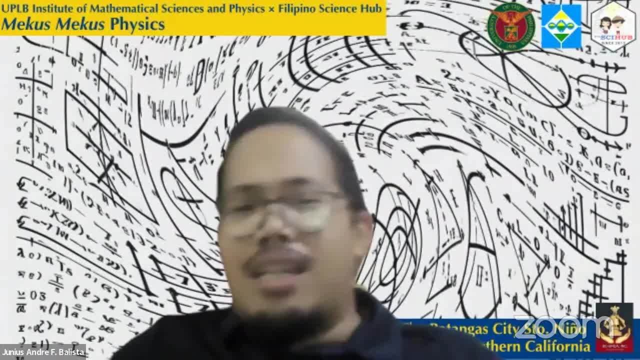 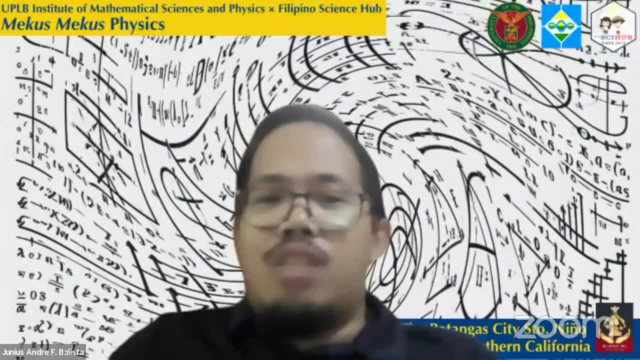 Okay, Don't feel bad. Of course we cannot siyempre siguro sa mga public high, sa high school we need to compete na dapat magaling yung estudyante natin sa ganitong exam, etc. 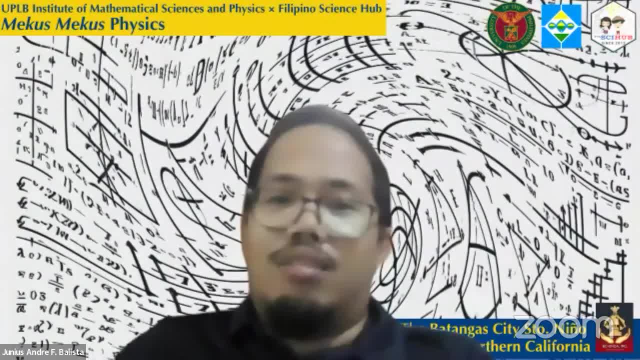 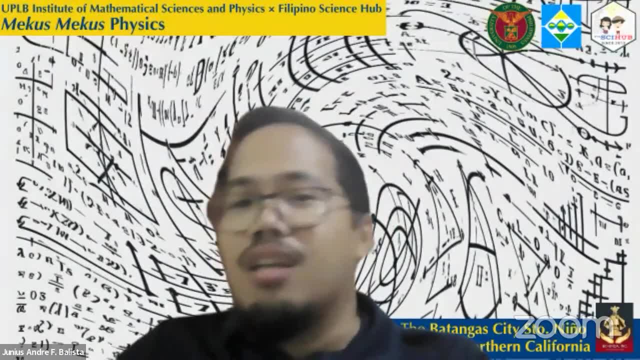 Pero I personally don't agree with it. You can, there are things na nandyan talaga, So you just keep on doing, keep on trying. So don't penalize the teacher. Encourage them, that don't penalize. 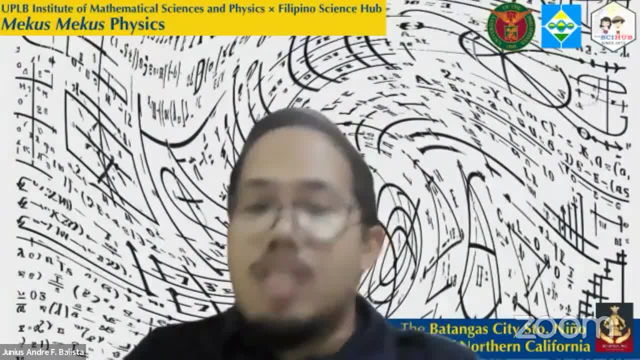 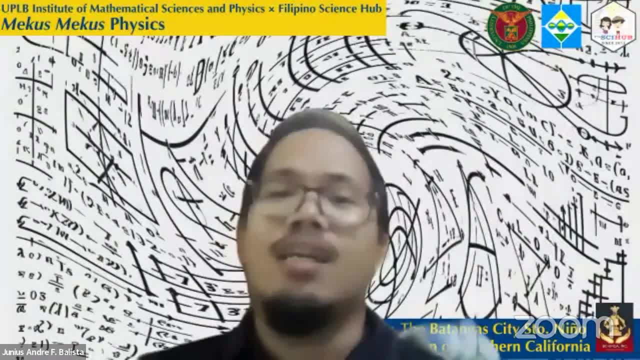 Don't. don't penalize the students. Just keep on trying to teach it And accept that there's a possibility that the misconception still remains. Okay, lang yan, Just move on to the next level, All the more that you must be encouraged to go to the next level. 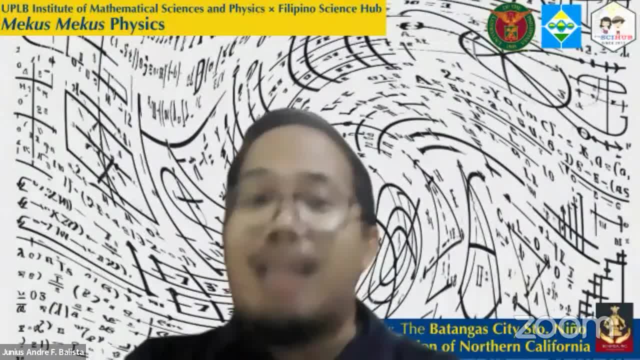 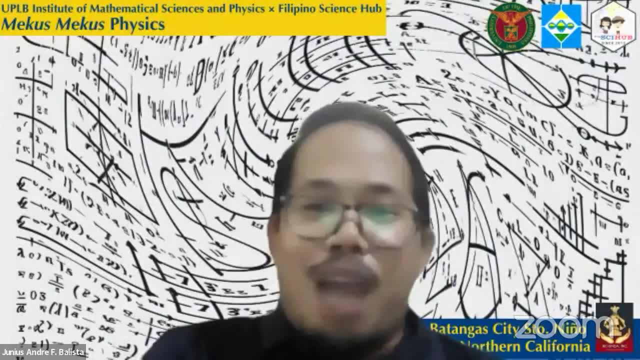 So don't feel bad and don't think badly of those who have misconceptions. Okay, I appreciate yung daming questions po, So siguro hindi na natin masagot lahat. But I emphasize, this is just a short conversation. 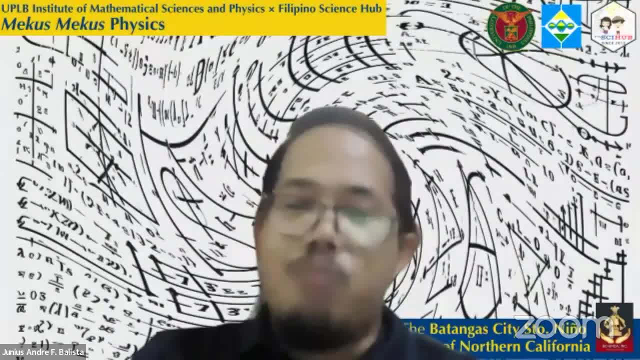 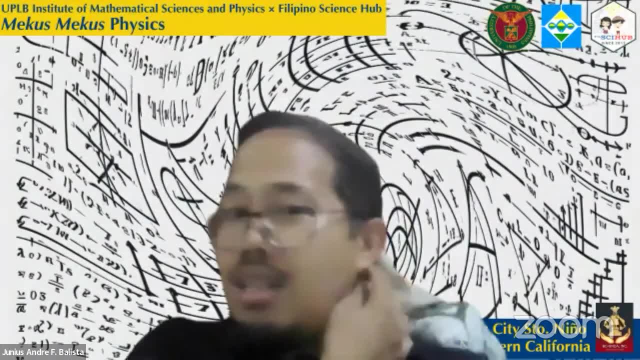 We have, we have. I'm realistic but optimistic about my expectation for this lecture, So we're still willing next time meron pang next time. So thank you for those who ask questions. Pasensya na po yung hindi masagot. 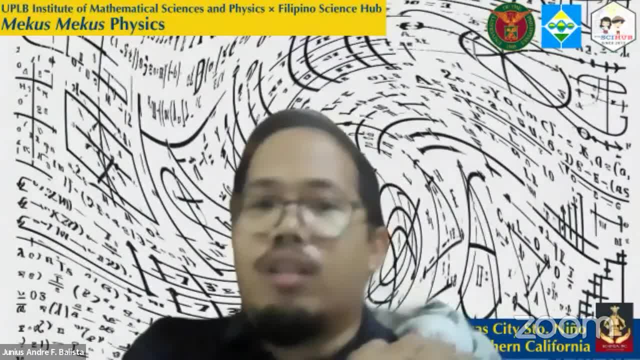 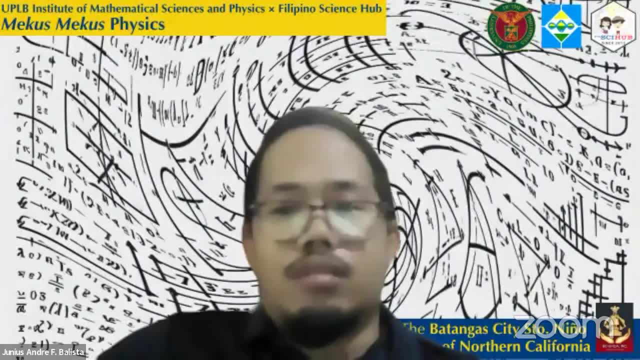 But you can. maybe you can still email me or contact me. if you have more questions, I'll try to answer them. Okay, Yes, that's right, sir. Again, thank you. Thank you, Dr Balista, Sir Junius, for that comprehensive discussion. 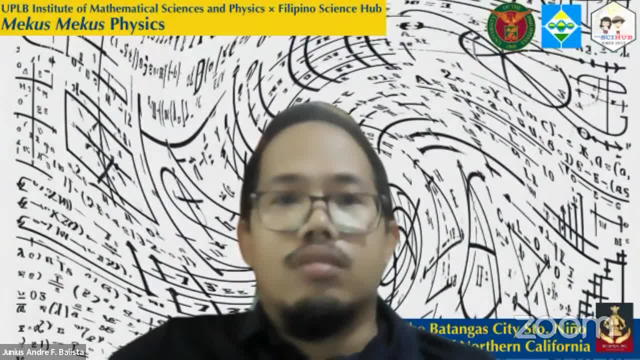 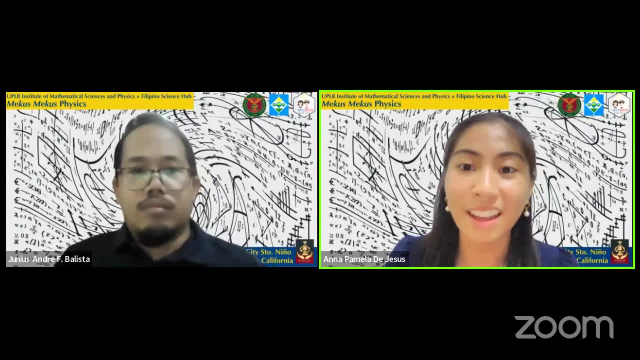 And also yung insightful na Q&A. Thank you, Sir Junius, for your answers And I hope a lot of our participants learned a lot through this event And we hope na na-address din yung mga common misconceptions in physics. 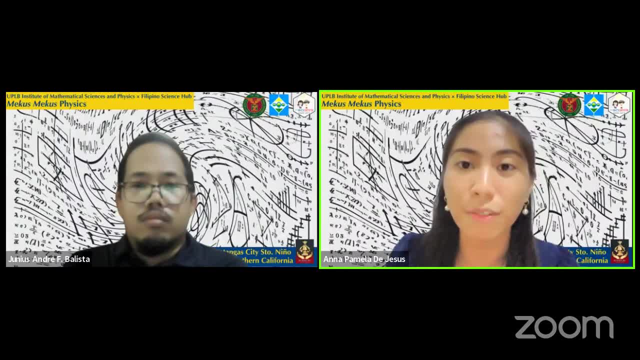 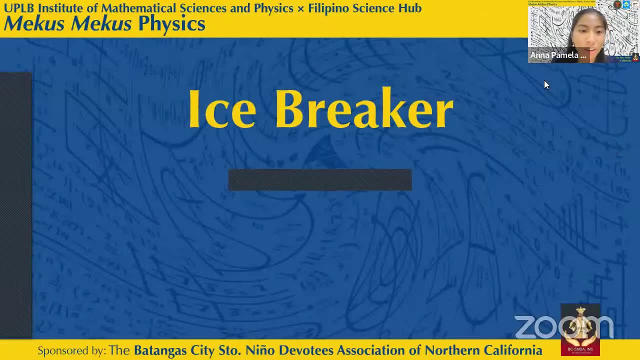 And we also would like to thank everyone for the participation. Doon sa quiz earlier, Pero at this point, before we have our announcements and before we end our program, we would like to invite all of you for a for an icebreaker. 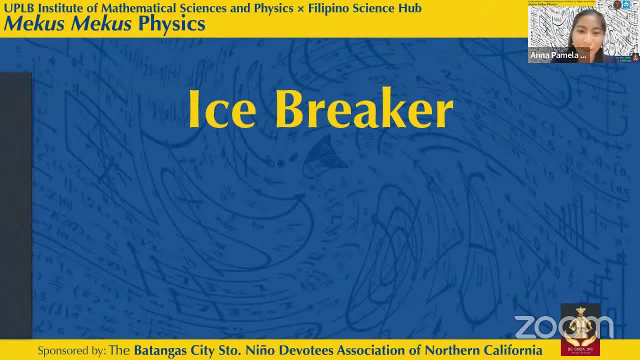 So this is another opportunity for our guests to participate. Yan So naka-flash na ba. Yan So very quick lang naman to. Our icebreaker is called Yan Bagong bago. Four picks, One word. 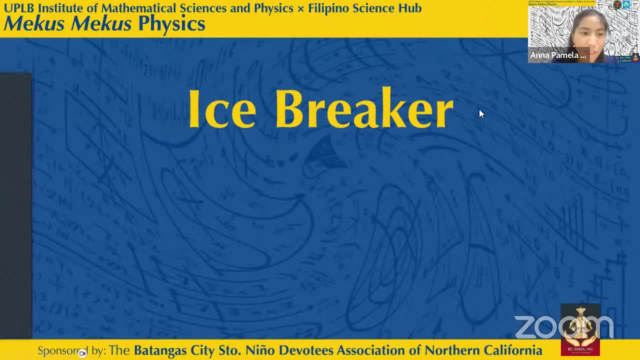 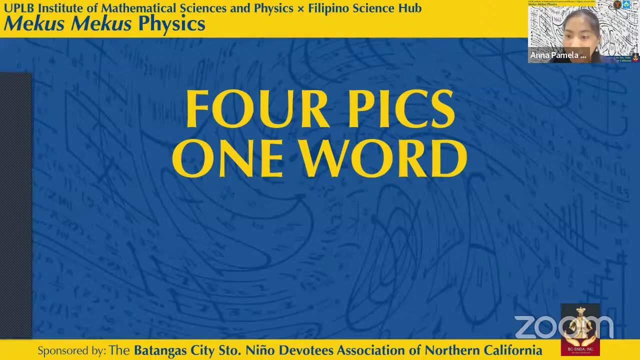 Yan, I'm sure we are all familiar with the game, So I'm going to show you four pictures And then paunahan na lang. siguro no na mag-type sa chat box, Yan, Paunahan mag-type sa chat box ng word that those pictures represent. 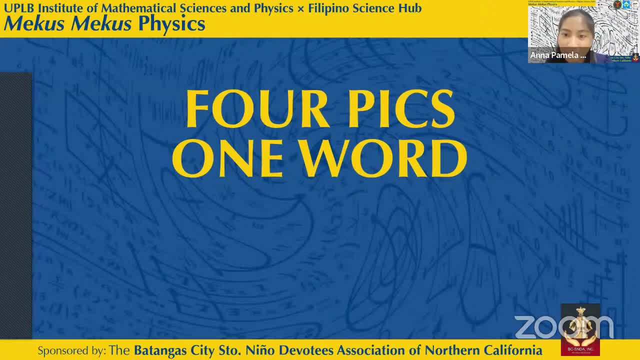 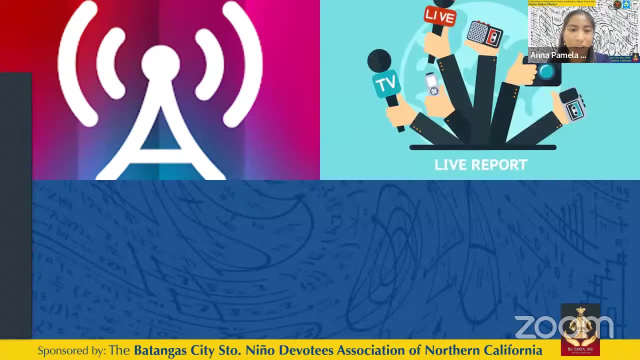 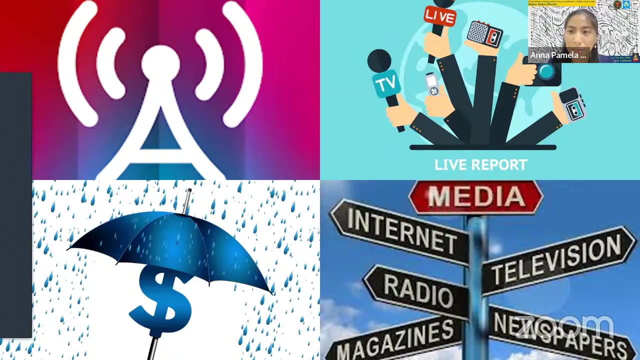 Sige, Baka pwede tayong mag-trial, Pwede pa natin ipakita yung four pictures. Okay, So ito yung first set of the four pictures. Ano, kaya ang nirepresent niyan. 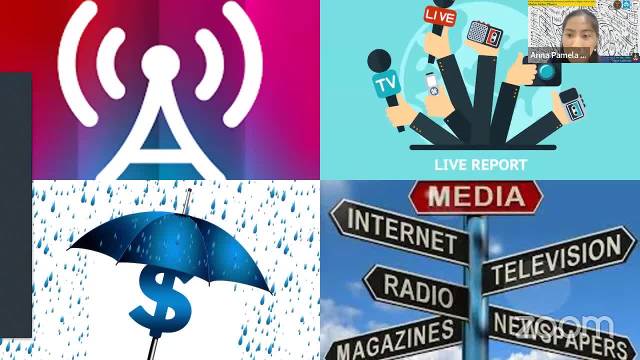 So meron tayong media signal, misconception, multimedia. Okay, The correct answer is: wait lang po. The correct answer is: Ang tamang sagot daw ay: coverage. Parang walang makasagot, Okay. 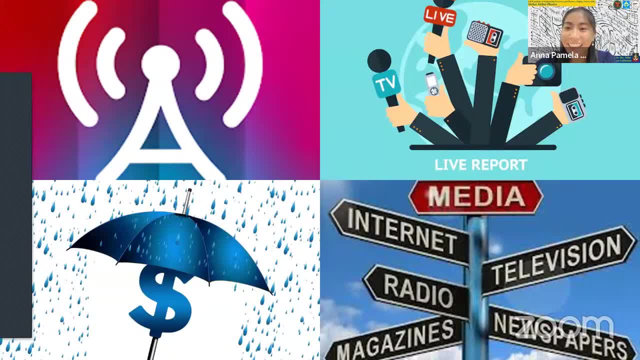 Pero trial lang naman yun. Trial lang naman Okay. Ito na yung totoo. So we have three sets of pictures, Tapos kung sino mang makakasagot ng una ay may prize. Ano po. 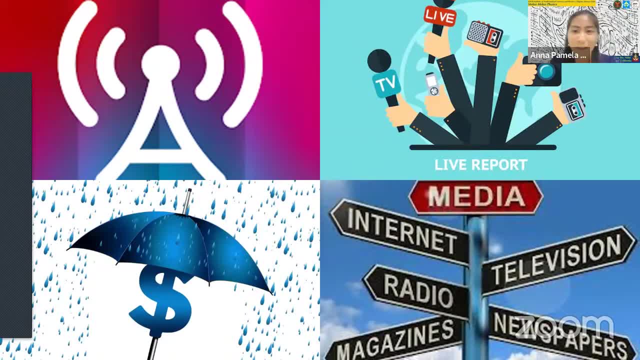 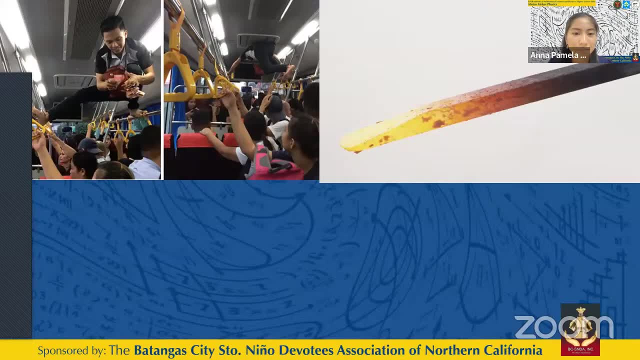 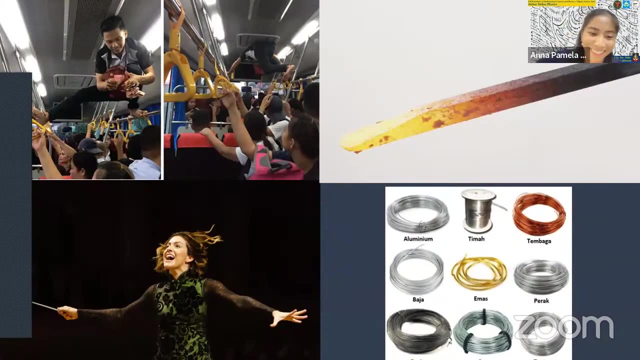 Yan. So the second set of pictures: Ayan, Okay, Ito na po ang mga answers. So the correct answer is conductor Okay, So the first one to answer is those Mike Kenneth Ingrito. So please wait for someone from the physics division of IMSP to message you for your prize. 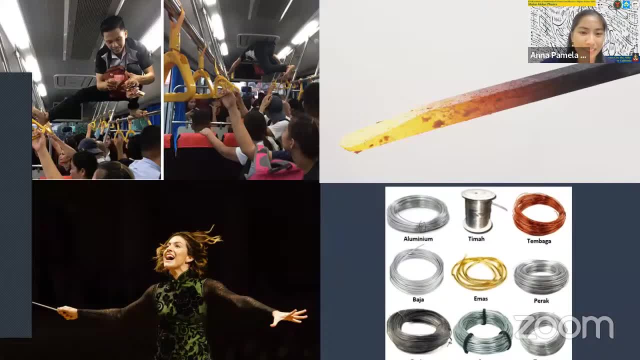 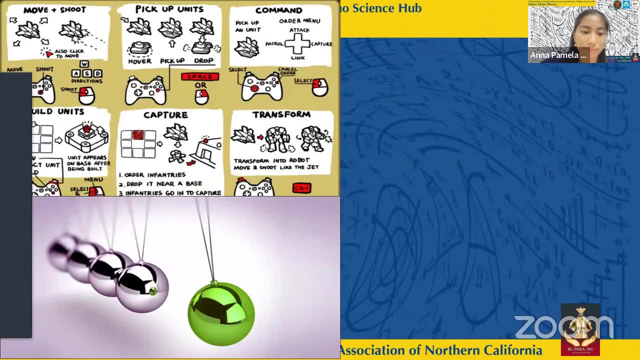 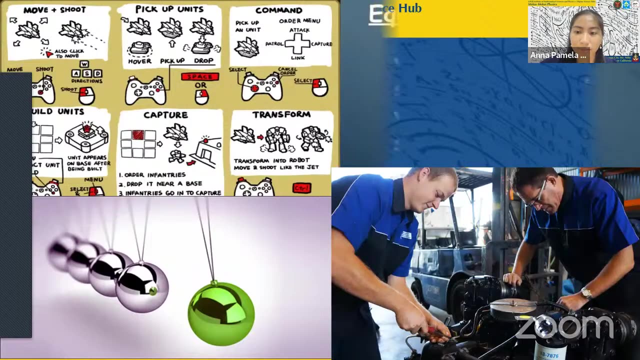 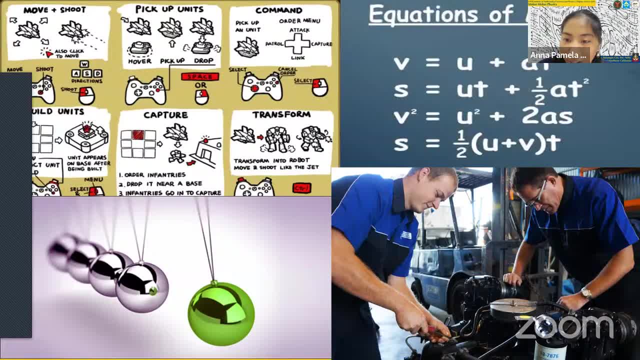 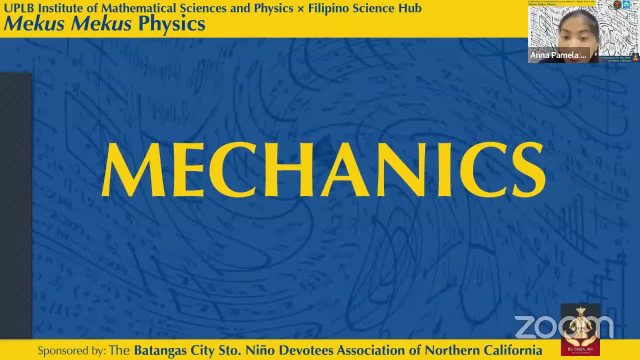 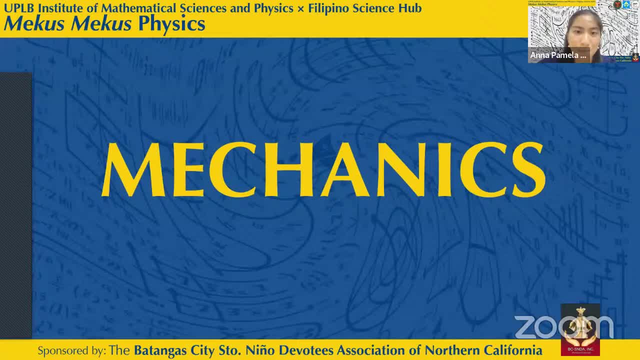 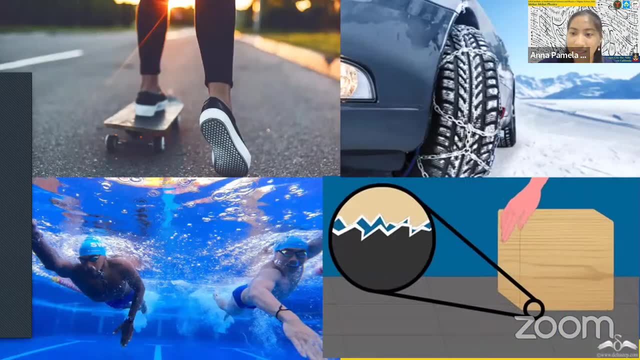 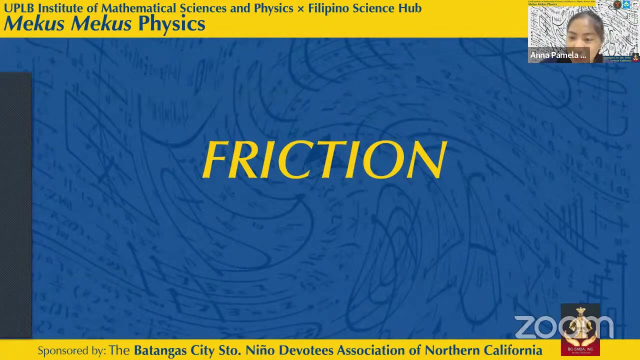 Ba Sing Pantaya isika Basa Ayan. so the correct answer is Friksyon, So Friksyon ayan. So our winner is EJ Zuniga, EJ Zuniga. So para sa mga winners, natin just wait for a message. 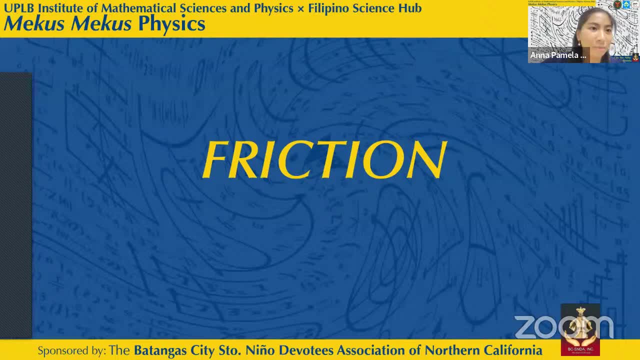 from one of the faculty members of physics division of UPLB-IMSP to claim your prize. Again, congratulations to all the winners And sana nakapag-enjoy kayo, Nag-enjoy kayo dito sa very sure. 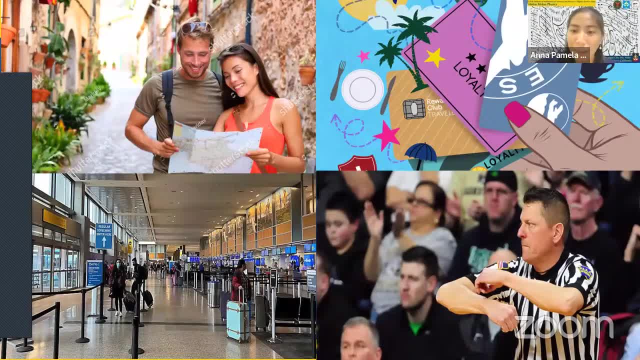 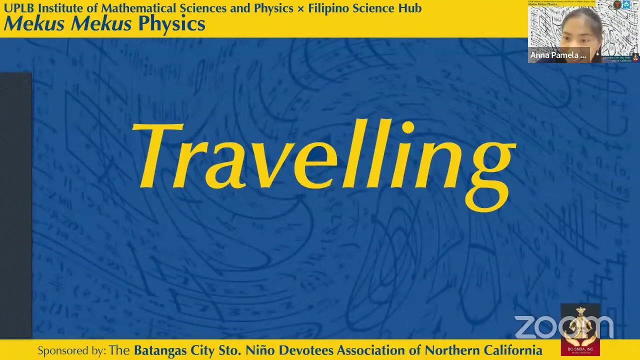 Ah, so we have one last. Ah, okay, Meron pa pala. Sorry, meron pa pala. Ayan, Meron. Ang tamang sagot ay traveling. The correct answer is traveling, Okay, so let's be strict, no. 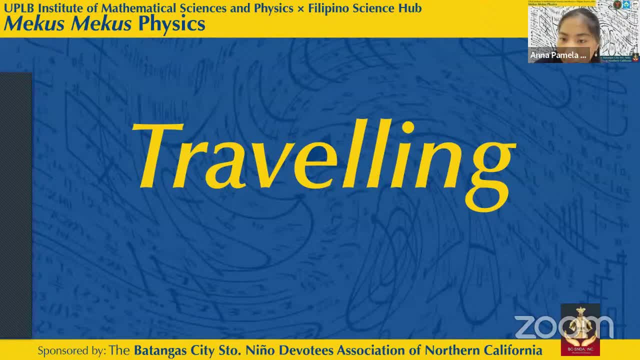 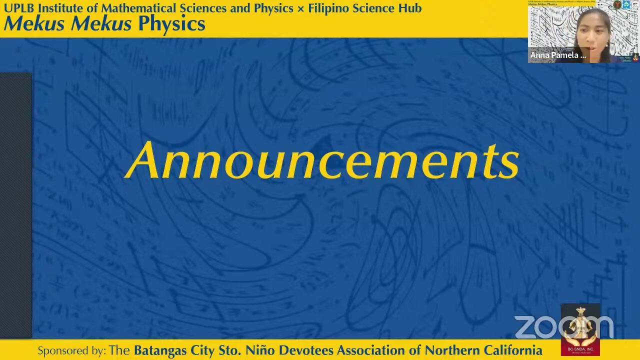 Ang tamang sagot ay traveling, So the first one to enter the correct answer is Princess Lorelie Gacusana. Okay, congratulations, Miss Princess. Do we have more items? Ah, okay, Announcements na. Alright, so congratulations again to all our winners. 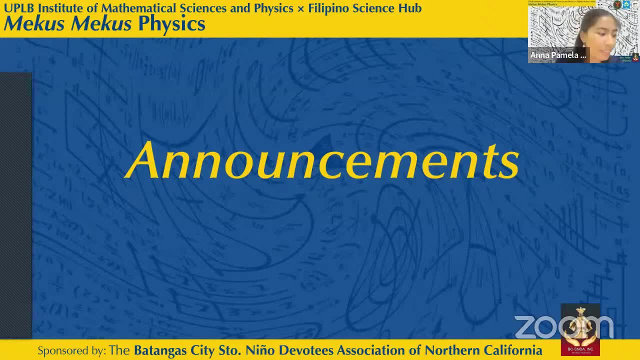 And just some announcement. Now we have one announcement. Ma'am Ana may nagtanong kanina saan yung site For FCI for teachers? So ito po fesportorg slash assessment FCI. So teachers lang po yung pwede dito na mag-access. 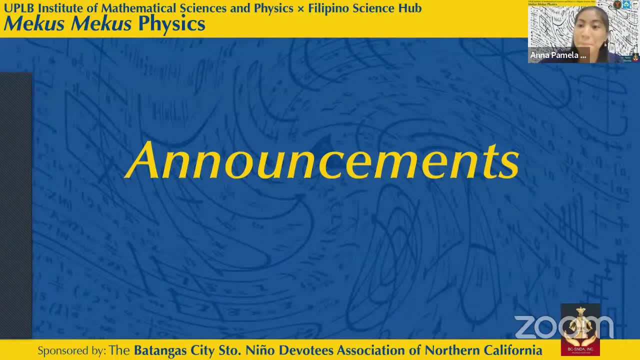 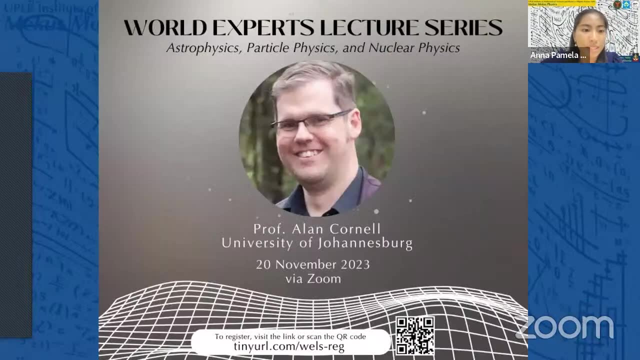 Thank you. Thank you everyone for the question. Welcome po for those who thank Okay po Sige pakiflash po ang ating announcement. The physics division IMSP UPLD, in coordination with FISICA, UP Applied Physics Society, will hold: 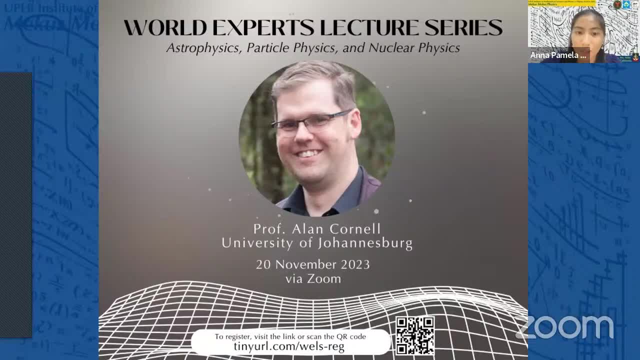 the Astrophysics, Particle Physics and Nuclear Physics Symposium on November 20, 2023, at the Physical Sciences Lecture Hall B. So that's on-site, but you can also attend via Zoom. So you may, you may. you may. just want to scan the QR code. 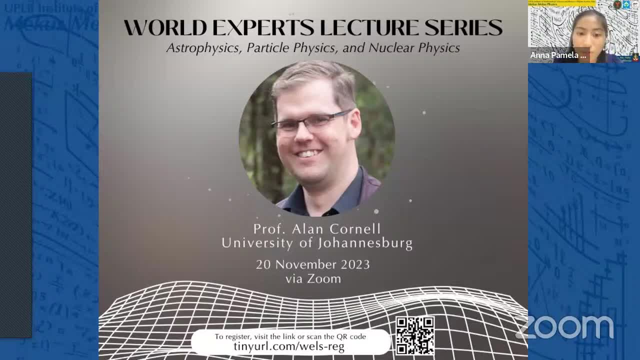 or just visit the link that's tinyurlcom: slash wells dash reg. Yeah, so this event is a part of the World Expert Lecture Series, or WELS, with Professor Alan Cornell from the University of Johnsburg as the main speaker. 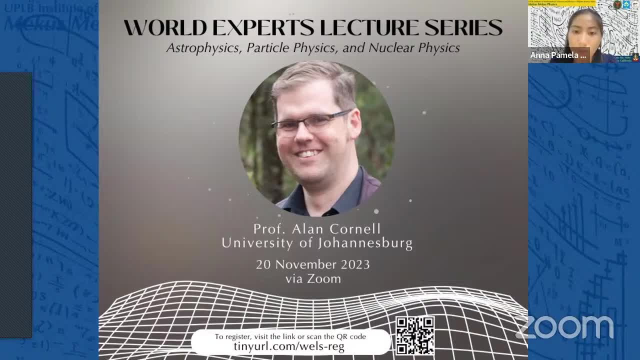 So WELS is a program by the UP System to further expose and inspire students, faculty and staff and in support of the internationalization goals of the university. So the main goal is for the promotion of astrophysics, particle physics. 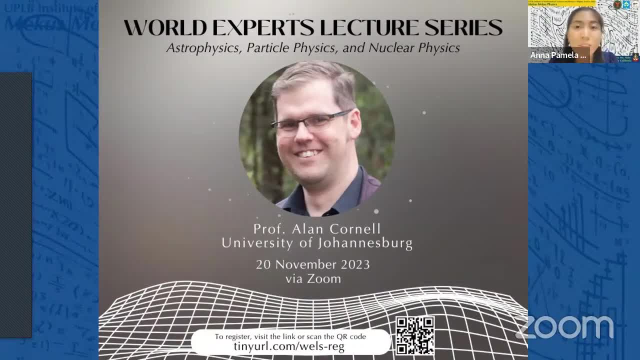 and nuclear physics in the country, So we are inviting you to this event. If you cannot come on-site, you may opt to join online. To register, just visit the link or scan the QR code on your screens. And we would also want to hear from you. 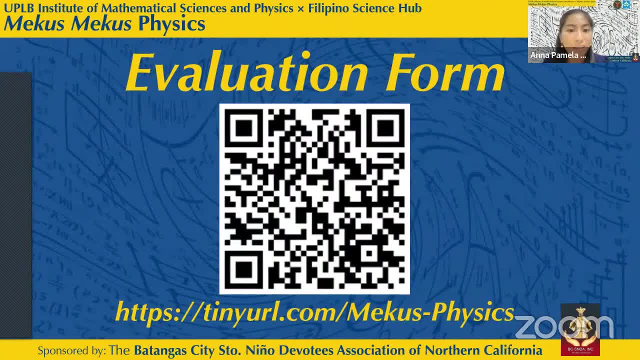 about how this event was conducted, so please fill out the evaluation form Again, you may just scan the QR code and after filling out, you shall receive your Certificate of Attendance. Okay, So I think that's it for our event this morning. 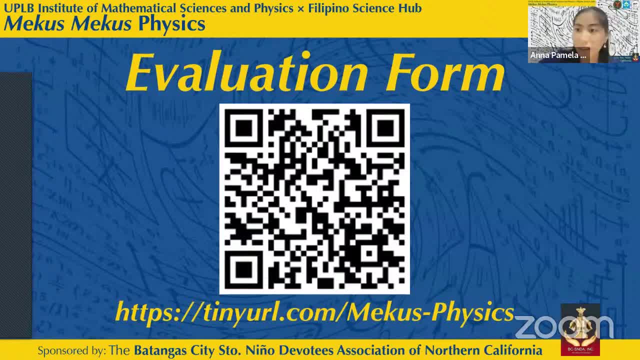 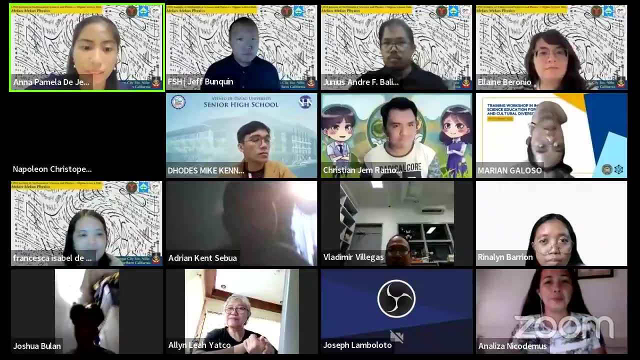 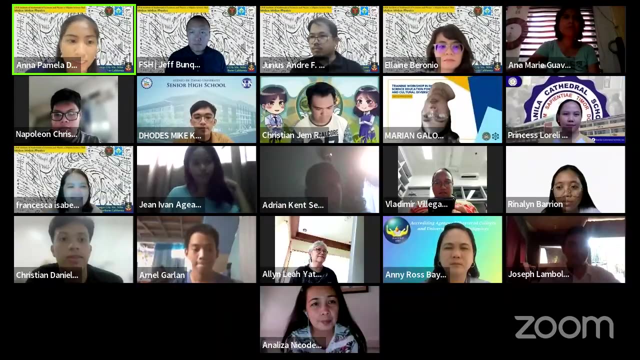 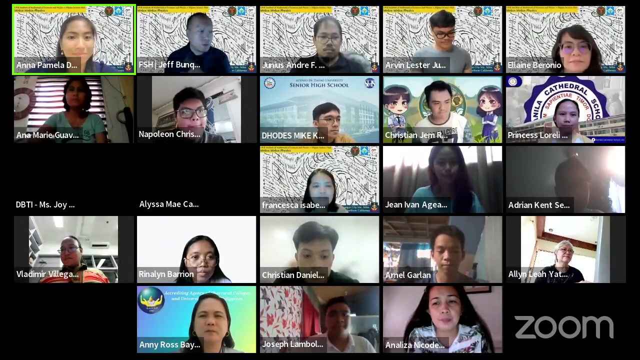 But before we leave the Zoom meeting, we would like to request everyone to turn on their cameras for our photo op. Sir Arvin, can you give us a screenshot? And also, by the way, Ms Ella. we also dropped the link.